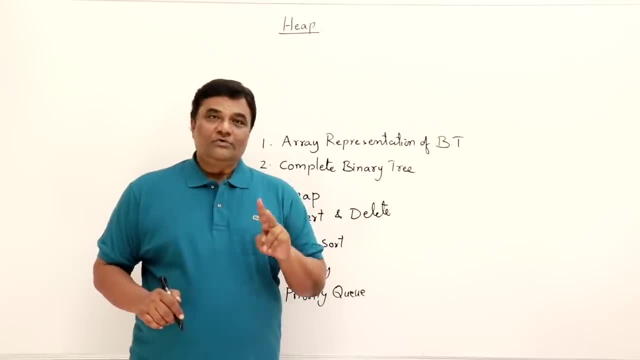 Now, before I start, I have to say something. See, I have two courses in Udemy. One is for CPUs- C++. Second one is for data structures. Both the courses are for beginner level as well as advanced level. Means if you already know data structure and C++, you have a lot of things to learn there. And also if you are a beginner, if you have never done any programming, then you can take up C++ course and start learning programming. And both the courses are suitable for academics as well as for interviews. So C++ programming- one course is there That is from beginners to beginners. 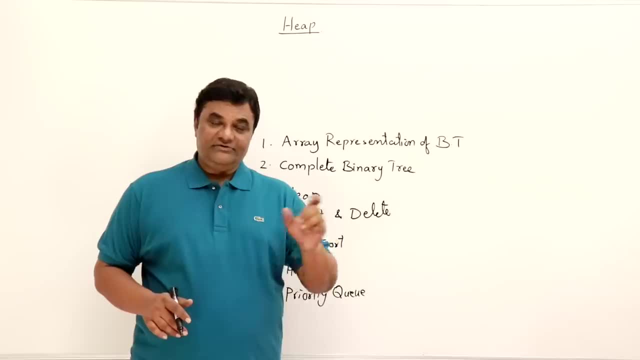 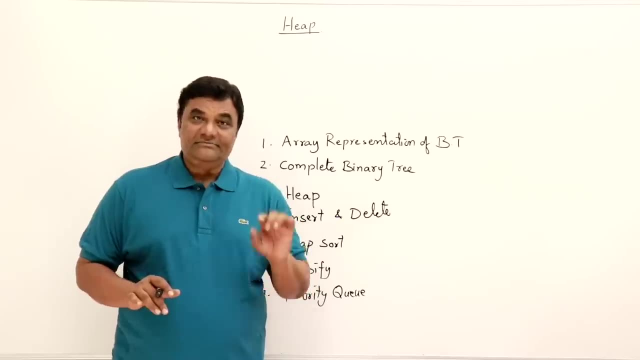 You can learn up to the level of interview. You can crack any interview. Then data structure course using C and C++ and some algorithms are there. It is not complete algorithm, It is just a data structure using C and C++ And few algorithms are there. So that subject is for academics as well as for cracking job interviews or coding interviews. So I have covered all the topics in greater detail So that will definitely improve your skills. So you can buy those two courses. Those are paid courses. 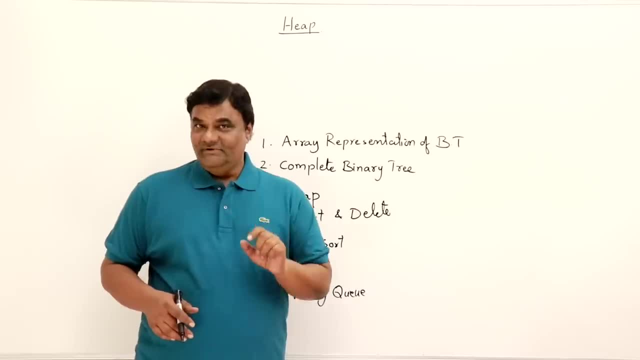 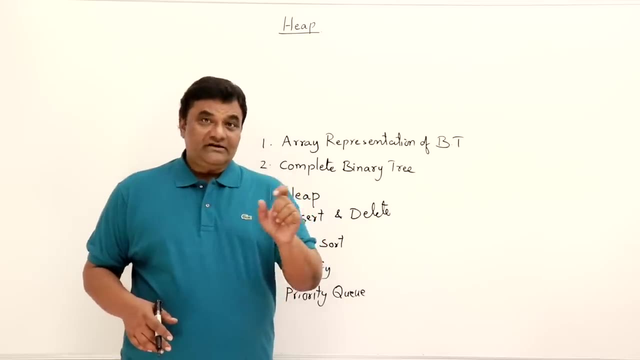 Those are not free And please don't ask for free coupons. The link for those courses is given in the description. You can check the description And there is a discount code. is there? Discount coupon code is there. That is around $10 or $11.. So you can click and go to Udemy And if more discounts are applicable, Udemy will give you that discount. Don't worry about that. If still it can be reduced, it will reduce it. So I suggest you take this course and by clicking on this link you go there. So let us start. 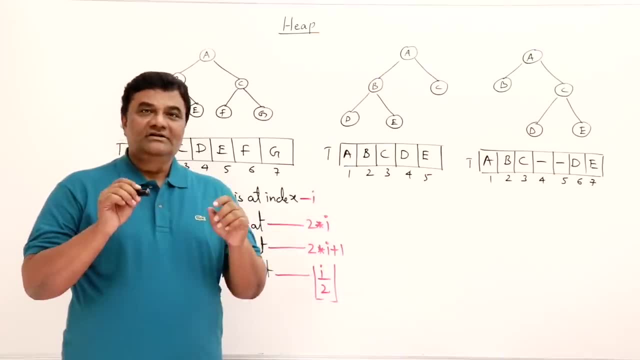 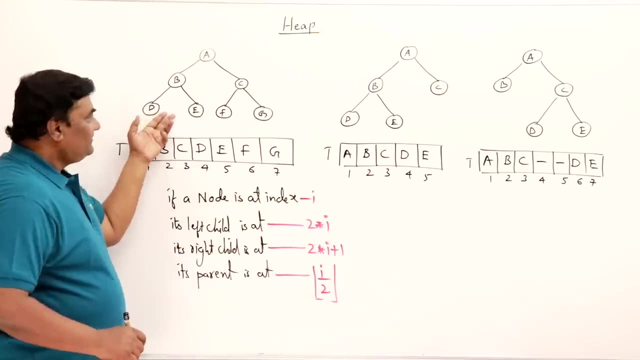 Let us start with the topic. First. I will discuss about representation of a binary tree using array. So here I have some examples. This is a binary tree. I have taken alphabets here So that easy to read. This is a binary tree And if I have to store it in an array, this is an array I already have taken In the C. C++ programming array starts from index 0. But here I have taken from 1 onwards. 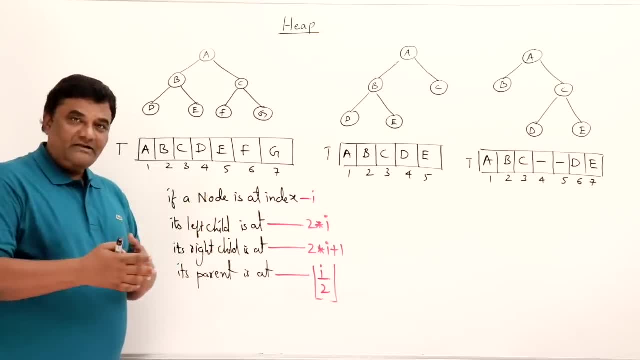 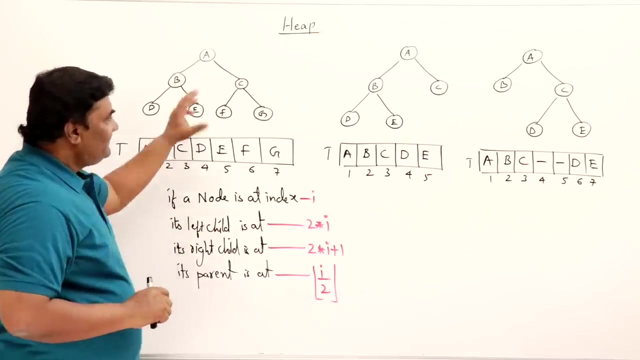 is just a theoretical on paper. when you want to program, write a program, then you can start from index 0 also. but usually this is studied by taking index 1 onwards, so i have taken index 1. then these elements are stored here. so how they are stored, see for storing a binary tree. 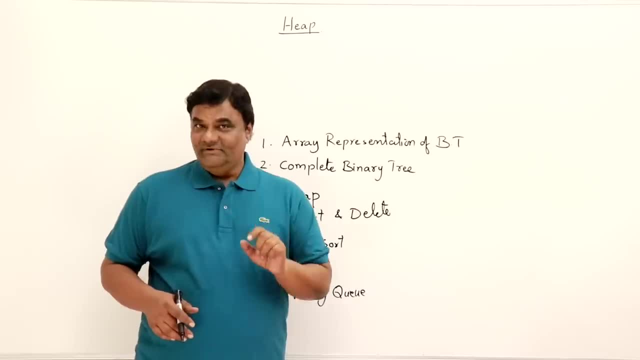 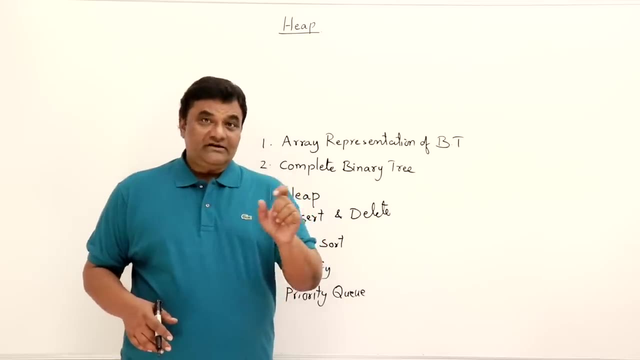 Those are not free And please don't ask for free coupons. The link for those courses is given in the description. You can check the description And there is a discount code. is there? Discount coupon code is there. That is around $10 or $11.. So you can click and go to Udemy And if more discounts are applicable, Udemy will give you that discount. Don't worry about that. If still it can be reduced, it will reduce it. So I suggest you take this course and by clicking on this link you go there. So let us start. 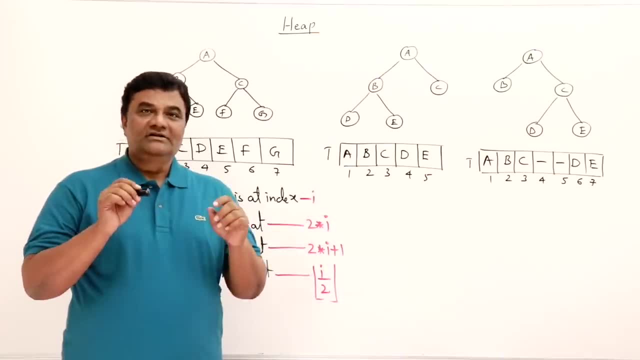 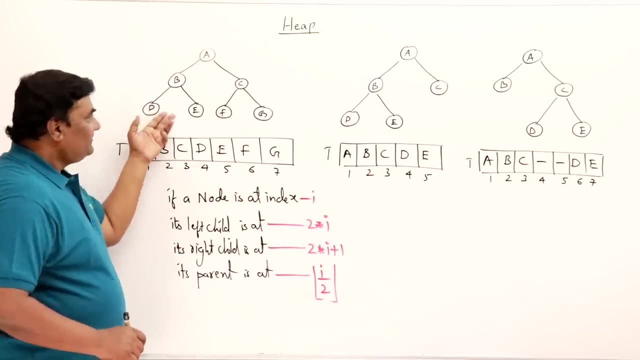 Let us start with the topic. First. I will discuss about representation of a binary tree using array. So here I have some examples. This is a binary tree. I have taken alphabets here So that is easy to read. This is a binary tree And if I have to store it in an array, this is an array I already have taken In C C++ programming array starts from index 0. But here I have taken from 1 onwards. So this is a binary tree And if I have to store it in an array, this is an array I already have taken In C. C++ programming array starts from index 0. But here I have taken from 1 onwards. So this is a binary tree And if I have to store it in an array, this is an array I already have taken. In C C++ programming array starts from index 0. But here I have taken from 1 onwards. So this is a binary tree And if I have to store it in an array, this is an array I already have taken In C. 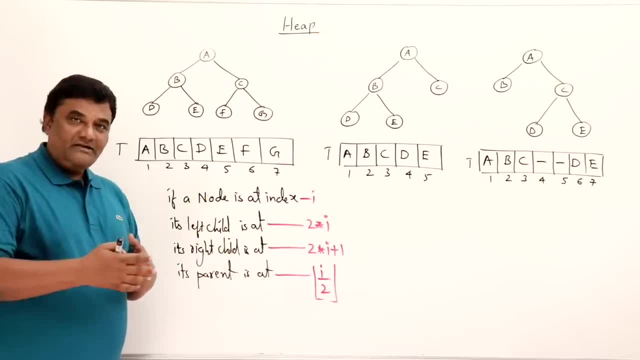 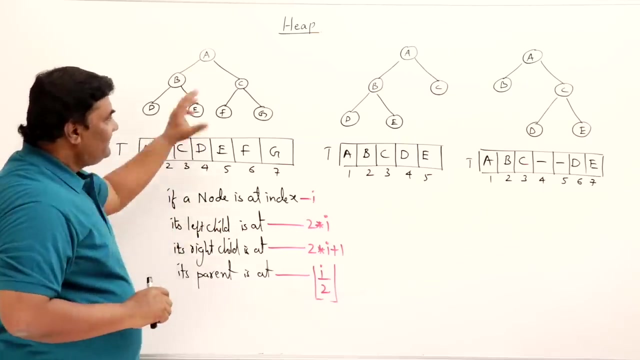 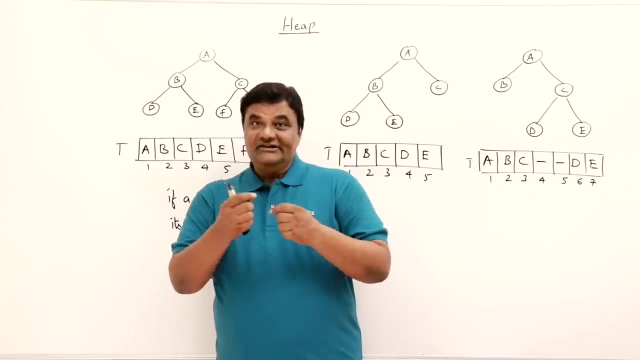 C++ programming array starts from index 0. But here I have taken from 1 onwards. So this is a binary tree, And if I have to store it in an array, this is an array I already have taken In C. So I have taken index 1.. Then these elements are stored here. So how they are stored, See for storing a binary tree, we have to take care of two things. One is we have to store all the elements. Second is the relationship between them: Who is a parent, Who is a child? Who is left child? Who is right child? So these are the two things. 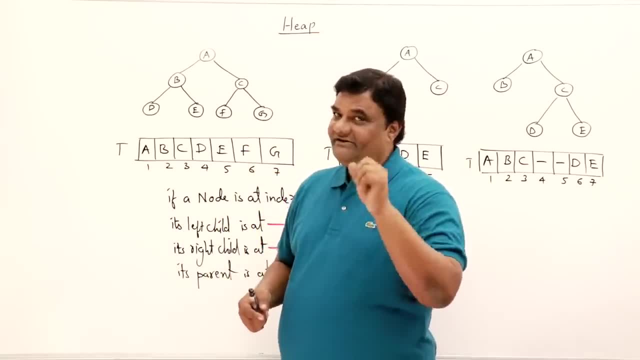 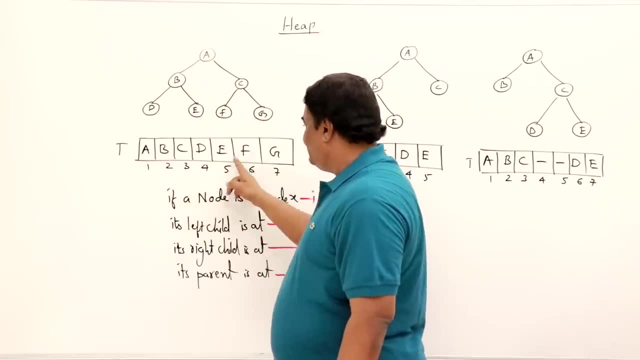 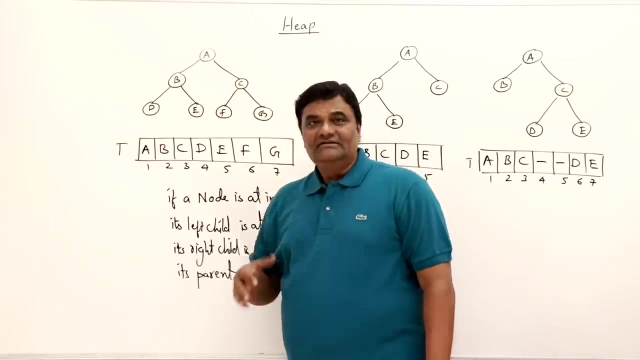 things that we have to take care, so elements and the relationship between the elements, so how they are preserved. watch here: see, the elements are stored here: a, b, c, d, e, f, g. so actually they are filled level by level: a, b, c, d, e, f, g. yes, they are filled level by level. then where is the 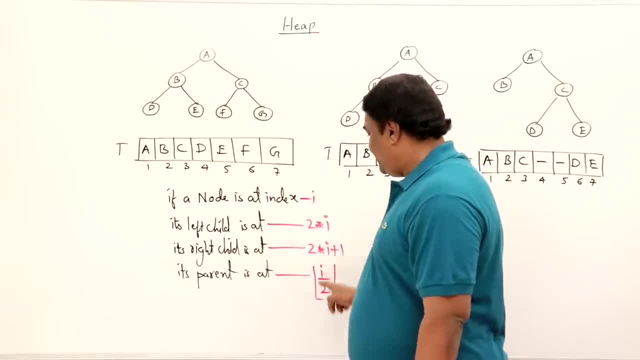 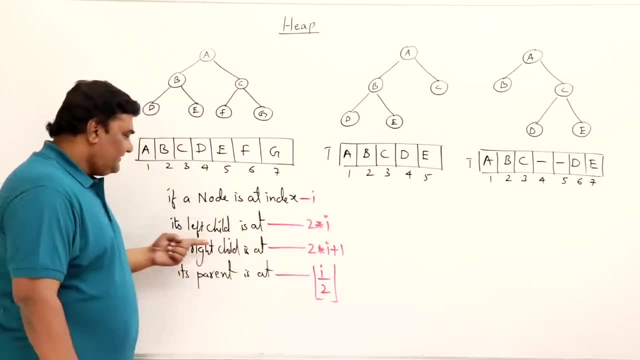 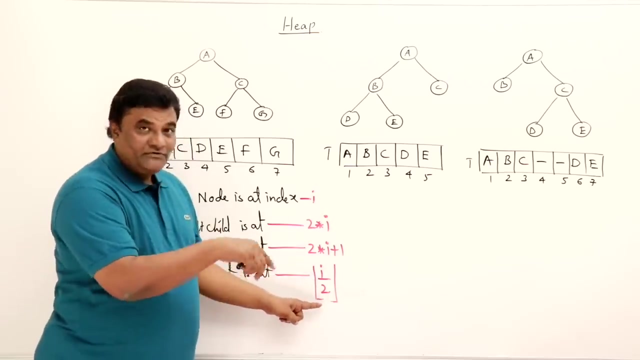 relationship, the relationship between them is formed by these formulas. so what are these? let us look at see: if any node is at index i, then its left child is at index 2 into i right child is 2, i plus 1 and its parent will be i by 2 floor value. so let us look into this example and observe. 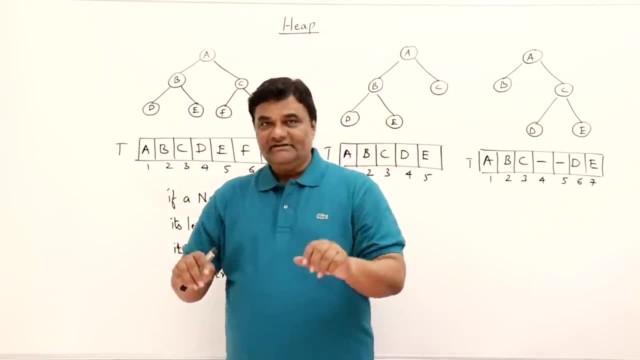 we have to take care of two things. one is we have to store all the elements. second is the relationship between them: who is a parent, who is a child, who is left child, who is right child? so these are the things that we have to take care, so elements and the relationship between the elements. 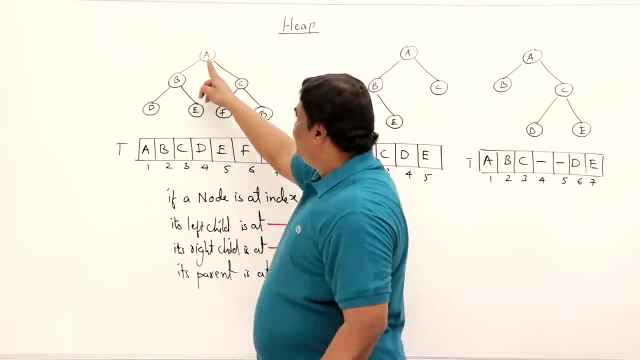 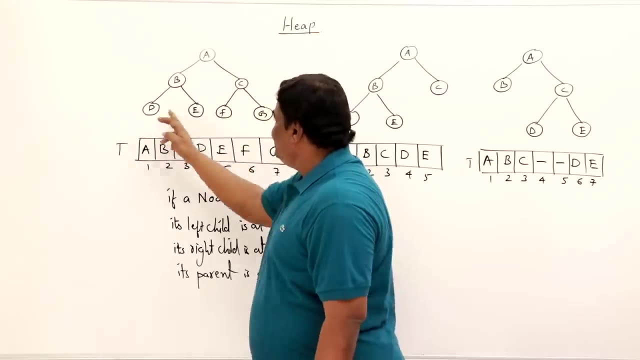 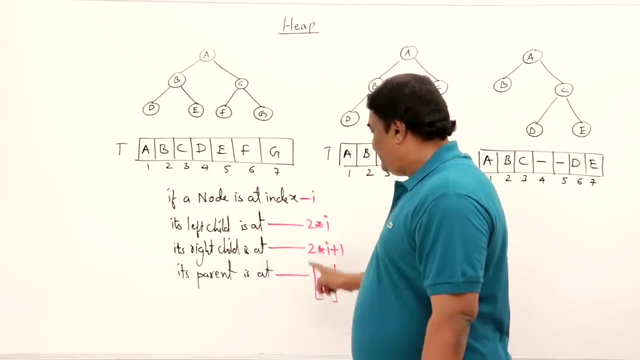 so how they are preserved. watch here: see, the elements are stored here: a, b, c, d, e, f, g. so actually they are filled level by level: a, b, c, d, e, f, g. yes, they are filled level by level. then where is the relationship? the relationship between them is formed by these formulas, so what? 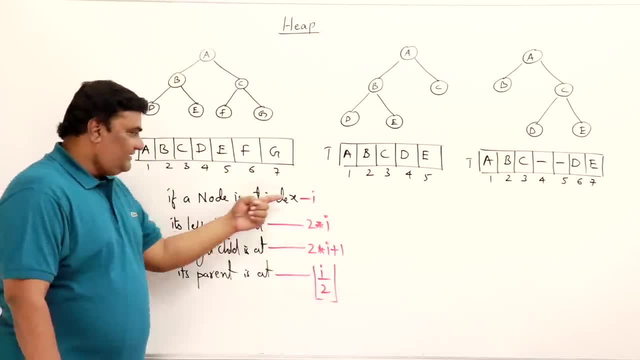 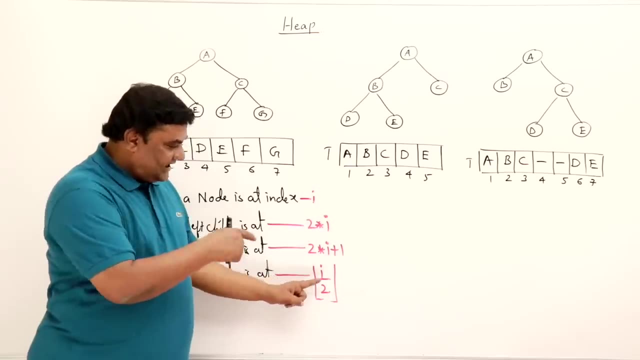 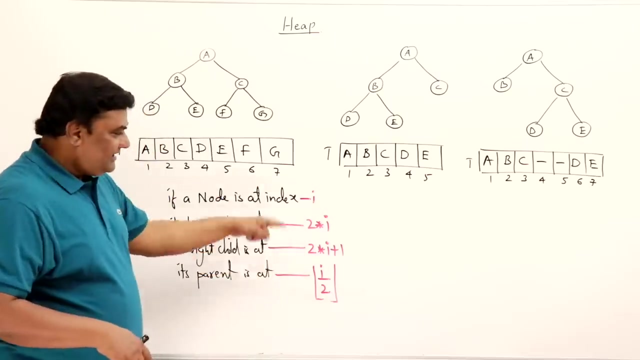 are these. let us look at see: if any node is at index i, then its left child is at index 2 into i right child is 2i plus 1 and its parent will be i by 2 floor value. so let us look into this example and observe: really these formulas are used here or not. let us 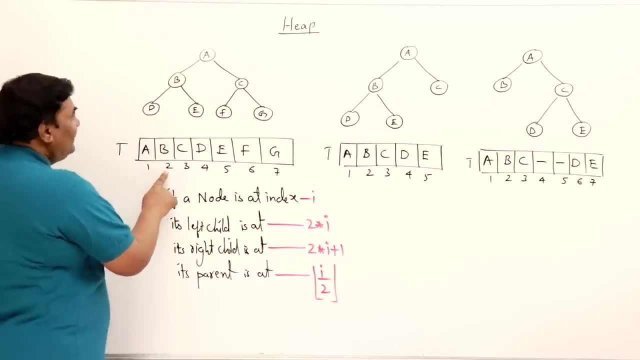 check b. b is at index 2 who is the left child of b d. so where it should be 2 into i, so 2 into 2, 4, yes, it is at 4.. then e is right child, where it should be 2 into i plus 1, 2 into 2. 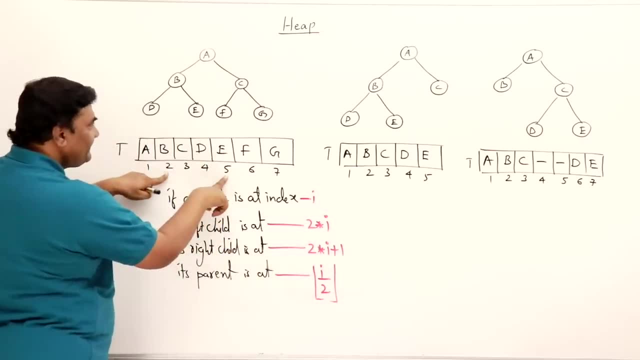 plus 1, that is 5.. so check on 5. yes, then c c is at index 3, then its left child, f, so 2, 3, 6, so it should be 6. yes, then a g is the right child. it should be 2 into i plus 1, 2 into 3 plus 1, 7. yes, 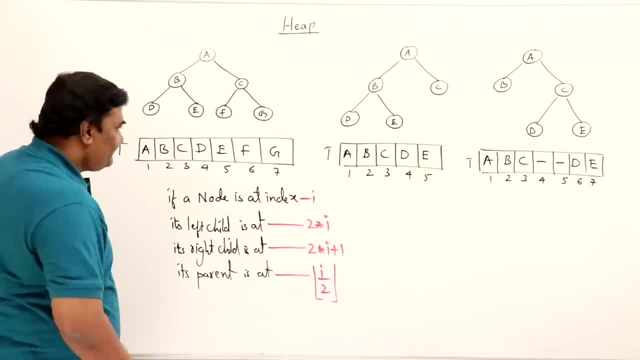 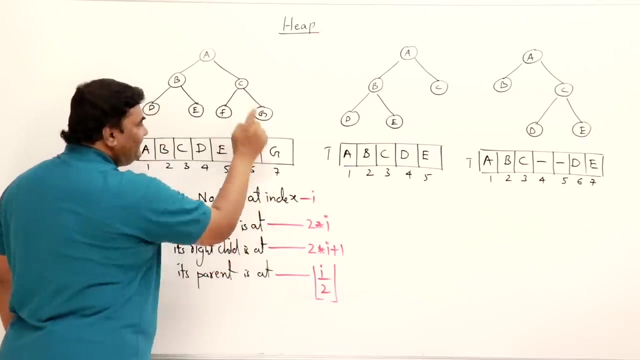 it is at 7.. so, yes, these are followed. now one more thing: f, who is the parent of f? this is 6. 6 by 2 is a. 3. go to 3. yes, c is the parent. so you check here in the tree. then for 7, this one g, who is the parent? c? 7. 7 by 2, 7 by 2 is 3.5. but we have to. 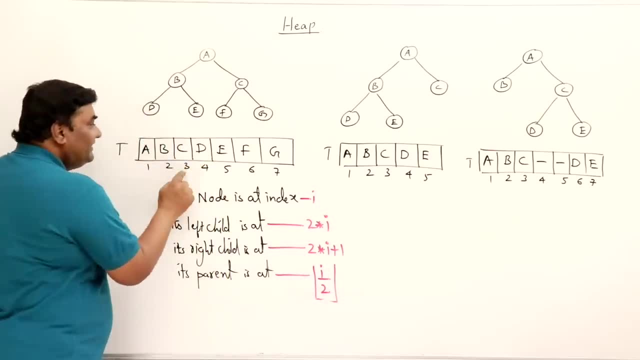 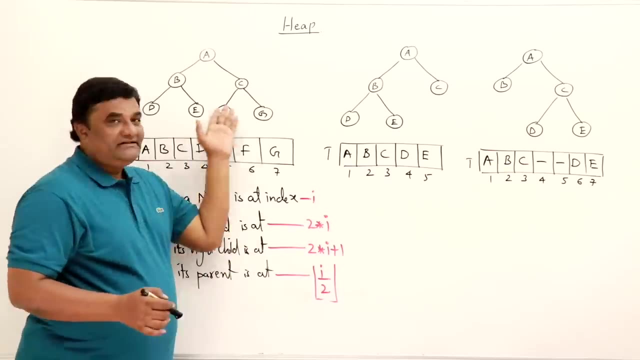 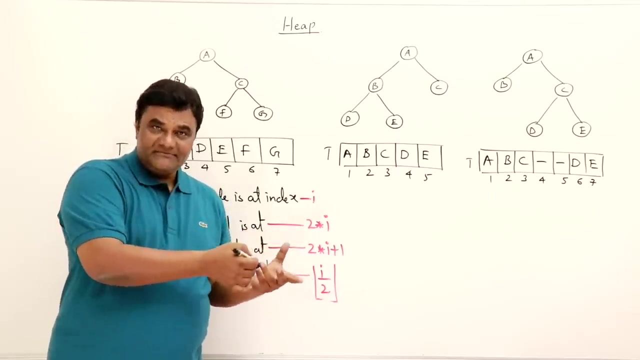 take floor valuements, just 3, so go to index 3. yes, c is there. so this gives the parent. so now we learn that actually these elements are stored by following the formula. now, every time you can't use the formula and put them right. so, instead of using the formula, one thing we do is. 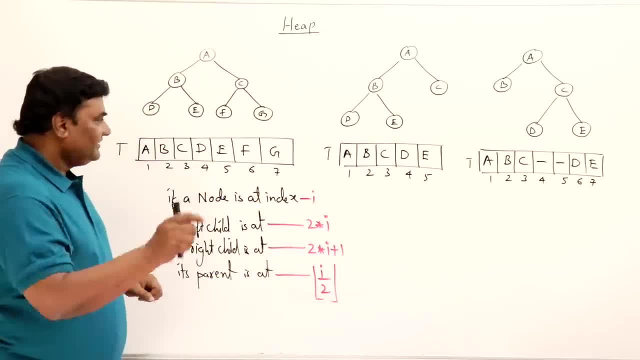 really these formulas are used here or not. let us check b. b is at index 2, who is the left child of b d. so where it should be 2 into i, so 2 into 2, 4. yes, it is at 4. b 2 into 2. 4 is at 2, so 2 into 2. 4 is at 2 m. and now let's look at the next one. let's talk about 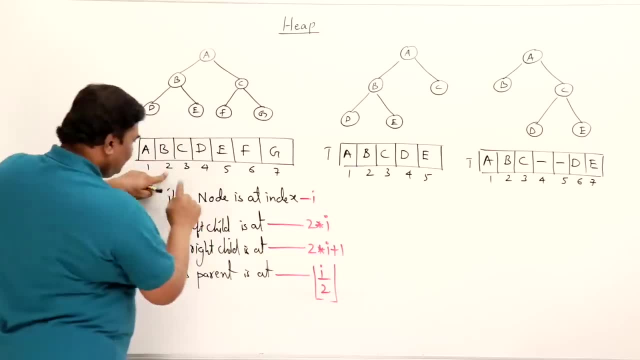 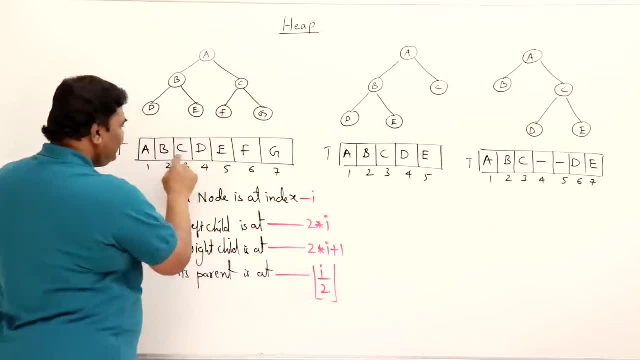 So check on 5, yes. Then C. C is at index 3.. Then it's left child F, so 2, 3, 6, so it should be 6, yes, Then G is the right child. it should be 2 into I plus 1, 2 into 3 plus 1, 7, yes, it is at 7.. 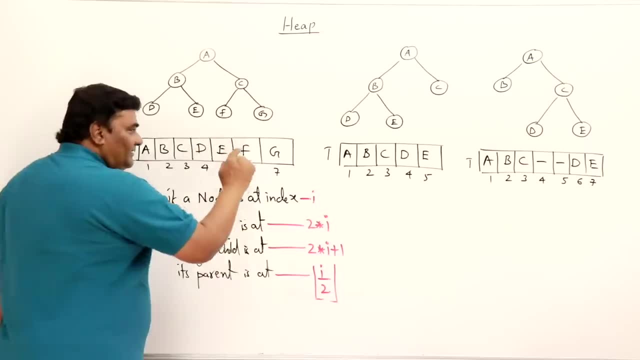 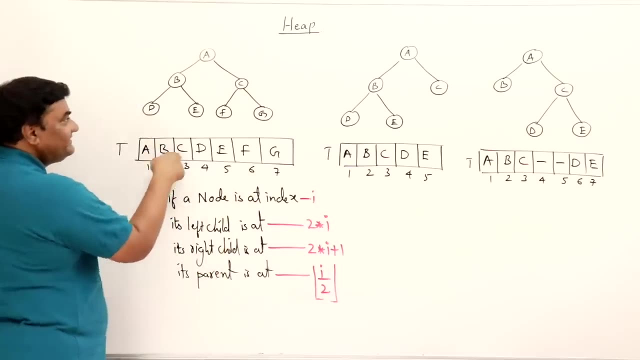 So, yes, these are followed. Now one more thing: F, who is the parent of F? This is 6.. 6 by 2 is 3, go to 3,. yes, C is the parent. so you check here in the tree. 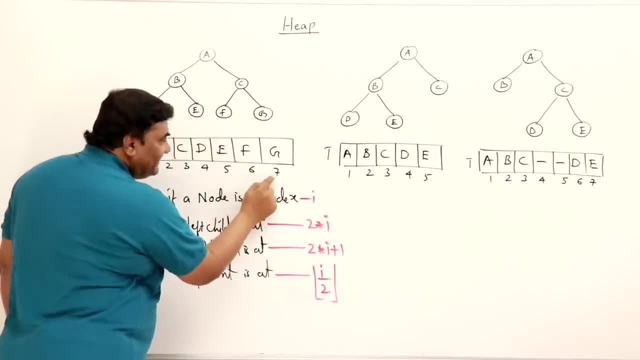 Then for 7, this one G, who is the parent C 7, 7 by 2, 7 by 2 is 3.5, but we have to take floor value and suggest 3.. So go to index 3,. yes, C is there. 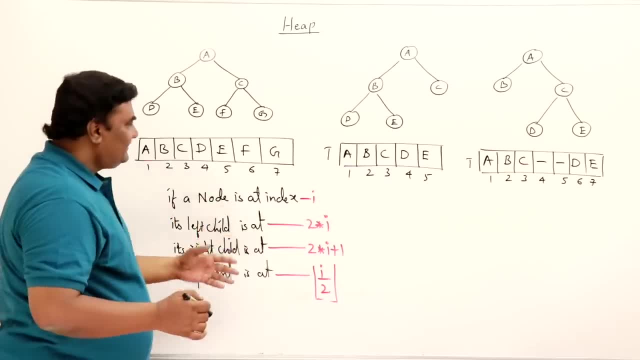 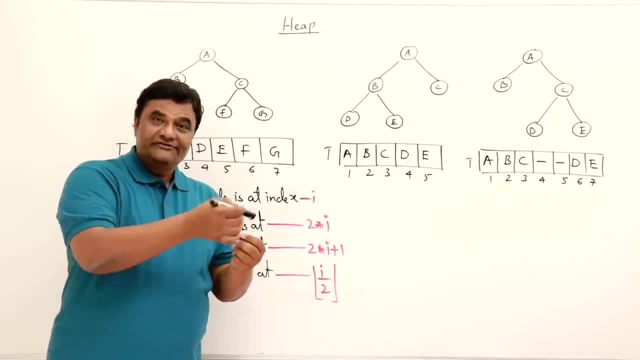 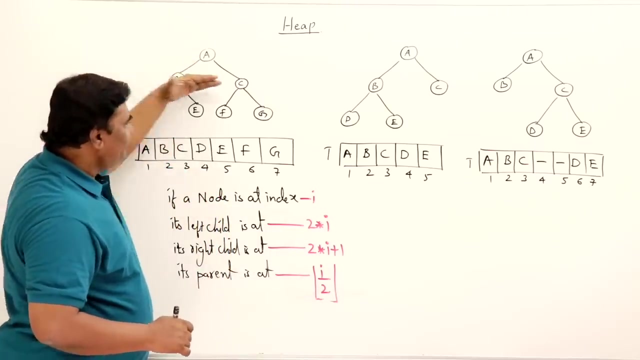 So this gives the parent. So now we learn that actually these elements are stored by following the formula. Now, every time you can't use the, So, instead of using the formula, one thing we do is we fill them level by level: A, B, C, D, E, F, G. so that's it. 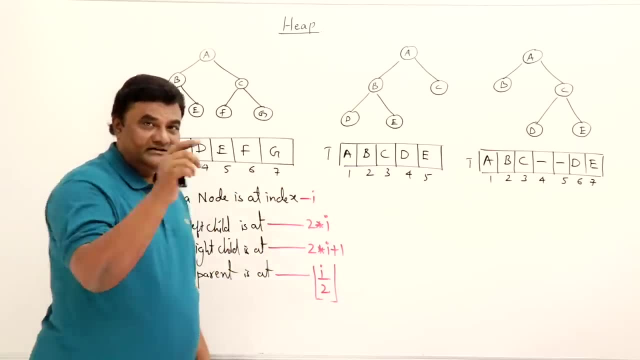 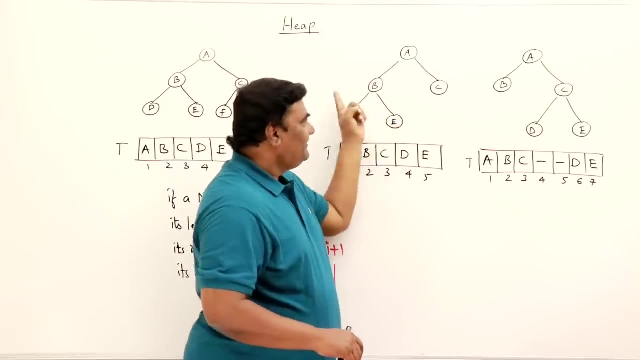 So these formulas are automatically followed. Now let us look at another example Here. I don't have these nodes, okay, no problem. Fill them level by level: A, B, C, D, E. tree ends here. so A, B, C, D, E. 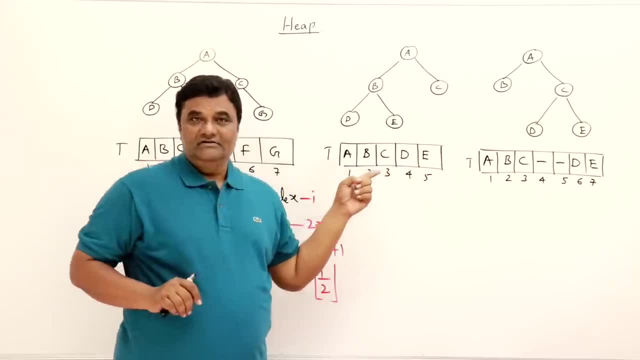 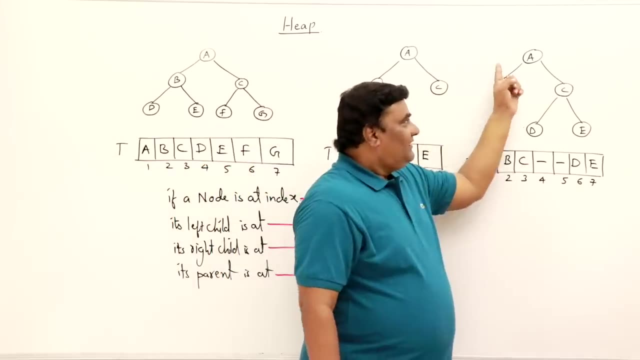 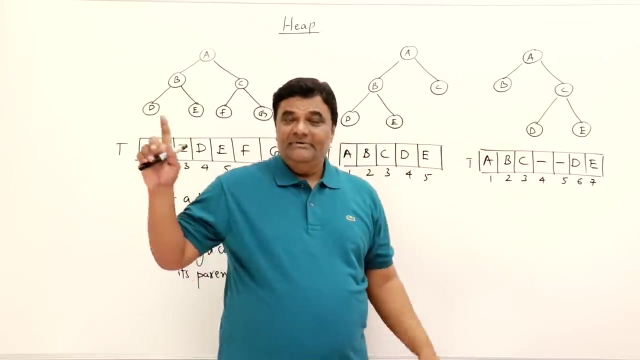 So if you apply those formulas, you check by yourself. they are followed: right, Left child, Right child and parent formulas are followed automatically. Now let us look at this one: A, B, C, then D. no, When I am filling level by level without using the formula, and I want the formulas to be followed automatically, 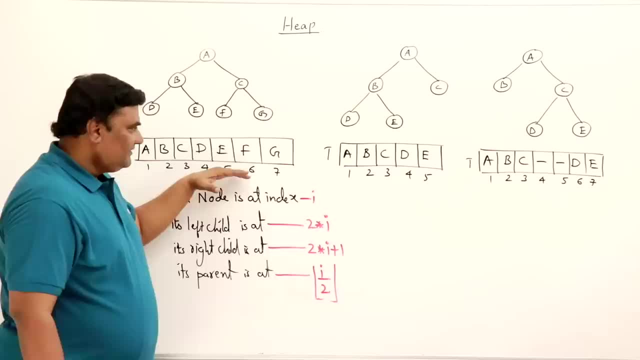 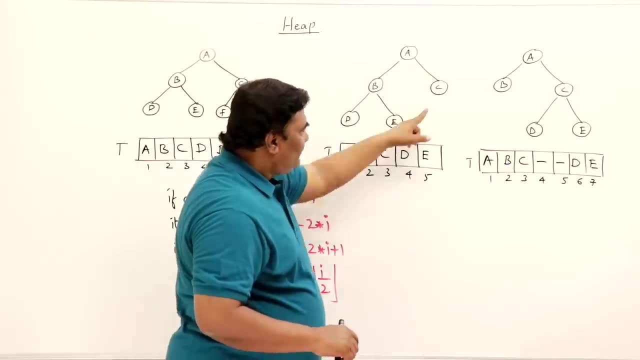 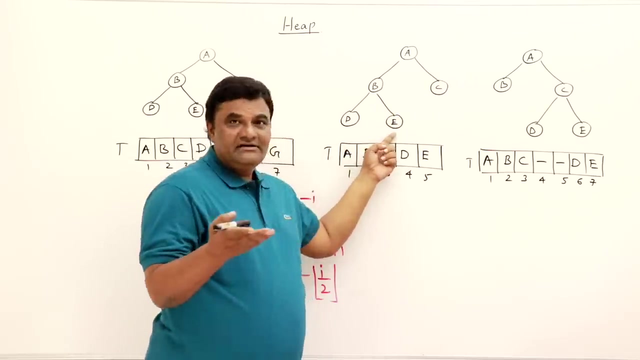 we fill them level by level: a, b, c, d, e, f, g. so that's it. so these formulas are automatically followed. now let us look at another example here. i don't have these nodes, okay, no problem. fill them level by level: a, b, c, d, e. tree ends here. so a, b, c, d, e. so if you apply those formulas, you 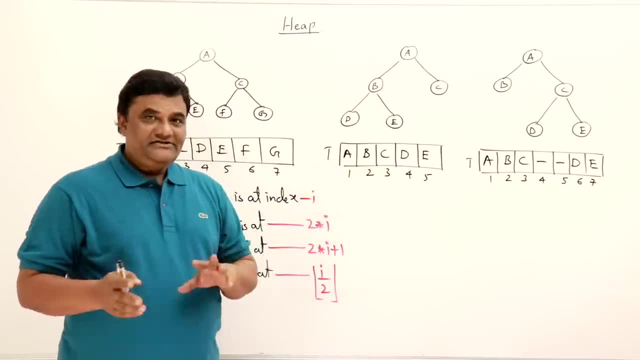 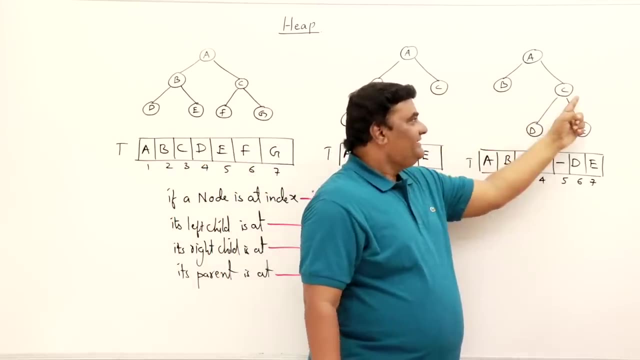 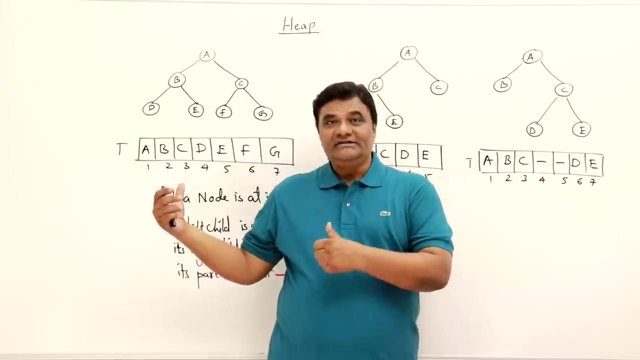 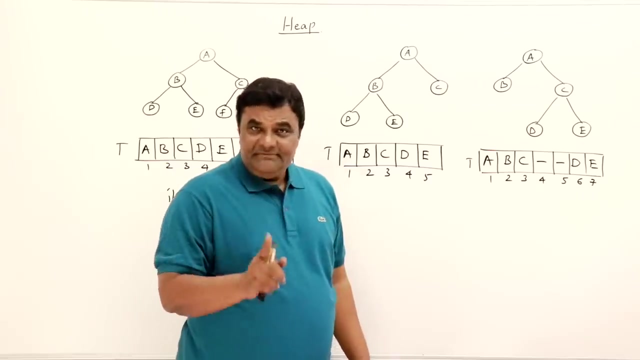 check by yourself. they are followed. right, left, child, right child and parent formulas are followed automatically. now let us look at this one: a, b, c, then d. no, when i am filling level by level without using the formula and i want the formulas to be followed automatically, then i should fill level by level and if any element is missing, i 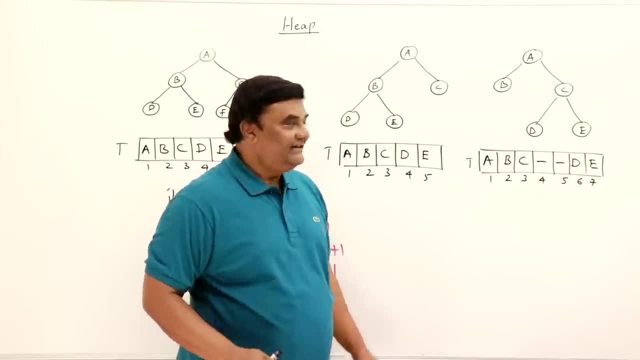 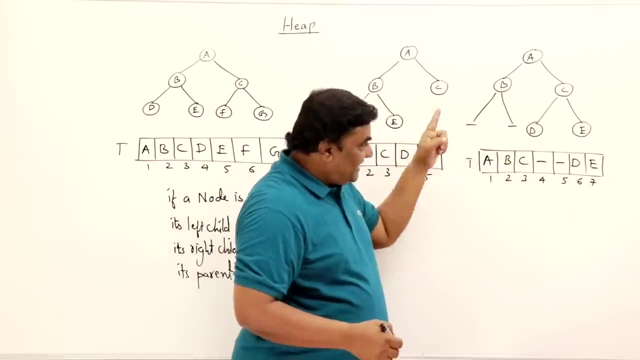 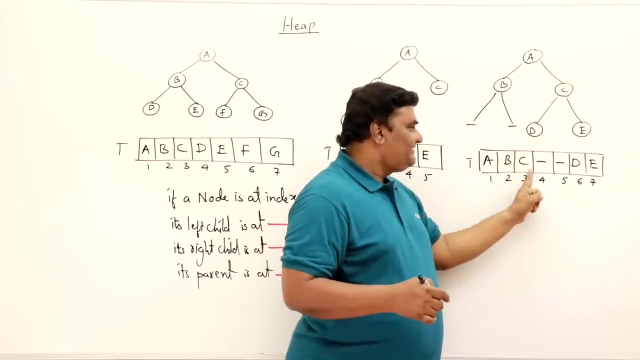 should leave a gap there. yes, this is the important point now. actually, b should have its left child, which is not there, right child, which is not there. so put a blank there. yes, a b c blank blank d e. a b c blank blank d e. this is how they are filled now. if you see d, who is a? 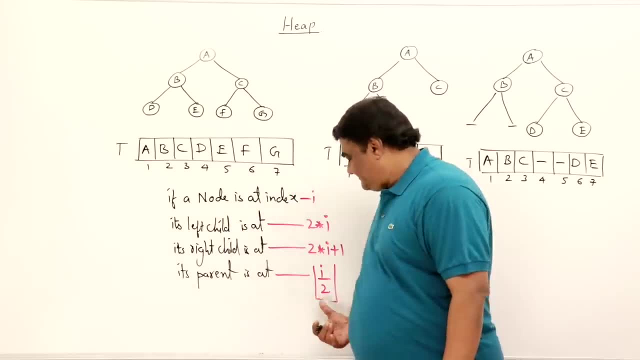 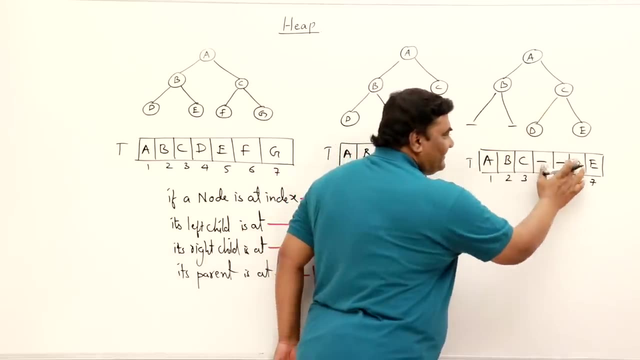 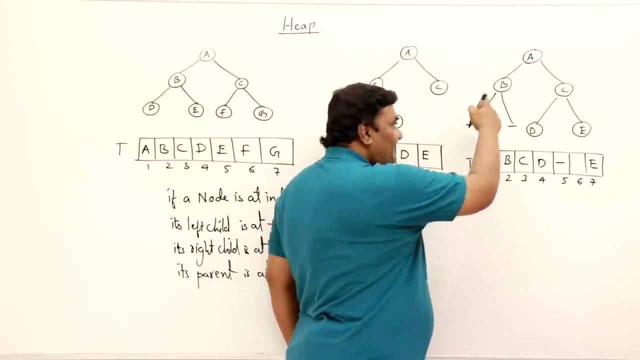 parent of d. six by two, this one, six by two, three, yes, three. who is there at three? c is there. if i don't write d there, if i write here, then it becomes a left child of b. that will be wrong, so it means is not there for b. so this place must be blank and d should be filled here. so, without following. 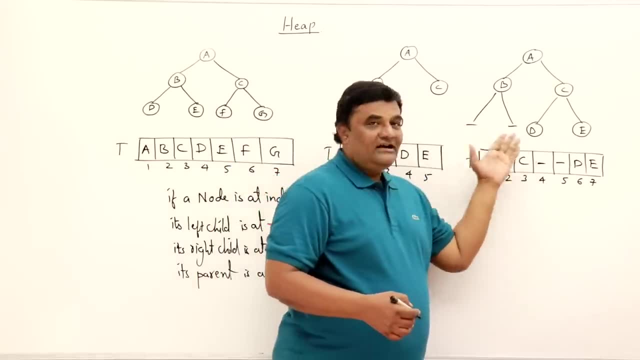 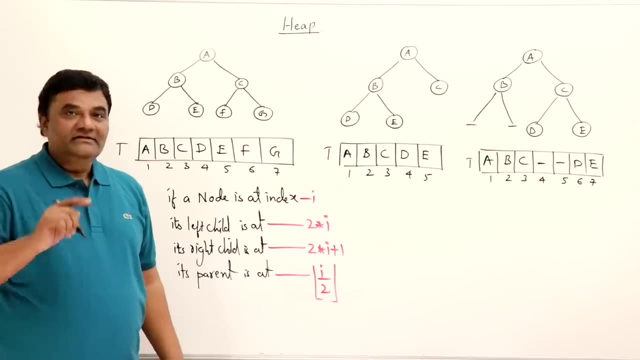 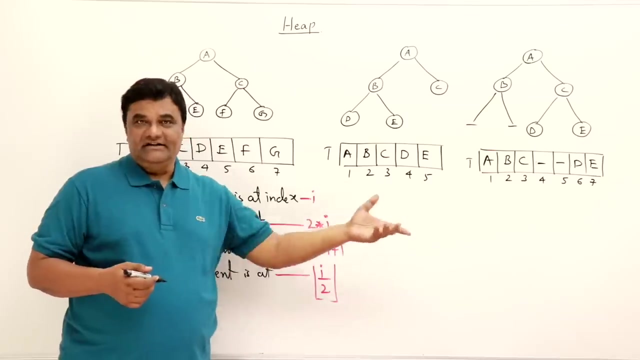 formulas. if you want to fill them, then make sure that if there are missing nodes you leave a blank there. so that's all about array representation of binary tree. that is done using these formulas. these formulas are for maintaining relationship and the elements are as it is stored in an array. 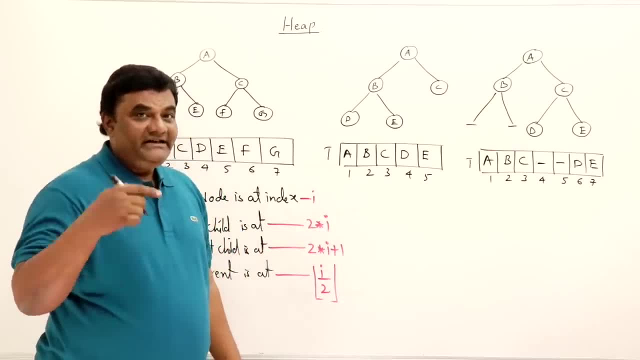 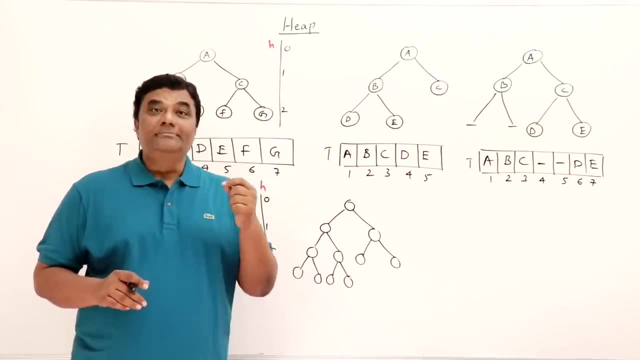 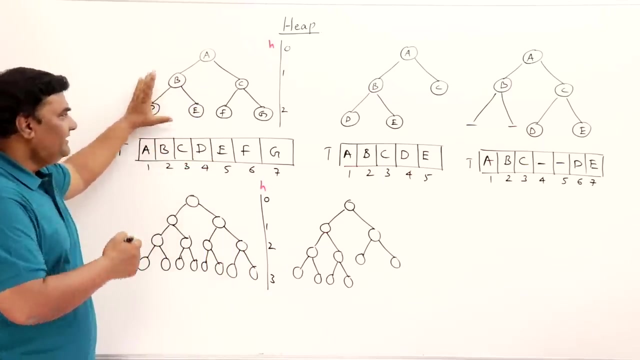 now. next, we will understand what is complete binary tree. now let us learn what is full binary tree and what is complete binary tree. so first, full binary tree. see this binary tree. this we have already seen it. so this is a full binary tree. what does it mean by full? see the height of a 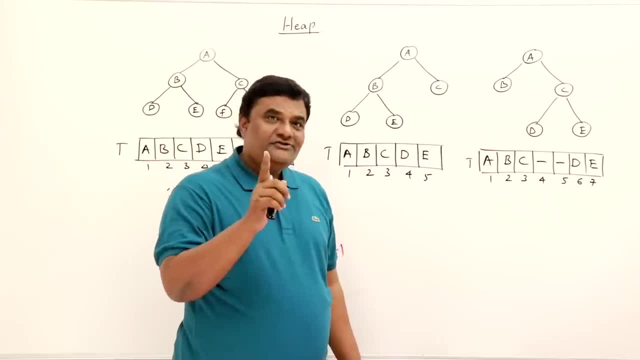 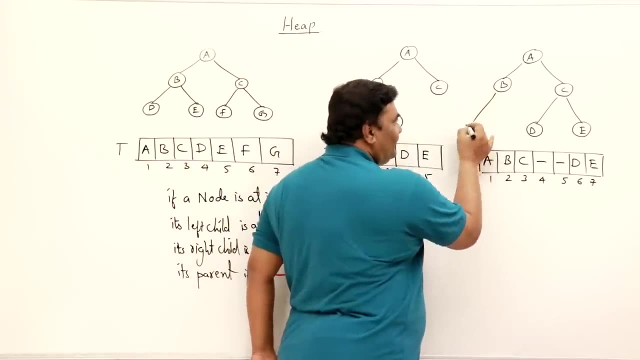 then I should fill level by level and if any element is missing I should leave a gap there. Yes, this is the important point Now. actually, B should have its left child, which is not there, Right child, Left child, which is not there. 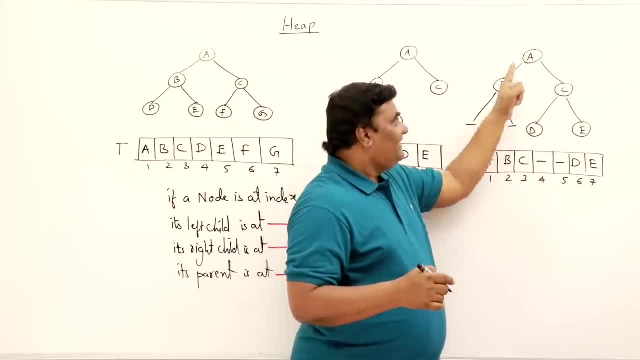 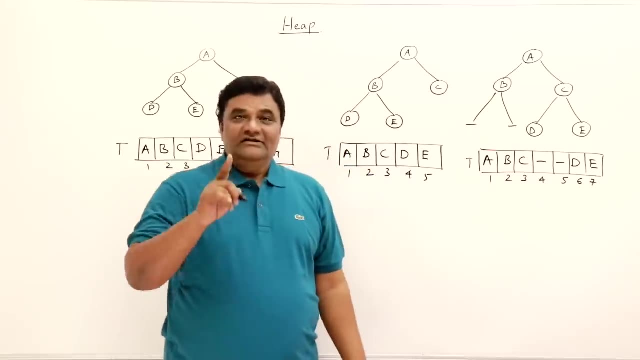 So put a blank there. Yes, A B C blank blank D E. A B C blank blank D E. This is how they are filled Now, if you see D, who is a parent of D. 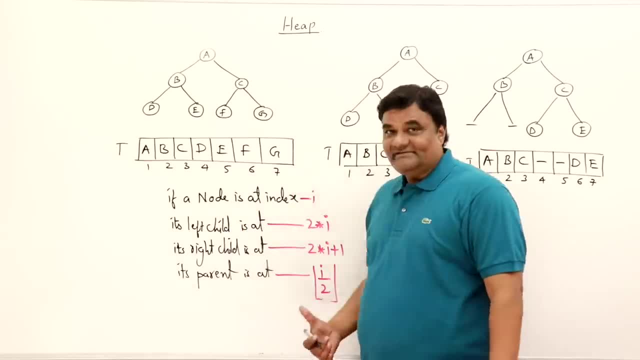 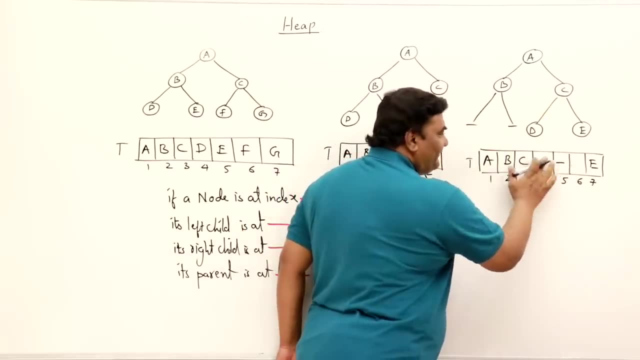 6 by 2, this one, 6 by 2, 3.. Yes, 3,. who is there at 3?? C is there. If I don't write D there, if I write here, then it becomes a left child. 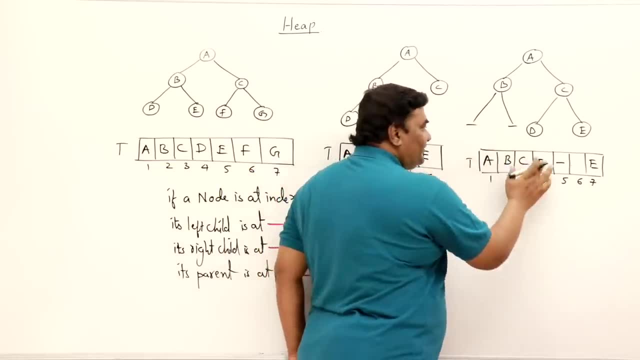 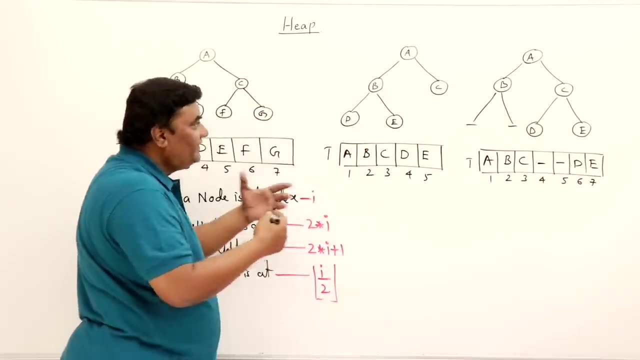 Left child of B. that will be wrong, So it means left child is not there for B. so this place must be blank and D should be filled here. So, without following formulas, if you want to fill them, then make sure that if there are missing nodes you leave a blank there. 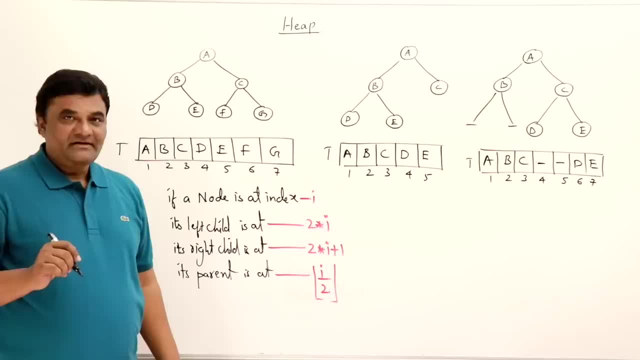 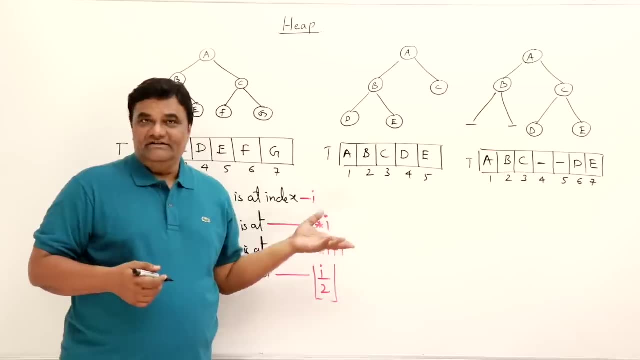 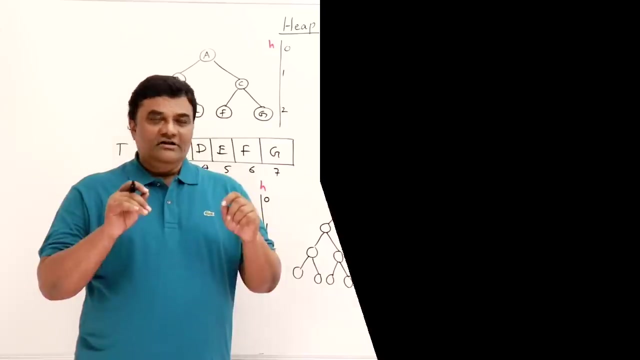 So that's all about array representation of binary tree. that is done using these formulas. These formulas are for maintaining relationship and the elements are, as it is, stored in an array. Now, next we will understand what is complete binary tree. Now let us learn. 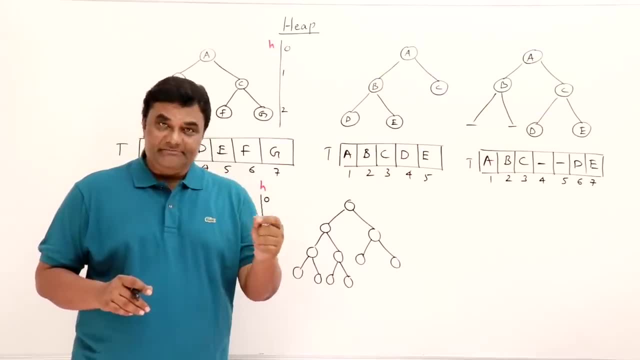 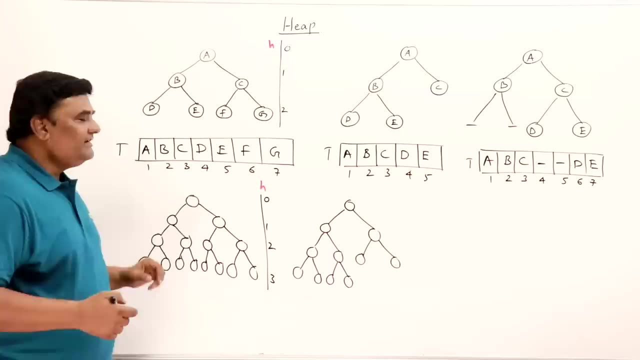 what is full binary tree and what is complete binary tree? So first, full binary tree. See this binary tree, this we have already seen it. So this is a full binary tree. What does it mean by full? See the height of a binary tree. this is 0, 1, 2, so the height is 2, 0, 1, 2.. 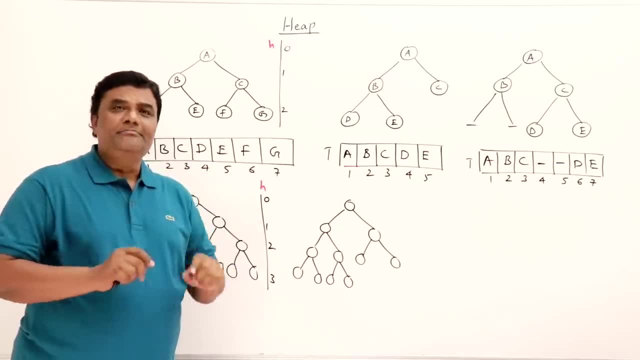 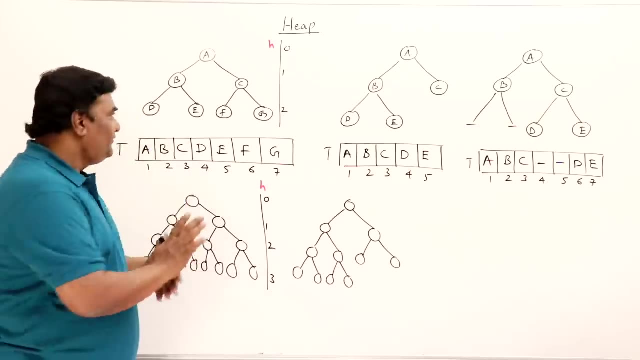 Height of a binary tree is 2. And in that height it is having maximum number of nodes. If you want to add any node, then the height will increase, And if you remove any node then this is missing. it is not having all possible node. 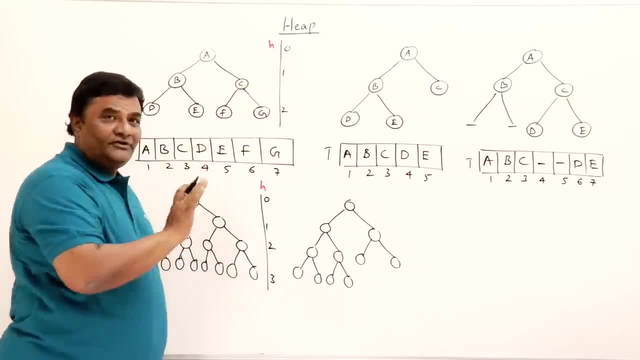 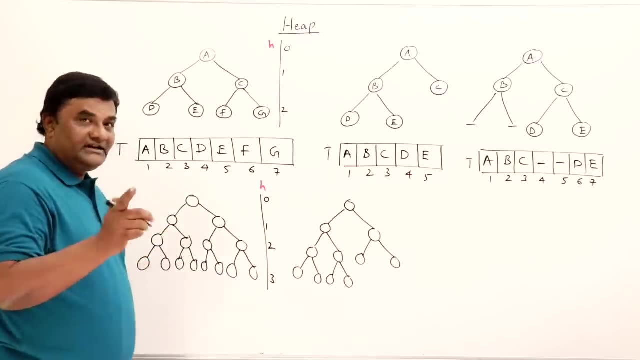 One more node is possible, so you can take this. So now this is having full in height 2.. Now this is in height 3, this is full binary tree. there is no space for any new node, So that tree is called as a full binary tree. 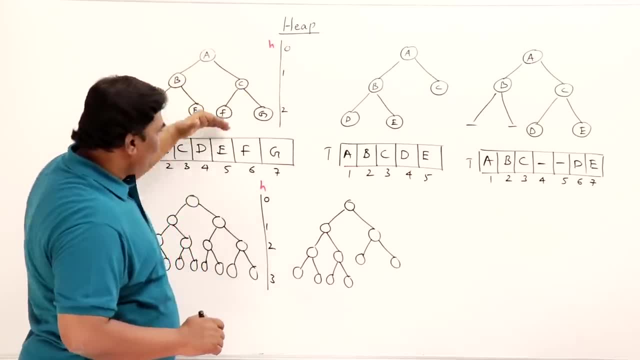 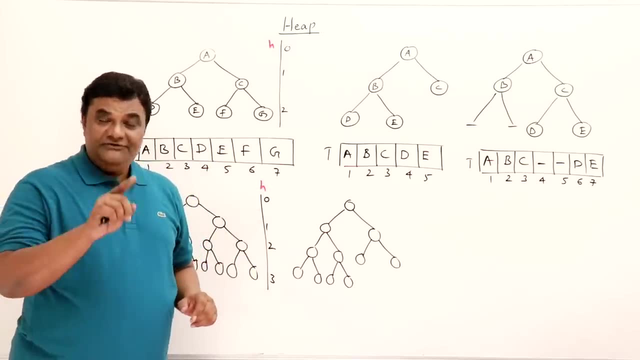 binary tree. this is 0, 1, 2, so the height is 2 0 1, 2. height of a binary tree is 2 and in that height it is having maximum number of nodes. if you want to add any node, then the height will increase, and if you remove any node then this is. 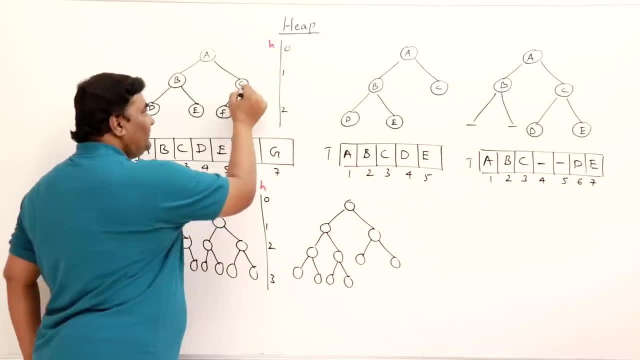 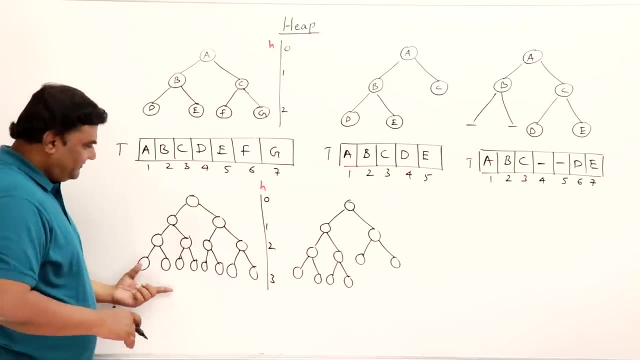 missing. it's not having all possible node. one more node is possible so you can take this. so now this is having full in height 2. now this is in height 3. this is full binary. there is no space for any new node, so that tree is called as a full binary tree. and if the height of a binary tree is h, 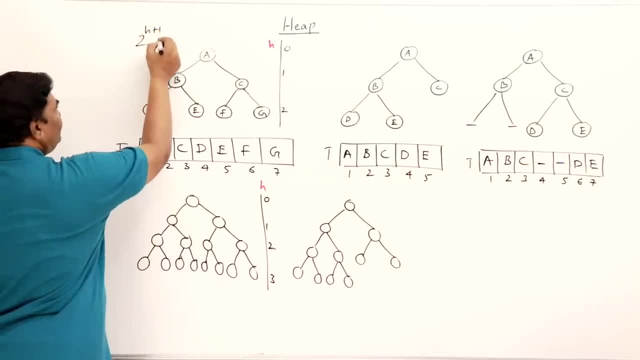 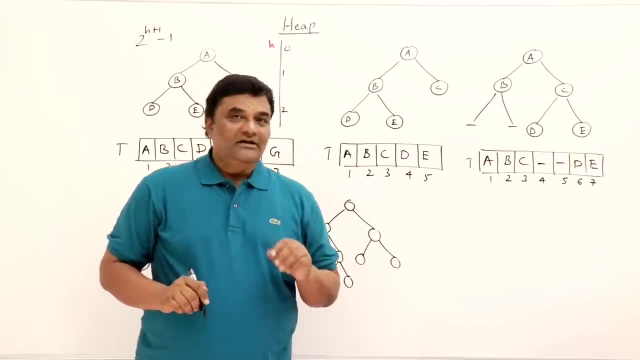 then a full binary tree can have 2 power h plus 1 minus 1 number of nodes, maximum, these many nodes. so a binary tree with maximum number of nodes is a full binary tree. now, what is complete binary tree? let us learn this. now see, look at this one when i have 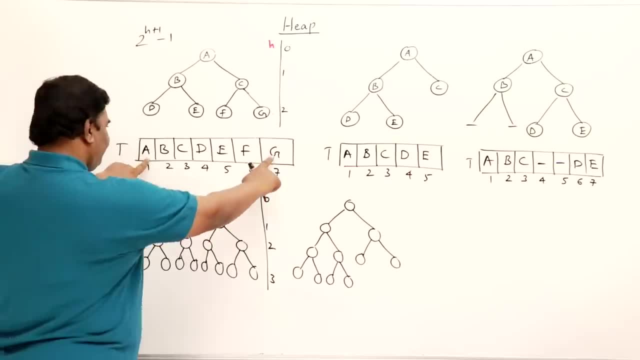 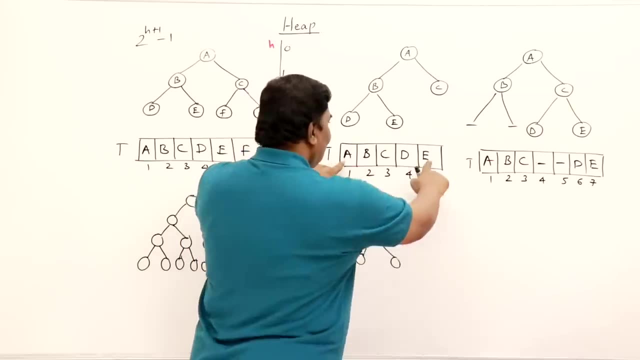 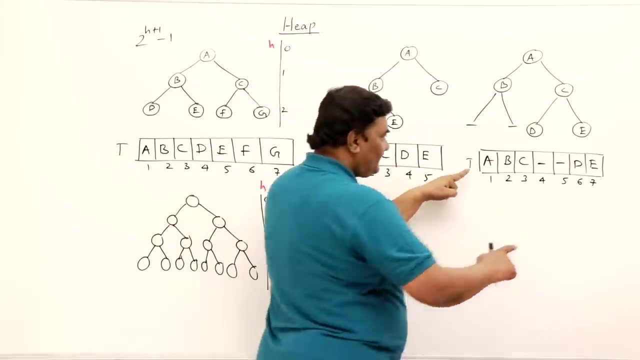 represented this in an array. then from last first element to the last element, there is no missing element. so this is complete. if you look at this, if you check the first and the last element, there is no missing element. it's a complete binary tree from the first element to the last element. if you check in an array, there are some missing elements. 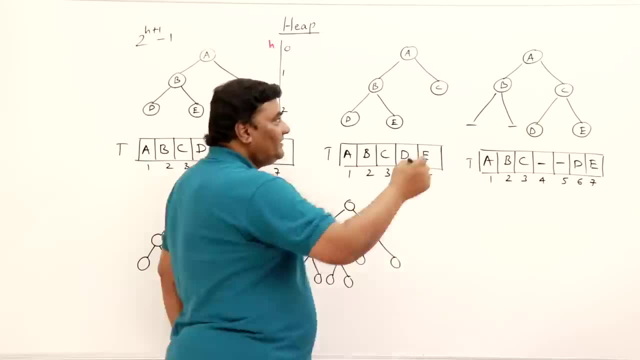 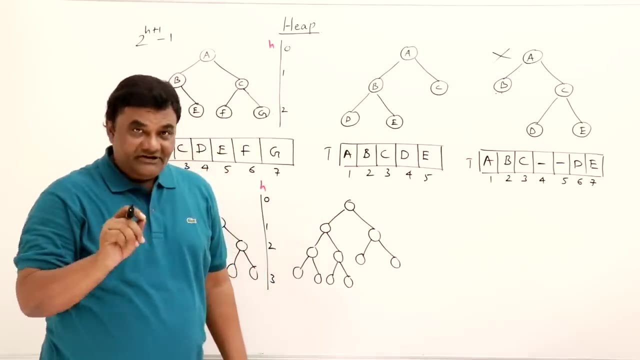 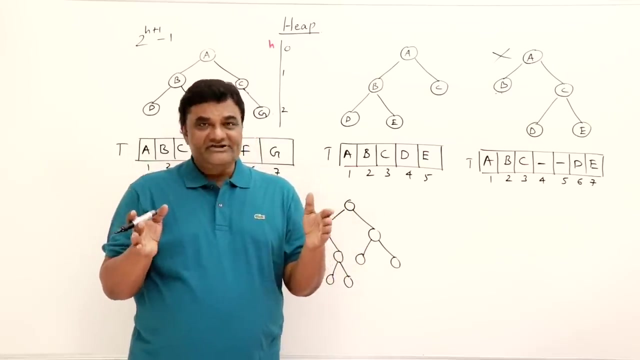 so even if there is a single missing element, it is not a complete binary tree. this is not a complete binary right. so the definition is. my definition is: if you represent a binary tree in an array, then there should not be any empty locations or gaps in between the elements. means from first. 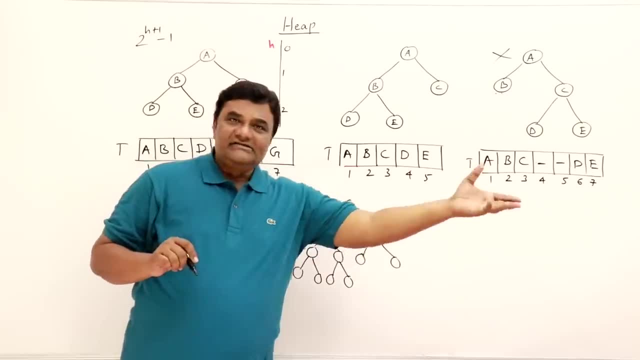 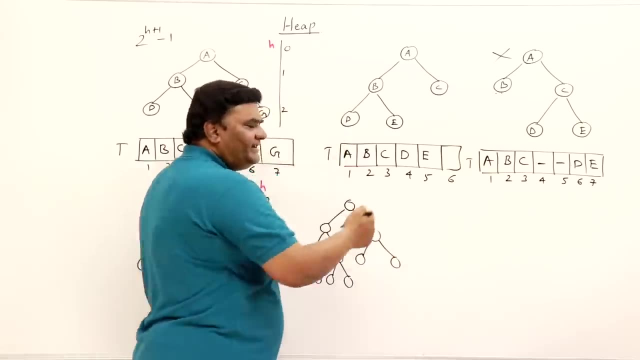 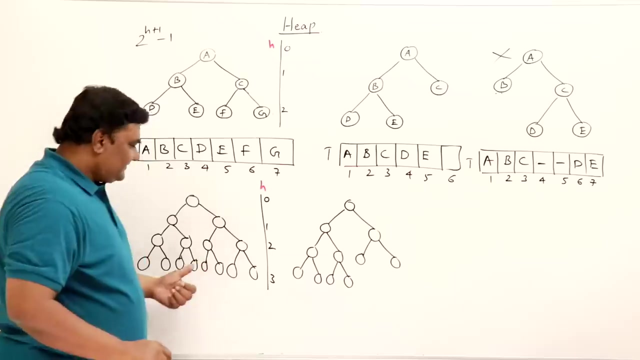 element to last element, in between, anywhere, right after the last element, space is there, then we, there is no problem. like suppose this array is having only five element. if i have one more, six, location, that is not a problem, right, but in between the elements, that is the important thing now. if you look at this now, you tell me whether it is complete or not. 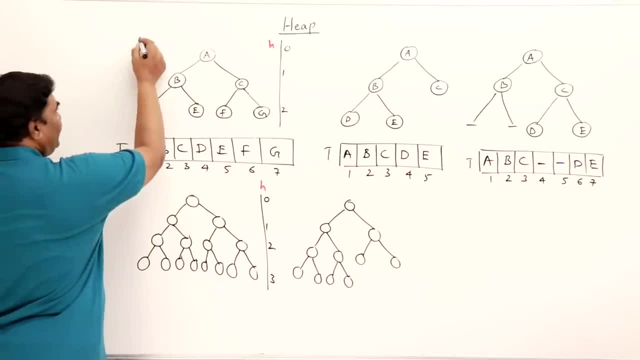 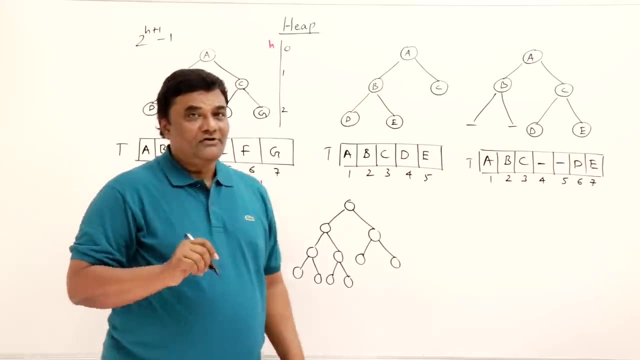 And if the height of a binary tree is h, then a full binary tree can have 2 power h plus 1 minus 1 number of nodes, maximum these many nodes. So a binary tree with maximum number of nodes is a full binary tree. 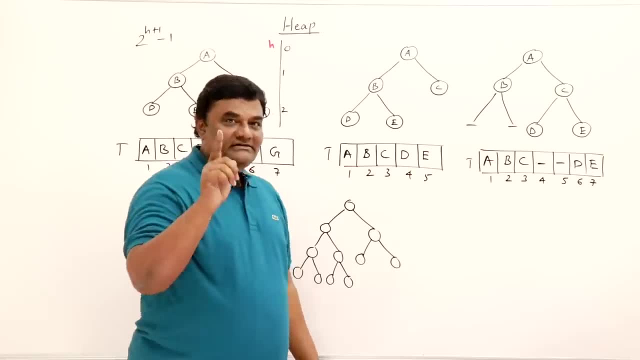 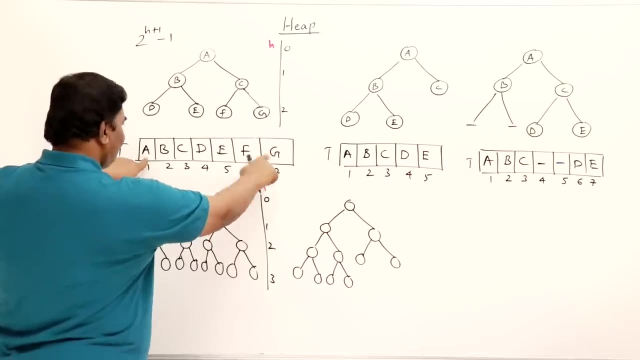 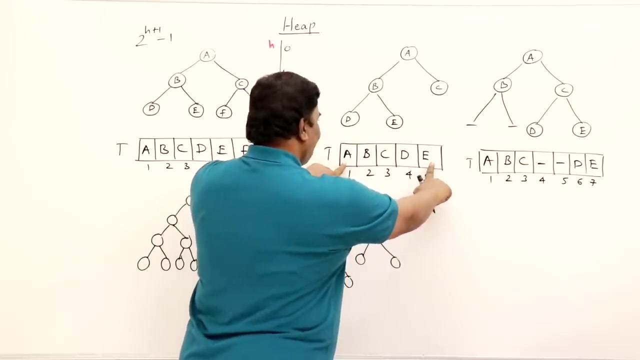 Now what is complete binary tree? Let us learn this. now, See, look at this one. When I have represented this in an array, then from last first element to the last element, there is no missing element. So this is complete. If you look at this, if you check the first and the last element, there is no missing element. 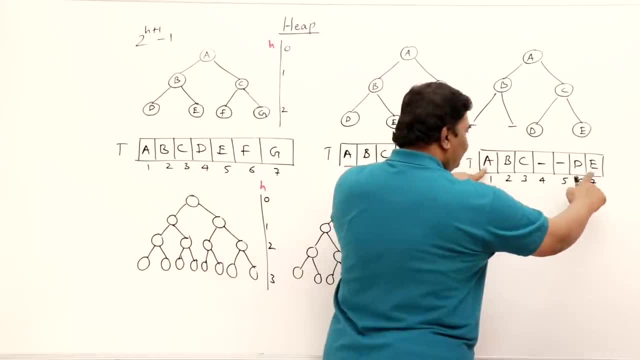 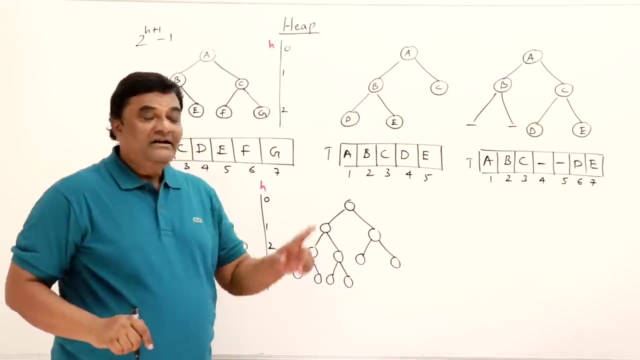 It's a complete binary tree here, from the first element to the last element. If you check in an array, there are some missing elements. So even if there is a single missing element, it is not a complete binary tree. This is not a complete binary tree. 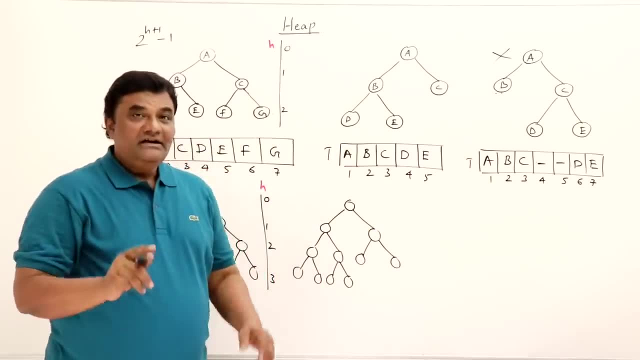 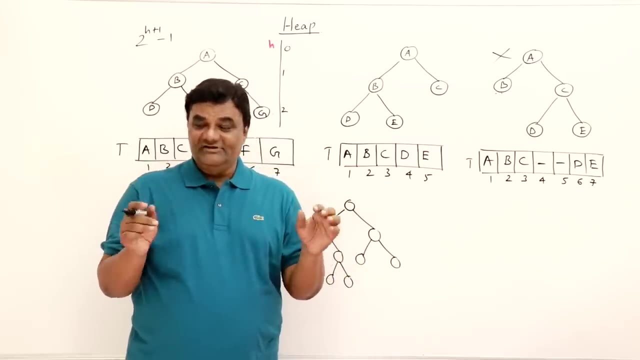 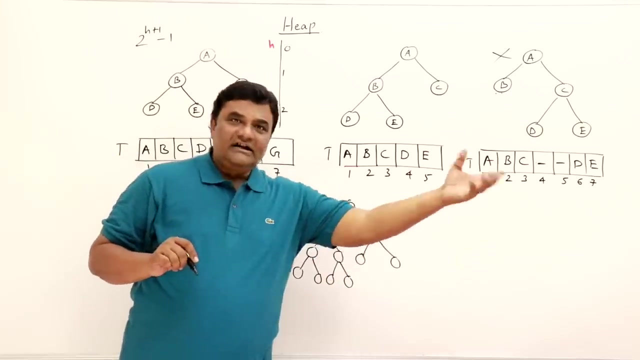 Right. So the definition is. my definition is: if you represent a binary tree in an array, then there should not be any empty locations or gaps in between the elements Means from first element to last element, in between, anywhere Right After the last element spaces. 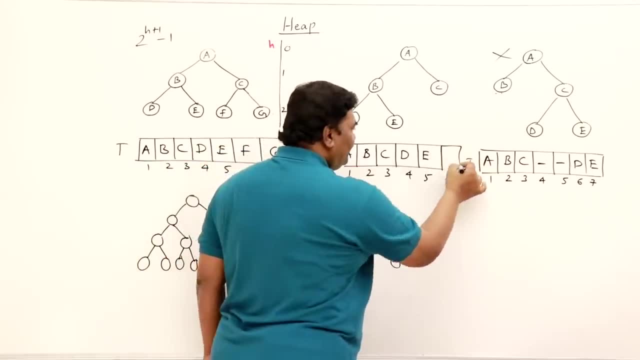 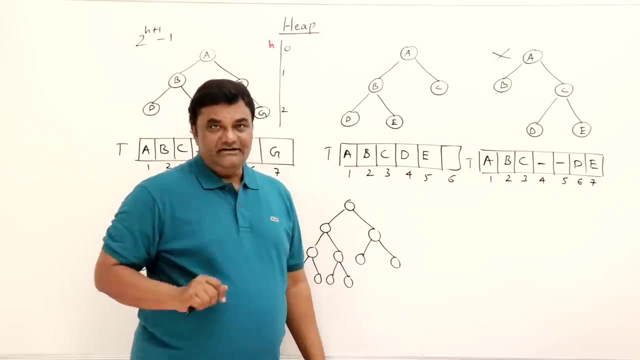 then there is no problem. Like suppose this array is having only five elements, If I have one more, six location, that's not a problem, Right, But in between the elements, that is the important thing. Now, if you look at this now, you tell me whether it is complete or not. 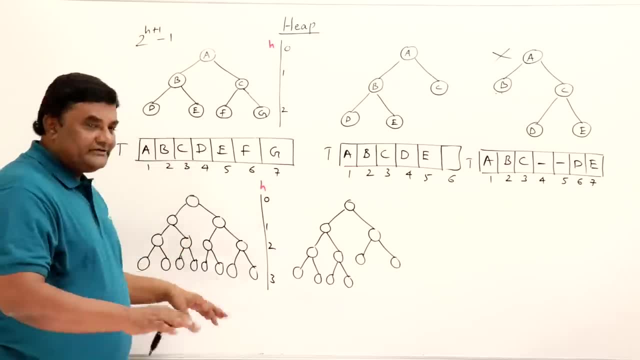 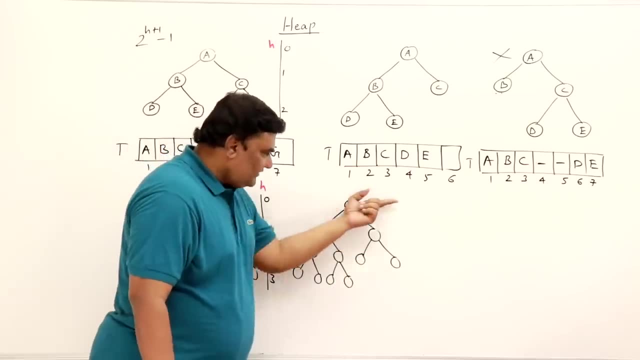 Yes, it is full as well as complete. So every full binary tree is also complete binary tree. Now check this: Is it complete or not? Check level by level. One node is there, two nodes are there. One, two, three, four nodes are there. 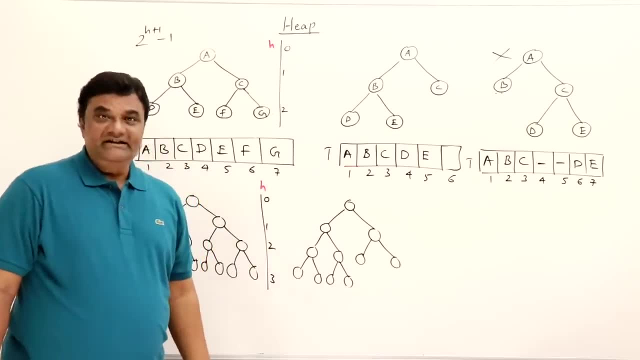 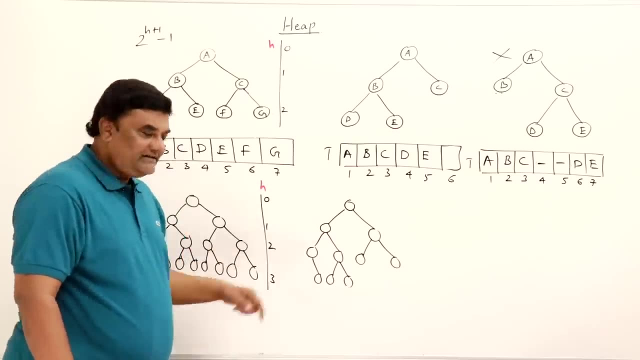 Then this next, next, next. Yes, it is complete binary tree. If I remove this node, then it's not a complete binary tree. This is missing. This is missing, So no node must be missing. If I remove this, then this is not a complete binary tree. 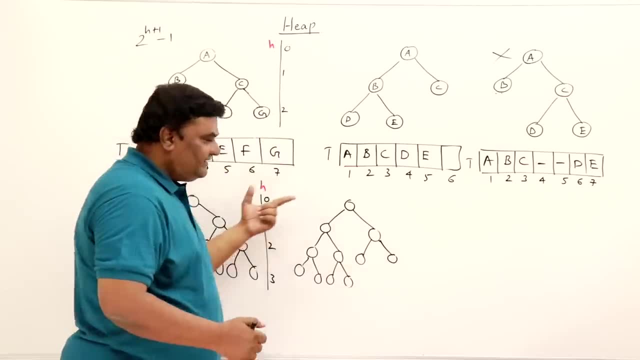 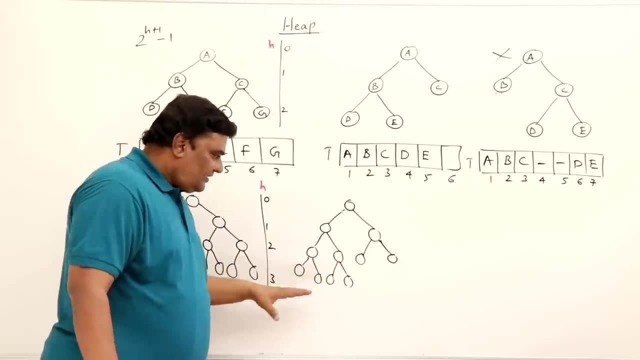 So this is missing. So if you go level by level, there should not be any missing One. then in this level, two nodes, this level, four nodes. Yes, all are there. Last level: All nodes are not there. All nodes are not there. 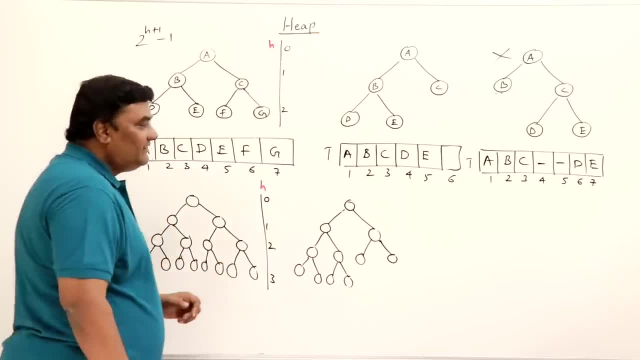 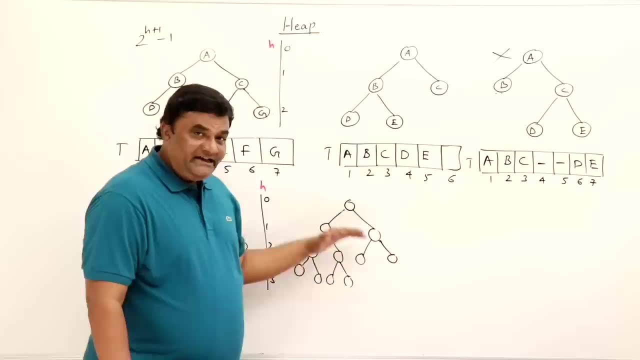 No problem, If all nodes are there, then it's a full binary tree, Right? So one more definition of complete binary tree. This mostly you find in the textbooks, See: a complete binary tree is a full binary tree up to height H minus one. 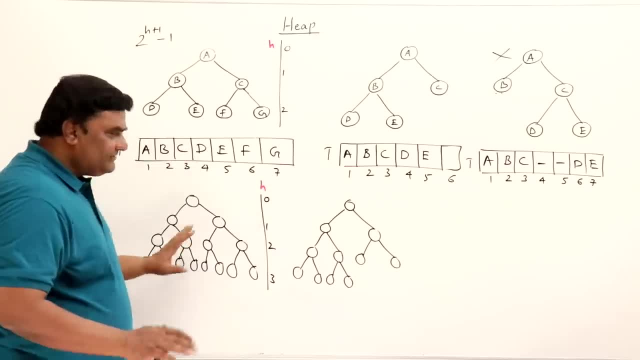 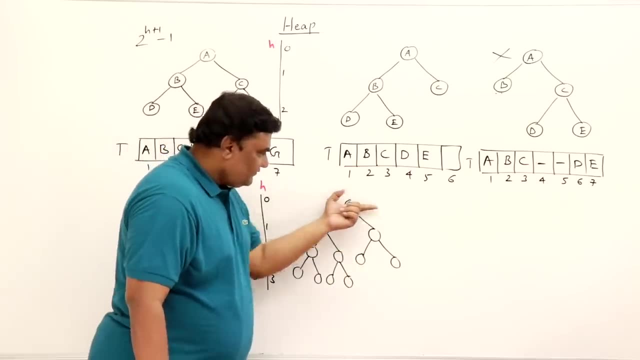 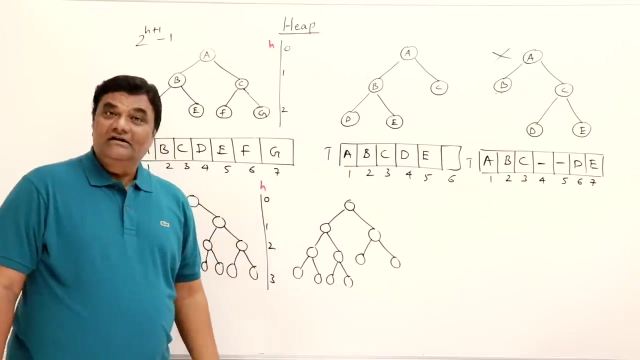 yes, it is full as well as complete. so every full binary tree is also complete binary. now check this: is it complete or not? check level by level. one node is there, two nodes? are there one, two, three, four nodes? are there then this next, next, next? yes, it is complete binary. if i remove this node, then it's not a complete binary. this is. 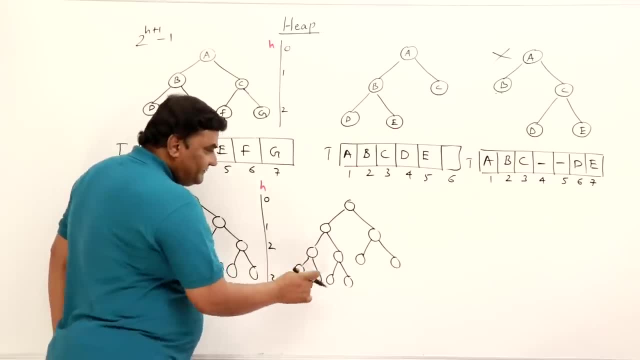 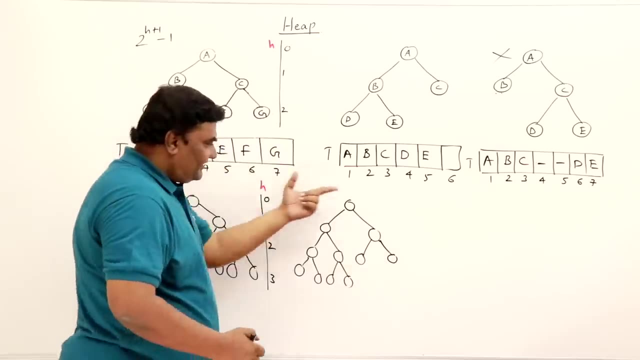 missing. this is missing, so no node must be missing. if i remove this, then this is not a complete binary. so this is missing. so if you go level by level, there should not be any missing one. then in this level, two nodes, this level, four nodes, yes, all are there. 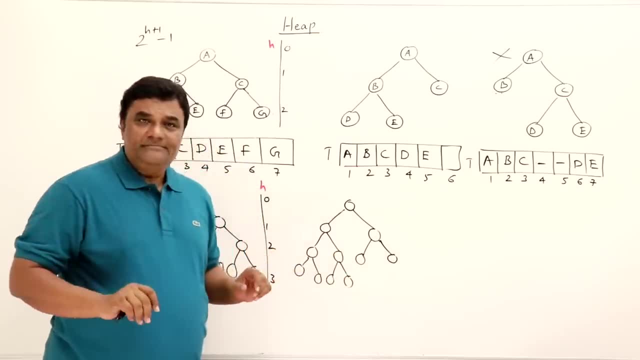 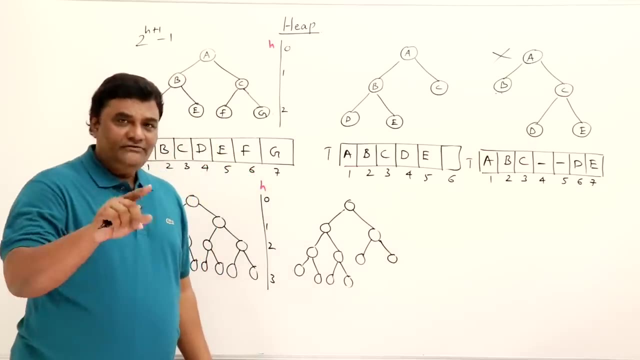 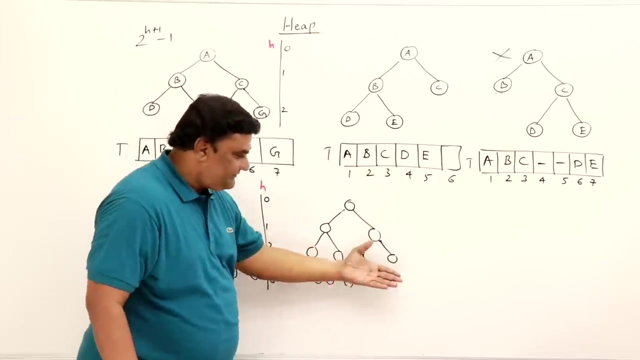 level all nodes are not there. all nodes are not there, no problem. if all nodes are there, then it's a full binary, right? so one more definition of complete binary. this mostly you find in the textbooks, see, of complete binary is a full binary up to height H minus 1. if you hide this NC, it's a full binary. and 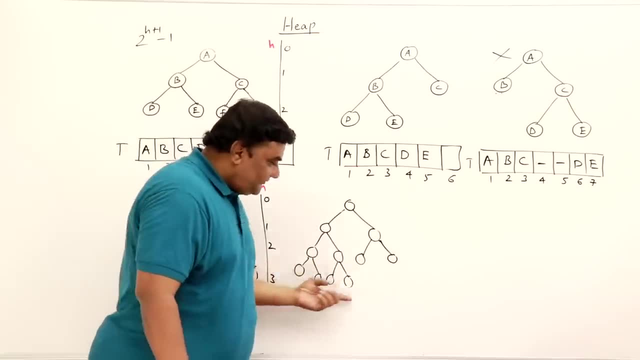 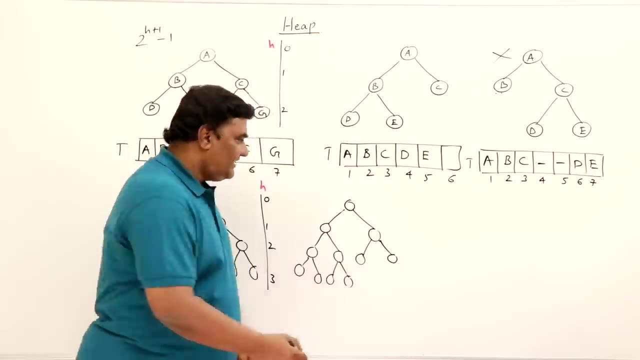 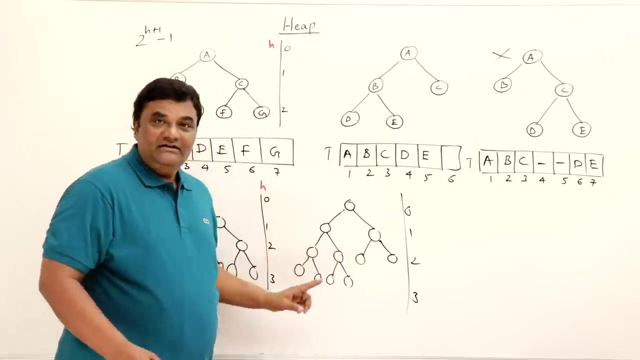 in the last level, the elements are fulfilled from left to right. this is one of the definition you will find in the textbooks: a complete binary of height H. height H is already a full binary. up to height H minus 1- last level, the elements are filled from left to right. that same thing. I am saying that if you represent 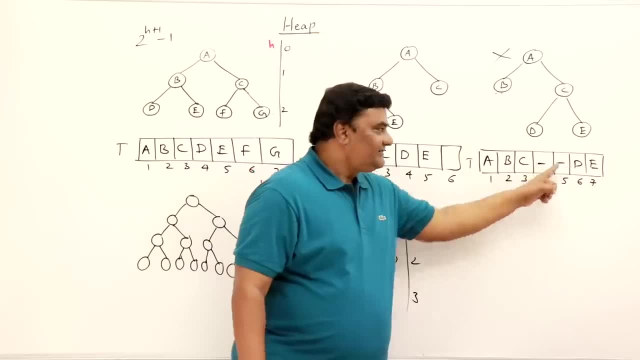 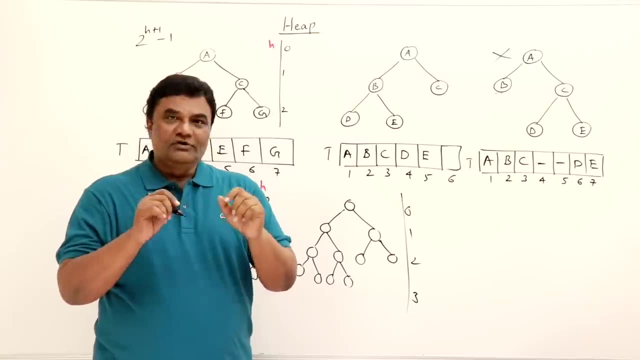 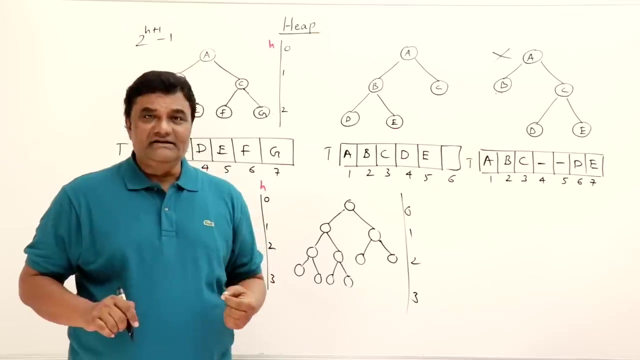 this in an array, you will not get gaps like this. if you are getting gaps, it's not a complete binary without gaps. it's a complete binary. now, one more important thing: see the definition of complete binary, what I gave you. sometimes, or some authors, some people call this as almost complete binary, also okay, but in most of 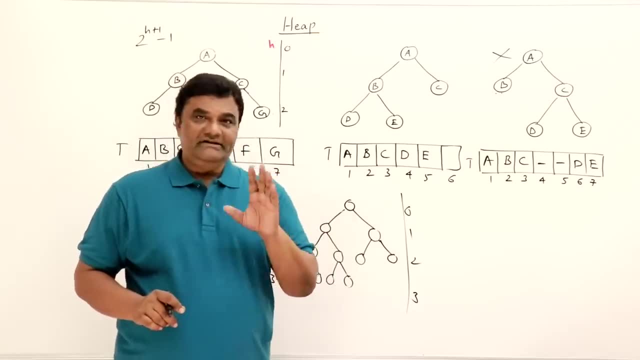 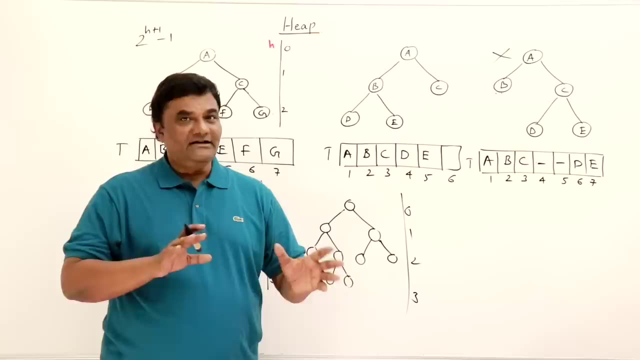 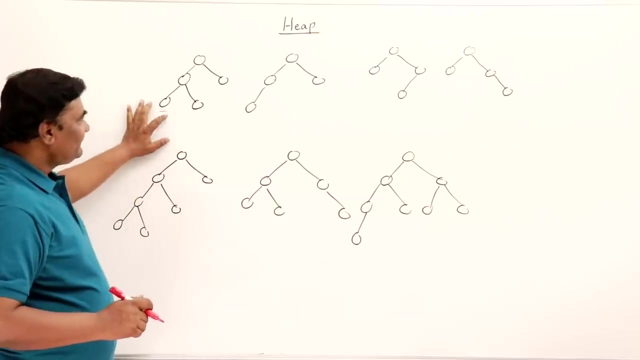 the textbooks you will find this as complete binary, so I am calling it as complete binary. now I will draw a few trees and show you which one is complete, which one is not complete, so that you get comfortable with complete binary trees. so I'll remove this and I will show few binary trees. look at this, is it? 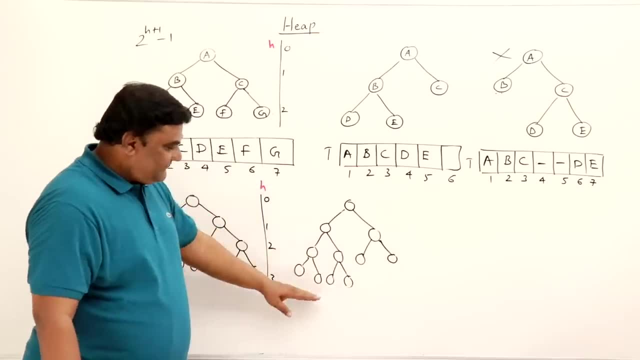 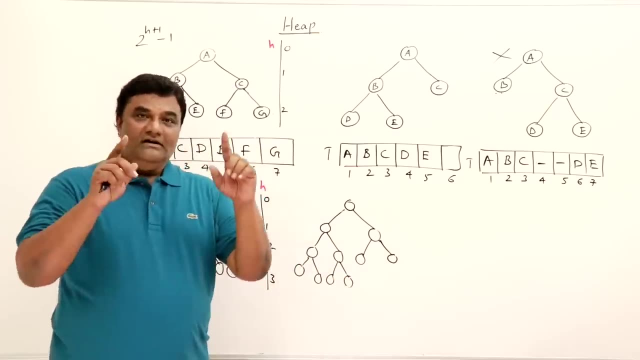 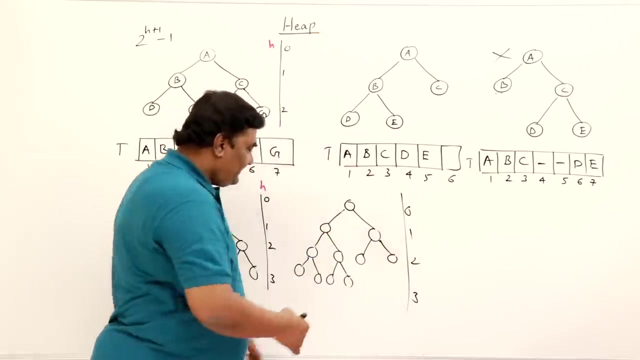 If you hide this NC, it's a full binary tree And in the last level the elements are filled from left to right. This is one of the definition you'll find in the textbooks: A complete binary tree of height H. H is already a full binary tree up to height H minus one. 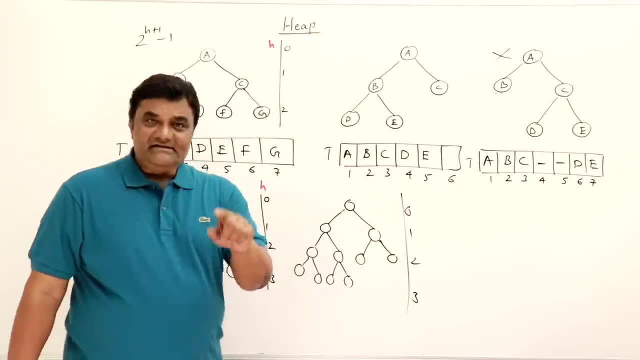 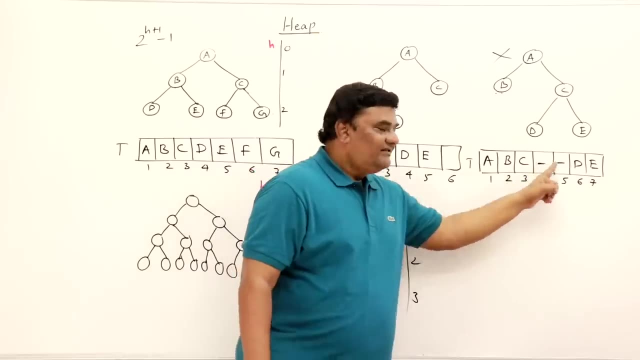 Last level, the elements are filled from left to right. That same thing. I am saying that if you represent this in an array, you will not get gaps like this. If you are getting gaps, it's not a complete binary tree Without gaps. it's a complete binary tree. 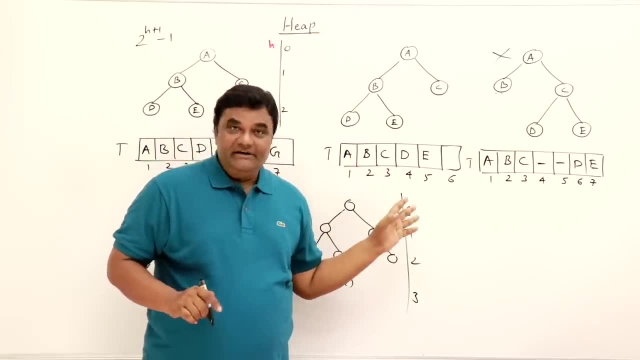 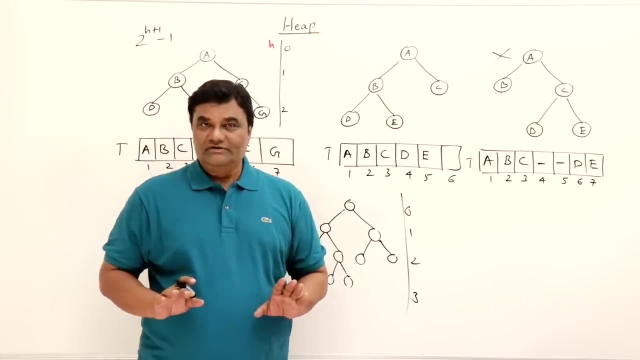 Now one more important thing: See the definition of complete binary tree, what I gave you sometimes, or some authors. some people call this as almost complete binary tree, also OK, but in most of the textbooks you will find this as complete binary tree. 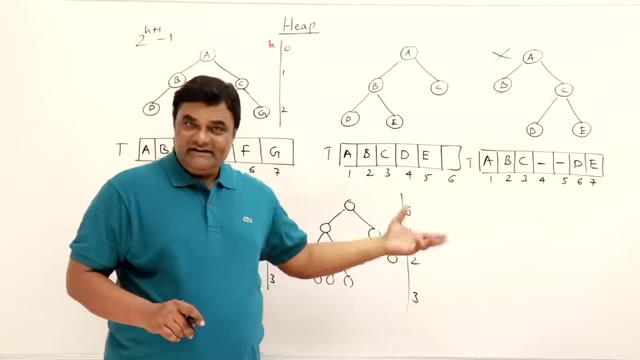 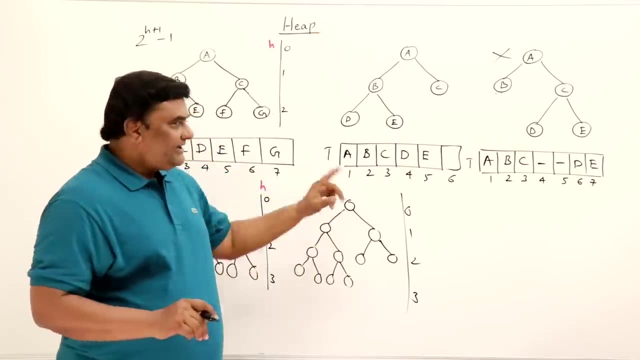 So I'm calling it as complete binary tree. Now I'll draw a few trees and show you which one is complete, which one is not complete, so that you get comfortable with complete binary trees. So I'll remove this and I will show a few binary trees. 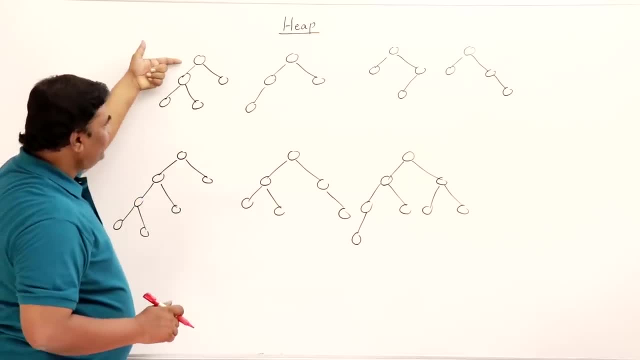 Look at this. Is it a complete binary tree Check level by level. First level, one node, then two nodes, Then four nodes. All four are not there. If you start from left side, then one, two, No node is missing. 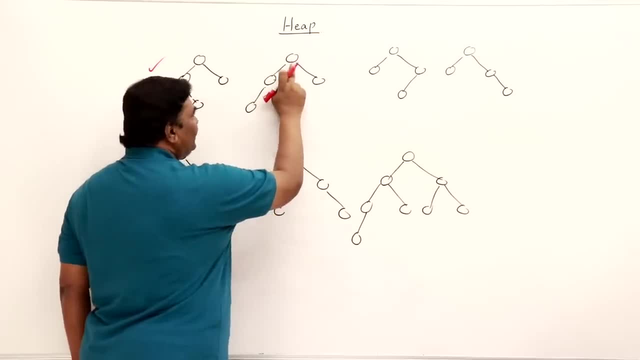 So it's a complete binary tree. Debt is one, root is one, then next level, two nodes, next level, four are there. All four are not there, but left hand side, the extreme left side, is there. So, yes, it's a complete binary tree. 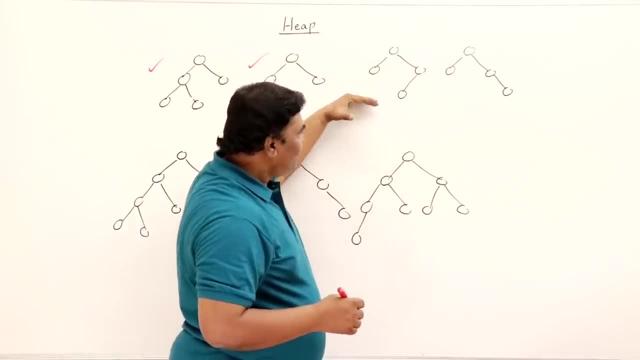 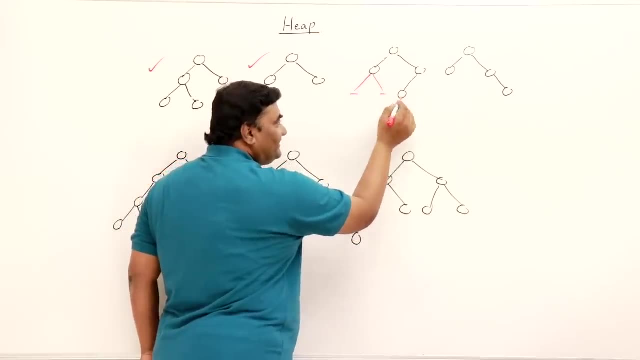 Root is one, then two, this level two, then next level. all nodes are not there, But first which node must be there? Actually it should have this node, then this node, then this is allowed. So these two are missing. 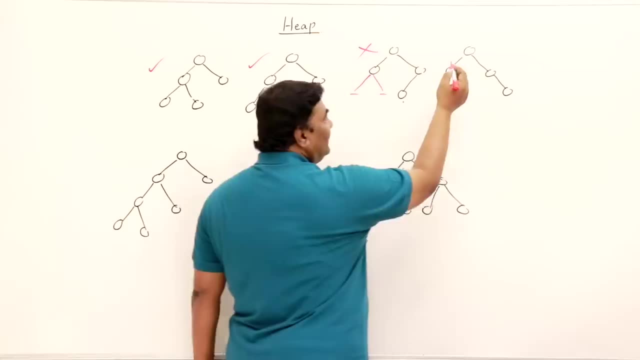 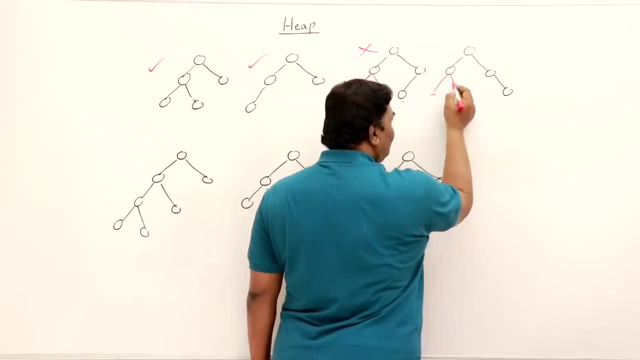 So it's not a complete binary tree. Now this one, first level one, the next two nodes, OK, next level, all nodes are not there, But first of all we should have this node, then this node, then this node, then we can have this. 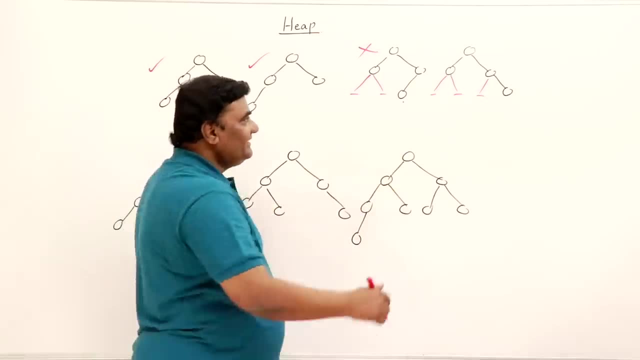 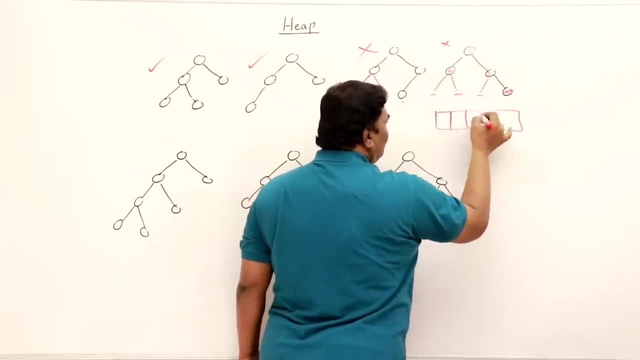 So we should have the nodes from left to right, But the three nodes are missing there. It's not a complete binary tree. So if you represent this in an array, let us say this is one, two, three and this is four. 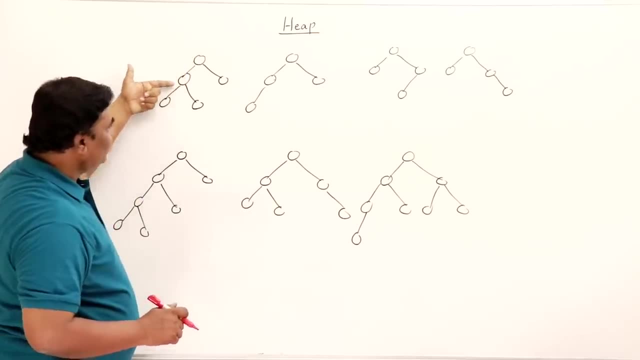 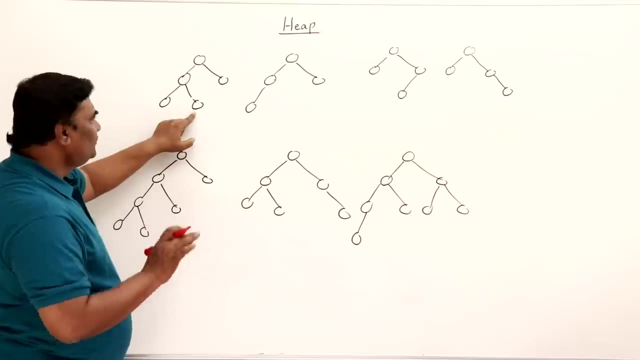 a complete binary or is it not a complete binary? or is it not a complete binary? a complete binary? check level by level. first level, one node, then two nodes, then four nodes. all four are not there. if you start from left side, then one, two. no node is missing. so it's a complete binary. get this one. root is one. the next: 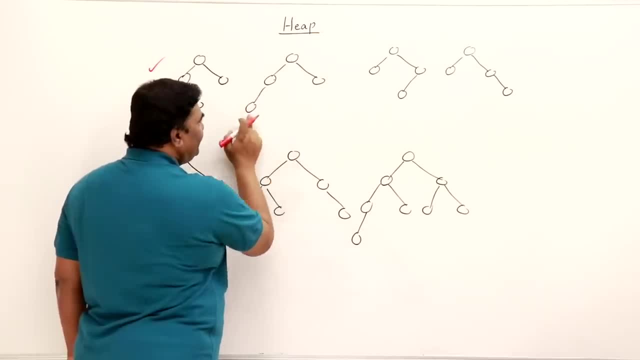 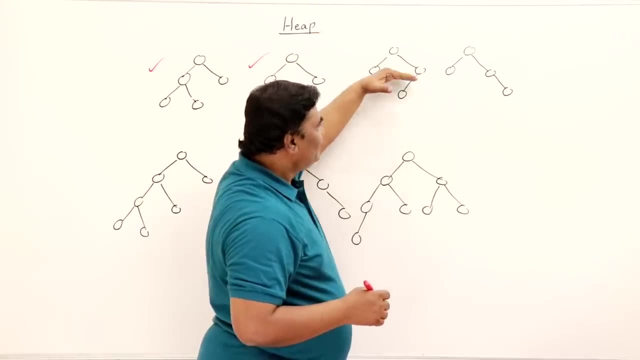 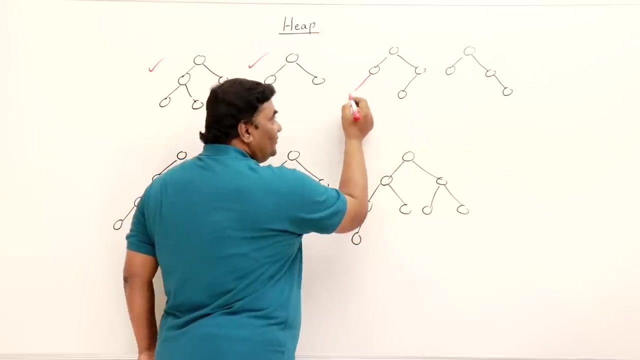 level two nodes, next level, four are there. all four are not there, but left hand side, the extreme left side, is there. so yes, it's a complete binary. root is one, then two, this level two, then next level. all nodes are not there, but first which node must be there? actually it should have this node than. 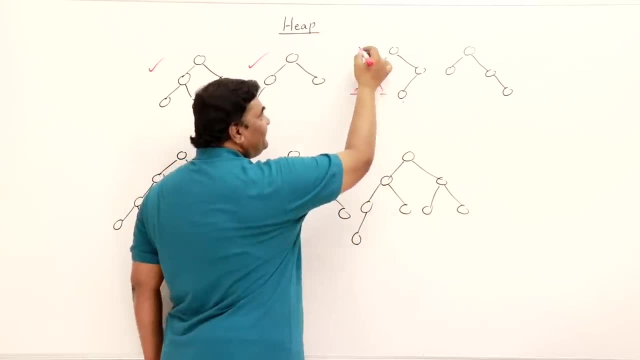 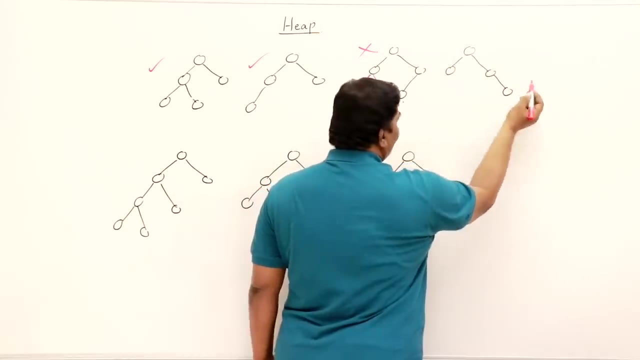 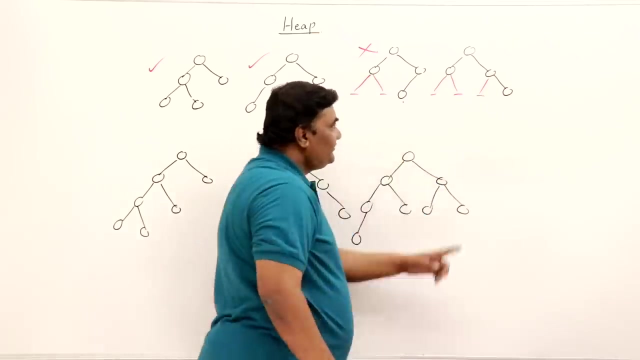 this node, then this is allowed. so these two are missing. so it's not a complete binary tree. now this one, first level one, the next two nodes, okay, next level. all nodes are not there, but first of all we should have this node, then this node, then this node, then we can have this. so we should have the nodes from left to 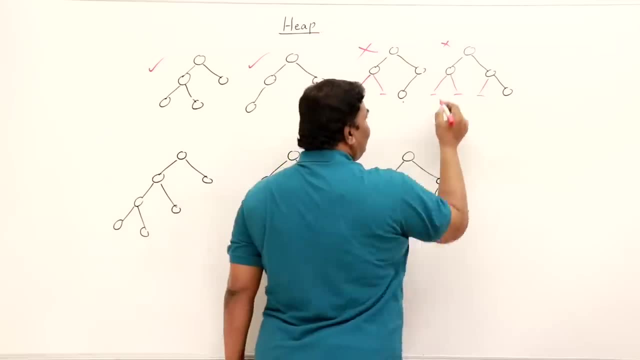 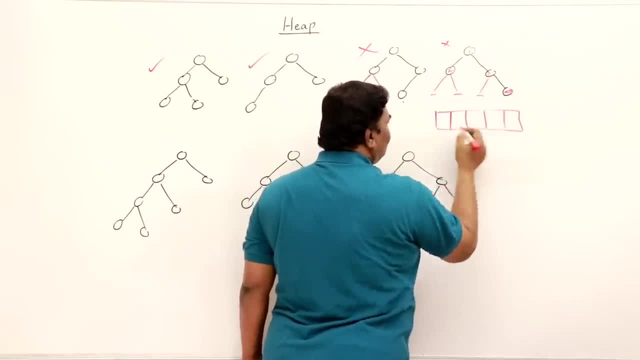 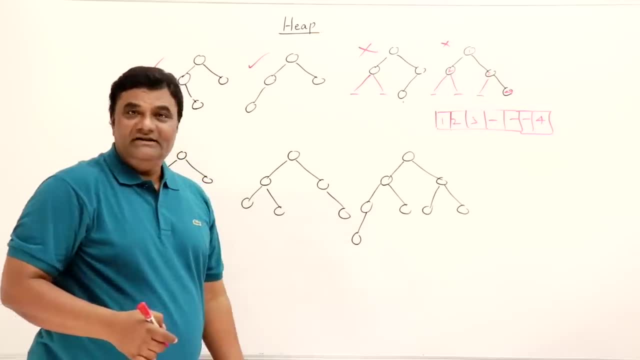 then one, two, three gap gap and a gap, and then four, so you'll get the three blank, then four, so you'll get the three blank, then four, so you'll get the three blank spaces in between the elements, so it's spaces in between the elements, so it's. 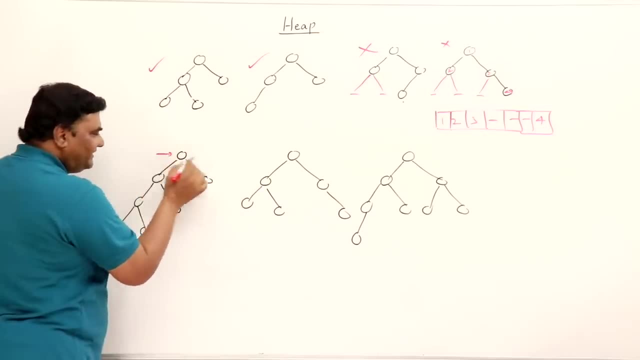 spaces in between the elements. so it's not a complete binary. what about this? not a complete binary? what about this? not a complete binary? what about this? let us check first level, one next level. let us check first level, one. next level: two nodes. next level: four nodes must be there: one, two, three, four. these are missing, so it's not a 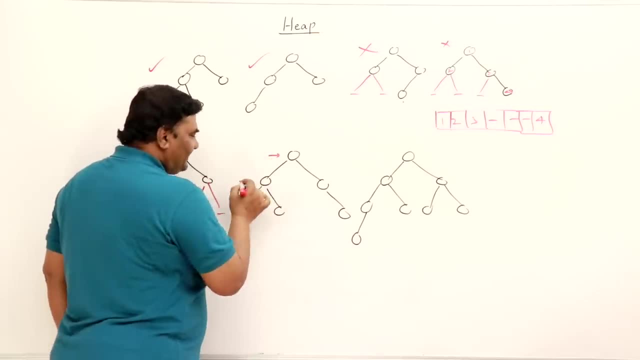 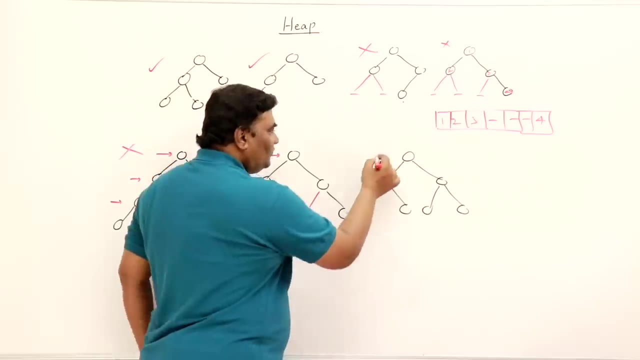 complete binary. what about this? this is there, right, two nodes, then four must be there one, two. this is missing, so it's not a complete binary. this one one, then here two nodes, then here one, two, three, four nodes. okay, then last level: all nodes are not there, but we have this extreme left. yes, this is. 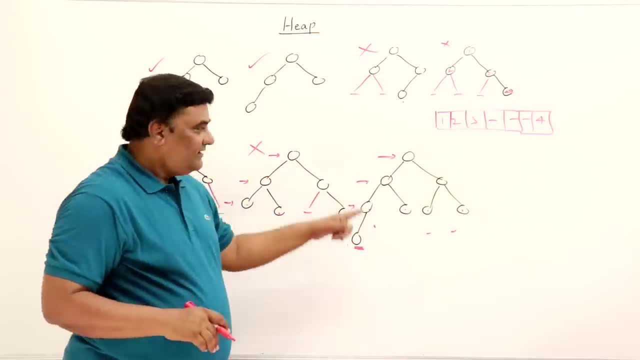 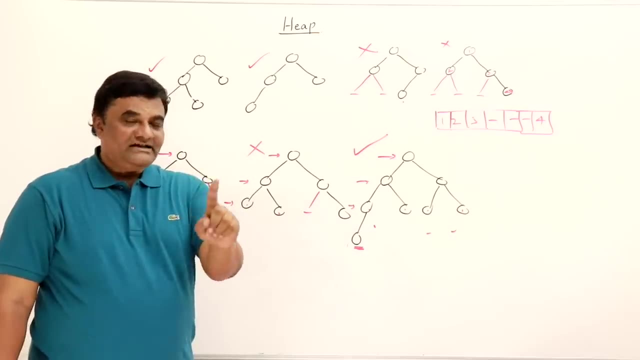 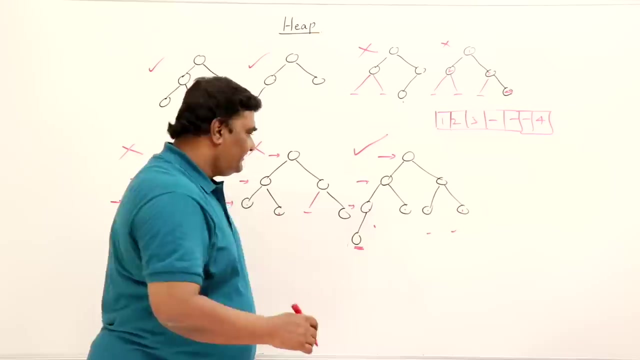 the end point after these nodes are not there, that is not a problem. this is a complete binary. now you are comfortable with what is complete binary. and one last point of a complete binary is that the height of a complete binary will be minimum. only that is log n height of a complete. 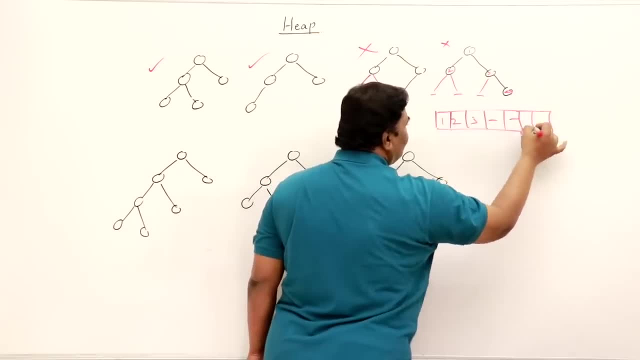 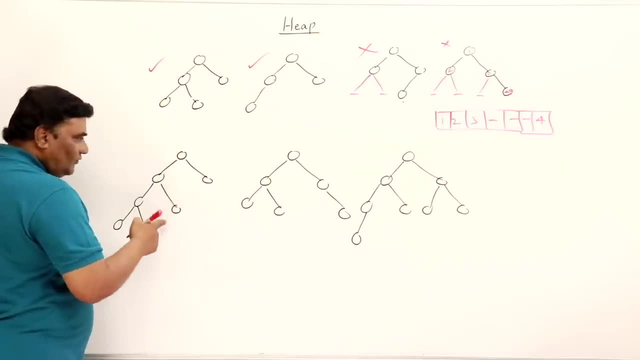 Then one, two, three, Gap gap and a gap and then four. So you'll get three blank spaces in between the elements. So it's not a complete binary tree. What about this? Let us check First level one. next level: two nodes. next level: four nodes must be there. 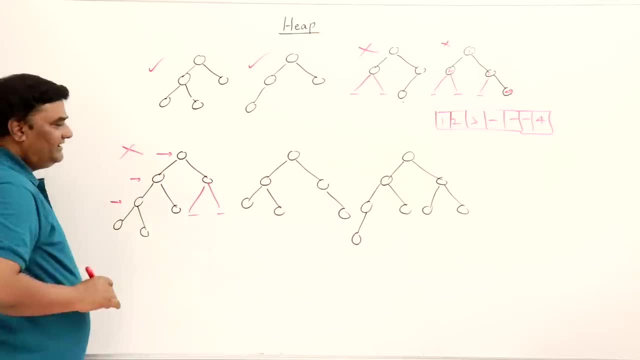 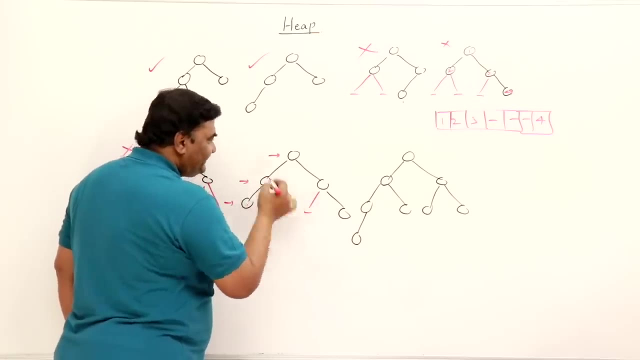 One, two, three, four. These are missing, So it's not a complete binary tree. What about this? This is there, right? Two nodes, then four must be there. One, two, this is missing, So it's not a complete binary tree. 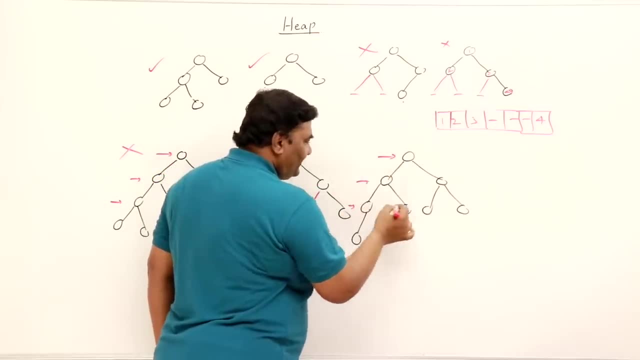 This one, one, then here two nodes, Then here one, two, three, four nodes. OK, then last level: all nodes are not there, But we have this extreme left. Yes, this is the end point after this. nodes are not there. 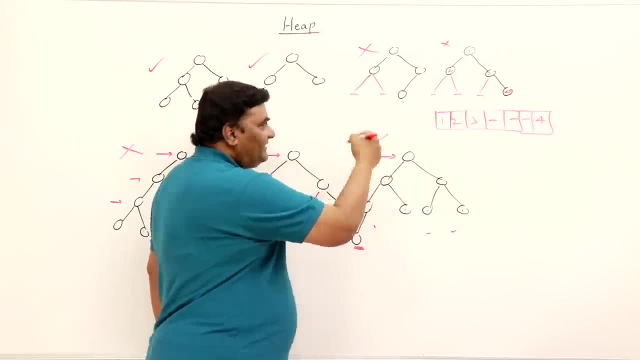 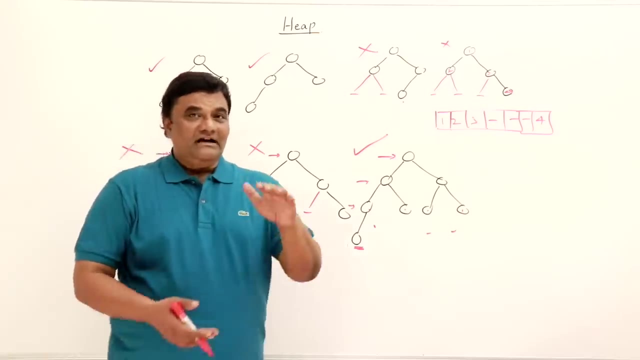 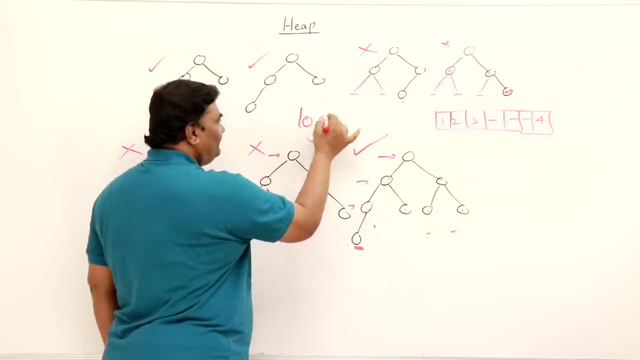 That is not a problem. This is a complete binary tree. Now you are comfortable with what is complete binary tree. And one last point of a complete binary tree is that the height of a complete binary tree will be minimum. only that is log n. Height of a complete binary tree will always be log n. 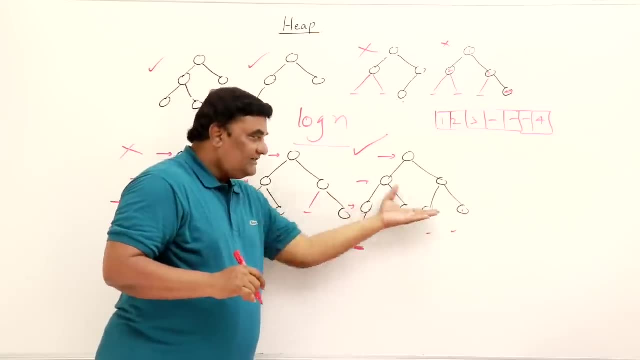 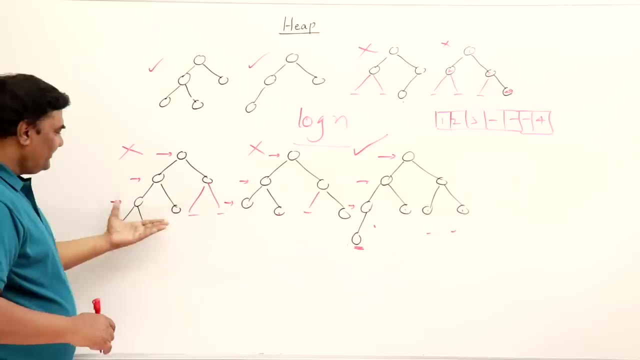 So unnecessary. we are not going to the next level unless one of the level is filled. Unless this is filled, we will not go to the next level. See, unless this is filled, we will not go to this level. It's not a complete binary tree. if you are going to the next level, 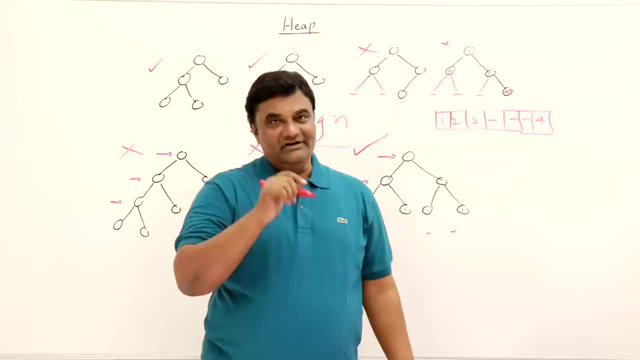 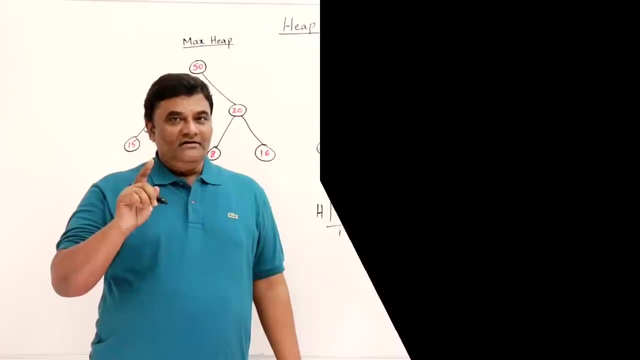 So always, the height of a complete binary tree will be minimum. That is log n. This is the interesting fact of a complete binary tree Now. next we will learn about heap. Let us learn heap. See for that. I have example binary trees here. 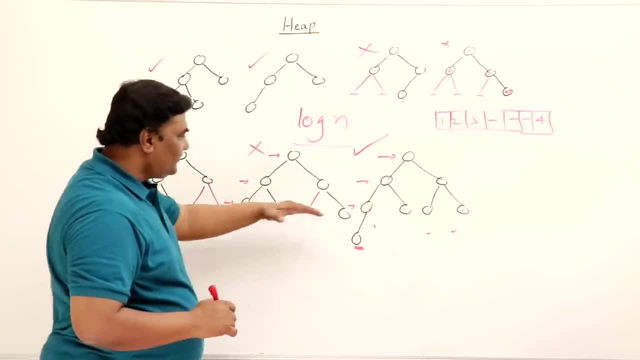 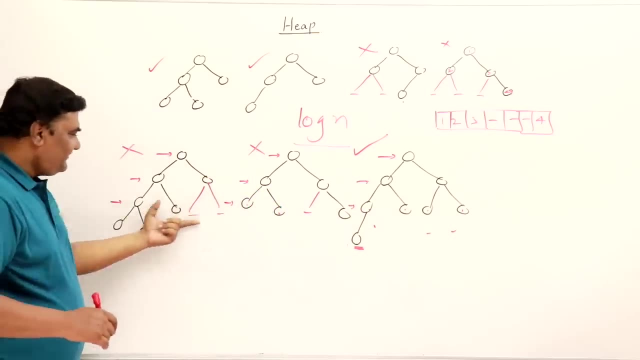 binary will always be log n because, unnecessarily, we are not going to the next level unless one of the level is filled. unless this is filled, we will not go to next level. see our. unless this is filled, we will not go to this level. it's not a complete binary. if you are going to 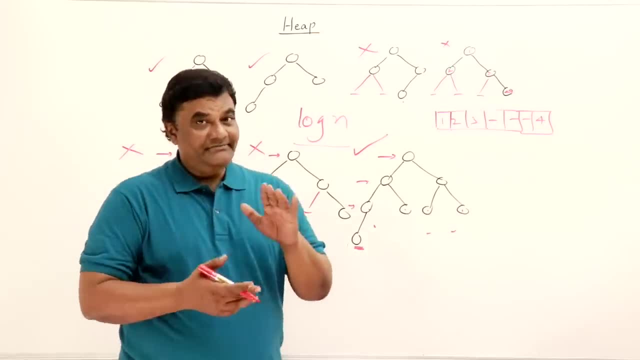 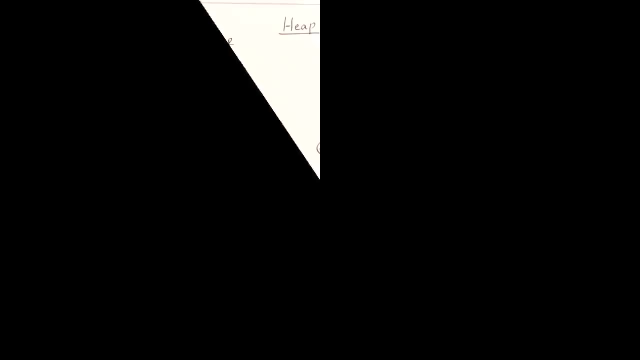 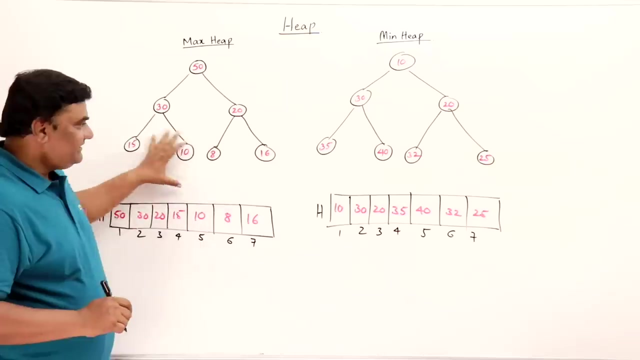 next level. so always the height of a complete binary will be minimum, that is, log n. this is the interesting fact of a complete binary now. next we will learn about heap. let us learn heap. see for that. i have example binary trees here. this binary tree is a full as well as it's a 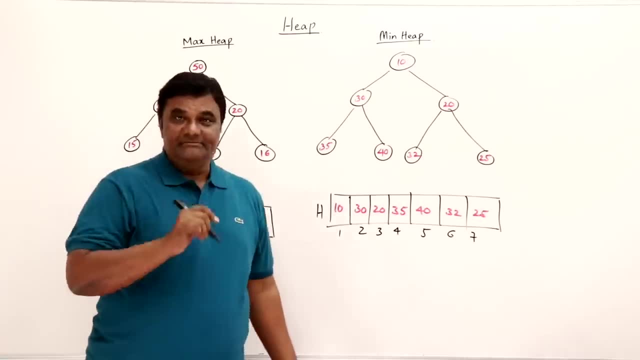 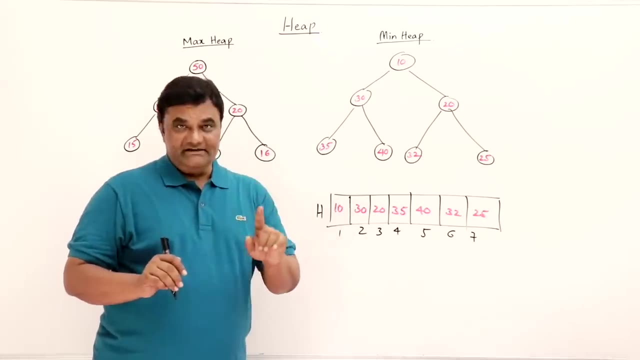 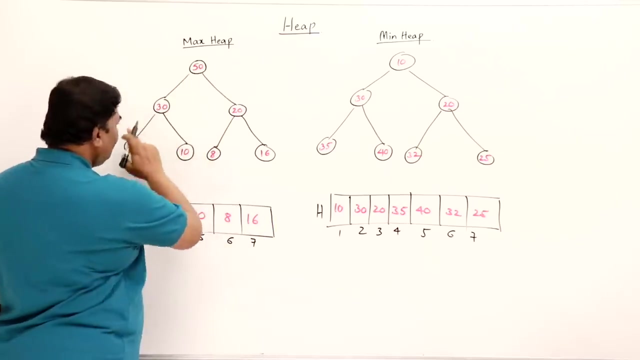 complete binary tree. yes, the important thing is: complete binary. this is also a complete binary. this is also complete. now, first of all, heap is a complete binary tree. then next condition: see the condition. let us look at the elements: 50. then 30 and 20 are smaller than 50. yes, 15 and 10 are. 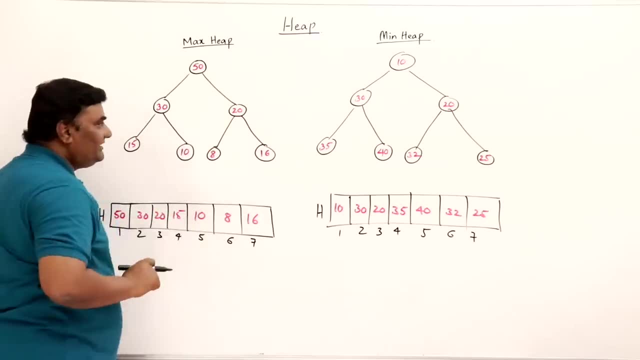 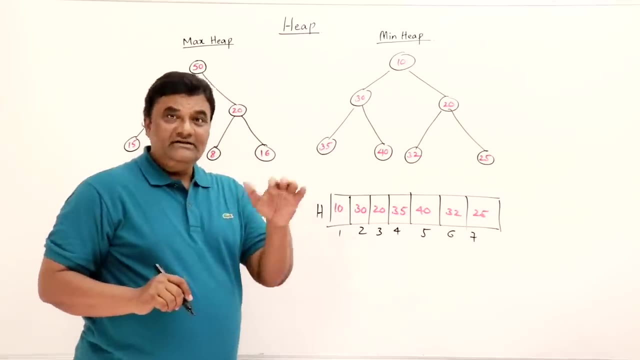 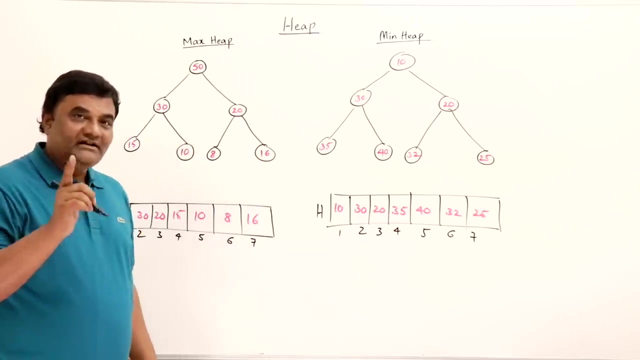 smaller than 30, and 8 and 16 are smaller than 20. so it means every parent is having the value greater than all its descendants. every node is having the value greater than all its descendants, so root will have the largest value. that is maximum value. so yes, if the elements are arranged, 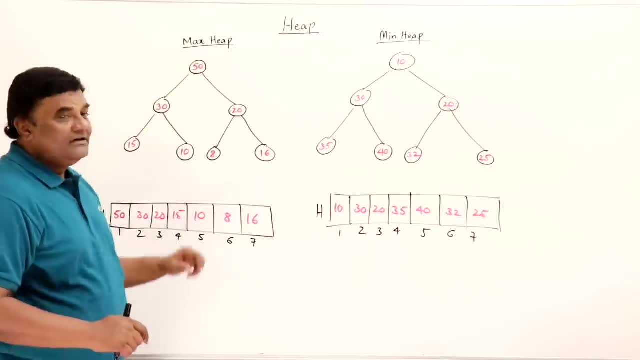 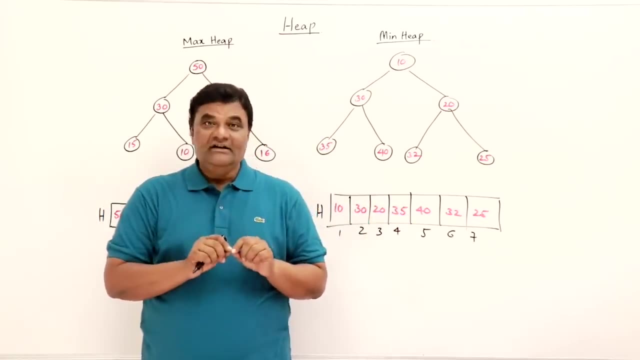 like this, then it is called as max heap. so i repeat: max heap is a complete binary satisfying the condition that every node is having the element greater than all its descendants, greater than or equal to also all its descendants. so duplicates are allowed here. so if you have 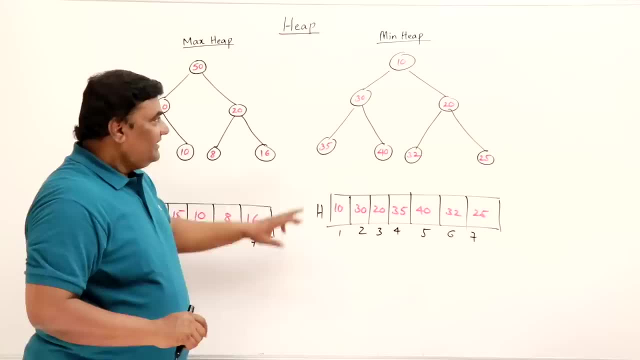 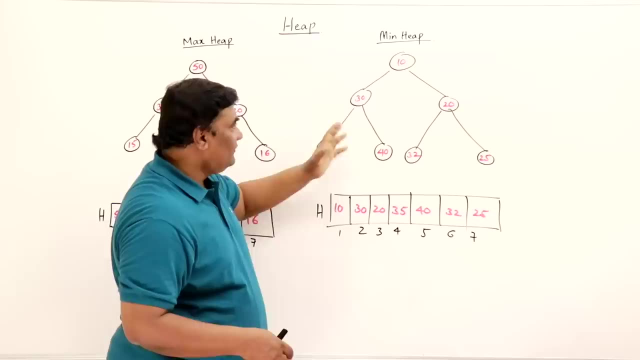 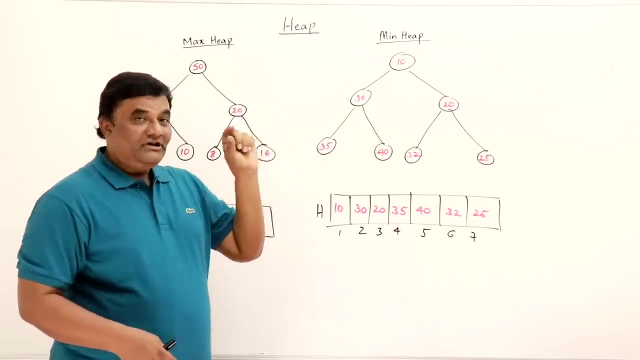 duplicates. you can have them in descendants. coming to this one here, this is 10, 30 and 30 are the children that are greater, and this 35 and 40 are greater than 30 and also 10. so 32 and 25 are greater than 20 and also, in turn, they are greater than be 10 also. so here the smallest. 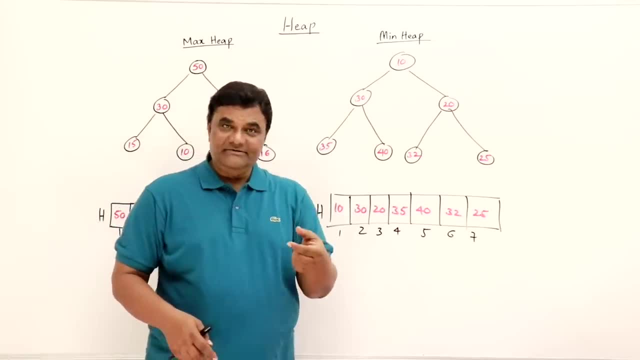 the element is there in the root. so every node is having the element smaller than all its descendants are smaller than or equal to all its descendants base nine. so this is called as min heap. so i can, i repeat: min heap is a complete binary, satisfying the condition as well. 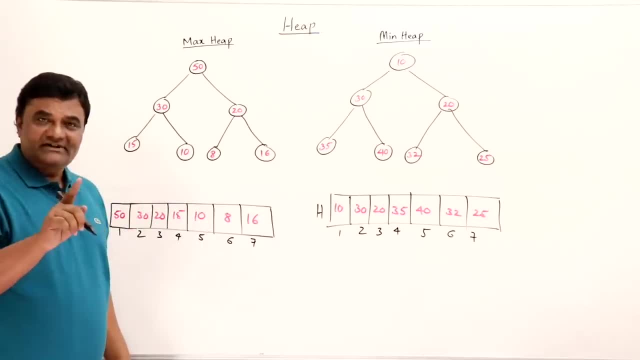 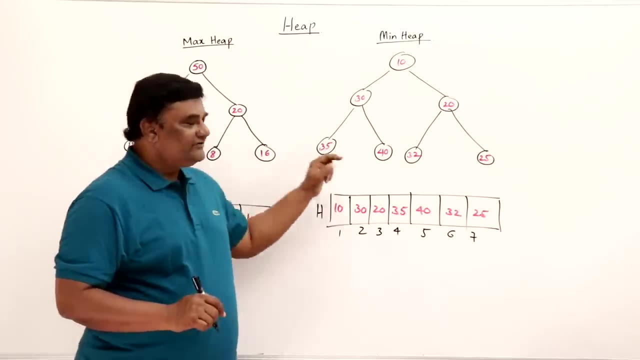 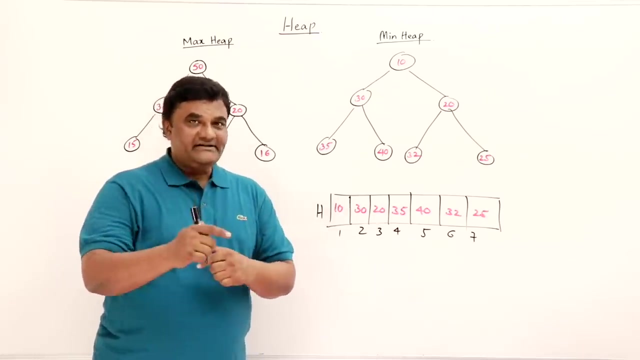 This binary tree is a full as well as it's a complete binary tree. Yes, the important thing is: complete binary. This is also complete. This also complete Now, first of all, heap is a complete binary tree. Then, next condition: 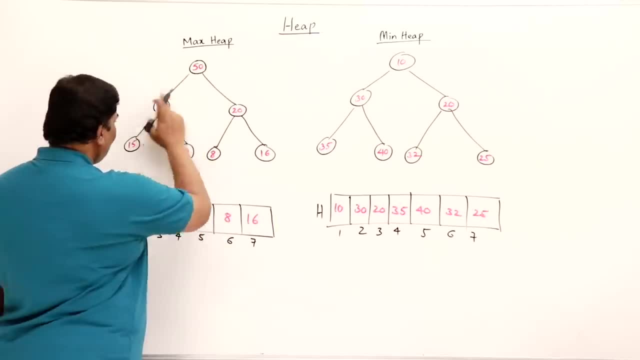 See the condition. Let us look at the elements 50,, then 30 and 20 are smaller than 50. Yes, 15 and 10 are smaller than 30, and 8 and 16 are smaller than 20.. So it means 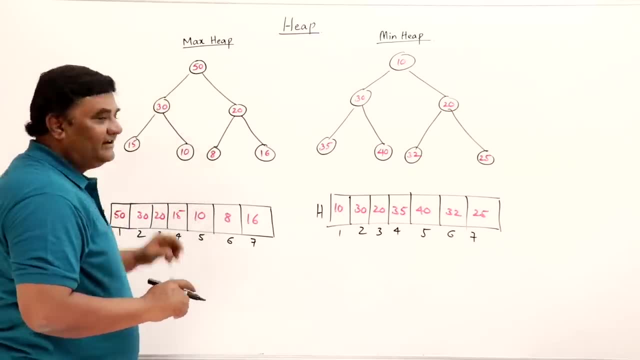 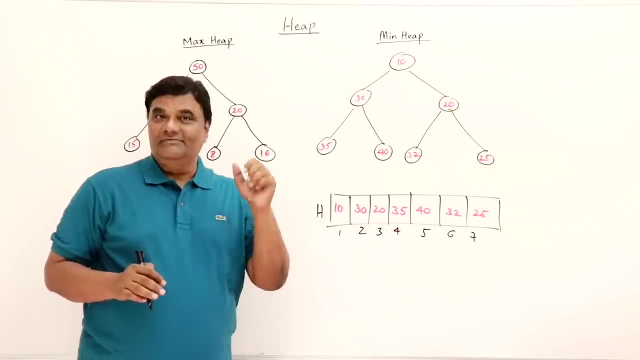 every parent is having the value greater than all its descendants. Every node is having the value greater than all its descendants, So root will have the largest value. that is maximum value. So yes, if the elements are arranged like this, then it is called as max heap. 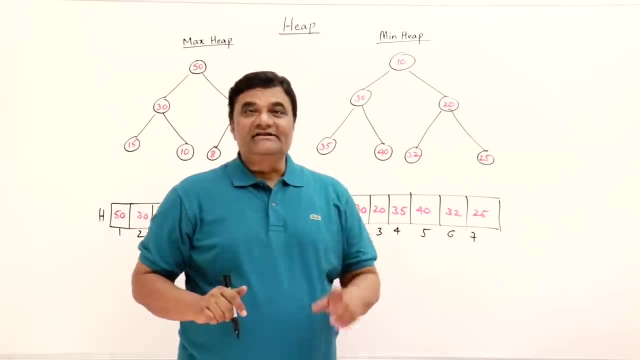 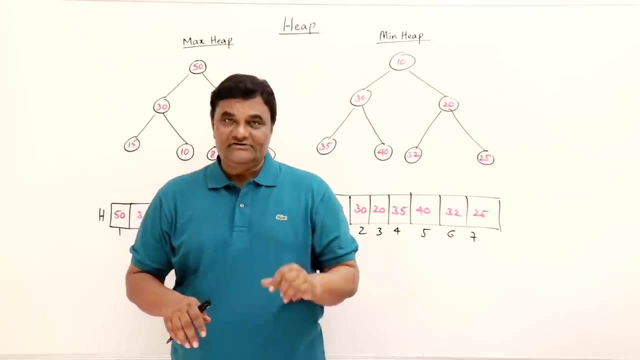 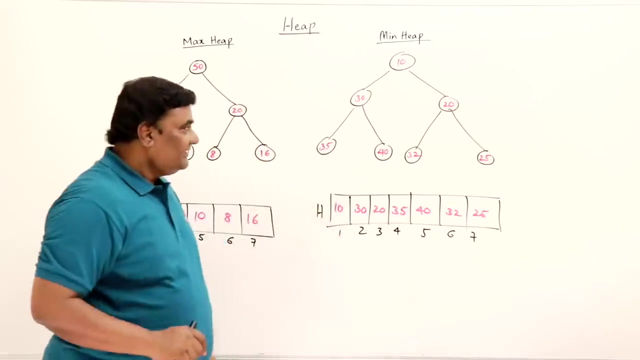 So I repeat, max heap is a complete binary tree, satisfying the condition that every node is having the element greater than all its descendants, greater than or equal to also all its descendants. So if you have duplicates you can have them in descendants. Coming to this one here, this is 10, 30 and 20 are the children that are greater. 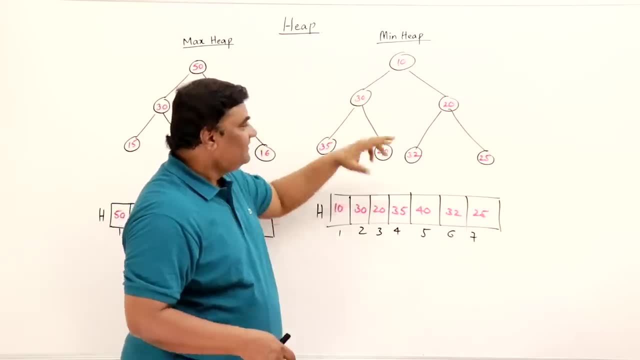 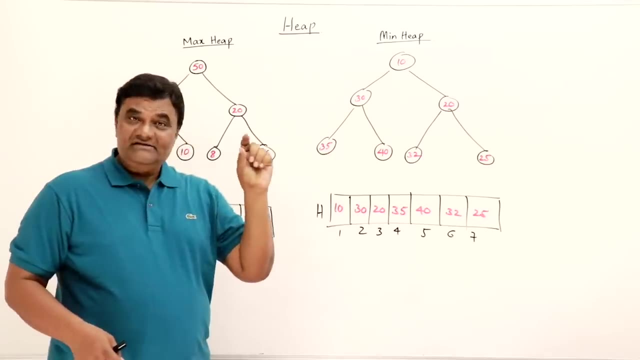 And this 35 and 40 are greater than 30 and also 10.. So 32 and 25 are greater than 20.. And also in turn they are greater than 10 also. So here the smallest element is there in the root. 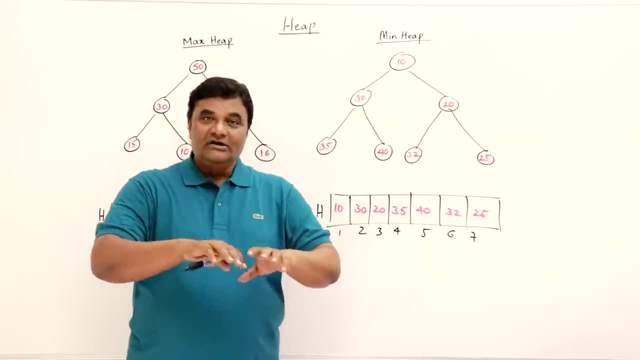 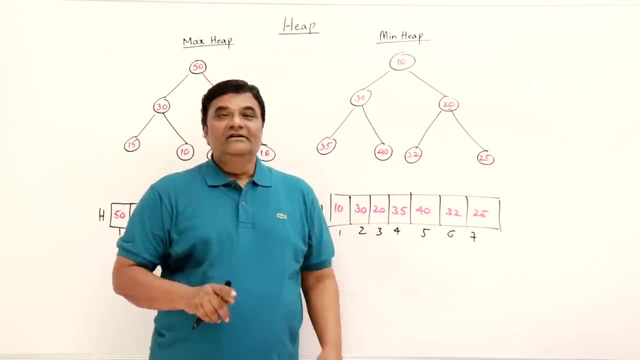 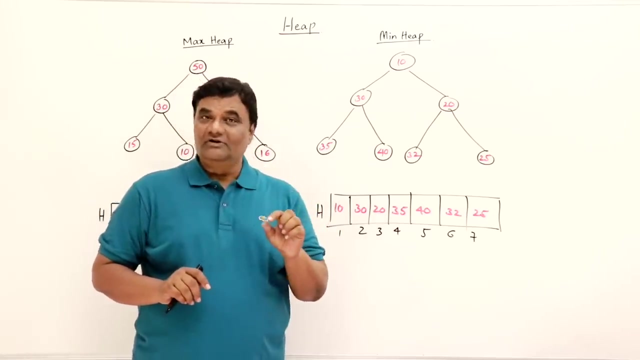 So every node is having the element smaller than all its descendants, or smaller than or equal to all its descendants. So this is called as mini heap. So again, I repeat, mini heap is a complete binary tree satisfying the condition that every node is having the element smaller than or equal to all its descendants. 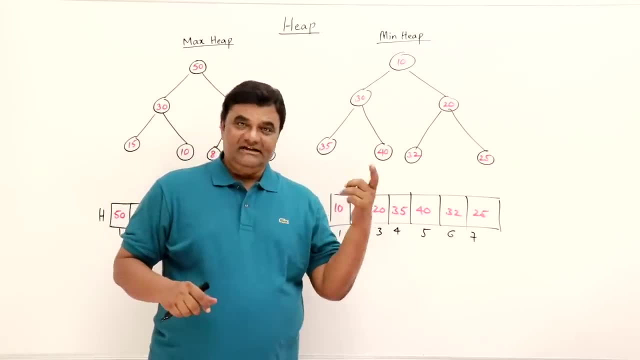 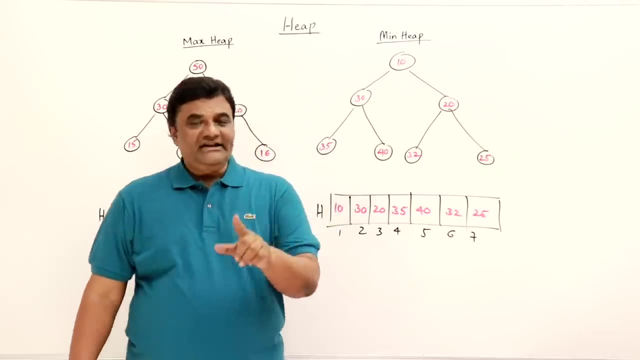 So there are two types of heap: max heap and mini heap. So whatever we have to study, we'll study upon one heap, and same thing applies on the next heap also. So we will take max heap and study this one. So we will learn how to insert and delete the elements. 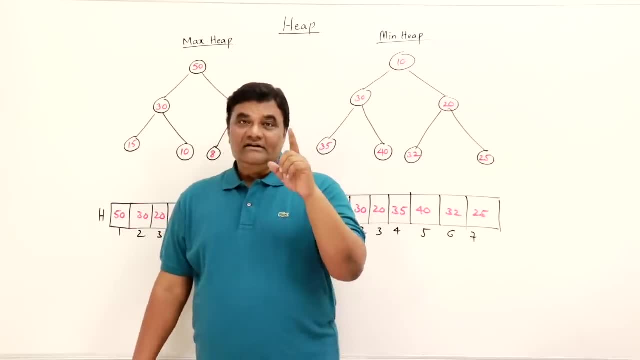 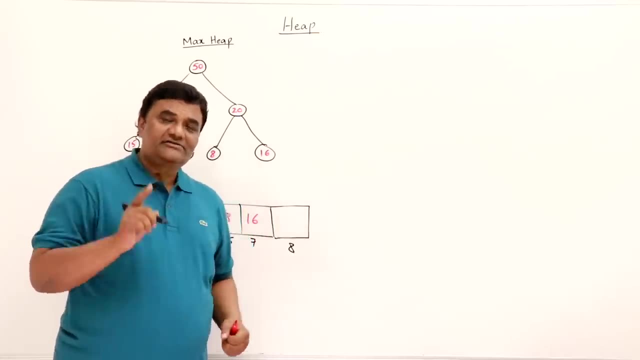 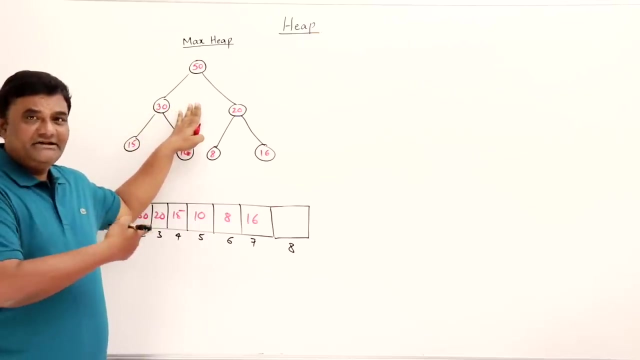 So first let us look at Insert operation in a max heap. I'll show you insert operation in max heap. Let us understand how insertion is done. So already I have a max heap here. This is a diagrammatic representation of a heap that is complete binary. 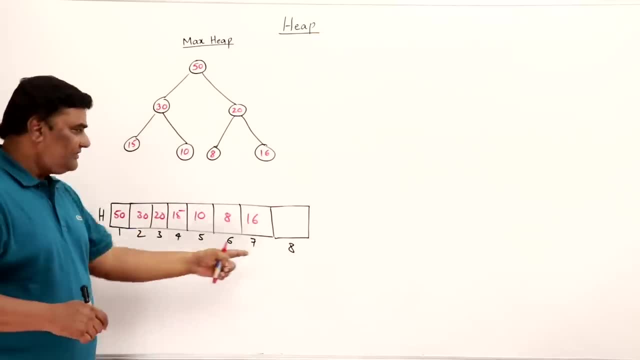 And that is. this is the array representation of same thing. This is stored in an array. If you check root 50, then this is 30, 20, 30, 20, 15, 10, 8, 16, 15, 10, 8, 16.. 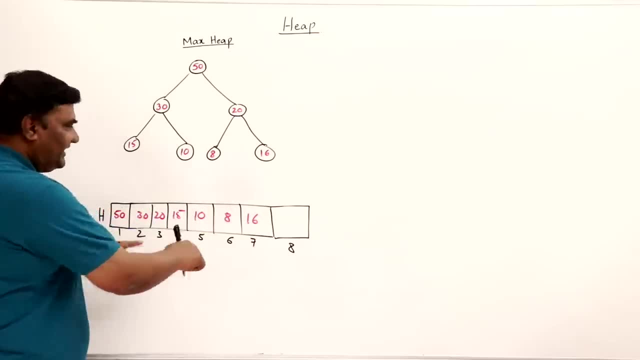 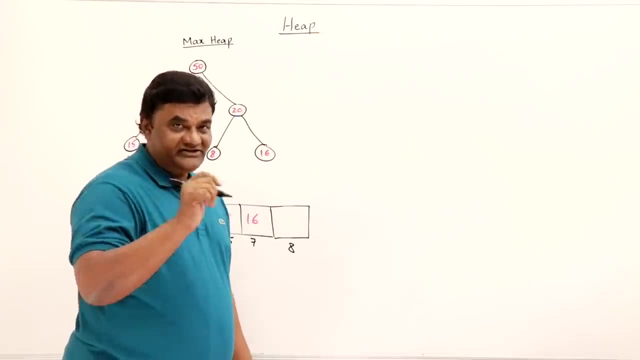 There are no gaps in between the elements, in between these two, There are no gaps. So it's a complete matrix. It's perfect. Let us insert- I want to insert an element 60. So let us insert 60. So I want to insert the 60 in this max heap. 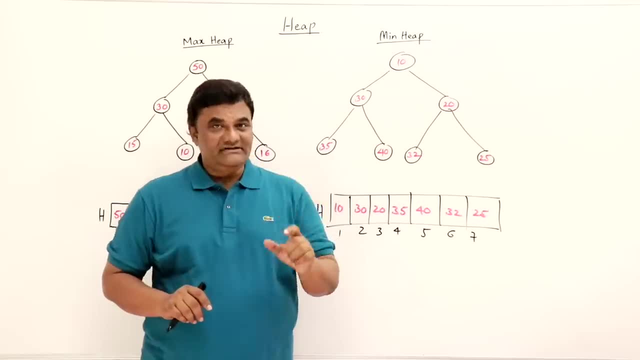 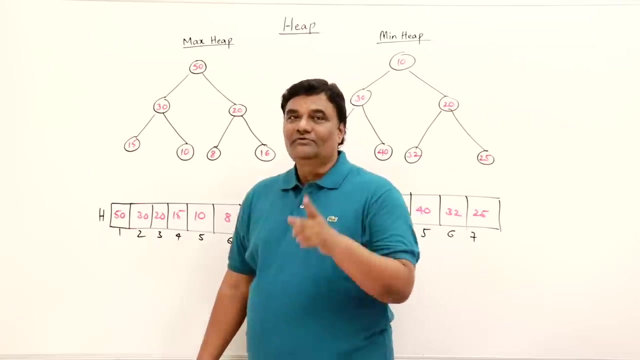 that every node is having the element smaller than or equal to all its descendants. so there are two types of heap: max heap and min heap. so whatever we have to study, we'll study upon one heap, and same thing applies on the next heap also. so we will take max heap and study this one. so 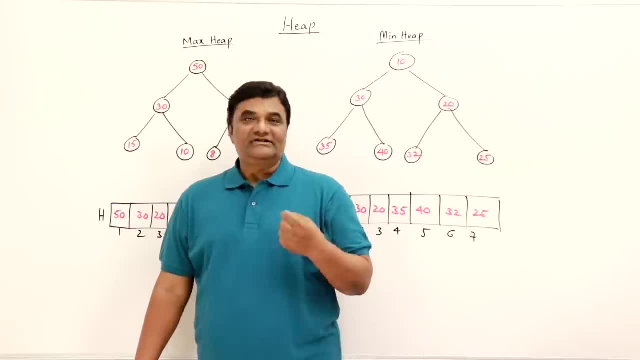 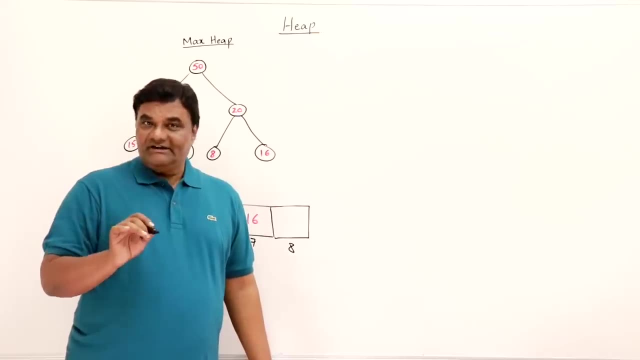 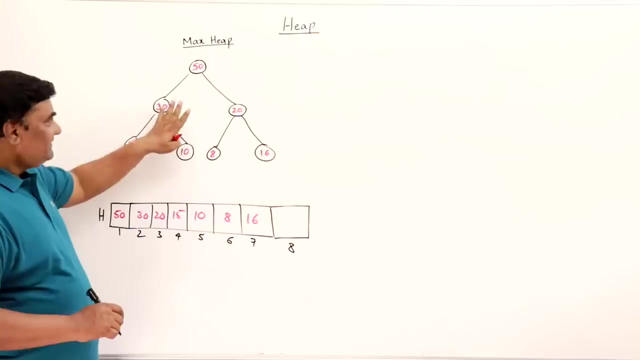 we will learn how to insert and delete the element. so first let us look at insert operation in a max heap. i'll show you insert operation in max heap. let us understand how insertion is done. so already i have a max heap here. this is a diagrammatic representation of a heap that is: 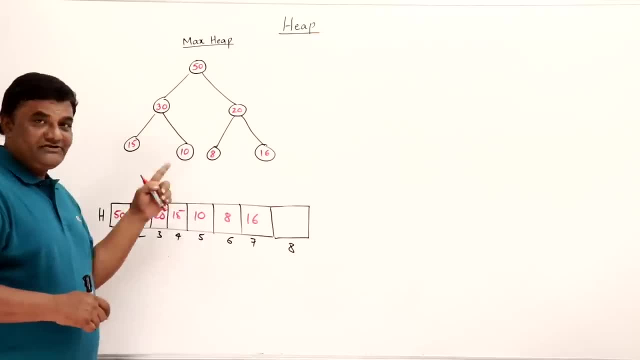 completely, and that is. this is the array representation of same thing. this is stored. if you check root 50, then this is 30, 20, 30, 20, 15, 10, 8, 16, 15, 10, 8, 16. there are no gaps in between. 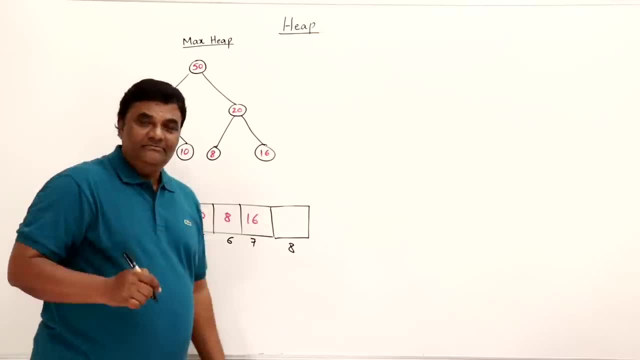 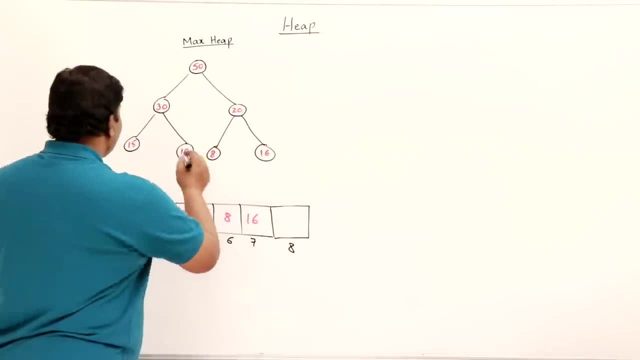 the elements a, a. between these two there are no gaps, so it's a complete magnet. it's perfect, let us insert. i want to insert a element 60, so let us insert 60. so i want to insert the 60 in this max heap, so let us. 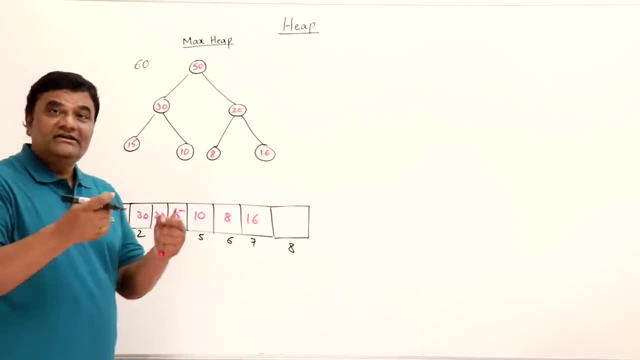 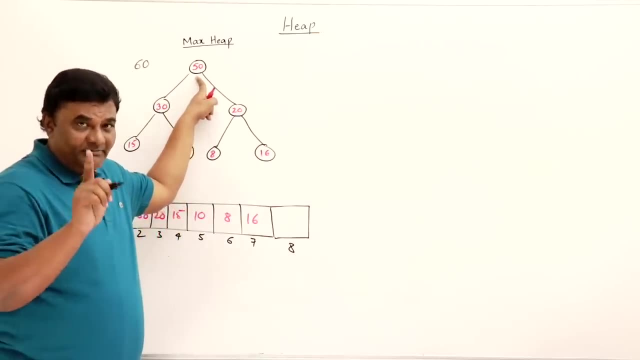 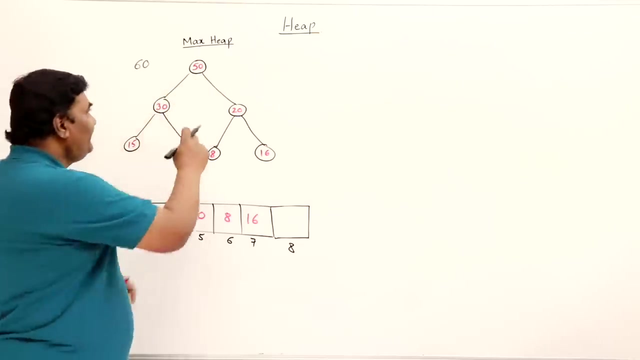 see. see where the 60 should come. root should have the largest element, so 60 should come in root. yes, now what usually people think. i will talk about that. then i will show you what is the right method. people think that 60 should be inserted here. then where 50 should go, 50 should go. okay, this is 30. 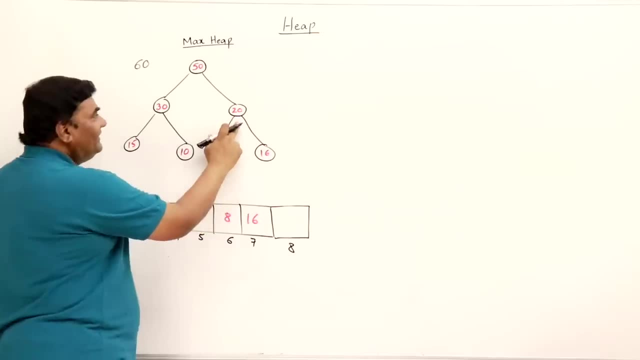 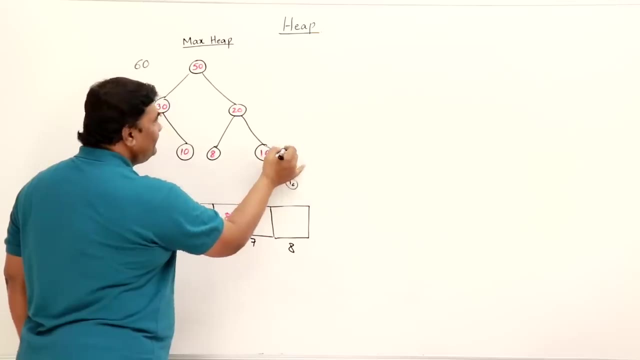 that is 20, so this is small enough. 50 should go this side. okay, then, where this 20 should go, 20 should come this side. so, in this way, it will extend in this direction: 16 will come here, and this will become 20, and this will become 50 and this will become 60. now, if we do it like this, 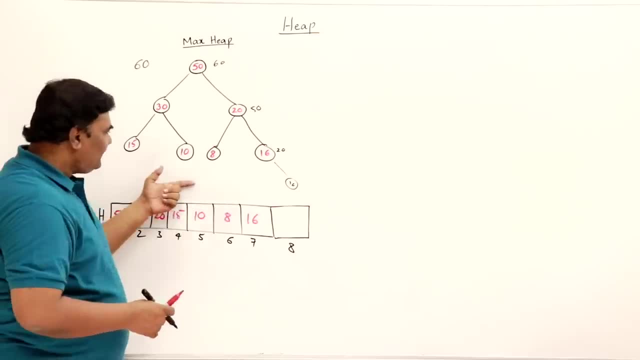 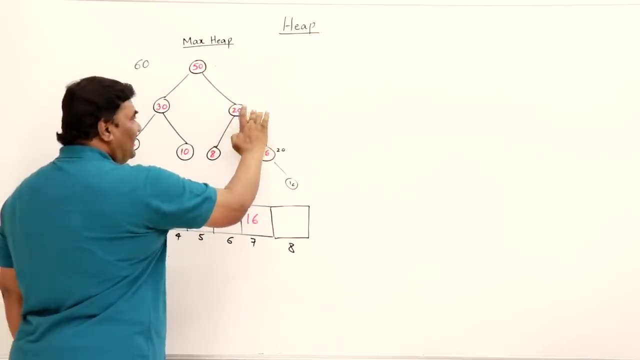 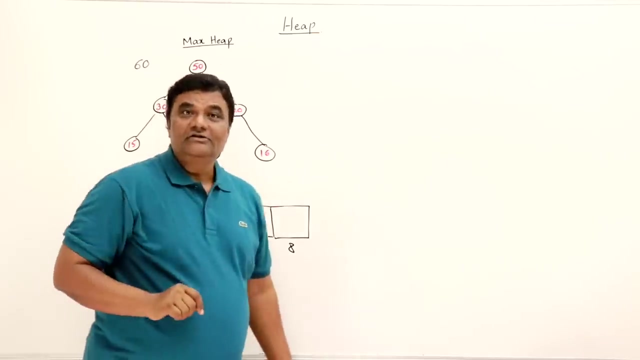 is it a complete binary tree? no, all these are missing element. then we have the 16 here. this is wrong, so don't insert it in the root. so i have shown you the wrong procedure or wrong assumption what people will have. this is wrong. it is not inserted in the root. then how it is inserted, where it is inserted: 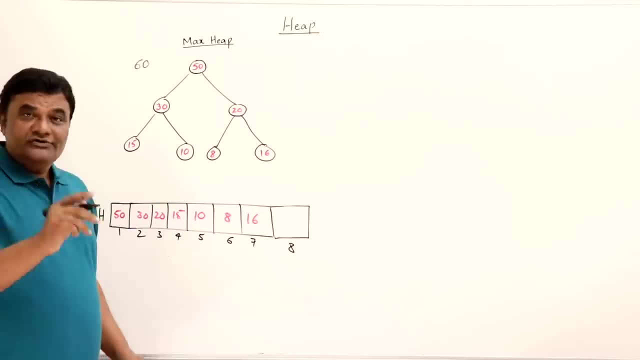 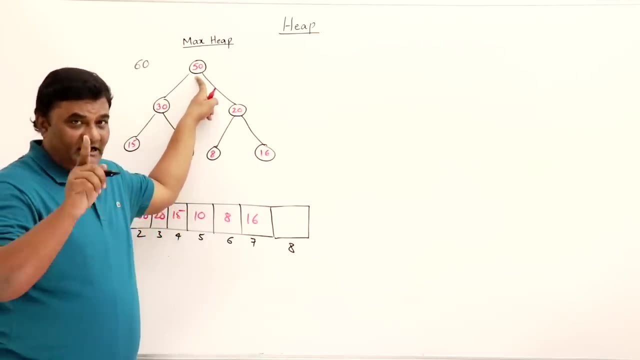 So let us see see where the 60 should come. Root should have the largest element, So 60 should come in root. Yes, Now what usually people think? I will talk about that, Then I will show you what is the right method. 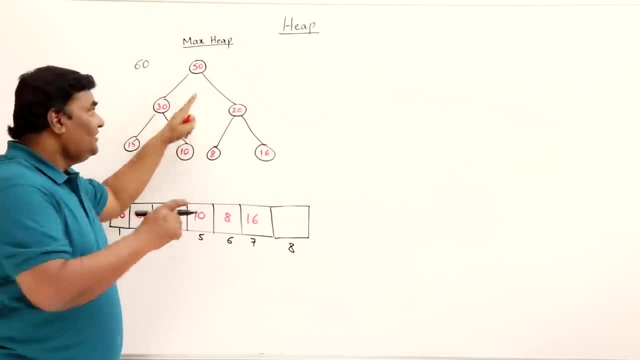 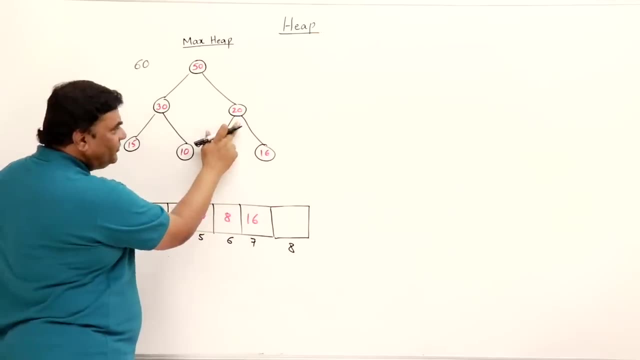 People think that 60 should be inserted here. Then where 50 should go, 50 should go. OK, this is 30. That is 20.. So this is small enough. 50 should go this side. OK, Then where this 20 should go, 20 should come this side. 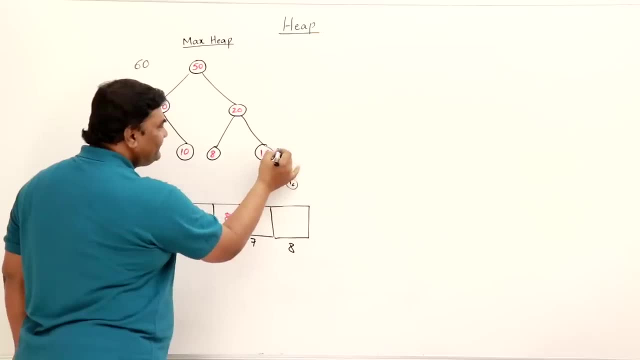 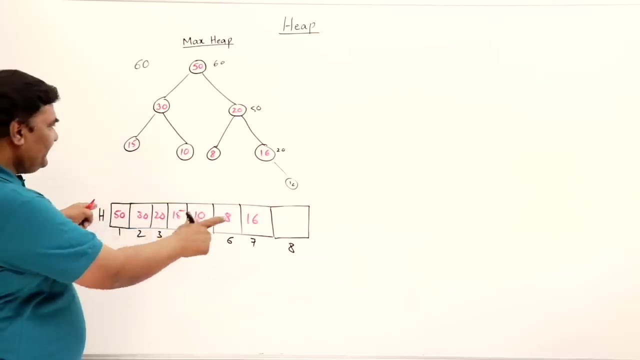 So in this way, it will extend in this direction: 16 will come here and this will become 20, and this will become 50, and this will become 60. Now, if we do it like this, is it a complete binary tree. 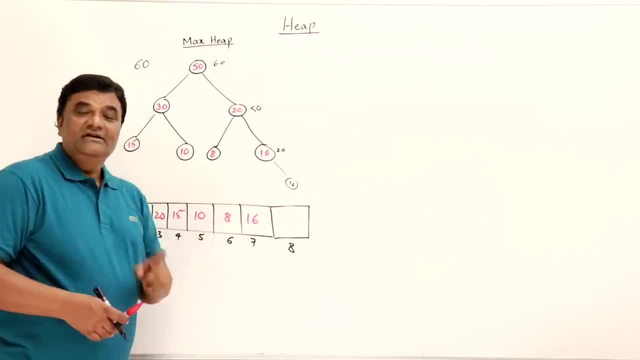 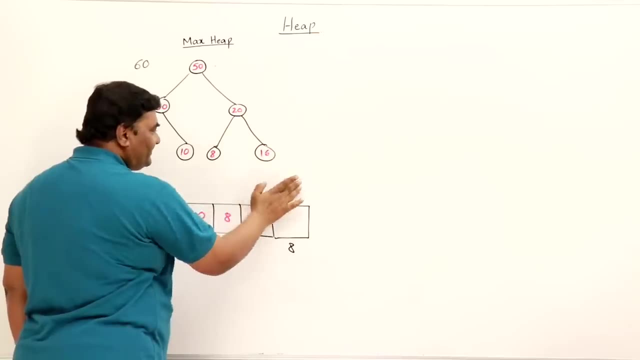 No, All these are missing element. Then we have the 16 here. This is wrong, So don't insert it in the root. So I have shown you the wrong procedure or wrong assumption. what people will have. This is wrong. It is not inserted in the root. 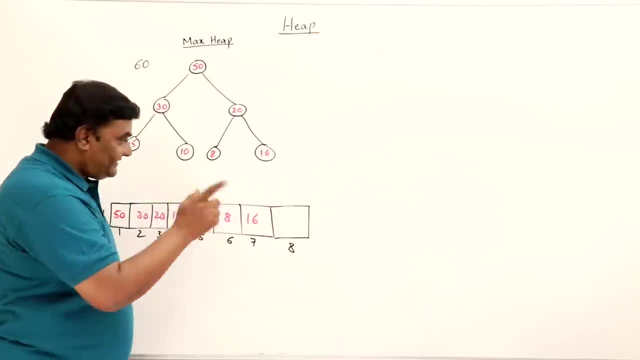 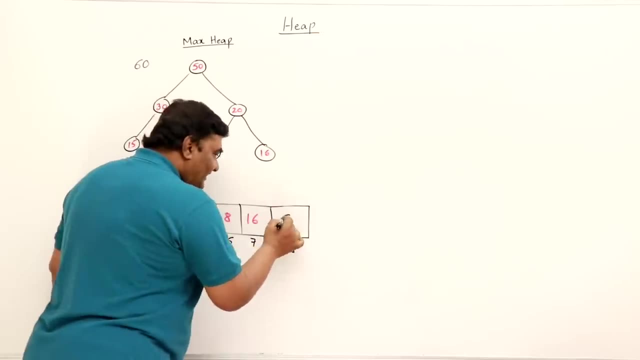 Then how it is inserted, where it is inserted. Look at this the correct procedure. See, we actually implement in an array So that 60 should be inserted here at the last free space in an array. Our heap was ending here, right. 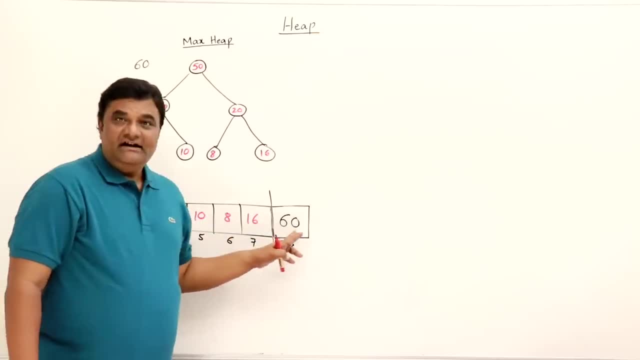 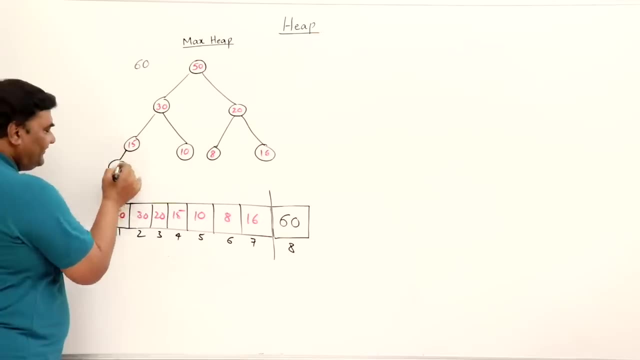 It was ending here. Now I have 16.. I have included it there and that's free space, right. So in diagram, where it will be, 60 will be on the left child of 15.. Check it: Where is 15?? 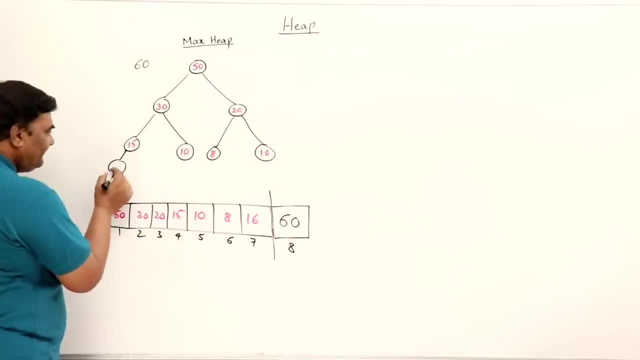 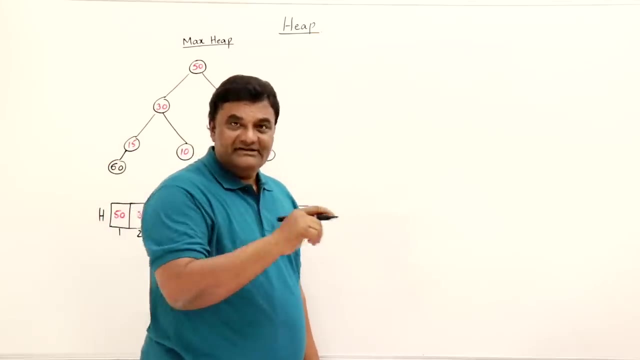 At 4.. 2, 4s, 8.. Yes, it is a left child of 15.. So this 60 is inserted here. inserted here. Yes, it's not a part of heap. I have kept it separately. Now is it forming a heap? 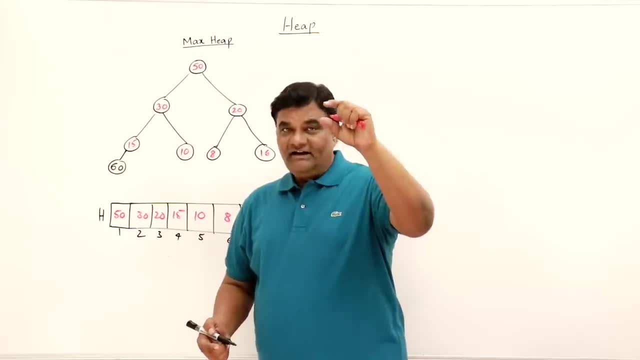 No, that condition is violated. Every node should have the value greater than all. It's not a descendant, but you see, 60 is there. That is a child of 15.. Wrong, Then, what to do? Adjust the element. Adjust the element. 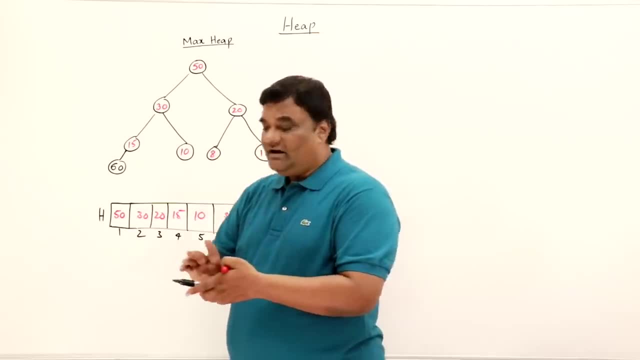 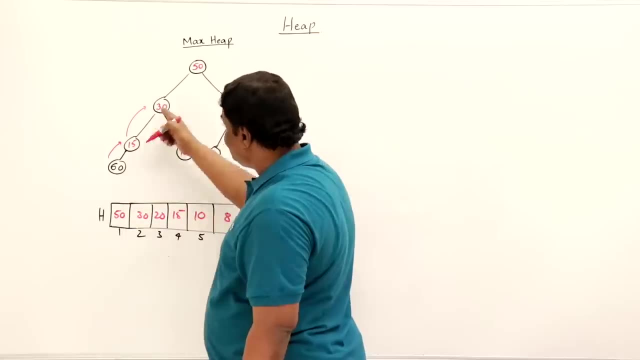 Make it as a heap or insert it in a heap. How? Compare with the parent, Who is the parent? 60 is greater than 15.. So 60 should go up. and again compare with the parent: 60 is greater than 30 also. 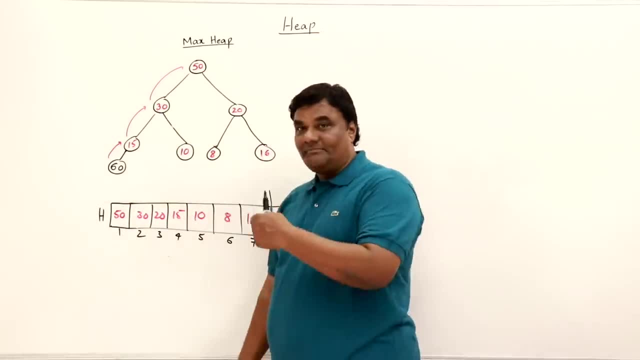 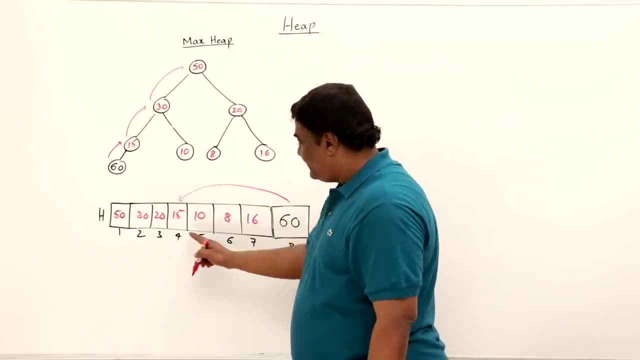 So it should go up. and 16 is greater than 50 also, So it should go up. So check here in this array, representation 8.. 8 by 2. 4. So check with this one: 4 by 2.. 2.. Check with this one. 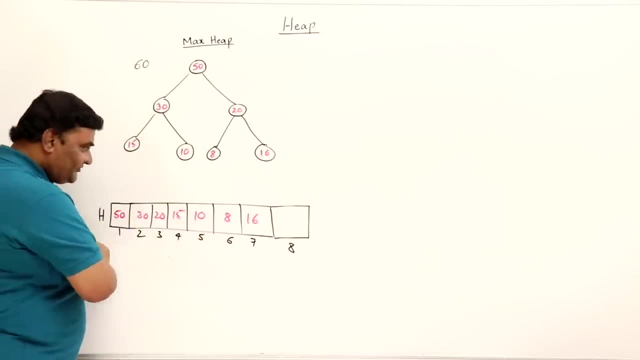 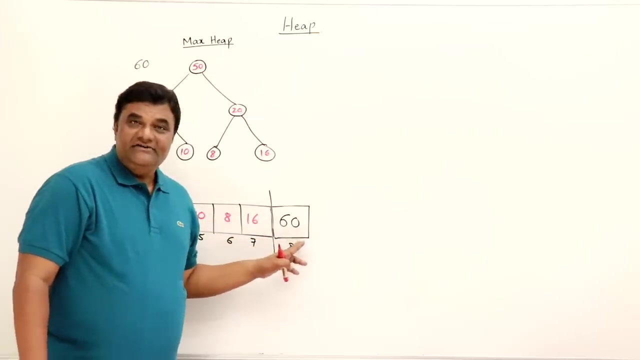 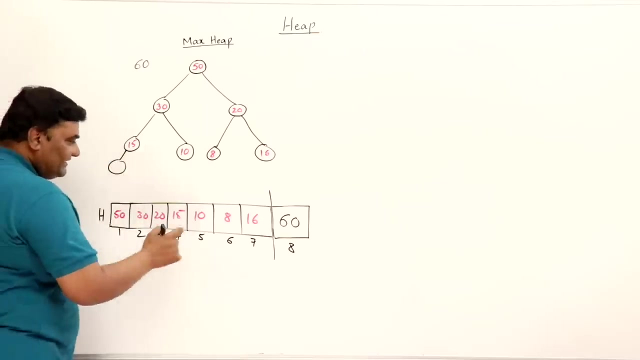 look at this the correct procedure, see. we actually implement in an array so that 60 should be inserted here, at the last free space in an array. our heap was ending here, right, it was ending here. now i have 60 included there and that's free space, right. so in diagram, where it will be, 60 will be on the left child of 15. check it, where is 15? 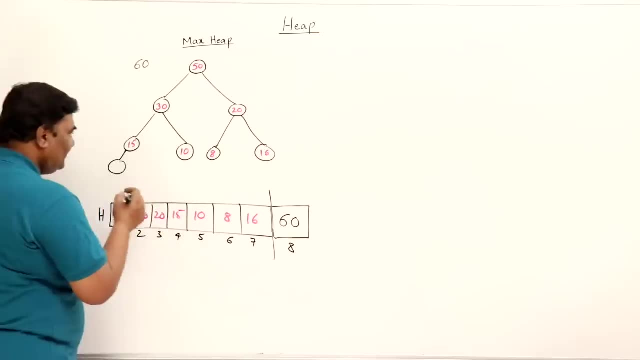 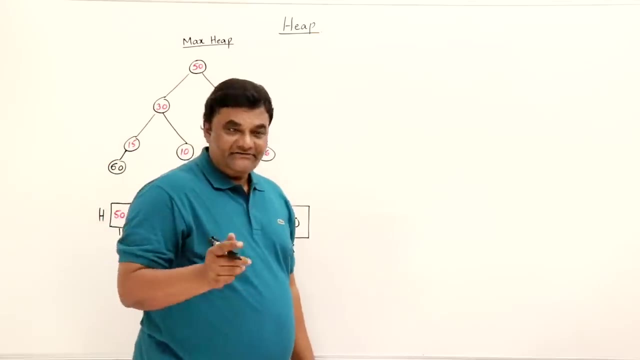 at 4, 2, 4, 8. yes, it is a left child of 15, so this 60 is inserted here. inserted here. yes, it's not a part of heap. i have kept it separately. now is it forming a heap? no, that condition is violated. 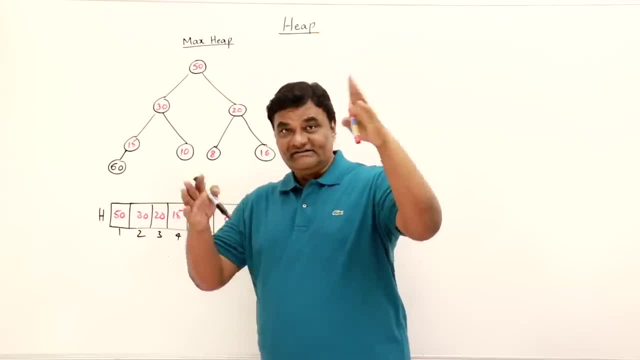 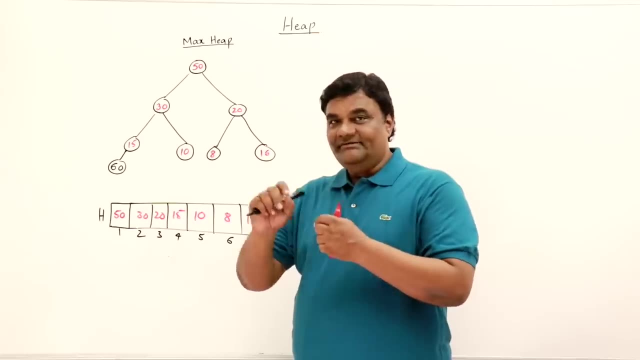 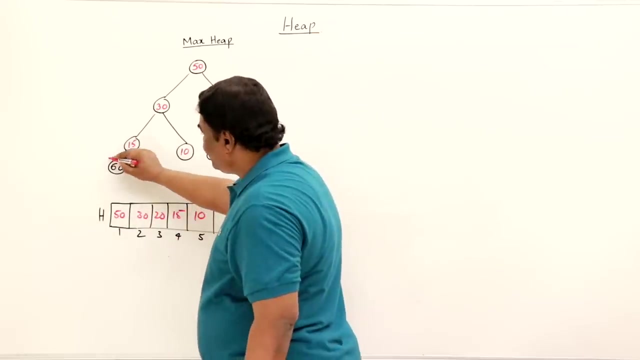 every node should have the value greater than all its descendant. but you see, 60 is there. that is a child of 15. wrong, then what to do? adjust the element. adjust the element, make it as a heap, or insert it in a heap. how compare with the parent? who is the parent? 60 is greater than 15, so 60 should. 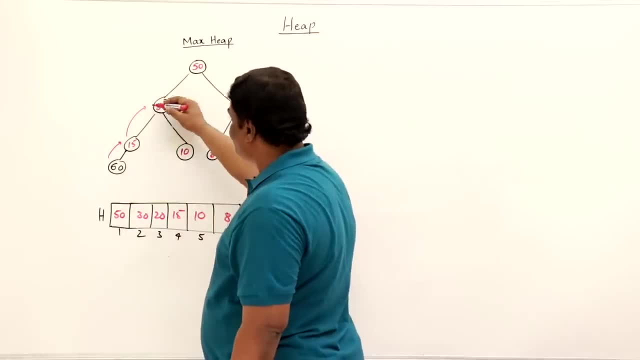 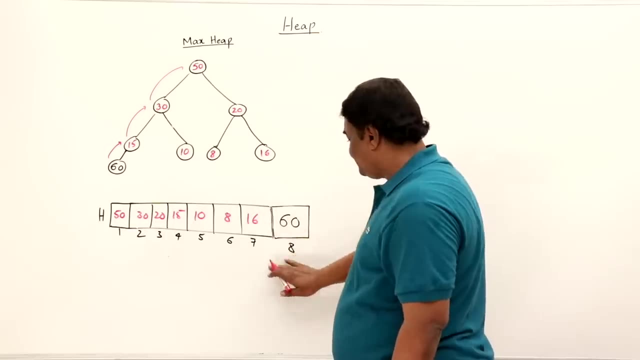 go up. and again compare with the parent: 60 is greater than 30 also, so it should go up. and 16 is greater than 50 also, so it should go up. so check here in this array: representation: 8, 8 by 2, 4. so 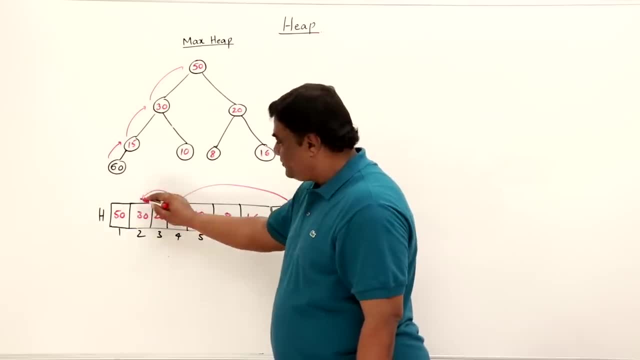 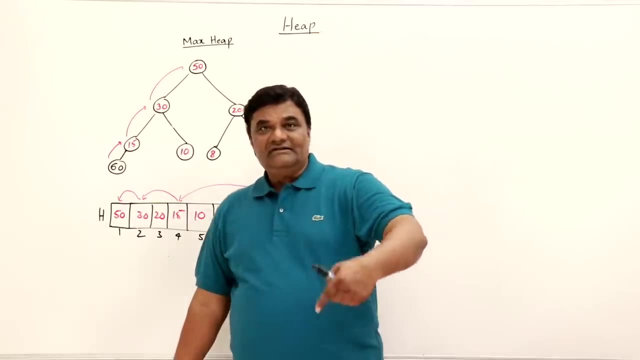 check with this one: 4 by 2. 2 check with this one: 2 by 2: 1 check with this one. so 60 is compared with this one and its parent and its parent. so 60 is compared with all its ancestors, and it will reach its right place. 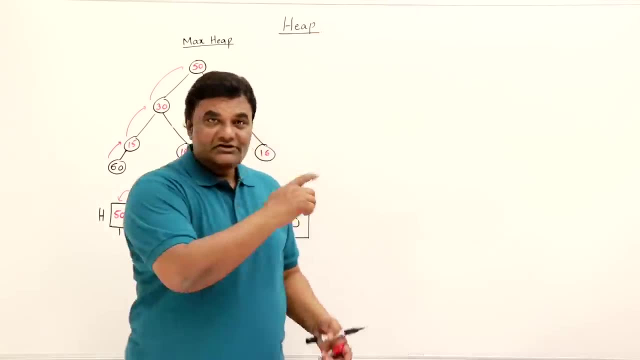 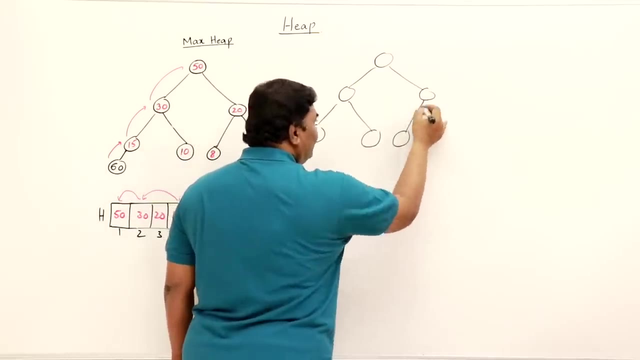 so it will swap all these elements and 60 will go there. so i will draw it here. see, 60 will come here. i will draw a tree first, then i will fill the elements right after inserting. how it looks like now. this is a array, so here i kept them empty. 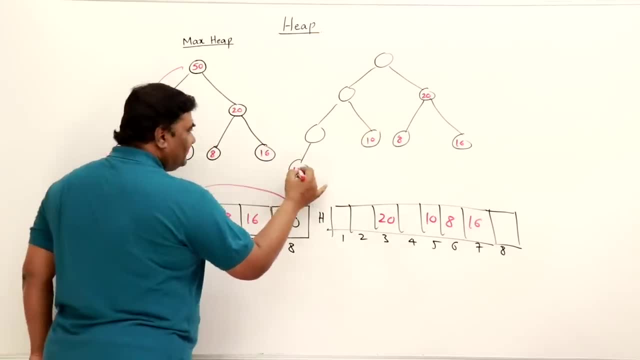 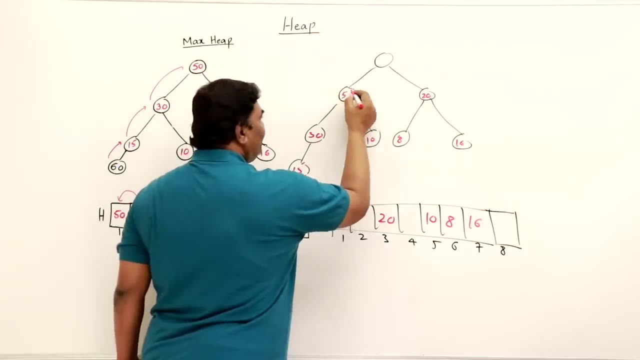 just watch it: 60 will go up, 15 will come down, and again 60 will go up and 30 will come down. 30 will come here, then 60 will go up and 50 will come down. so we adjust the element like this: so 60 comes here. 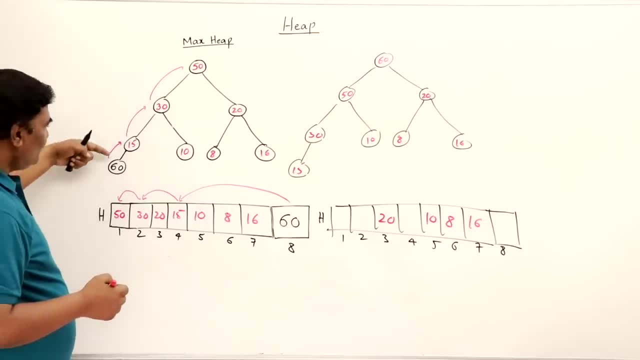 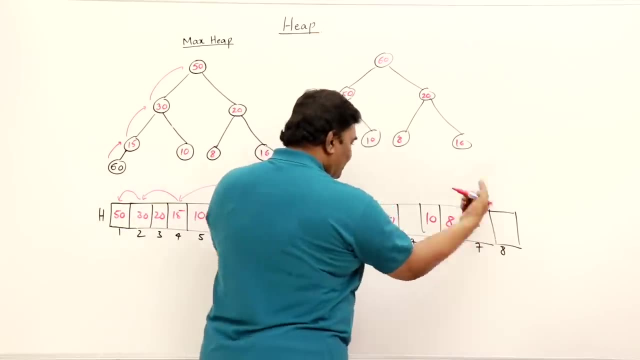 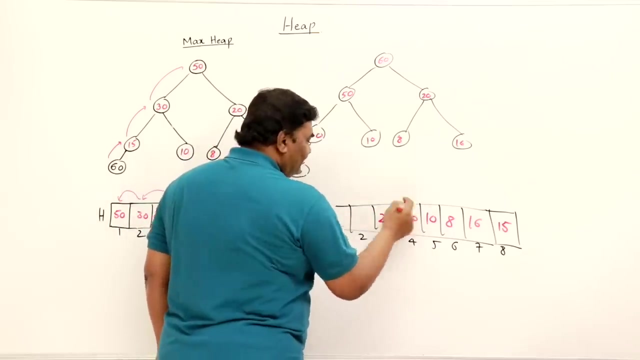 so it has moved up in the hierarchy towards the ancestors and it has reached the root, because now it is the largest element. so in an array, if you see, 60 was here, so 15 went, 60 was here, so this 15 went there and 60 came here, then again 30 went there and 60 came here, so this 15 went there and 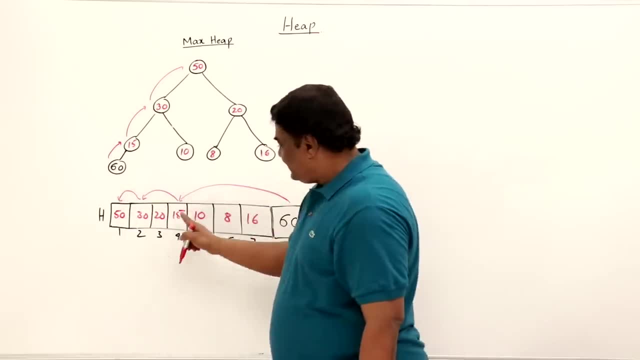 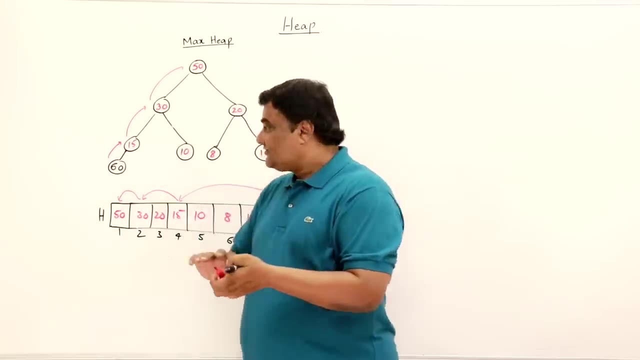 2 by 2.. 1. Check with this one. So 60 is compared with this one and its parent and its parent. So 60 is compared with all its ancestors and it will reach its right place. So it will swap all these elements and 60 will go there. 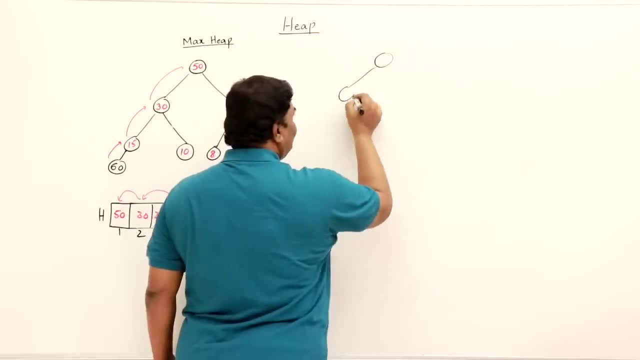 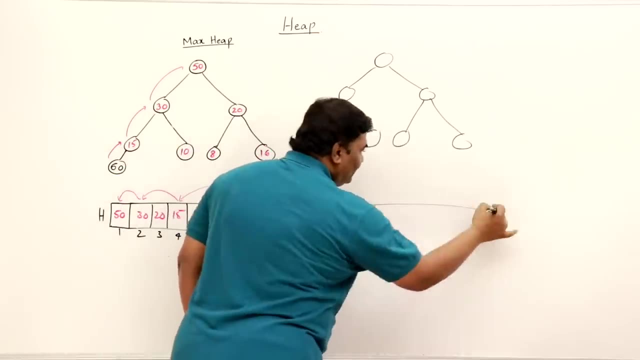 So I will draw it here. See, 60 will come here. I will draw a tree first, Then I will fill the elements right after inserting how it looks like Now. this is our array. So here I kept them empty. Just watch it. 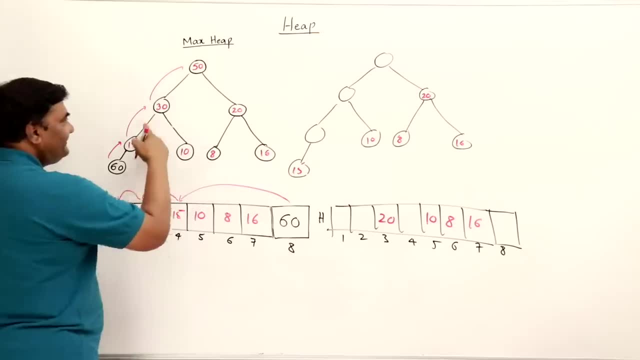 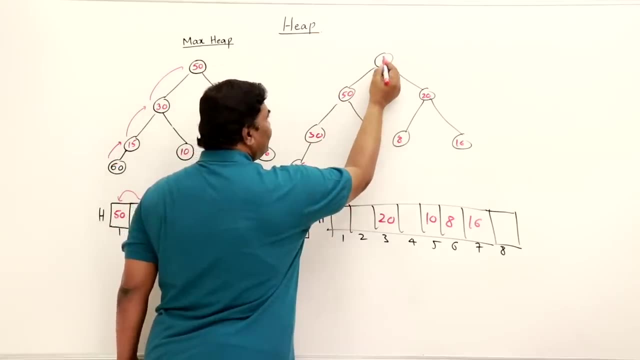 60 will go up, 15 will come down, and again 60 will go up and 30 will come down. 30 will come here, Then 60 will go up and 50 will come down. So we adjust the element like this: 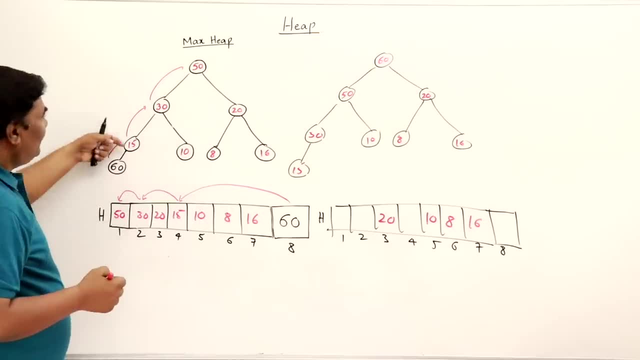 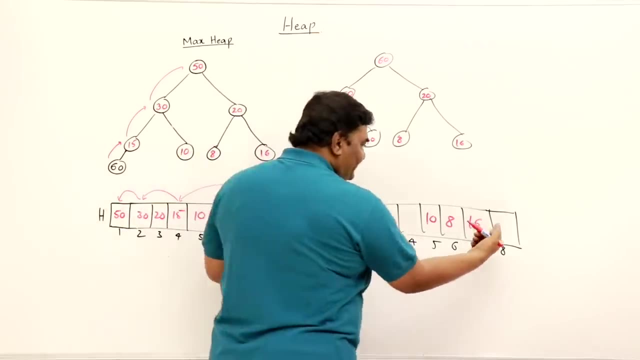 So 60 comes here. So it has moved up in the hierarchy towards the ancestors and it has reached the root, because now it is the largest element. So in an array, if you see, 60 was here, So 15 went, 60 was here. 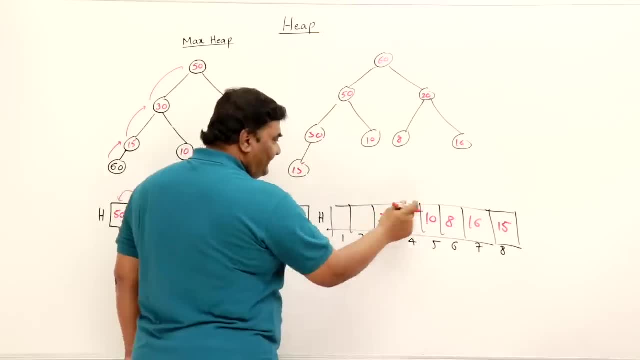 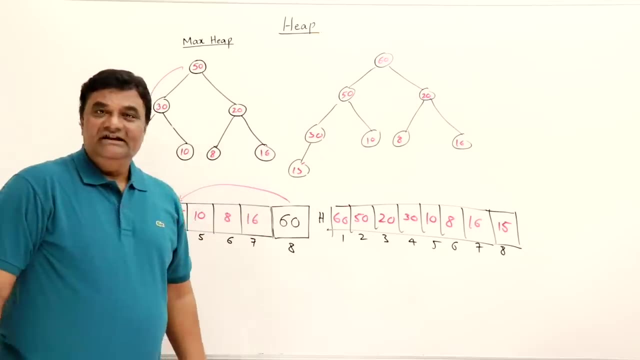 So this 15 went there, 60 came here, Then again 30 went there and 60 came here, Then 50 went to its place and 60 is inserted here. So this is how the heap looks like diagrammatically and also in an array. 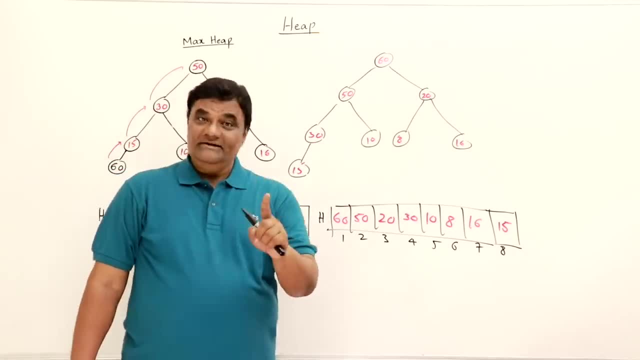 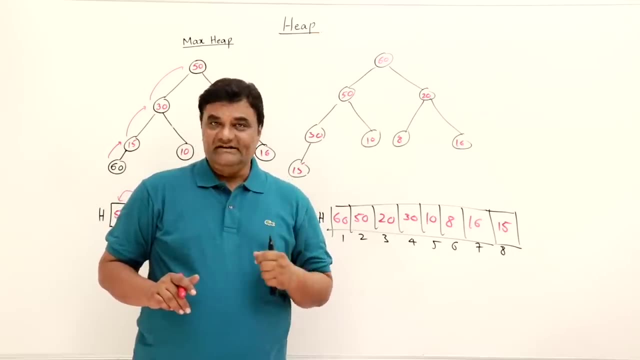 So this is insertion. We have inserted only one element in a heap that we have taken max heap. Now a little bit analysis. How much time it has taken. It has taken the time equal to the number of swaps. So maximum how many swaps? 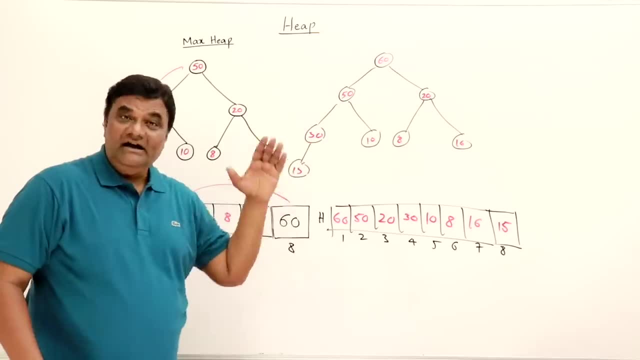 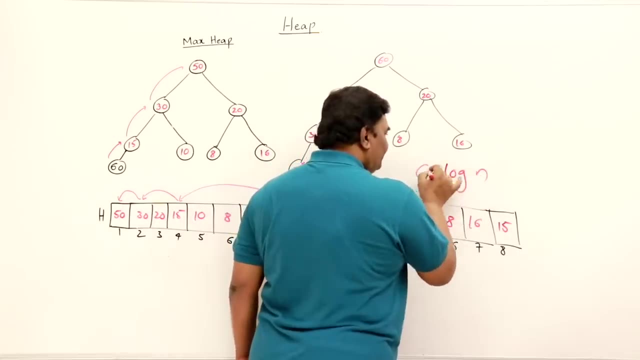 One, two, three. So actually this is depends on the height of a tree. So what is the height of a complete binary tree? Height of a complete binary tree is log n. Yes, So it means the time is big O of log n or order of log n. 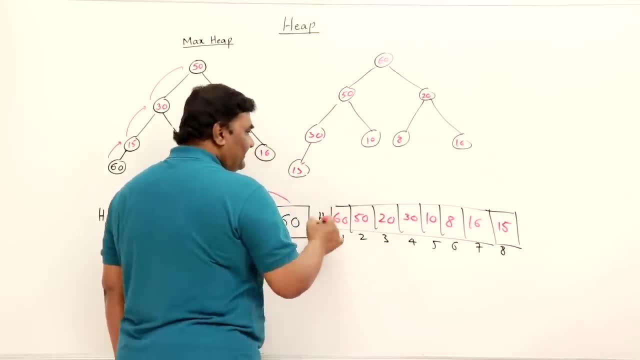 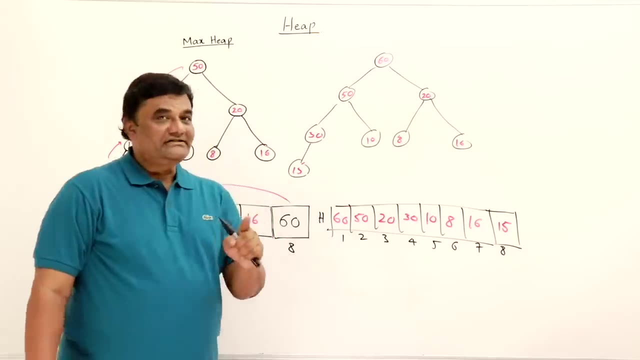 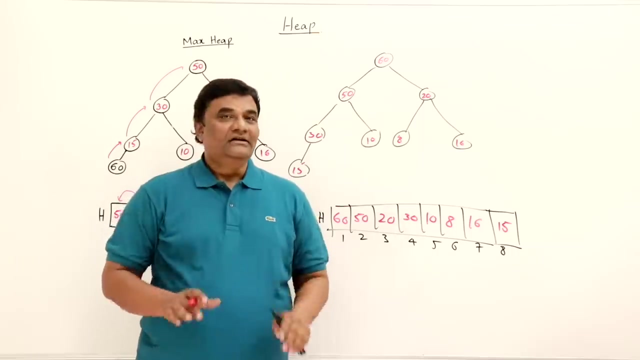 60 came here, then 50 went to its place and 60 is inserted here. so this is how the heap looks like diagrammatically and also in an array. so this is insertion. we have inserted only one element in a heap, that we have taken: max heap. now a little bit analysis: how much time it has taken. it has taken. 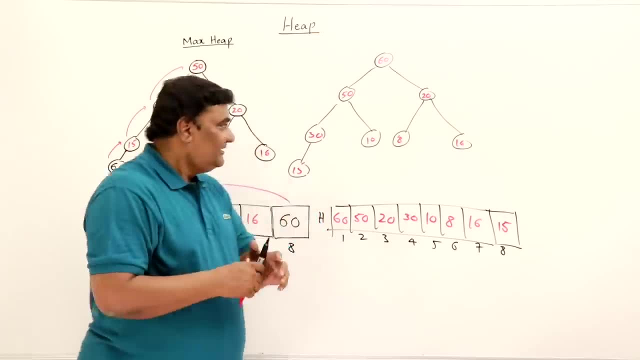 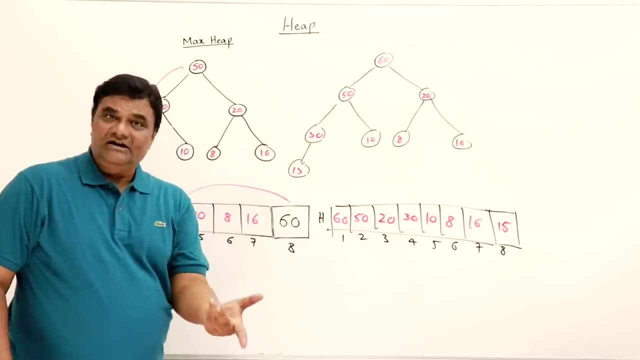 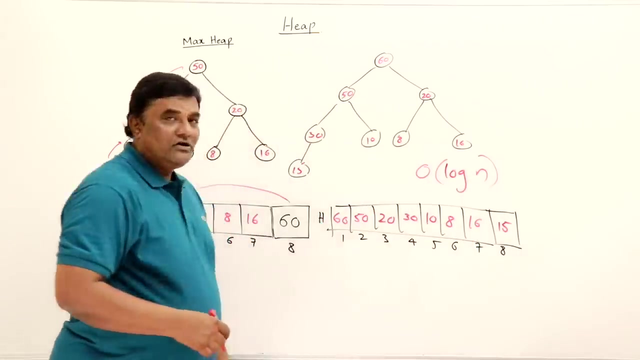 the time equal to the number of swaps. so maximum, how many swaps? one, two, three. so actually this is depends on the height of a tree. so what is the height of a complete binary tree? height of a complete binary tree is log n. yes, so it means the time is big O of log n or order of log n. so the time taken for 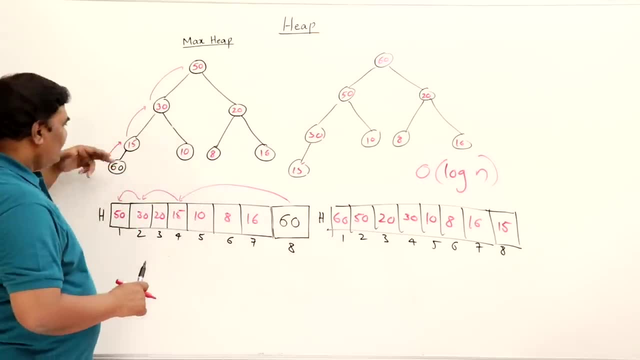 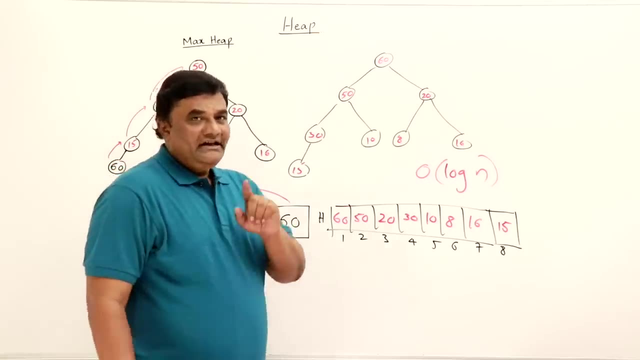 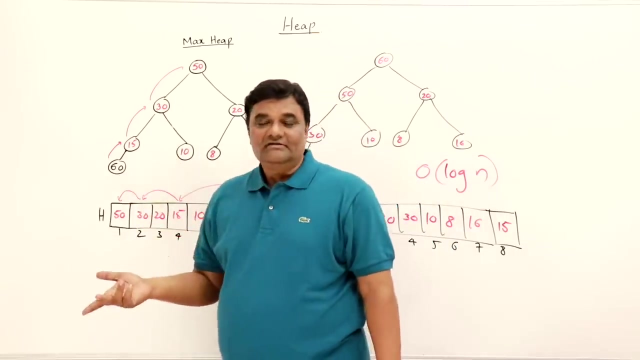 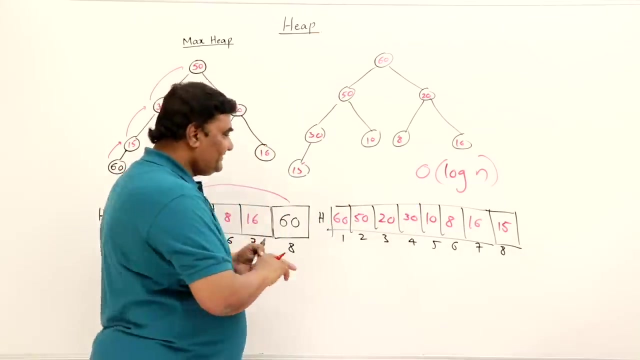 insertion is log n. how many swaps are required? one, two, three. so that depends on the height log n number of swaps are required. and one more thing: if suppose this was not 60, if this was 6, then we don't have to swap anything, zero swaps. so we can say that the time taken for inserting one element in a heap is minimum. big O of. 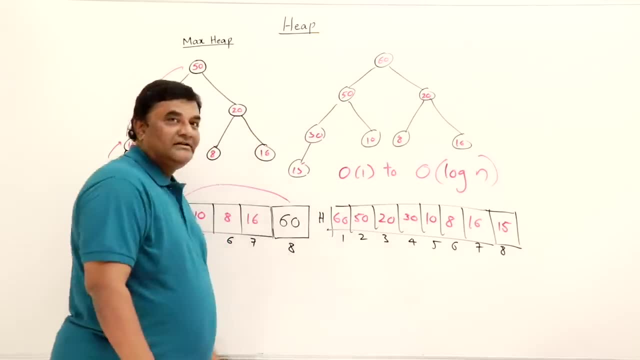 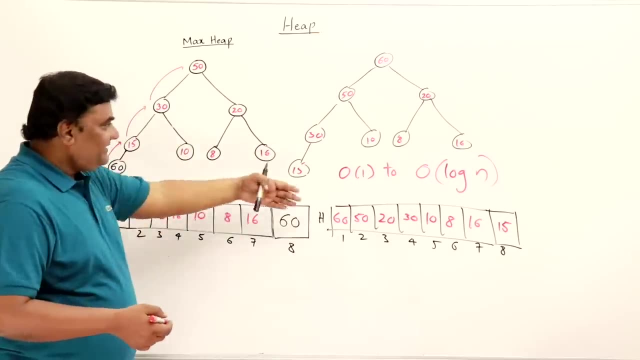 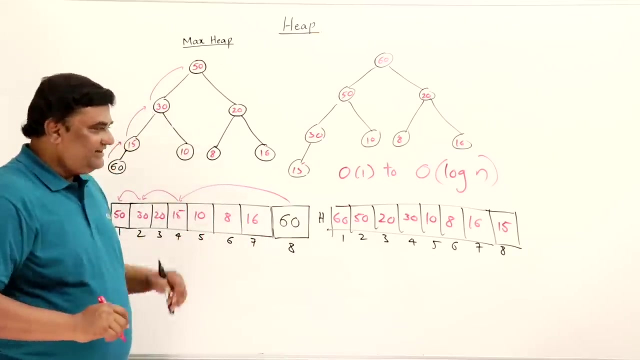 one and maximum is log n. it can be from one constant to log n. minimum time is no swapping is required. maximum the swapping requires depends on the height. so that is log n. so this was inserting just one element in existing heap. now, before going to delete, I have something to show you. so this is: 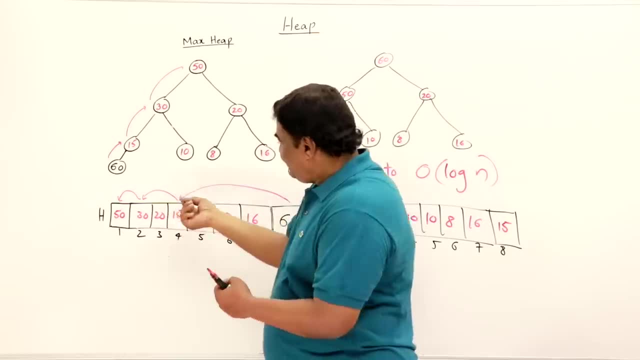 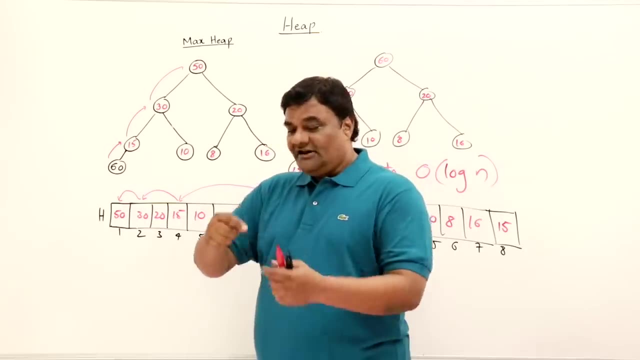 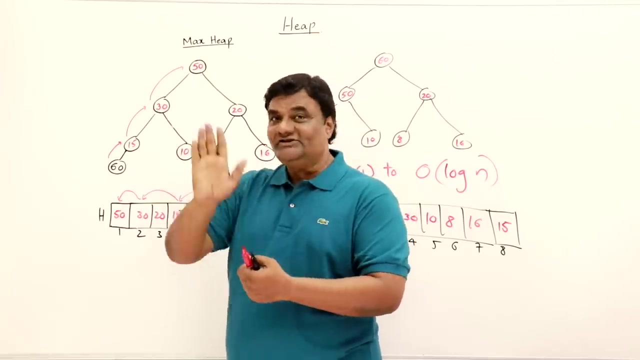 just one element in existing heap. now, before going to delete, I have something to show you. observe one thing: see, when we are inserting we have to send the element upwards. first we add the new element as a leaf, then we adjust it by comparing with the ancestors. so element moves from leaf towards root. so the direction of 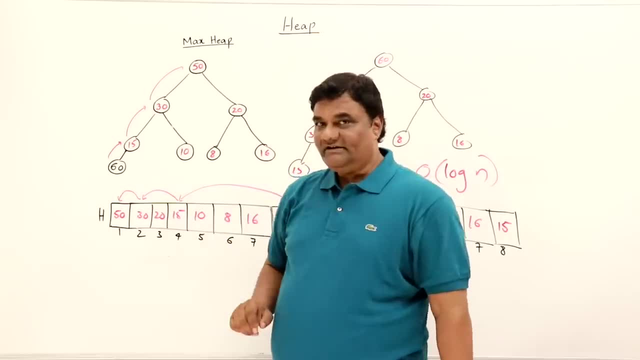 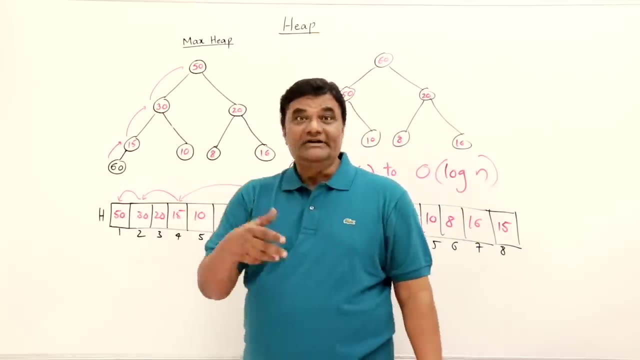 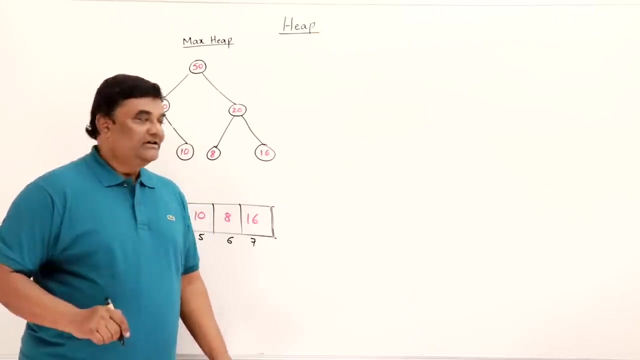 adjustment is upwards. this is the important thing. this is the important thing. so, anyway, next I will take the same example, then in this one, only I will show you how to delete. so let us look at the now. let us look at delete operation on max heap. here is a max heap. 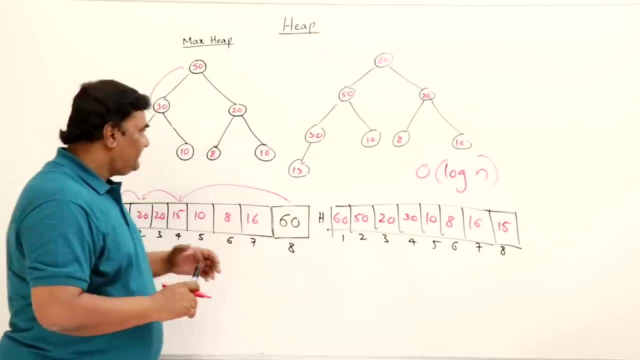 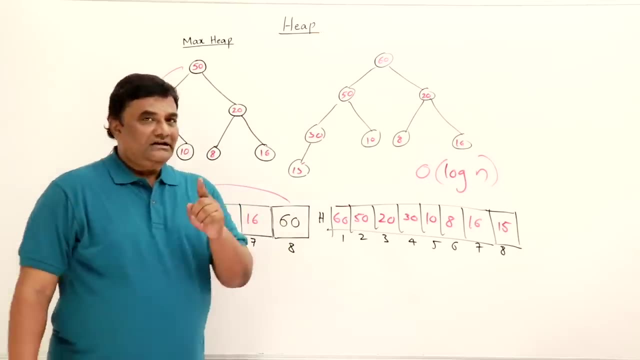 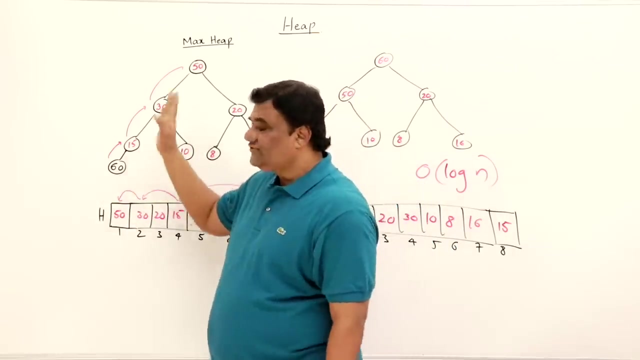 So the time taken for insertion is log n. How many swaps are required? One, two, three. So that depends on the height Log n number of swaps are required. And one more thing: If suppose this was not 60. If this was six, then we don't have to swap anything. 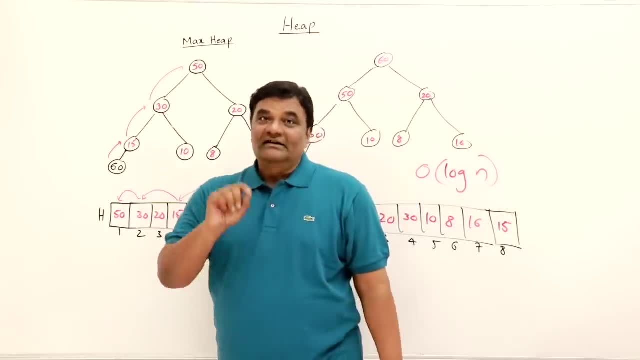 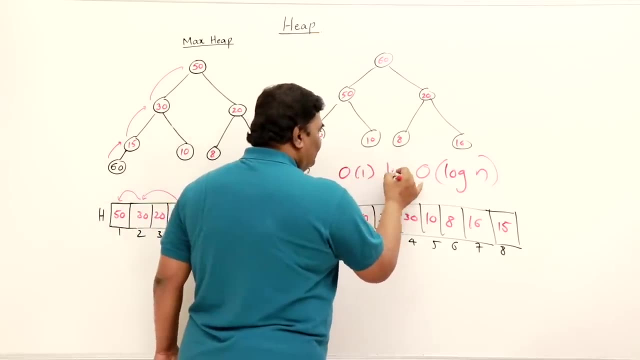 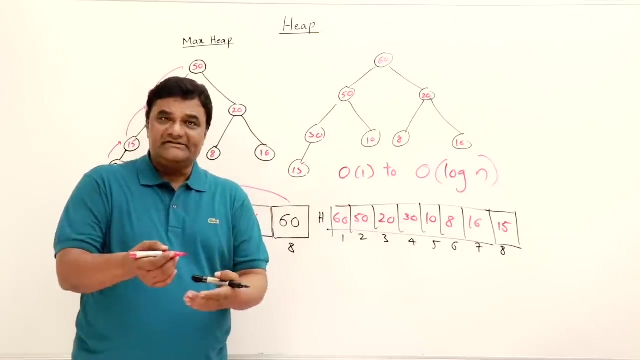 Zero swaps. So we can say that the time taken for inserting one element in a heap is minimum, big O of one and maximum is log n. It can be from one constant to log n. Minimum time is no swapping is required. Maximum the swapping requires depends on the height. 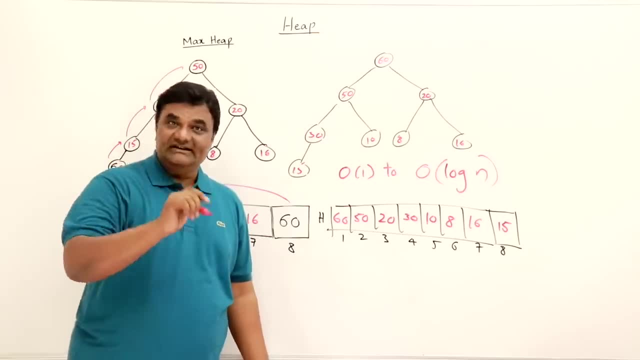 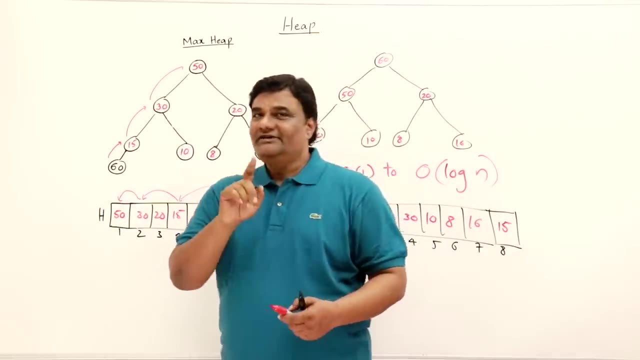 So that is log n. So this was inserting just one element In existing heap. Now, before going to delete, I have something to show you. Observe one thing, See: when we are inserting, we have to send the element upwards. 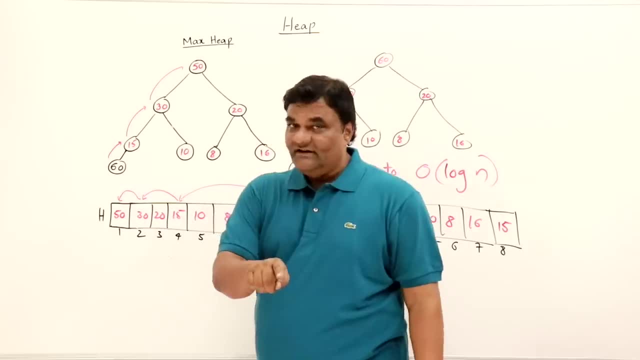 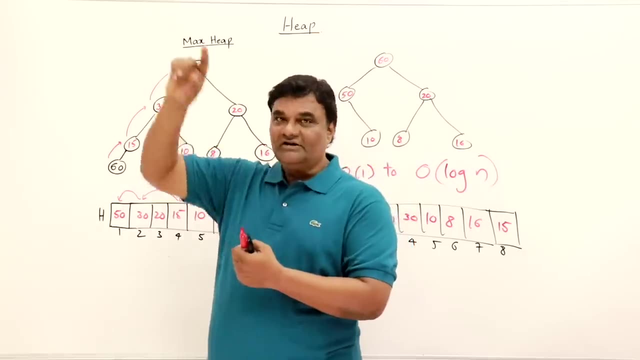 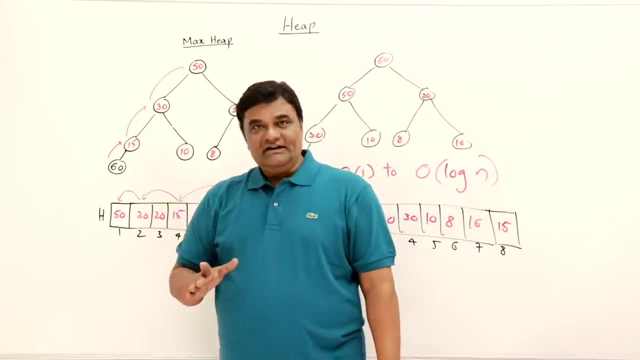 First we add the new element as a leaf, Then we adjust it by comparing with the ancestors. So element moves from leaf towards root, So the direction of adjustment is upwards. This is the important thing. This is the important thing. So, anyway, next, 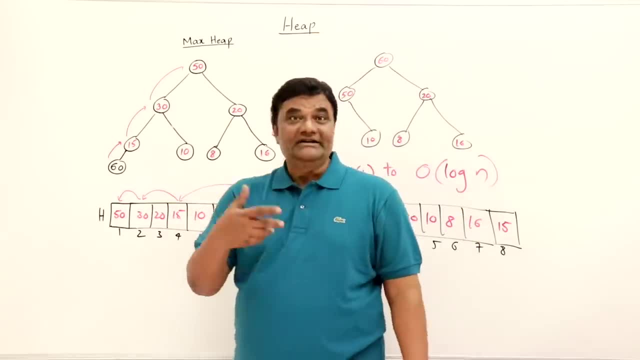 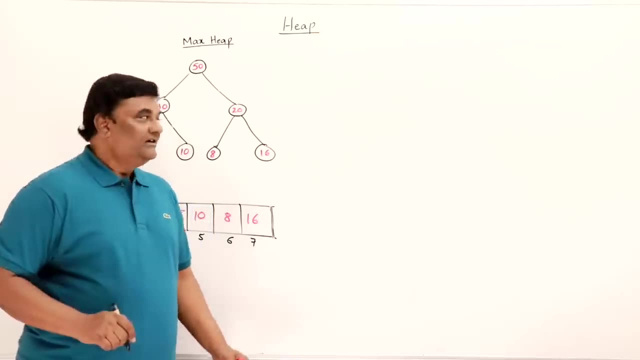 I will take the same example Then in this one only, I will show you how to delete. So let us look at it Now. let us look at delete operation on max heap. Here is a max heap with seven elements that are also there in an array. 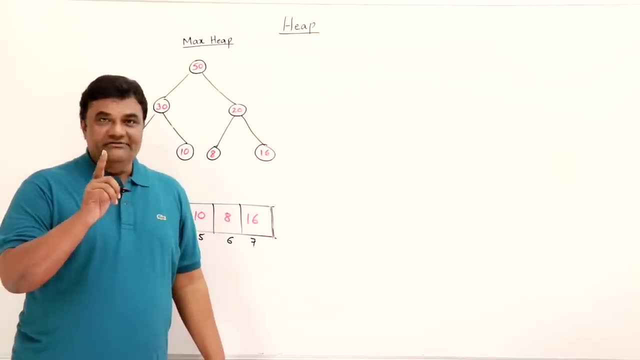 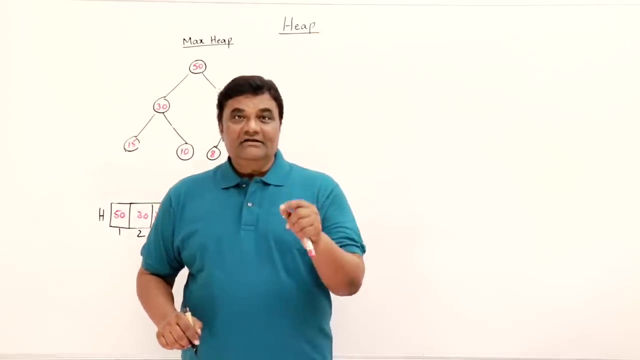 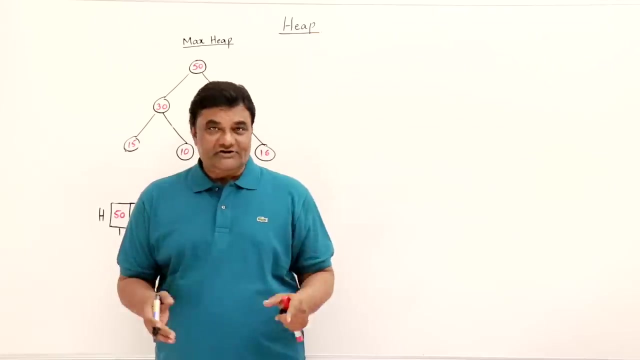 Now which element you want to delete. See the first and important thing: you cannot delete any other element. You should not delete any other element but root element. So only one element is deleted from the heap, without asking or without giving any options or choices. 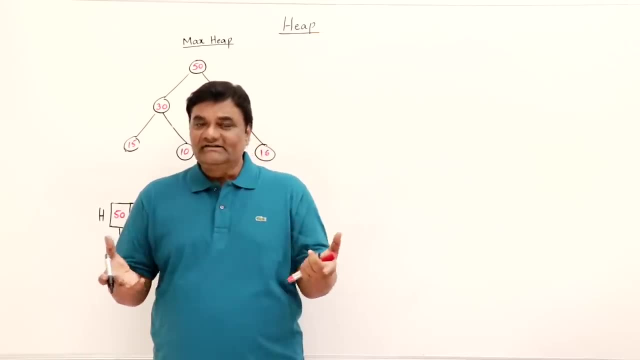 Only root element is deleted. Yes, if you're deleting root element, then only it's a heap. See, this heap is just like if you have seen in the market at a fruit shop, If apples are arranged how they arrange. They arrange it like a pyramid heap, like 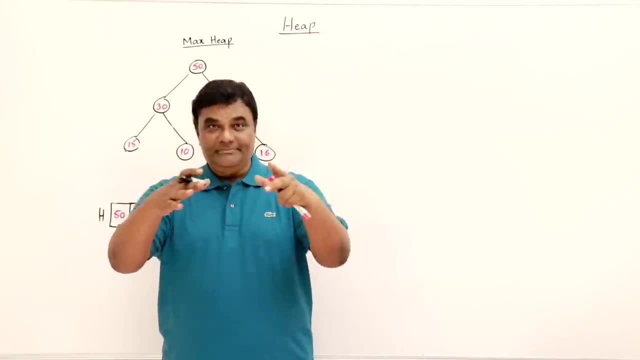 So the apples are arranged one above another, like forming a pyramid, like shape, So on the top which apple is kept. The best apple, The most shiny one among all, fresh one is kept on the top, So that is the best one. 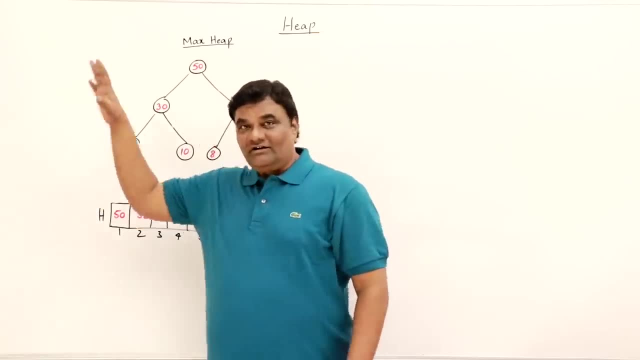 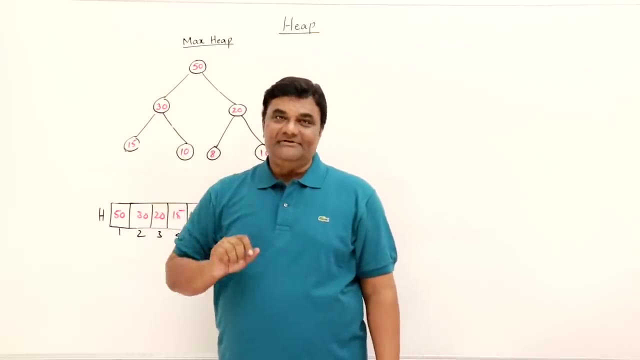 So same concept is used in heap also. So all these elements are there. which is the top, most element, best element, What is best for us, Maximum element, So that is max heap. So 50 is on the top. So if you want to remove the apple, which apple you remove? 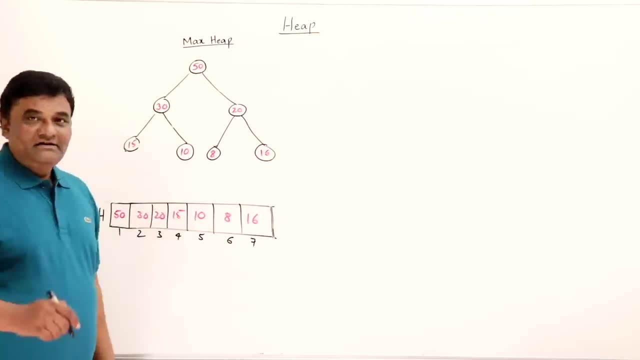 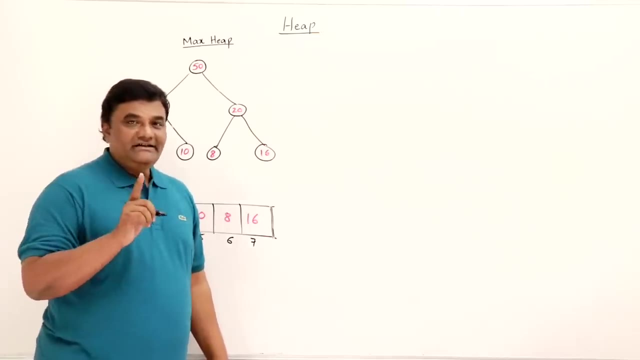 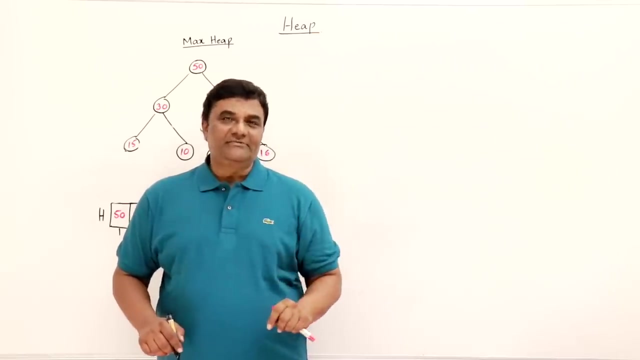 with seven elements that are also there in an array. now which elements want to delete? see the first and important thing: you cannot delete any other element. you should not delete any other element but a root element. so only one element is deleted from the heap, without asking or without giving any options or 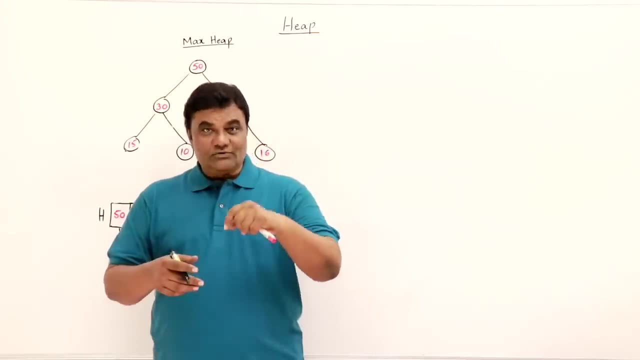 choices, only root element is deleted. yes, if you are deleting root element, then only it's a heap. see this heap is just like if you have seen in the market at a fruit shop if apples are arranged how they arrange. they arrange like a pyramid heap like. so the apples are arranged. 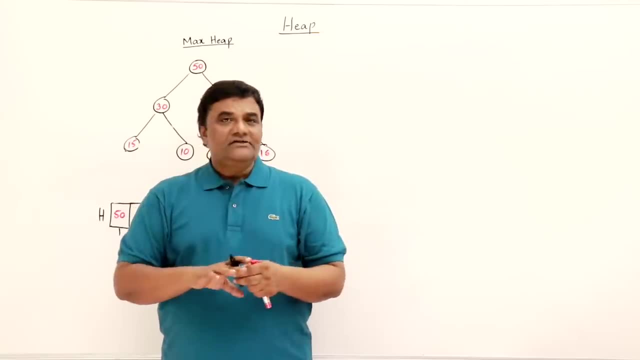 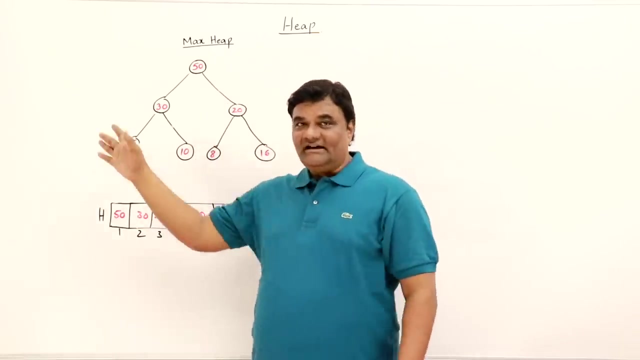 one above another, like forming a pyramid, like shape. so on the top which apple is kept? the best apple, the most shiny one among all, fresh one is kept on the top, so that is the best one. so same concept is used in heap also. so all these elements are there. which is the? 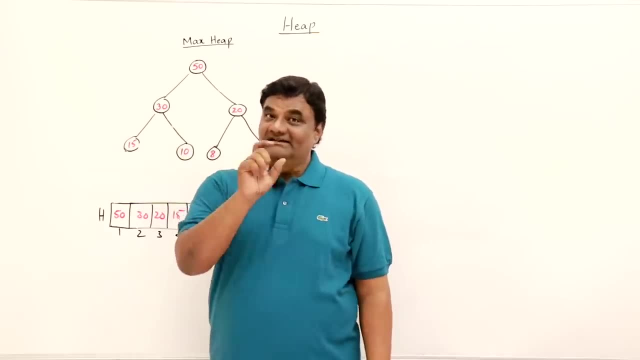 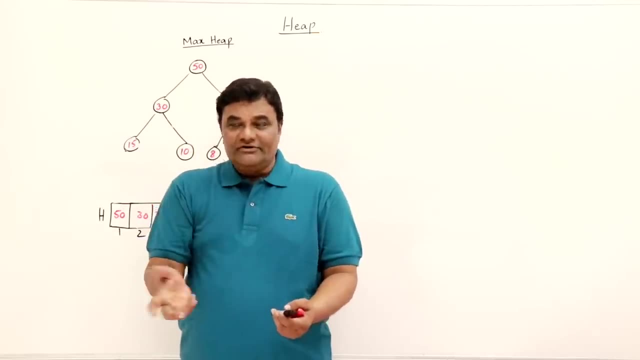 topmost element, best element, what is best for us, maximum element. so that is max heap. so 50 is on the top. so if you want to remove the apple, which apple you will remove? you cannot remove any other apple from that heap. you have to remove the topmost apple only. 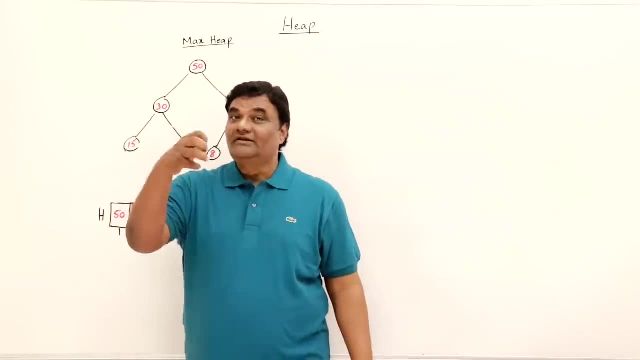 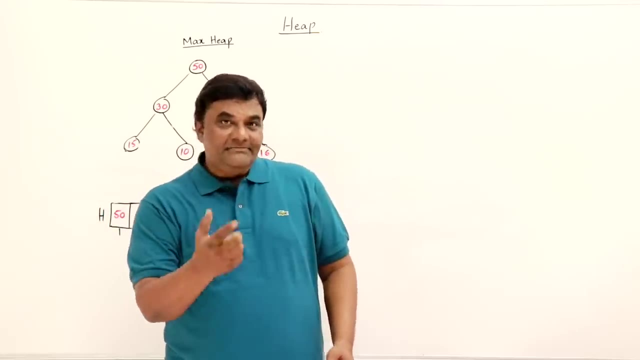 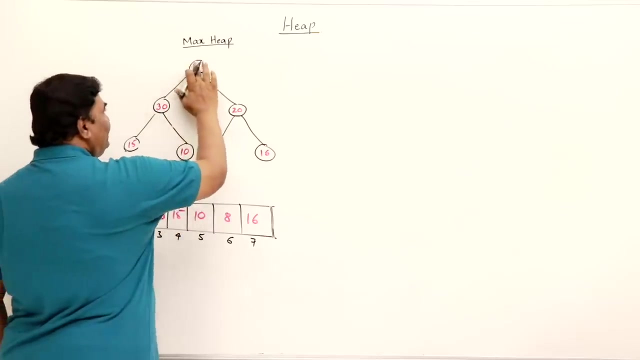 that's what. so we follow the same method here. we will remove only the root element, right. similarly in mini heap also. if you say no, maximum element is not important for us, minimum is important, then that will follow mini heap. okay, coming to this, let us delete the element so only i can delete 50. 50 is gone, now again. 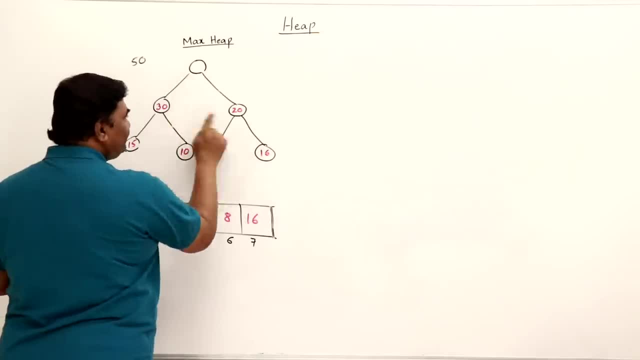 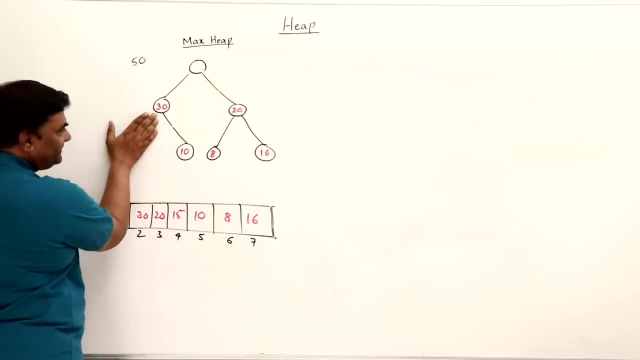 sometimes people mistake here the thing that 30 should go up because this is bigger. okay, 30 will go up. then who will come at the place of 30, 15? so if 15 goes here, 30 goes here, then this node is gone. if this node is gone, is it looking like a complete binary? no, so if 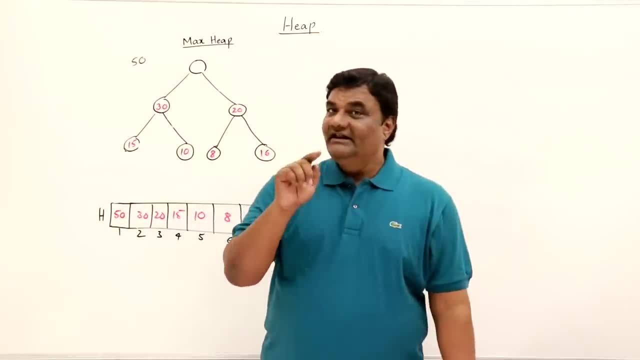 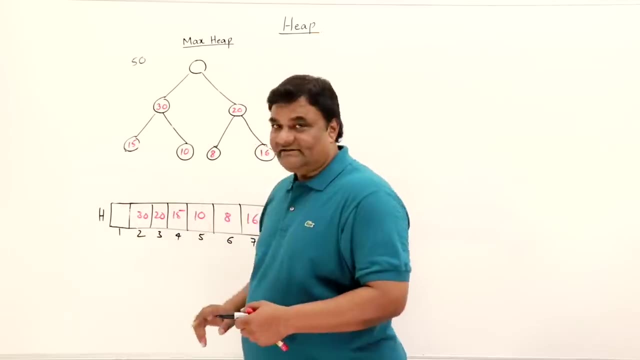 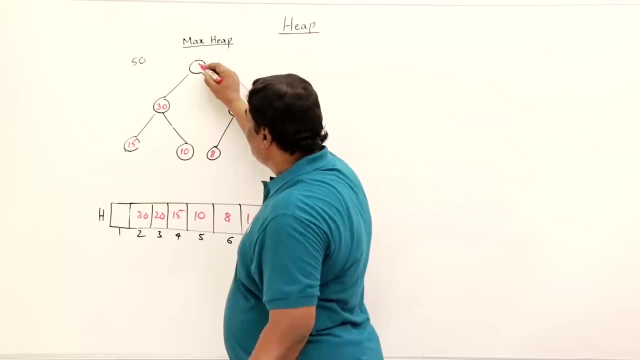 just as you like. it will not be a complete binary, so you have to be careful for preserving complete binary property. then what to do? so when 50 is gone, who should take its place? see the last element in complete binary: this element. this element will come in its place. 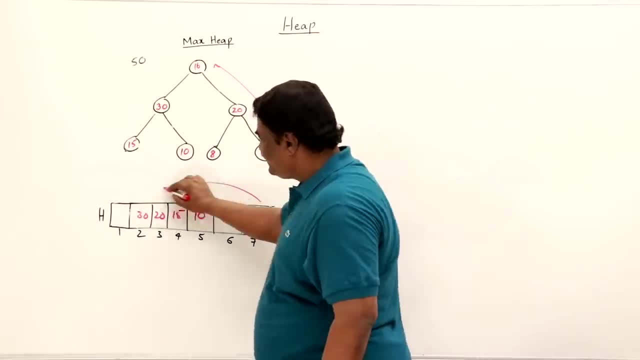 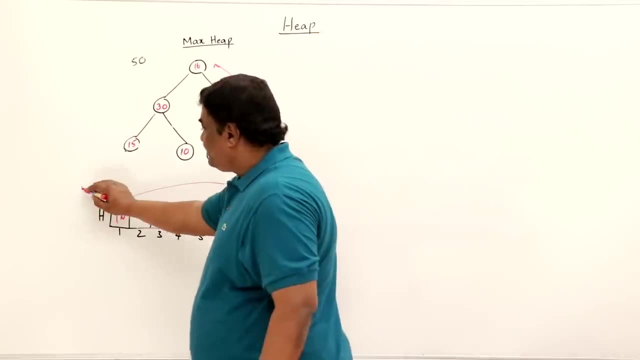 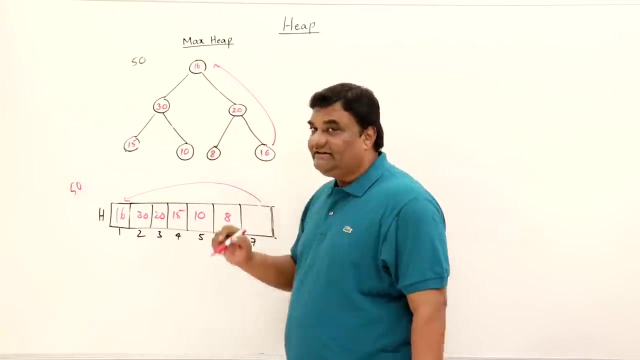 that is, 16 will come here. so 16 is removed from here. so 16 is brought here. 16 is removed from here. this is gone, so 16 is brought there. 50 is gone. gone outside. we have deleted the element at 50. 50 has gone out. we have deleted it. then in its place the last element in complete. 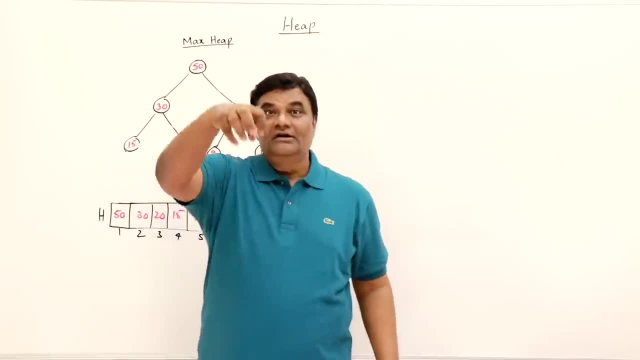 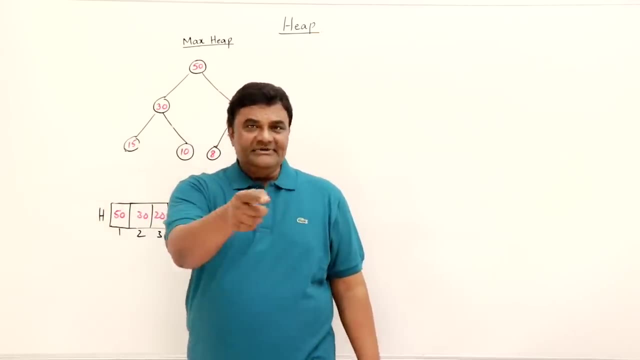 you cannot remove any other apple from that heap. You have to remove the top most apple only. That's what. So we follow the same method here. We will remove only the root element right. Similarly in min heap also. If you say no, maximum element is not important for us. 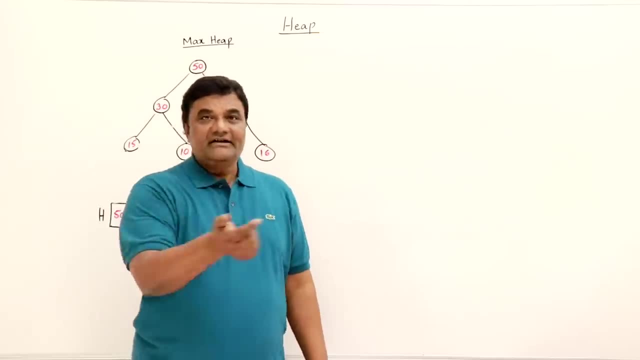 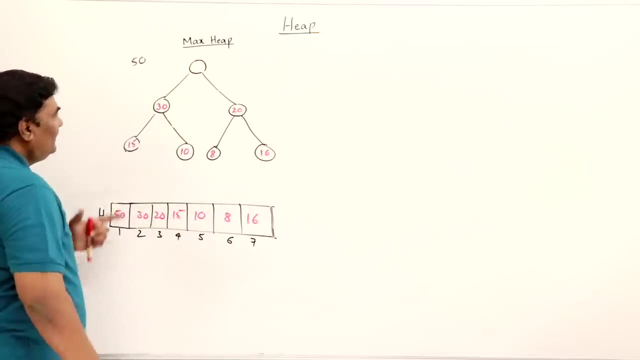 Minimum is important, Then that will follow min heap. OK, coming to this, Let us delete the element So only I can delete 50,. 50 is gone. Now again. sometimes people mistake here The thing that 30 should go up because this is bigger. 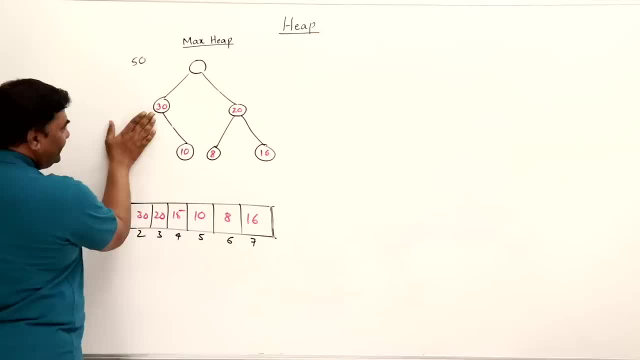 OK, 30 will go up. Then who will come at the place of 30? 15.. So if 15 goes here, 30 goes here, then this node is gone. If this node is gone, is it looking like a complete binary? 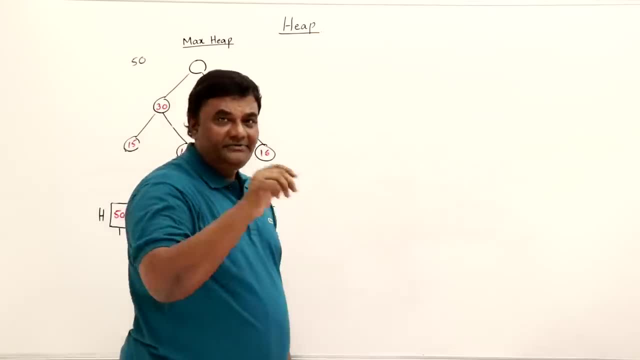 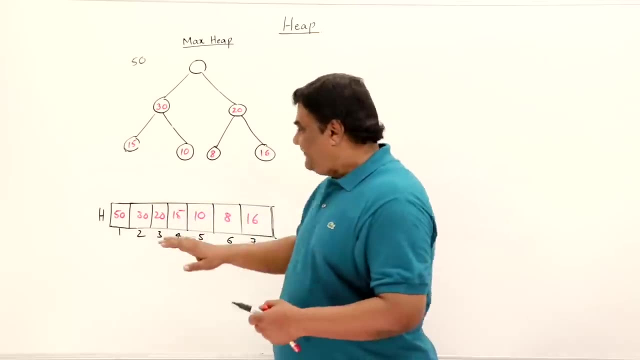 No. So if you try to adjust as you like, it will not be a complete binary, So you have to be careful for preserving complete binary property. Then what to do? So when 50 is gone, who should take its place? See the last element in complete binary. 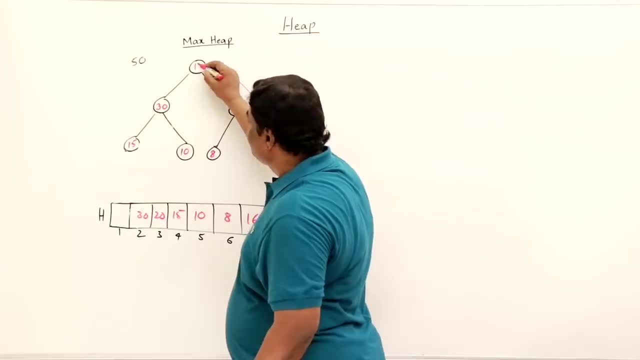 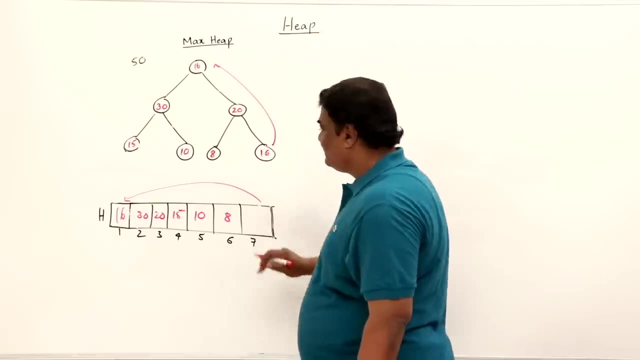 This element. this element will come in its place, That is, 16 will come here, So 16 is removed from here. So 16 is brought here. 16 is removed from here. This is gone, So 16 is brought there. 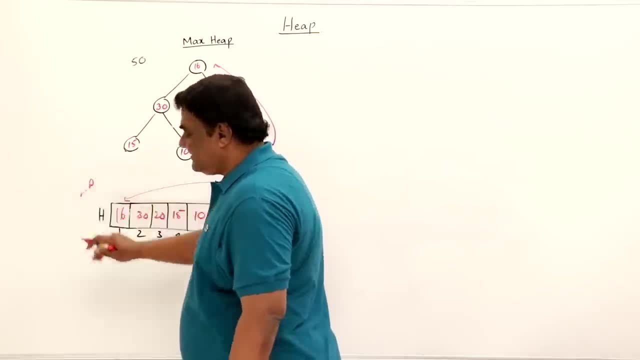 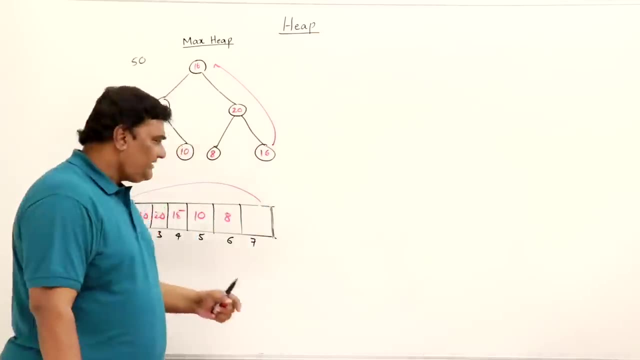 50 is gone outside. We have deleted that 50.. 50 has gone out. We have deleted it. Then in its place, the last element in complete binary. Last element in complete binary means in an array the last element will take its place. 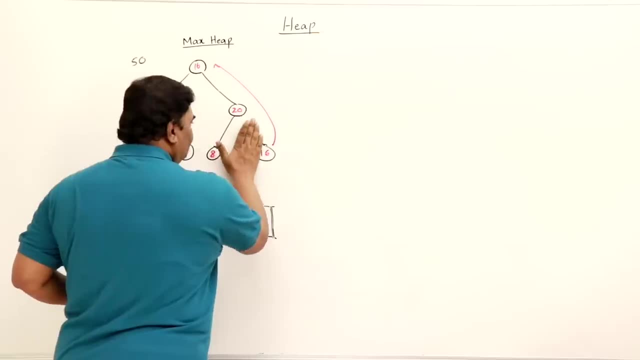 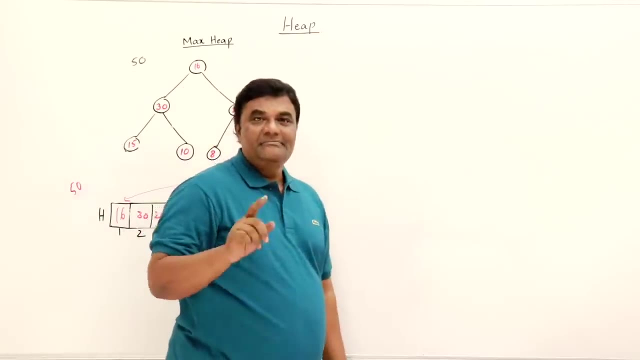 Now this is how it looks like, So I'll remove this one now. OK, I'll remove this. This is gone. So you have already seen it. It's here now. Now, this is complete binary, but not a max heap. 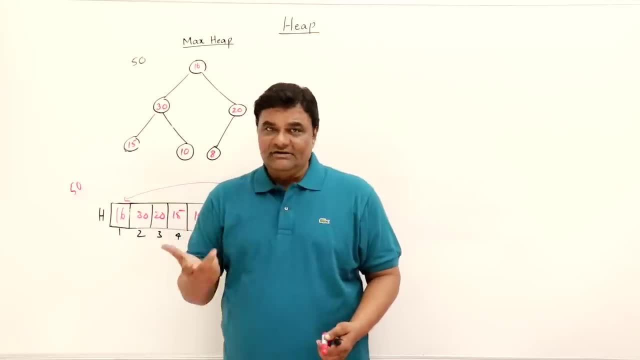 So we have to adjust the elements. OK, we will adjust the element. That is not a big deal. Maintaining complete binary property is very important, So we preserve that Now adjusting the element, So we will adjust How, From the root towards leaf, we will send it. 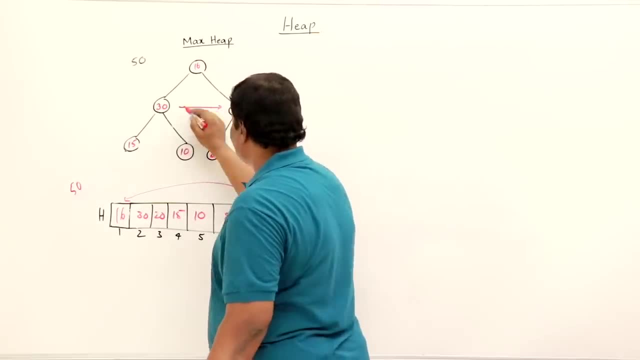 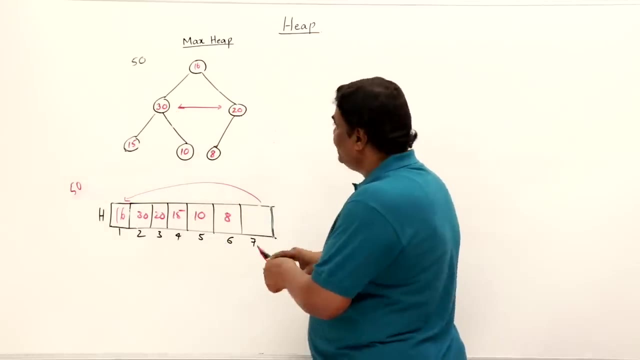 So let us check how to do this. Compare children of this 16, that is new root. Which child is greater? 30 is greater, So 30 will take its place. 16 will come into its place, So I will draw it here. 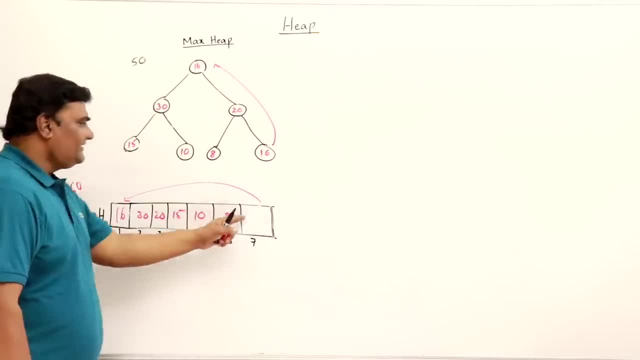 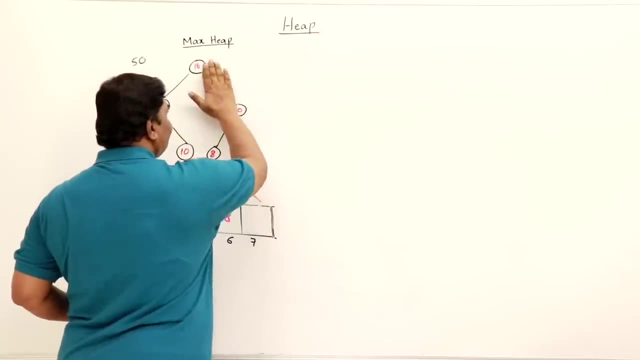 binary: last element. in complete binary means in an array, the last element will take its place. now this is how it looks like, so i'll remove this one now. okay, i'll remove this. this is gone. so you have already seen it. it's here now. now this is complete binary, but not 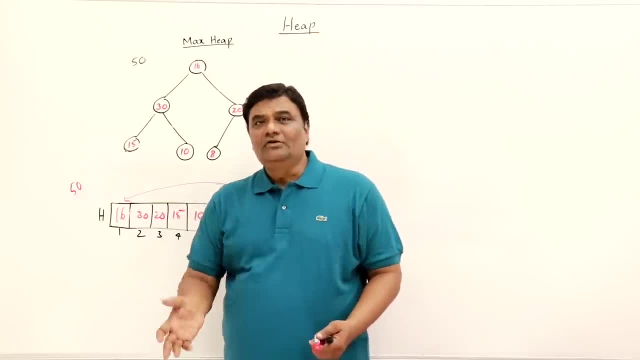 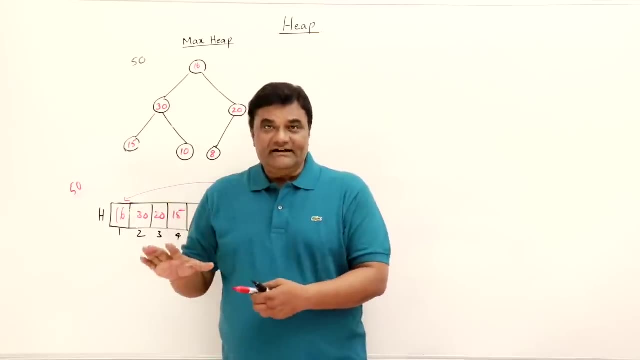 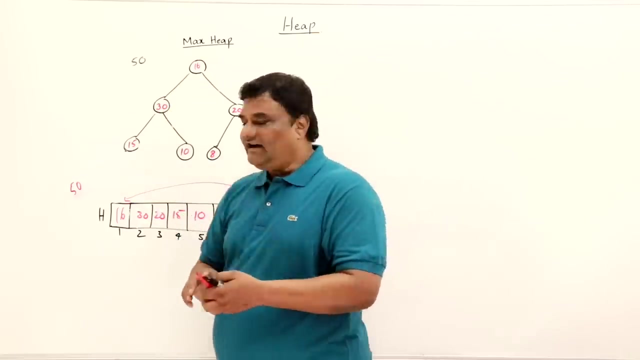 a max heap. so we have to adjust the elements. okay, we will adjust the element. that is not a big deal. maintaining complete binary property is very important, so we preserve that now. adjusting the element, so we will adjust how, from the root towards leaf, we will send it. so let us check how to. 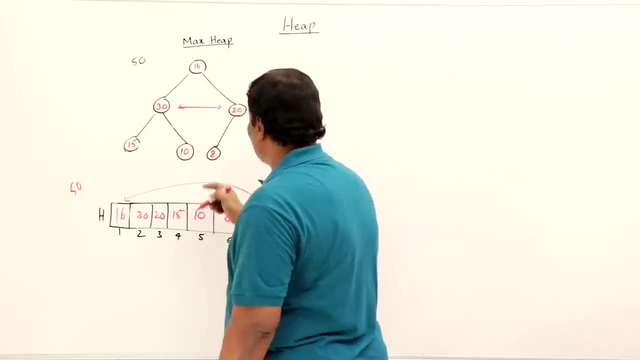 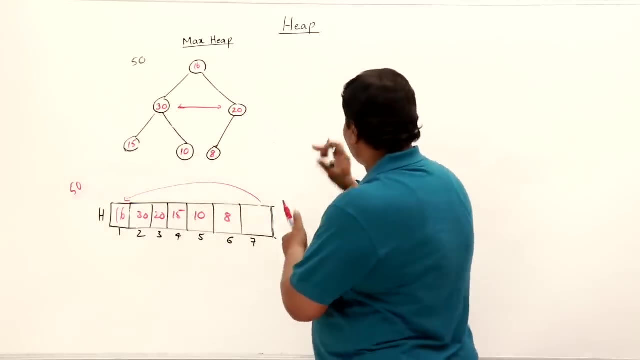 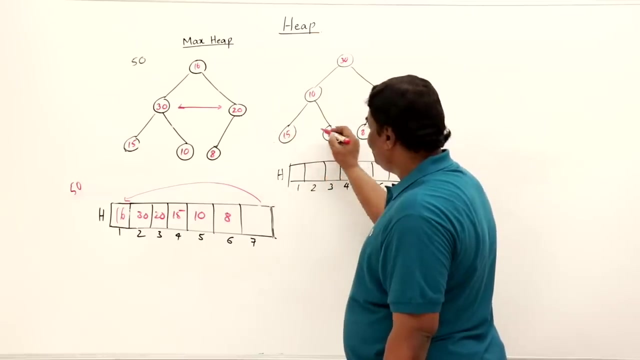 do this. compare children of this: 16, that is new root. which child is greater? 30 is greater, so 30 will take its place. 16 will come into its place, so i will draw it here. so here 30 goes, here 20 and 8 remain, 16 comes here and 15 and 10 as it is, so i'll fill them in this. 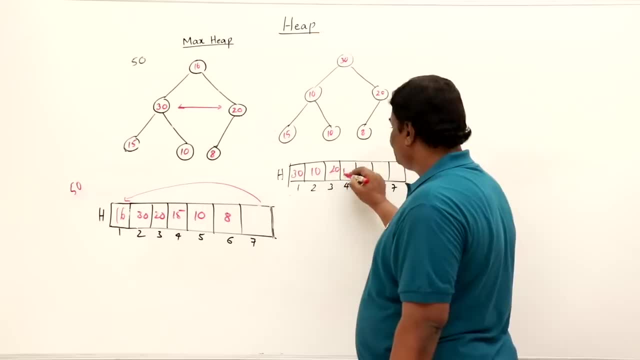 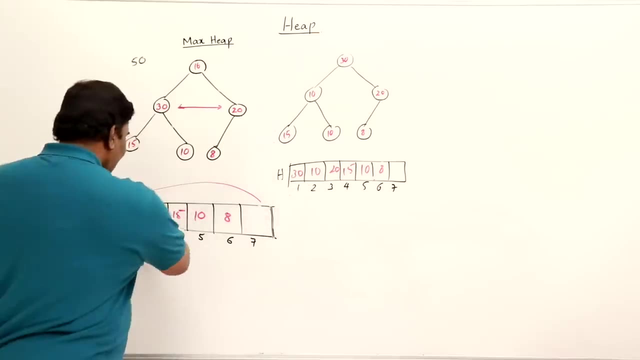 array. also, 30 is here, 10 and 20 and this is 15 and 10 and 8. this place is free. last place is free. so how we have done it is see this: 16 was compared with its children, who are children of 16, 2 and 3- left child and right child, left child and right child. 1 into. 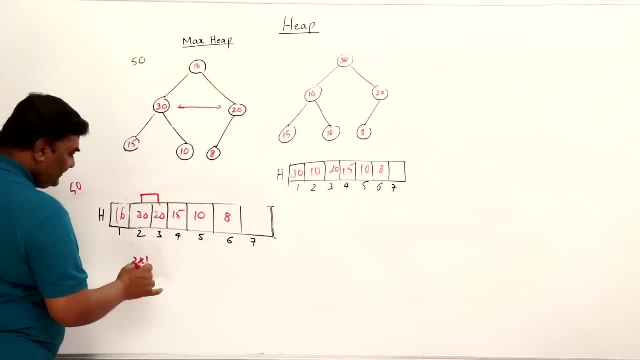 2, 1 into 2 plus 1, so 2 into 1 and 2 into 1 plus 1. so if you remember this formula, 2i, 2i plus 1, so this is 2 and this is 3. 2 and 3. these are children of 16. 2 and 3, this is: 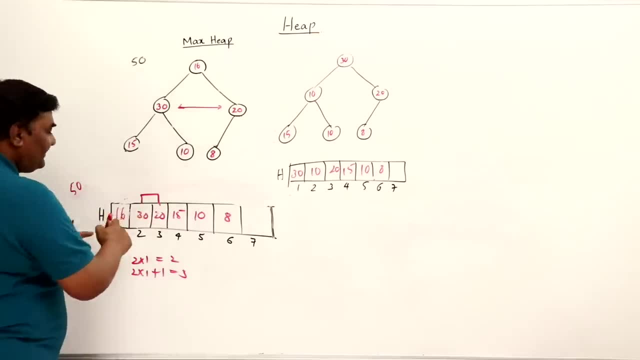 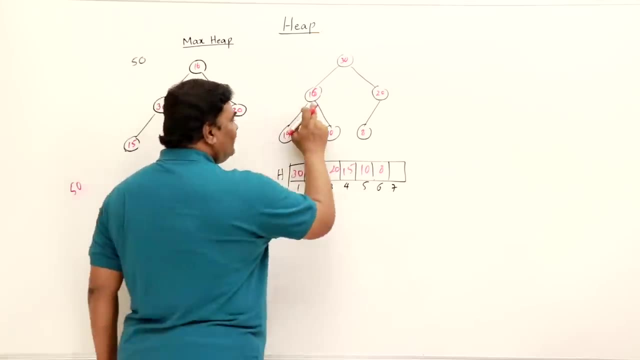 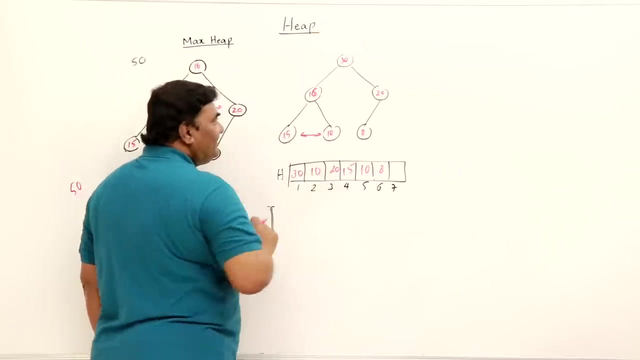 4, 3 and 1, and then gr 10 is 0. we compared and 30s brought here. so now this is 1 step we have completed. still we have to check with the descendants. so let us check with the descendants. 16, who are the children of 16, 15 and 10. compare them, which is greater? 15? now is this 15 greater? 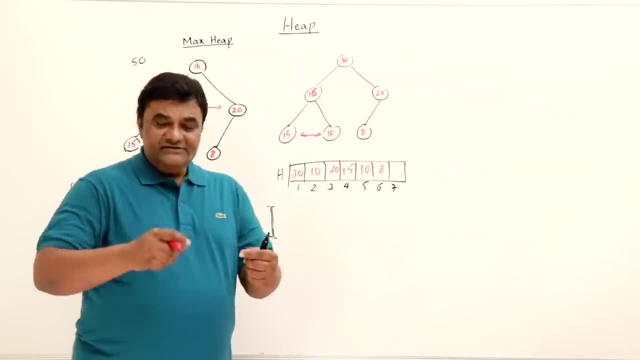 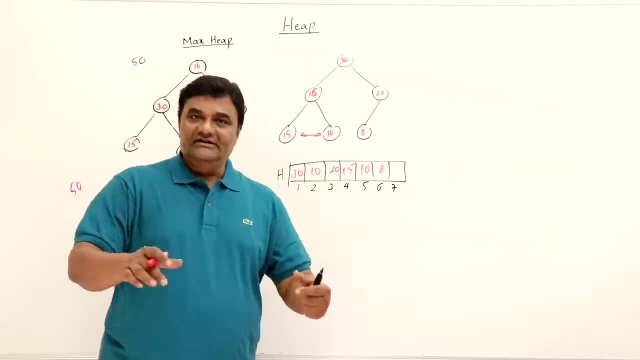 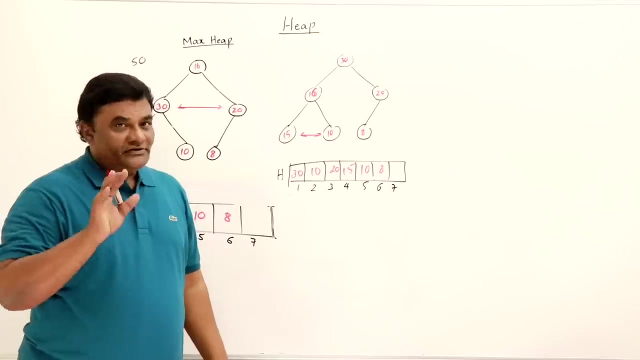 than 16. no, first of all compare the children and whichever child is greater that you compare with the parent. okay, afterwards you compare it now, but 16 is greater than both of them, so leave it, its already there, max heap. so this is a max heap. you don't have to swap them. so this is a delete. 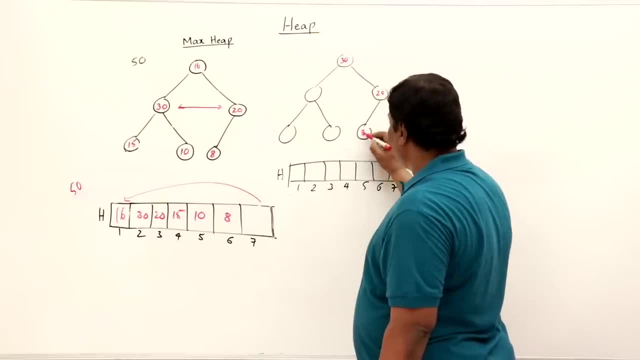 So here, 30 goes, here, 20 and 8 remain, 16 comes here and 15 and 10 as it is, So I'll fill them in this array also. 30 is here, 10 and 20.. And this is 15 and 10 and 8.. 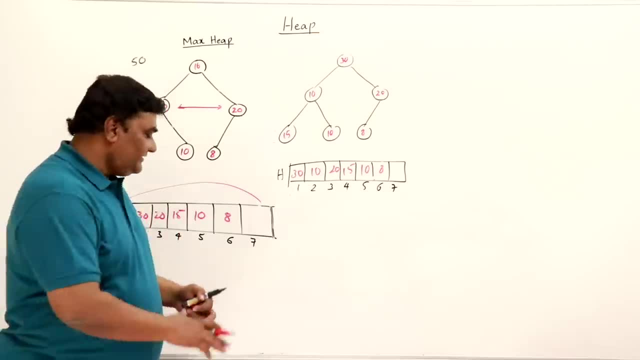 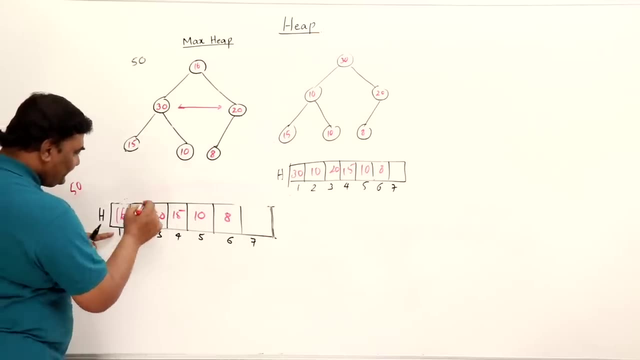 This place is free. Last place is free. So how we have done it is see the 16 was compared with its children, Who are children of 16? 2 and 3.. Left child and right child. left child and right child. 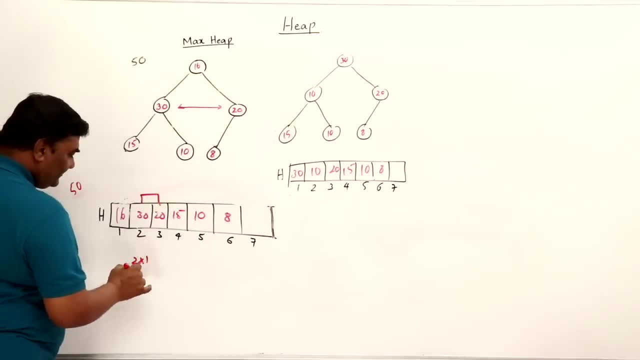 1 into 2, 1 into 2 plus 1.. So 2 into 1 and 2 into 1 plus 1.. So if you remember this formula, 2i, 2i plus 1.. So this is 2 and this is 3.. 2 and 3.. 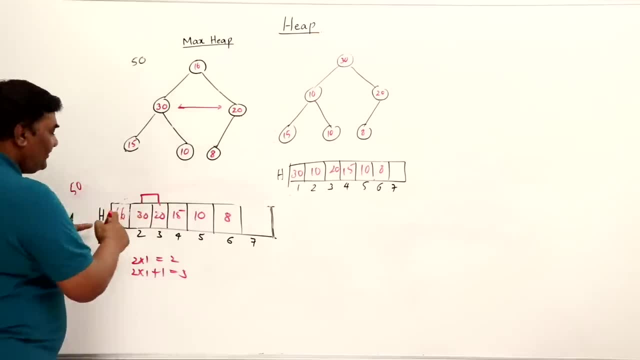 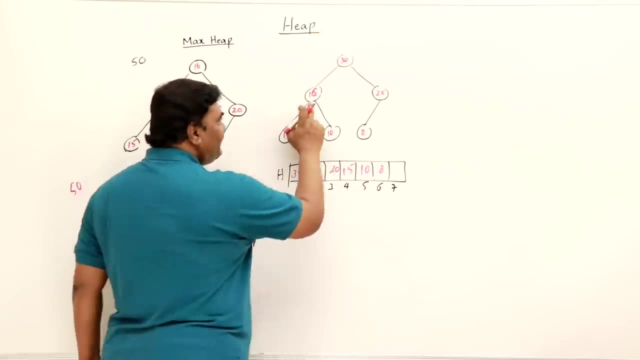 These are 20 and 30 are the children We compare, and 30 is brought here. So now this is one step we have completed. Still we have to check with the descendants. So let us check with the descendants 16.. Who are the children of 16?? 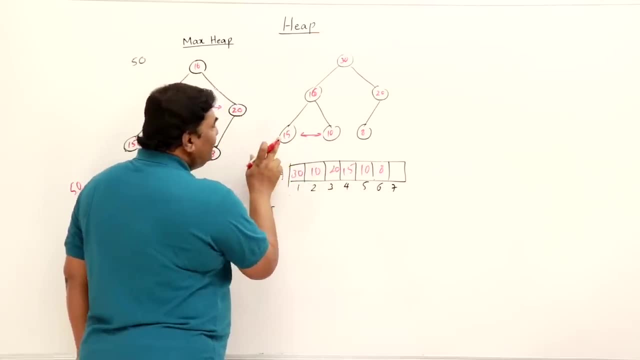 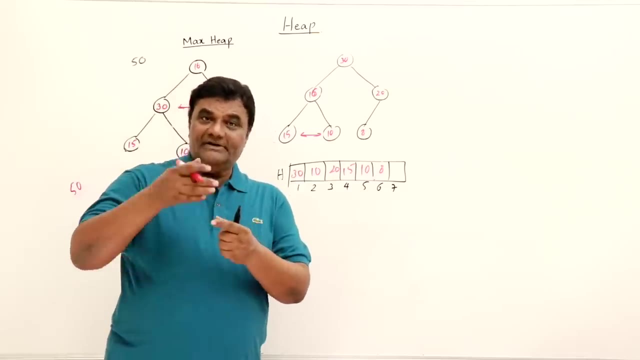 15 and 10. Compare them. Which is greater, 15. Now, is this 15 greater than 16? No, First of all, compare the children and whichever child is greater that you compare with the parent. OK, afterwards you compare it. 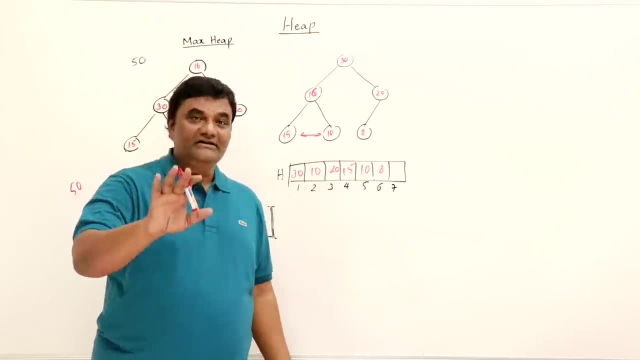 But 16 is greater than both of them, So leave it. It's already there in max heap, So this is in max heap. You don't have to swap them. So this is a DELETE procedure. So I'll just repeat the steps quickly. 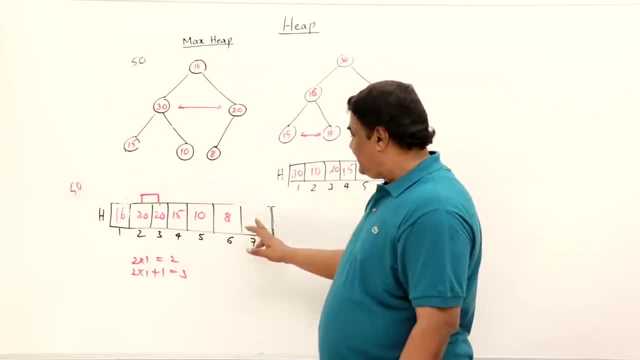 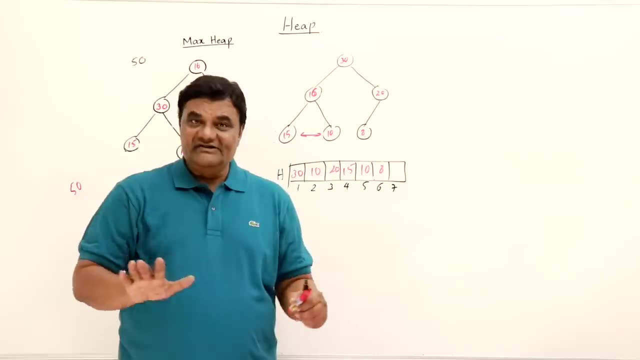 See: always in DELETE we remove root and the last element in COMPLETE BY ENTER will take the place and we push the element downwards towards leave and adjust the elements to form a max heap. So we have adjusted downwards Right, So from root towards leaf. 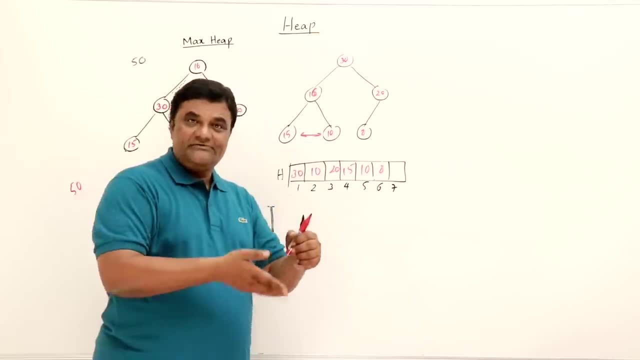 If you remember, in INSERT the adjustment was done from leaf towards root, But now the adjustment is done from root towards leaf. So in DELETION adjustment is done, but the direction is different. So in both INSERT and DELETE adjustment is done, but the directions are different. 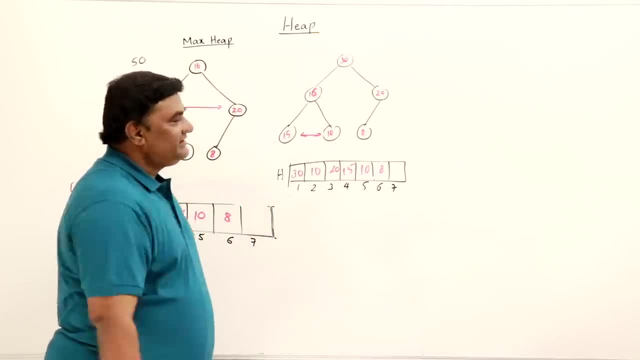 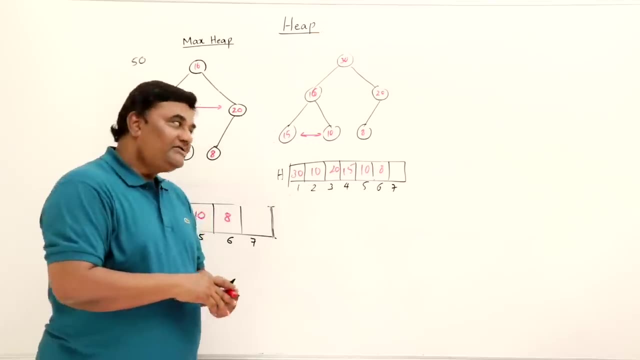 Now a little bit of analysis. How much time it has taken for deleting one element? It depends on the height. So what is the maximum adjustment you have to do? That depends on the height. So the maximum time is log n, Log n- Yes. 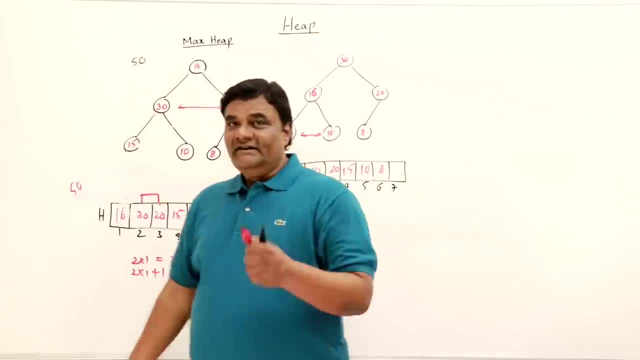 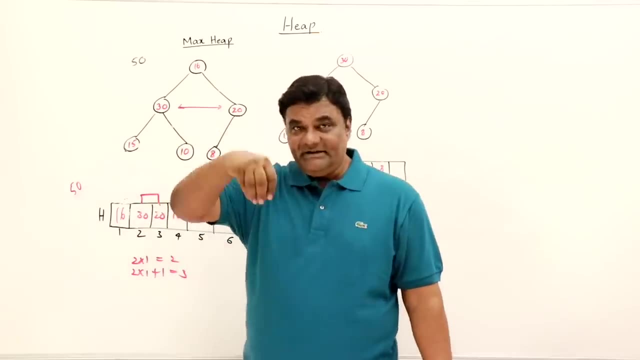 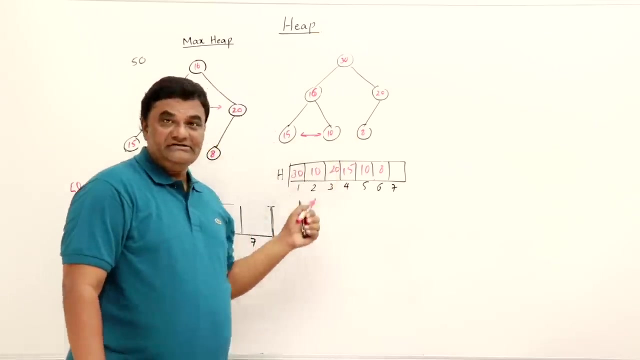 procedure. so I'll just repeat the steps quickly. see, always in delete we remove root and the last element in complete binary will take the place and we push the element downwards towards leaf and adjust the elements to form a max heap. so we have adjusted downwards right. so from root towards leaf, if you remember. 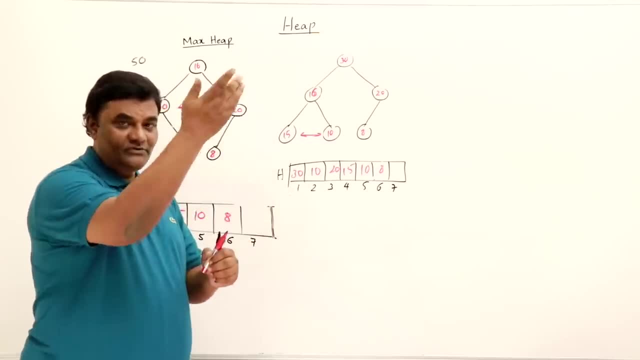 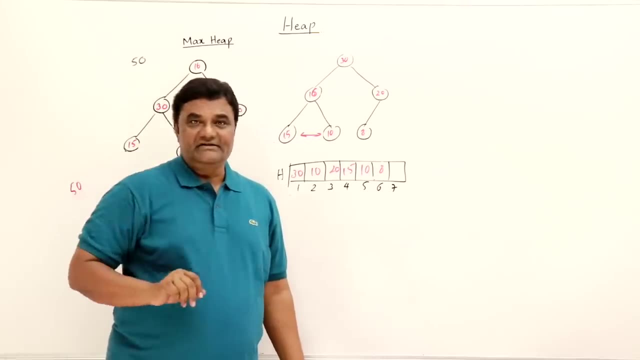 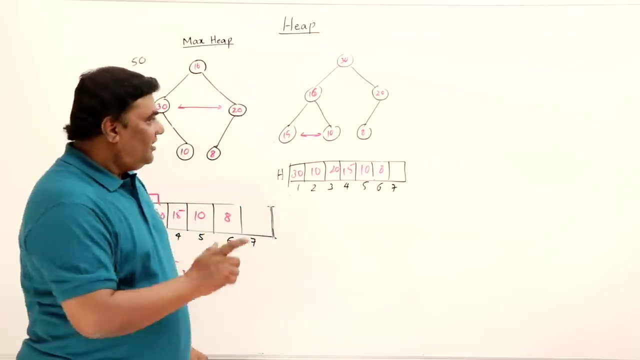 in insert the adjustment was done from leaf towards root, but now the adjustment is done from root towards leaf. so in deletion adjustment is done, but the direction is different. so in both insert and delete adjustment is done, but the directions are different. now little bit of analysis. how much time? 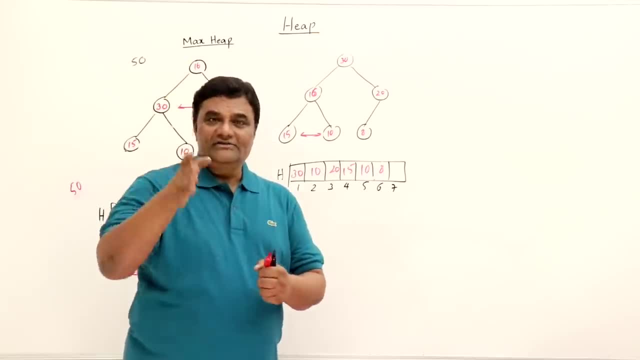 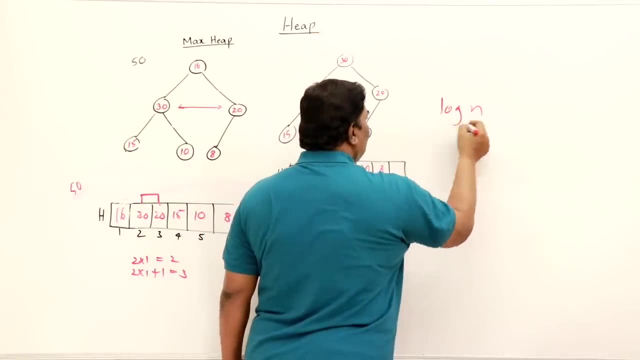 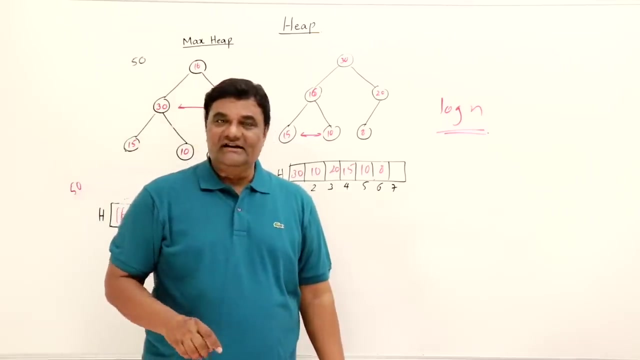 it has taken for deleting one element. it depends on the height. so what is the maximum adjustment you have to do? that depends on the height. so the maximum time is log n. yes, so deletion takes log n time. now one important thing we understood here is that from the max heap, whenever you delete, you get the largest element from. 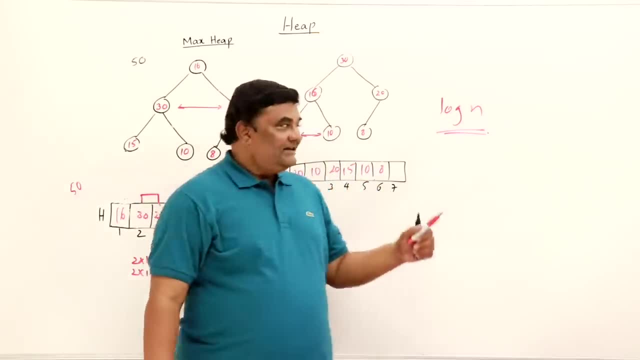 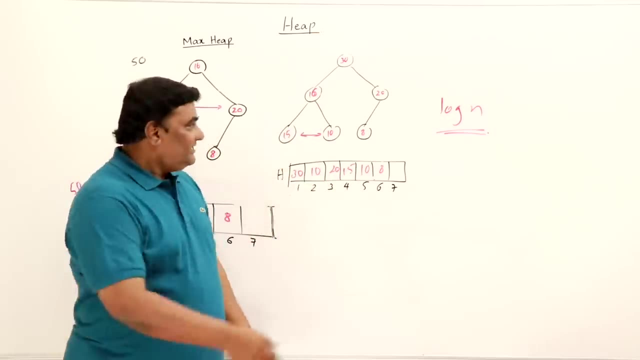 the heap. 50 was largest, 50 was gone. but now who is largest? next largest element is 30. if you delete, which will be deleted, 30, then from the remaining 20, who will come and sit in the root? 20 will come and sit in the root. so if you 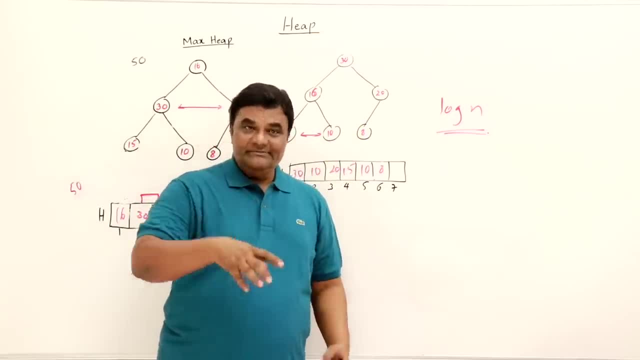 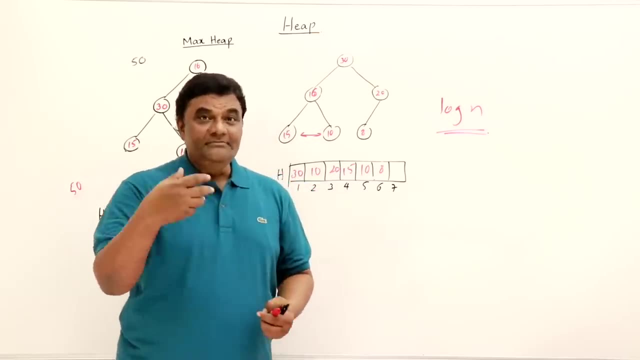 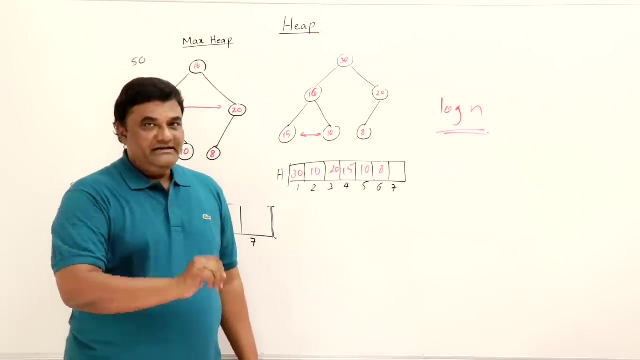 delete, next 20 will be deleted. yes, so from max heap, whenever you delete, you get the next largest element. from min heap, whenever you delete, you get the next minimum element. so you get the smallest, then next smallest, the next smallest, and so on. now, last important thing. this is very important, listen. 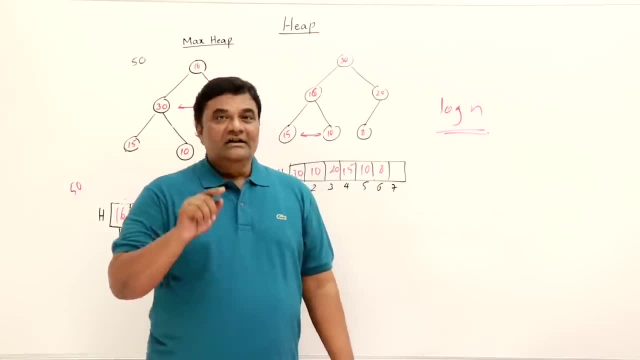 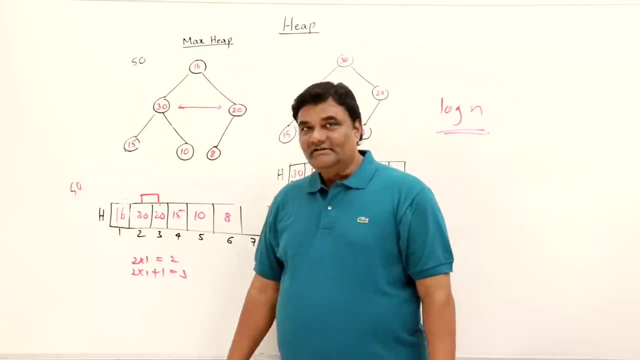 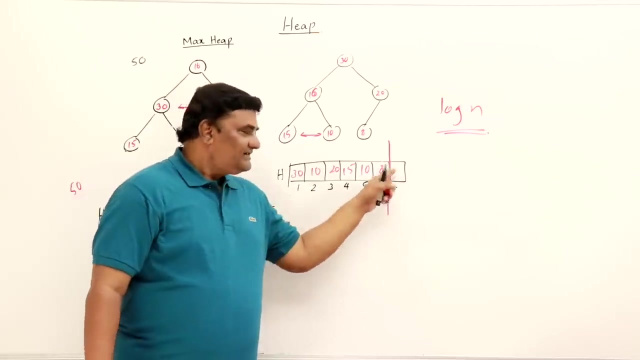 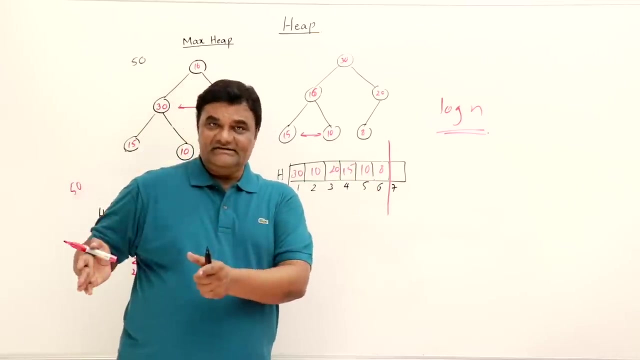 carefully. right, see, this is important here. the array size was 7. one element is deleted. now what is the heap size? 6 heap is still 6, only from 1 to 6. 7th place in an array is free. that is not a part of heap. yes, leave it, no problem, our heap is still 6, only that space is. 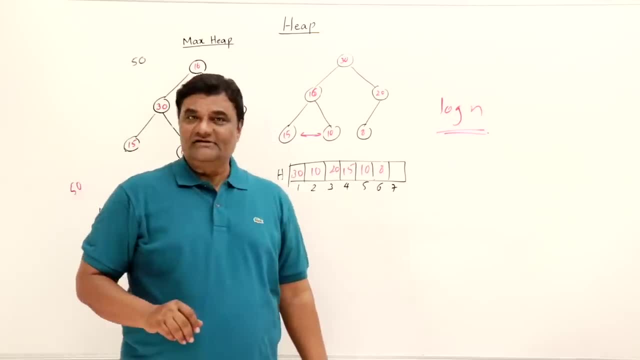 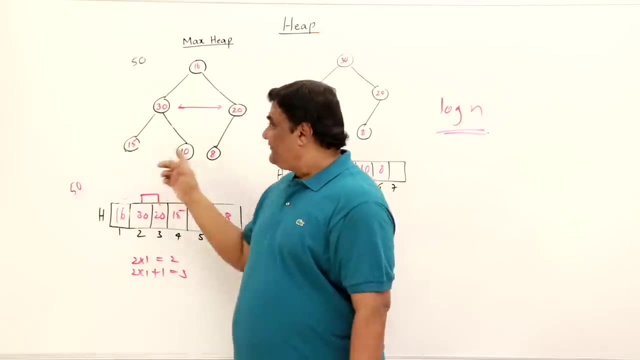 So deletion takes log n time. Now, one important thing we understood here is that from the max heap, whenever you delete, you get the largest element from the heap. 50 was largest, 50 was gone. But now who is largest? 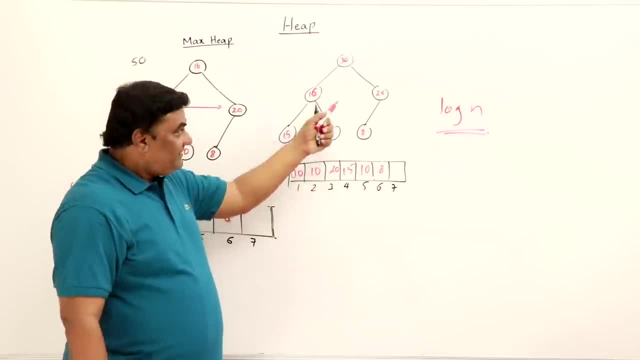 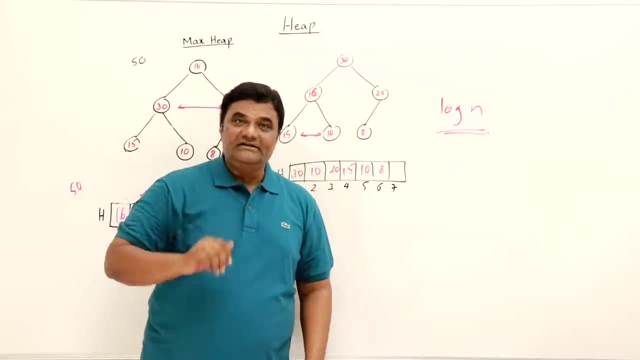 Next largest element is 30. If you delete, which will be deleted, 30. Then from the remaining 20, who will come and sit in the room? 20 will come and sit in the room. So if you delete, next 20 will be deleted. 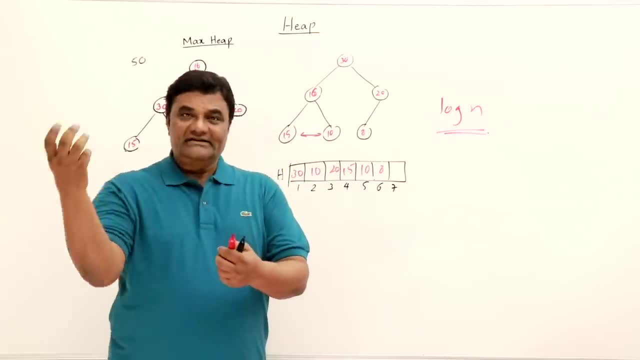 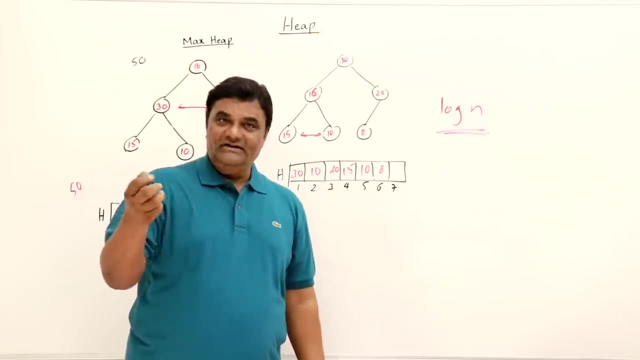 Yes, So from max heap, whenever you delete, you get the next largest element. From min heap, whenever you delete, you get the next minimum element. So you get the smallest, the next smallest, the next smallest, and so on. Now, last important thing. 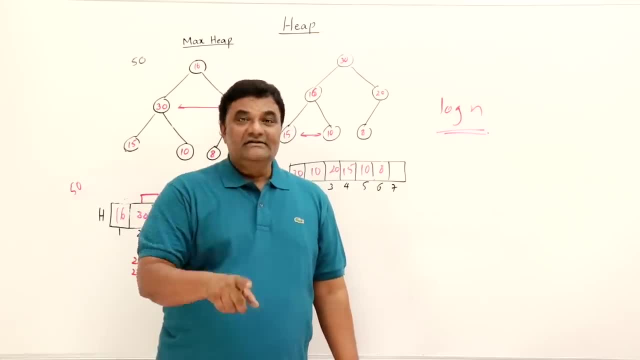 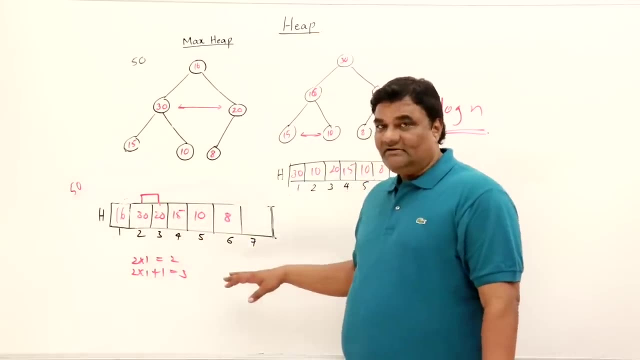 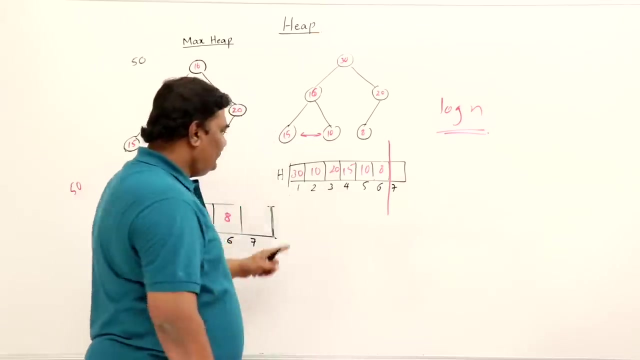 This is very important. Listen carefully Right, See, this is important Here. the array size was 7.. One element is deleted. Now what is the heap size? 6.. Heap is still 6, only from 1 to 6.. 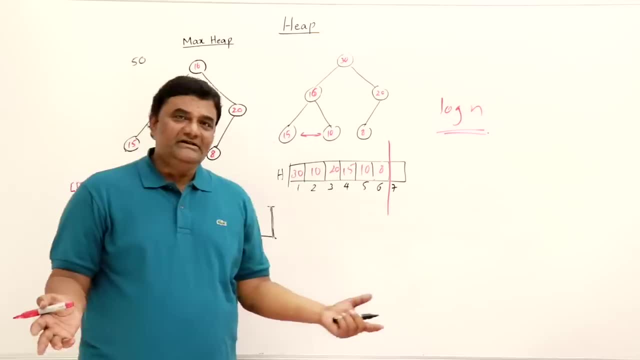 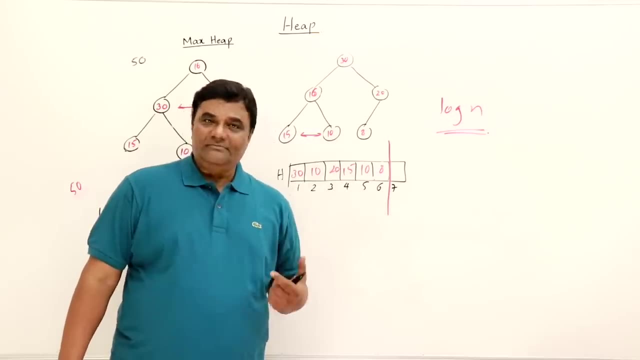 Seventh place in an array is free. That is not a part of heap. Yes, Leave it, No problem. Our heap is still 6, only That space is vacant after that. So it's not a problem for us. But what element we deleted? 50. Where it is. 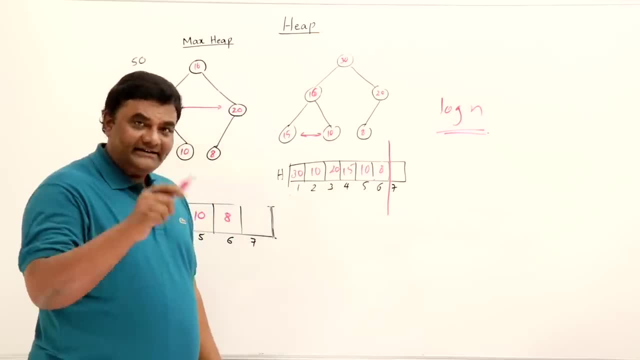 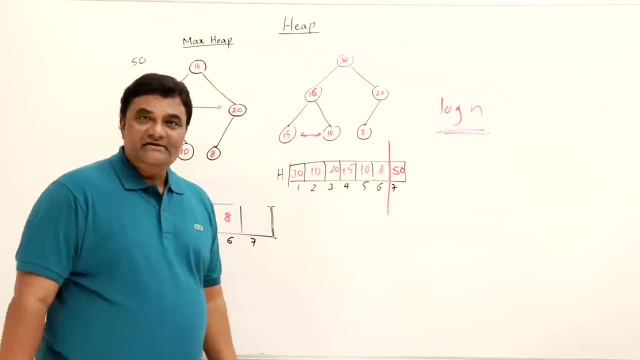 We are using it. But if you want to maintain that copy of 50, there is a free space here- You keep 50 here. This is interesting. I kept 50 there. Is it a part of heap? No, It's outside heap. Yes. 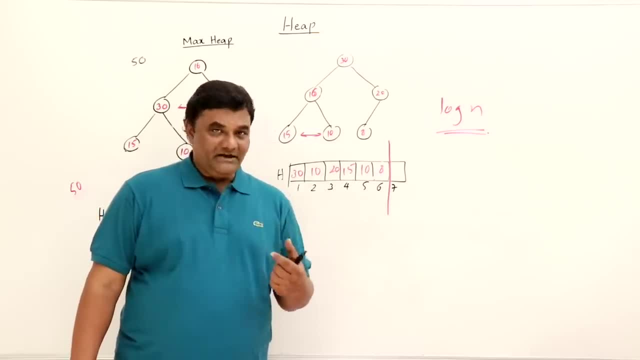 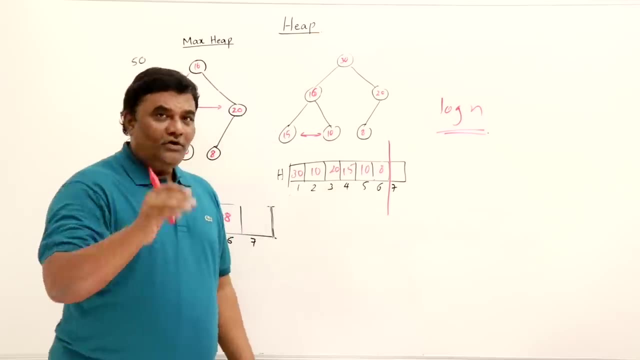 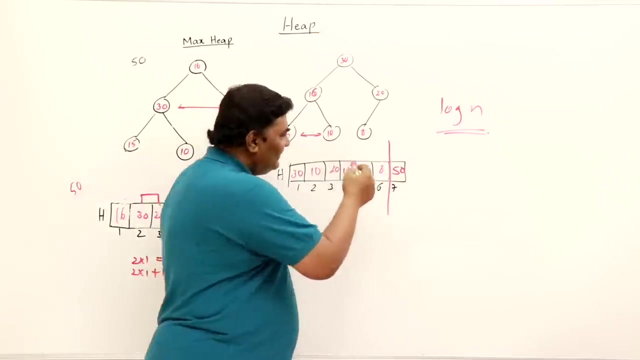 vacant after that. so it's not a problem for us. but what element we deleted? 50 where it is, we are using it. but if you want to maintain that copy of 50, there is a free space here. you keep 50 here. this is interesting, I kept 50 there. is it a part of heap? no, it's outside heap. 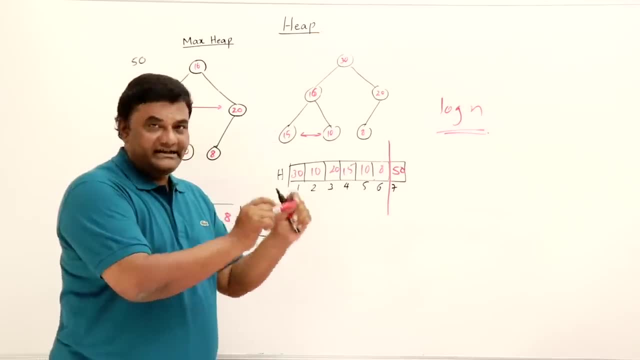 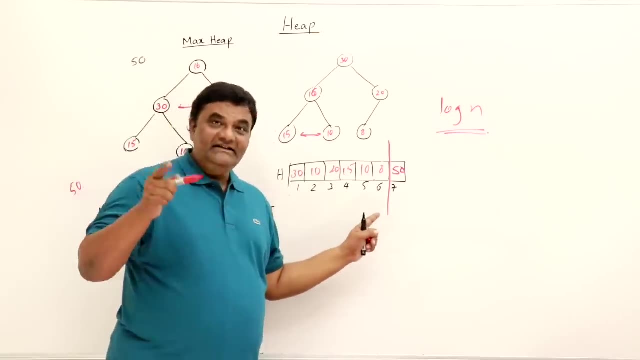 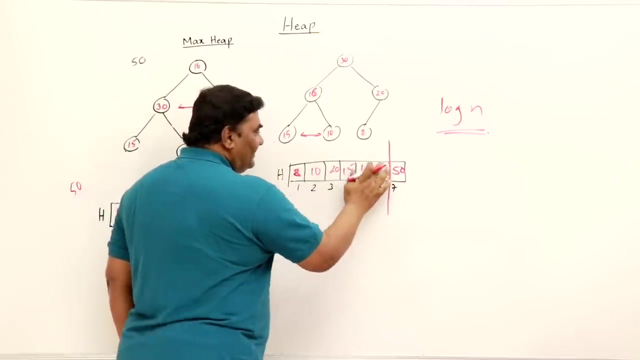 here, so it's not a part of it. just a space was free so I kept it there. that's all away from heap. right now. from the six elements- if I delete again, what will believe it? 30 will be deleted and 8 will come here. then we adjust so 20 comes. 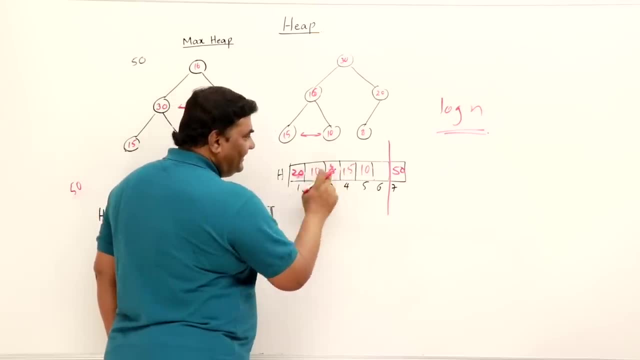 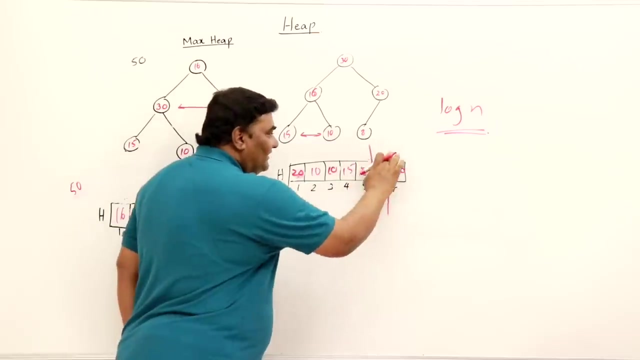 here and 8 goes here, then with it's a child, that is 10. so 10 comes here, 8 goes there. so now the heap reduces to this. so the heap size is 5, which element i deleted just now- 30. these two places are free already. 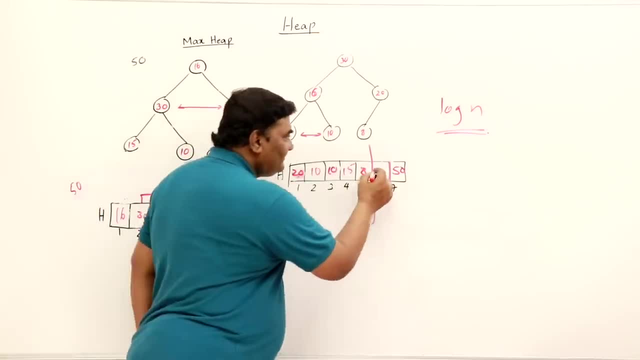 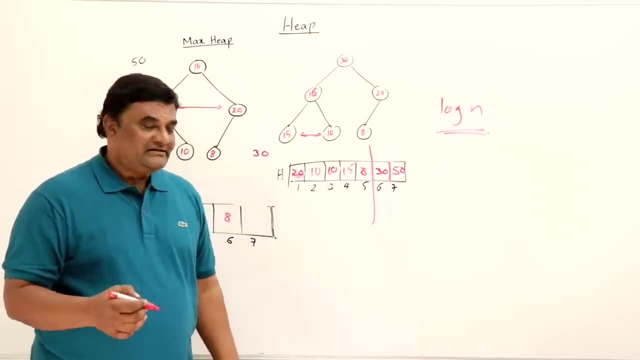 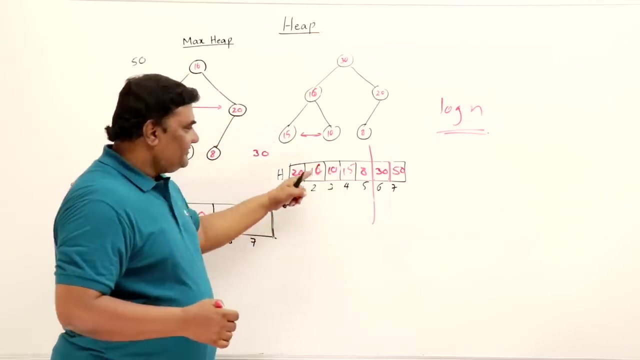 i kept 50 there, now 30. keep it here, next free place. if i do this, what happens? what happens? next element will be 20, next element will be 10, and so on. see, this was 16. i think yes, so it will be so on. so what happens? you, we are getting the elements largest, the next largest. 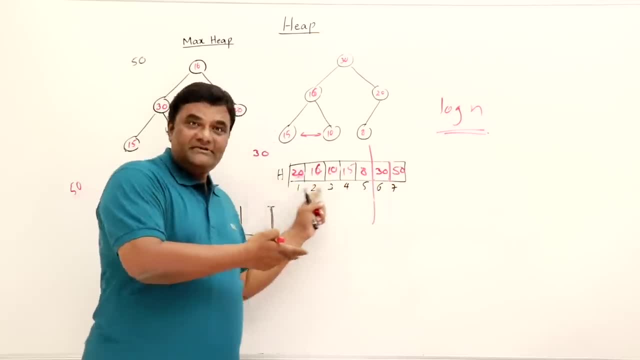 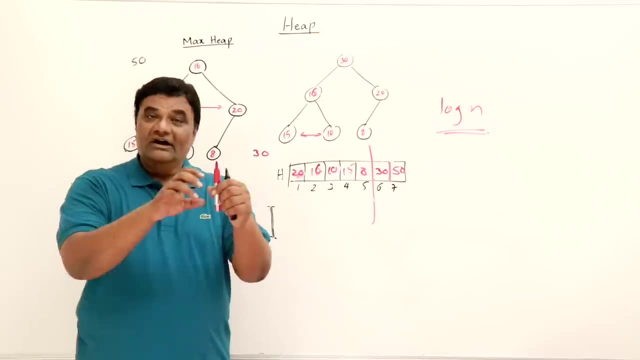 the next largest, the next largest, largest. so if you read the element from this side, they are sorted. they are sorted. yes, this is the idea of heap sort. if you have a heap, then delete the element and fill it in the empty place obtained after deletion. so if you go on filling the 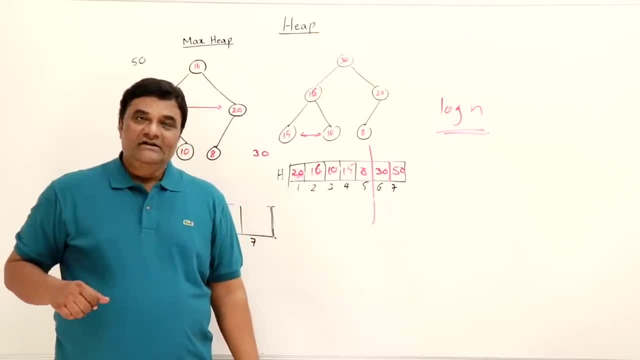 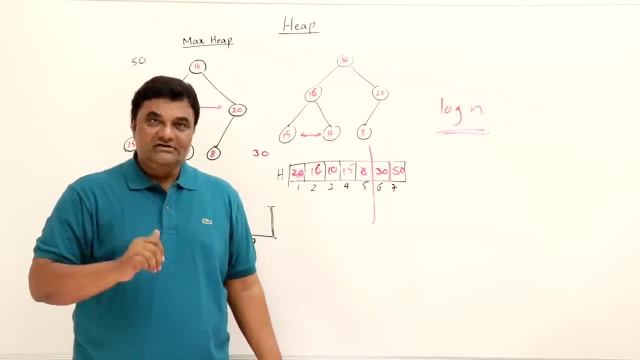 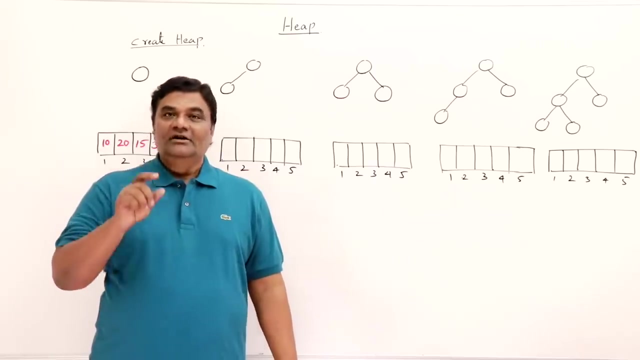 elements there then automatically gets sorted. so from the heap go on deleting the elements and start filling them in free spaces. so this is heap sort. so let us take few elements and see the complete heap sort right now. heap sort, heap sort have two steps. first is for 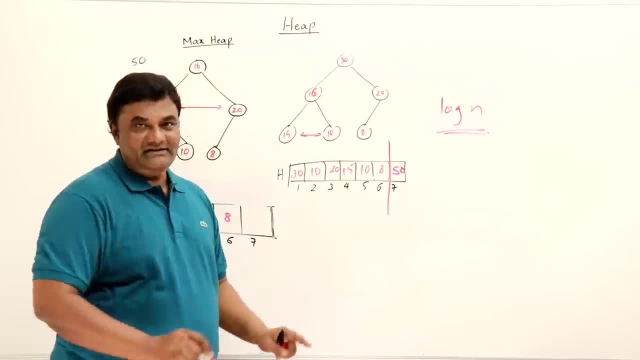 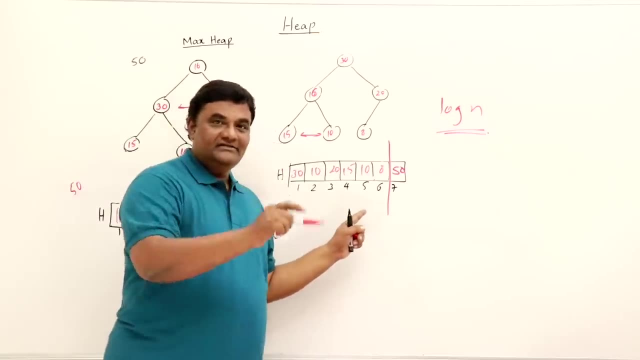 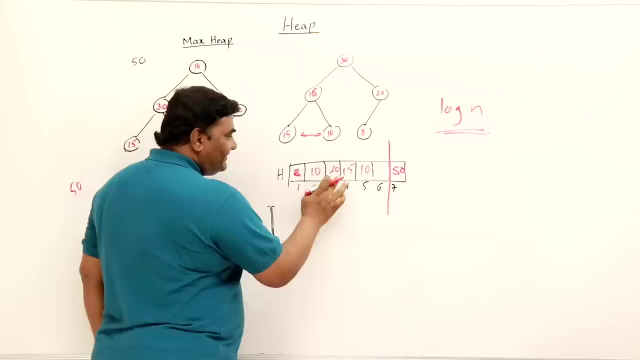 So it's not a part of heap, Just a space was free So I kept it there. That's all Away from heap Right Now. from the six elements, if I delete again, what will be deleted? 30 will be deleted and 8 will come here. Then we adjust. 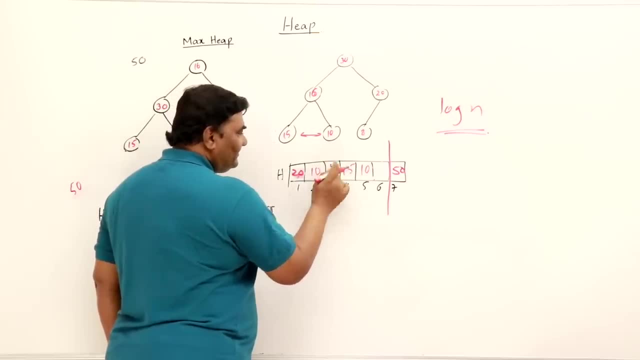 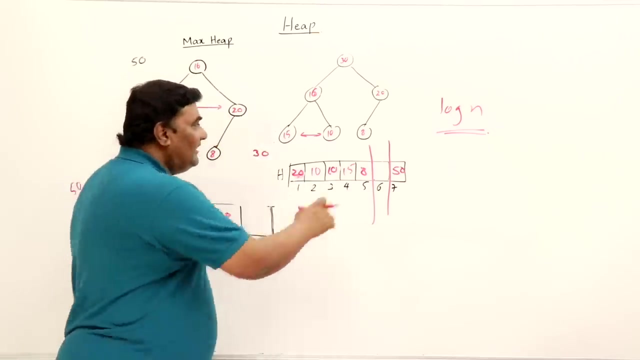 So 20 comes here and 8 goes here, Then 8 with it's a child, That is 10.. So 10 comes here, 8 goes there. So now the heap reduces to this. So the heap size is 5.. Which element I deleted just now? 30.. 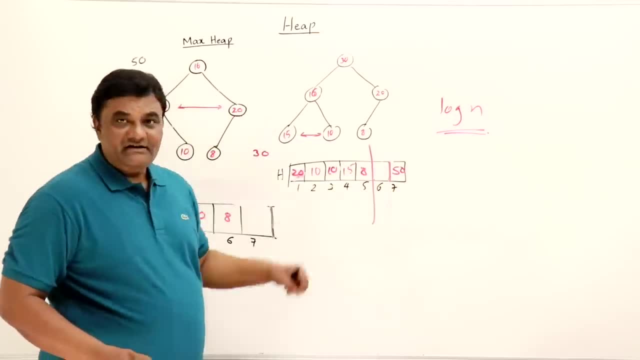 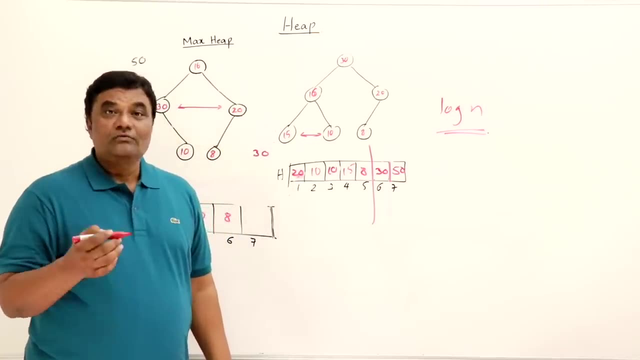 These two places are free Already. I kept 50 there, Now 30.. Keep it here Next free place. If I do this, what happens? What happens? Next element will be 20.. Next element will be 10, and so on. 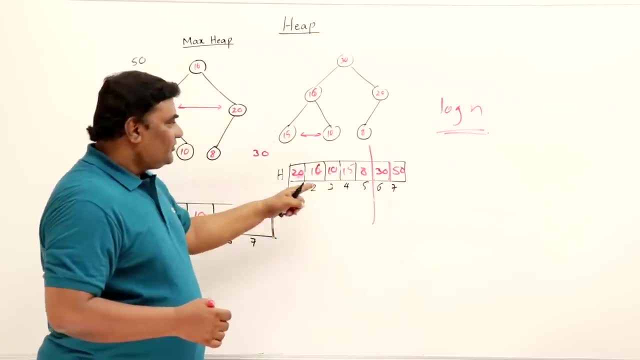 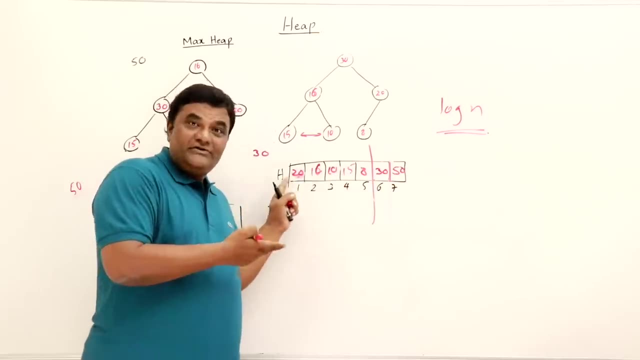 See, this is 16, I think is So. it will be so on. So what happens? We are getting the elements largest, the next largest, the next largest, the next largest. So if you read the elements from this side, they are sorted. 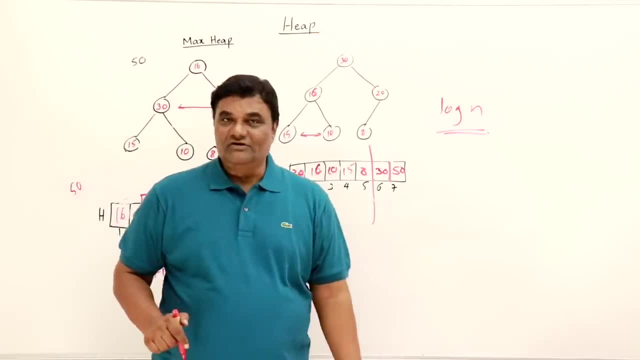 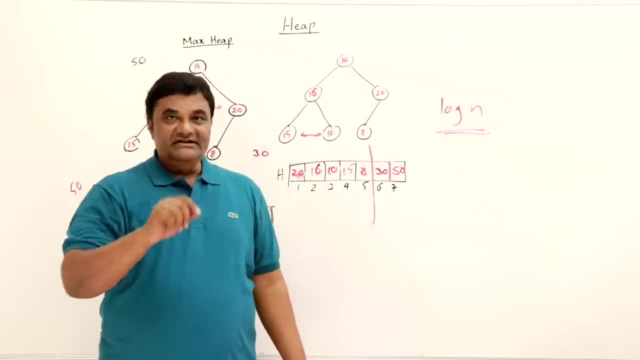 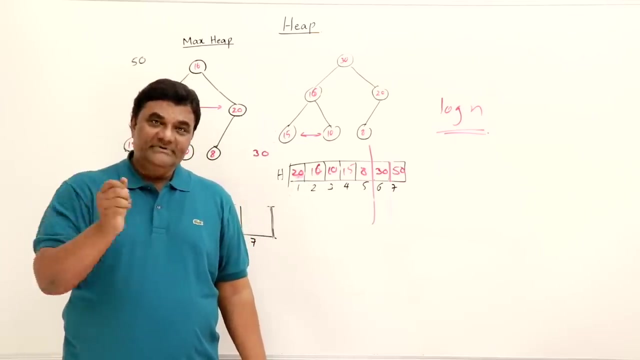 They are sorted. Yes, this is the idea of heap sort. If you have a heap, then delete the element and fill it in the empty place obtained after deletion. So if you go on filling the elements there, then automatically gets sorted. So, from the heap, go on deleting the elements and start filling them in free spaces. 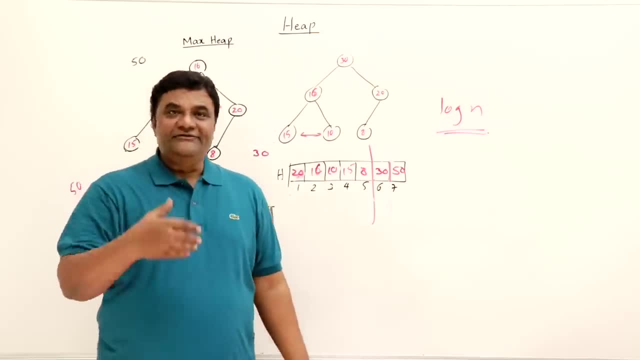 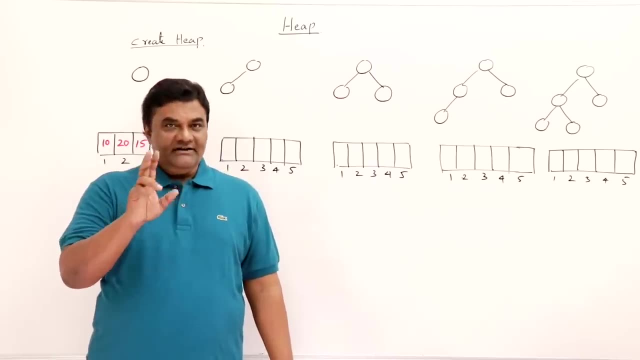 So this is heap sort. So let us take few elements and see the complete heap sort Right Now. heap sort. Heap sort have two steps. First is, for a given set of elements, create a heap by inserting all the elements one by one. 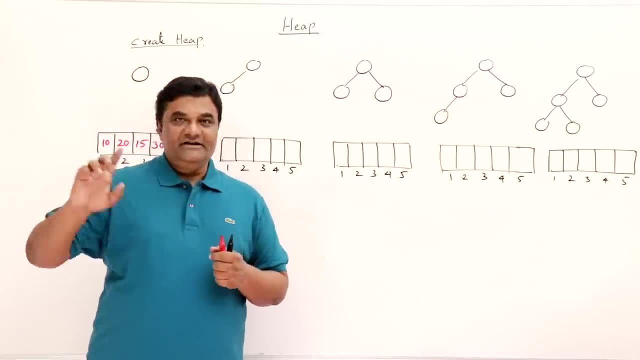 Then, once the heap is formed, delete all the elements from the heap, one by one. The elements will get sorted. So I repeat, the procedure of heap sort have two steps for a given set of number. First of all, create a heap, then delete all the elements from the heap. 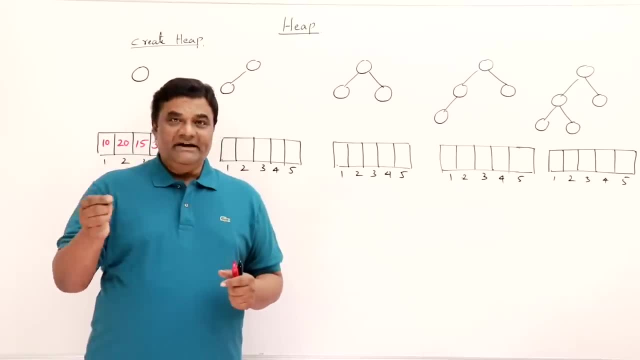 a given set of elements. create a heap by inserting all the elements one by one. then, once the heap is formed, delete all the elements from the heap one by one. the elements will get sorted. so i repeat the procedure of heap sort. have two steps for a given set of number. first of all, create. 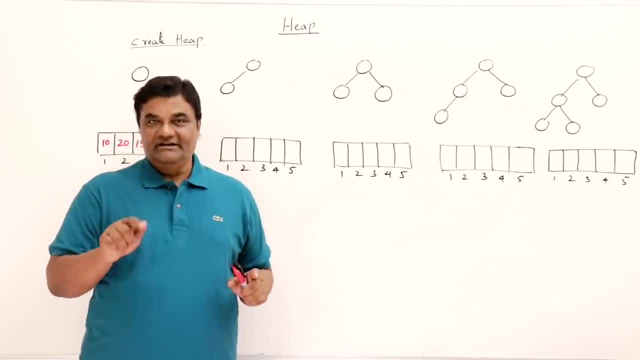 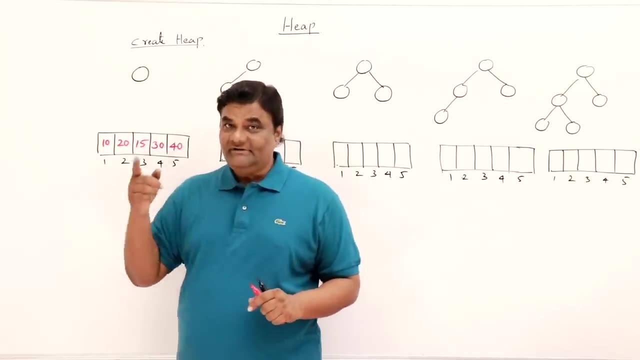 a heap, then delete all the elements from the heap. first step: create a heap. second step: delete all the elements from a heap. so i already have some set of elements here in an array. these are the elements. we have to sort them. so i will first show you how to create a heap. 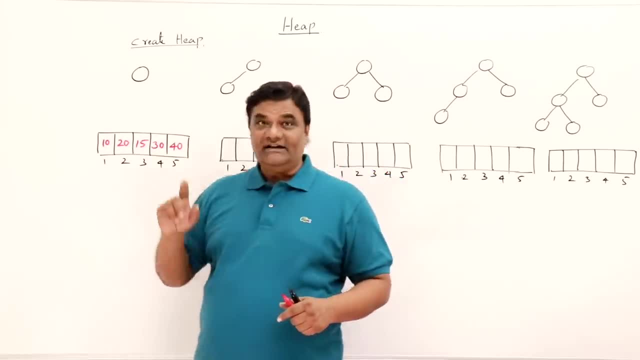 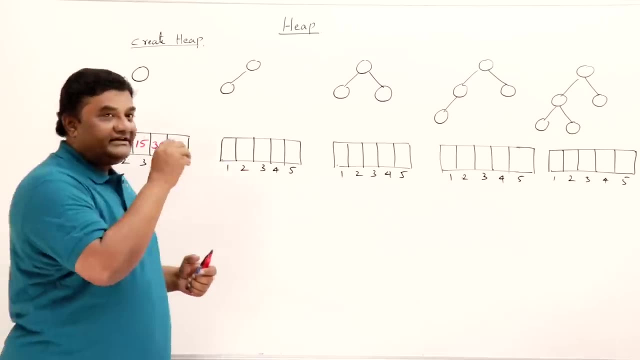 how the heap will be created inside the array. i am also going to show you diagrammatically. let us start. suppose these are the set of elements that we have to sort. they are not sorted, so first of all create a heap. so for that initial array, these elements are initial. 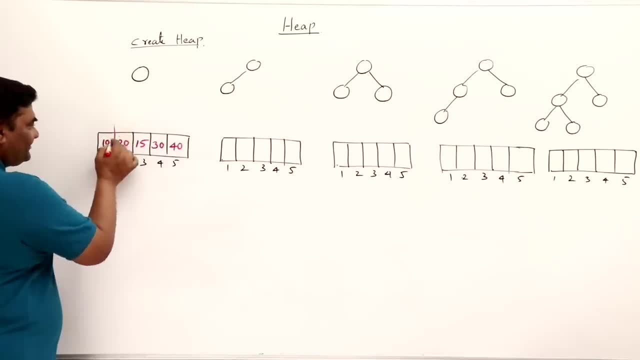 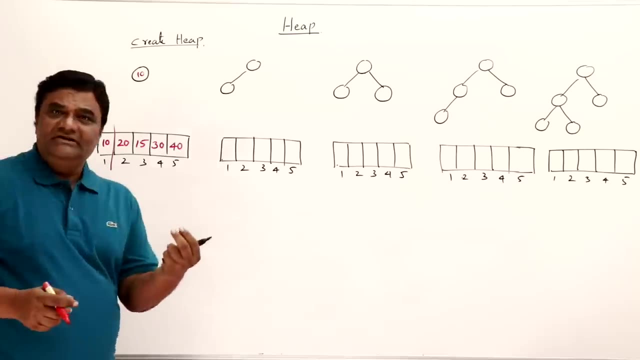 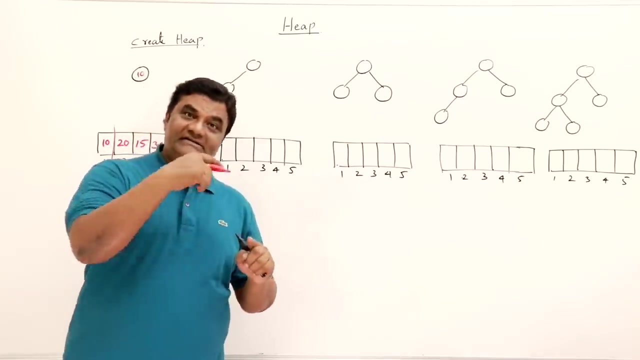 array. so we assume that in this first element is already in a heap. so this is 10. so right now there is only one element in the heap. so when you have only one element you can call it as max heap, also min heap also it is a heap, definitely it is a heap. now we will insert. 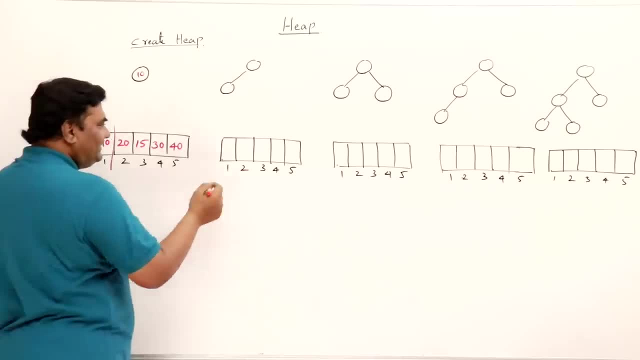 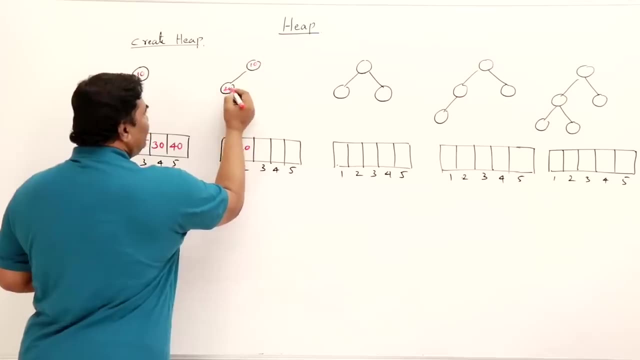 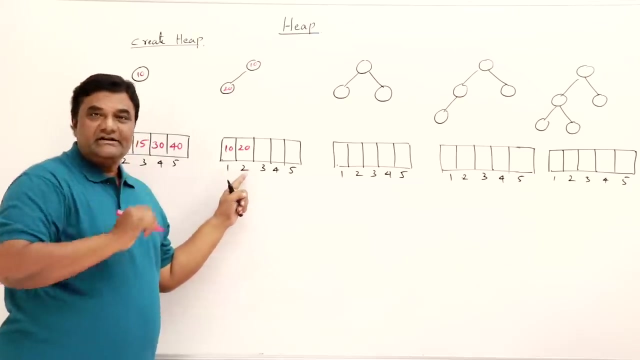 second element we will insert, that is, 10, is already in the heap. now we will be inserting 20. so 10 is already there, so 20. we will insert. so 10 here, 20 here. so rest of the elements. i am not writing them. okay, i will be writing one by one now inserting 20. how to insert already i have 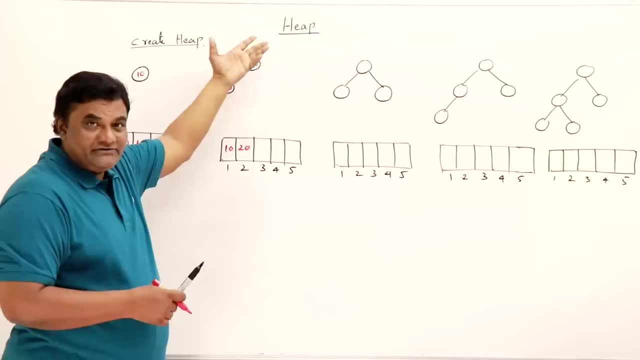 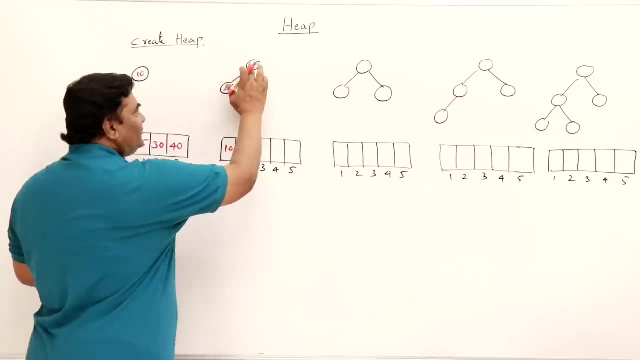 shown you. compare with the ancestor, that is, parent and its parent and so on, and try to adjust the element. check 20 with 10, right, so this is greater. so 20 should go up and 10 should come down. so here in an array, 2 is the index of 20, 2 by 2 is one. compare with: 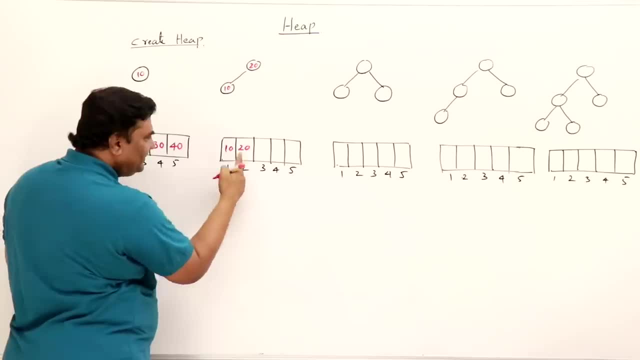 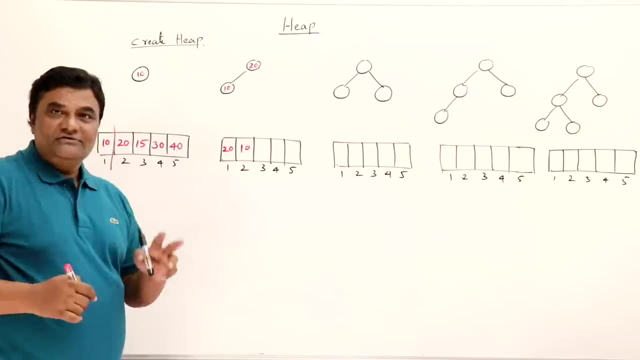 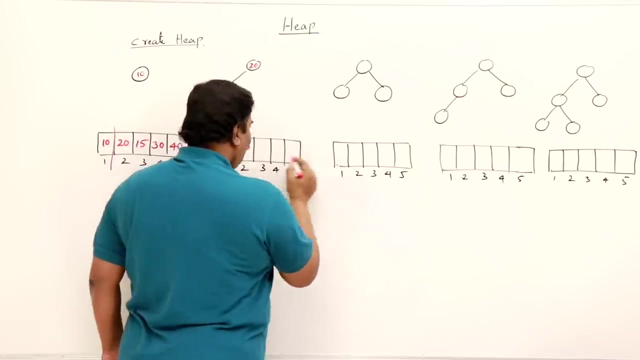 the parent: 1. so yes, 20 will come here, 10 will go there. right now this is heap, so we have a heap of two elements. there is a heap of two elements. now, third element we will include. so right now we have 20 and 10. now the new element is the next free space, so next free. 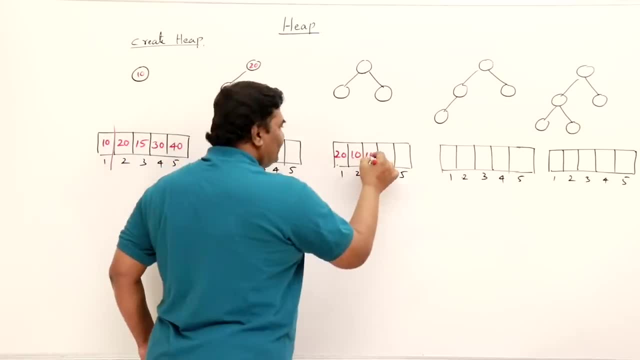 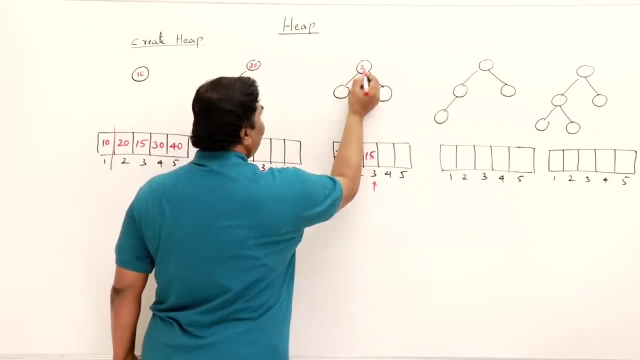 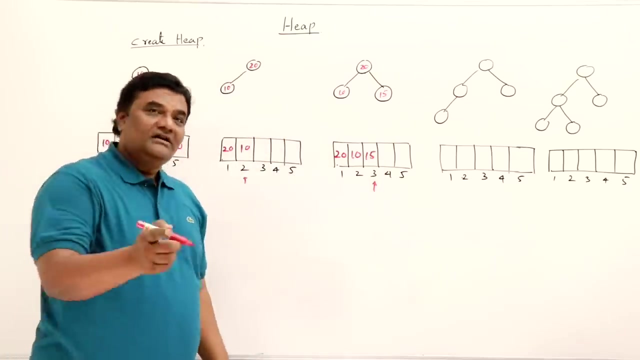 space. is this one? yes, so the element is 15, so we are going to insert. so we have 20, 10, 15, now this one. earlier we have inserted the element from here. right now 15 we are inserting. so right now we have 20 and 10 here. so 15 is in inserted here. now try to adjust it. how compare? 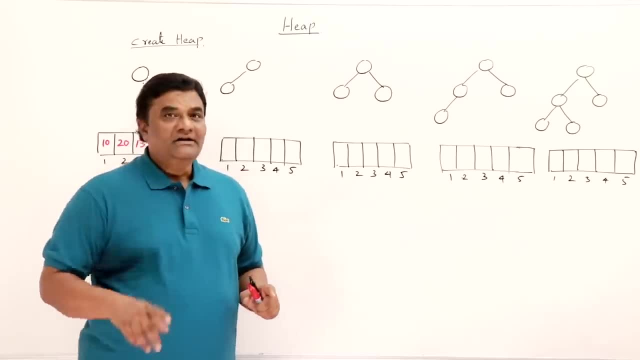 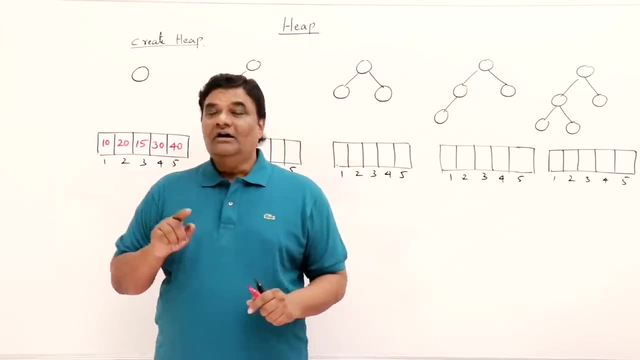 First step: create a heap. Second step: delete all the elements from a heap. So I already have some set of elements here in an array. These are the elements. We have to sort them. So I will first show you how to create a heap. 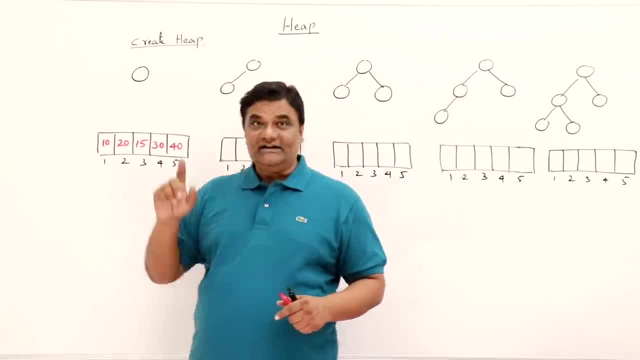 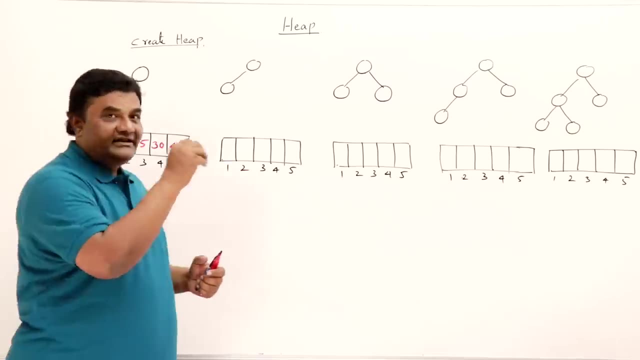 How the heap will be created inside the array. I am also going to show you diagrammatically. So let us start. Suppose these are the set of elements that we have to sort. They are not sorted, So first of all, create a heap. 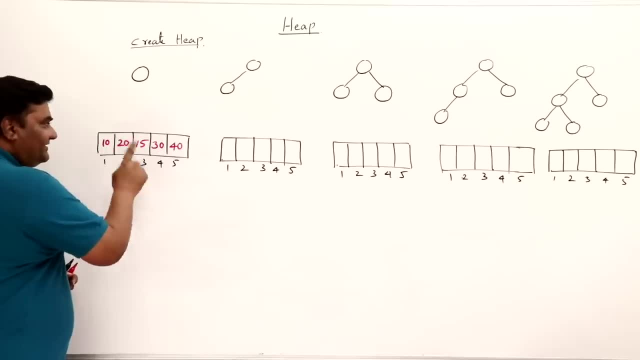 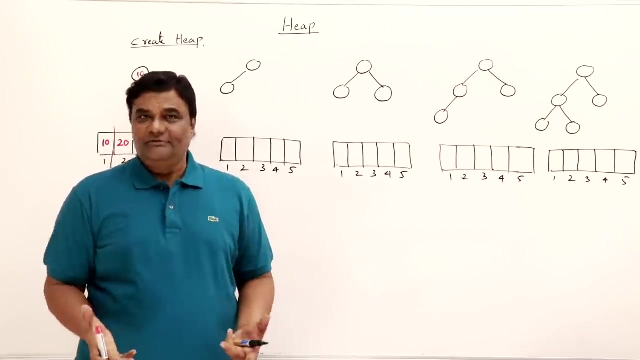 So for that initial array these elements are initial array. So we assume that in this first element is already in a heap, So this is 10.. So right now there is only one element in a heap. So when you have only one element, you can call it as max heap also, min heap also. 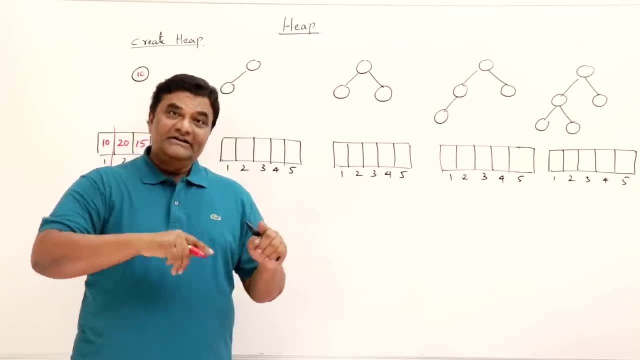 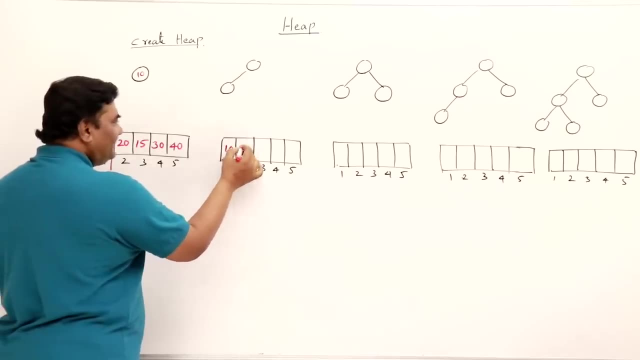 It's a heap. Definitely it's a heap. Now we will insert the second element. So second element we will insert. That is 10 is already in the heap, Now we'll be inserting 20. So 10 is already there. 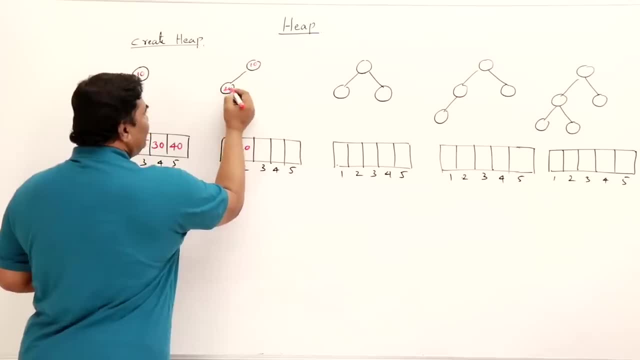 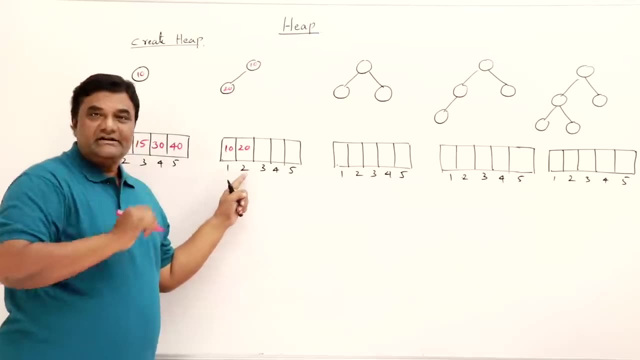 So 20. we will insert. So 10 here, 20 here. So the rest of the elements, I am not writing them. OK, I'll be writing one by one Now inserting 20.. How to insert Already I have shown you. compare with the ancestor, that is parent. 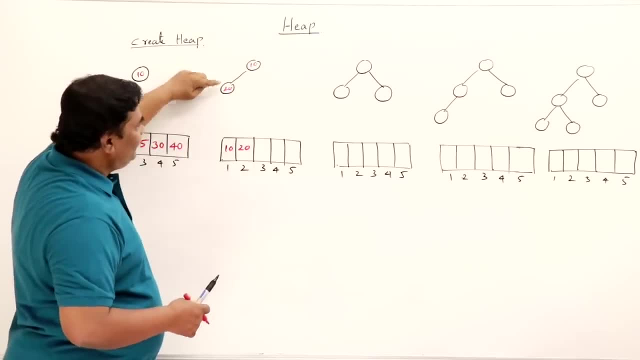 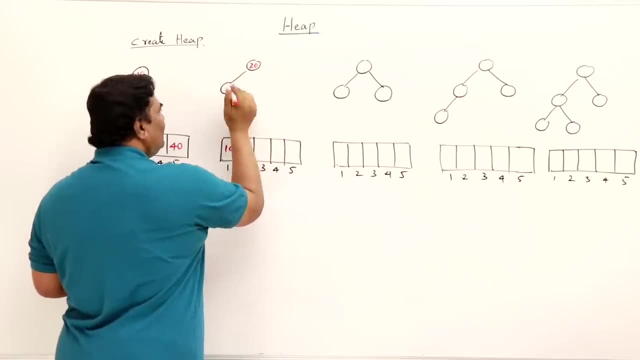 and its parent and so on, and try to adjust the element Check 20 with 10, right, So this is greater. So 20 should go up and 10 should come down. 20 should go up and 10 should come down. 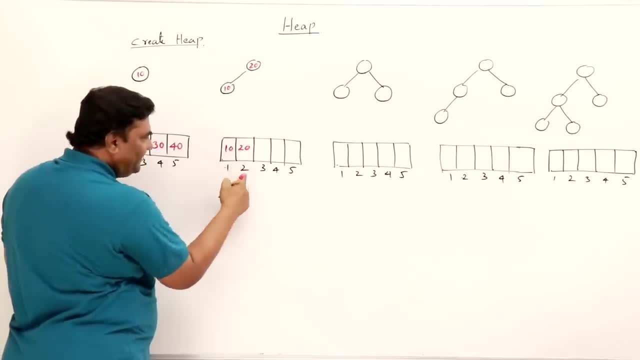 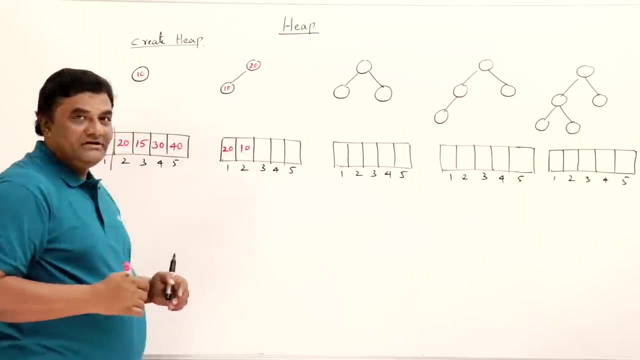 So here in an array, 2 is the index of 20.. 2 by 2 is 1, compared with the parent, 1.. So, yes, 20 will come here, 10 will go there right Now. this is heap. 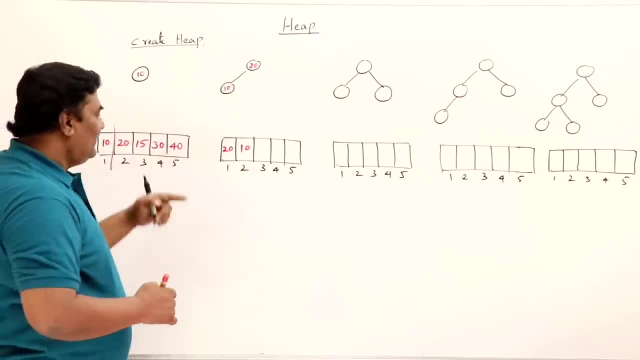 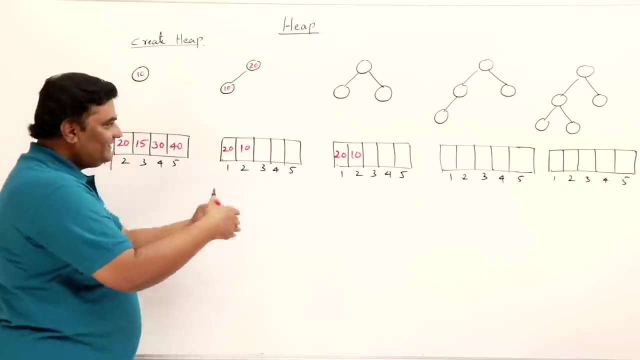 So we have a heap of two elements. There's a heap of two elements. Now, third element we will include. So right now we have 20 and 10.. Now the new element is the next free space. So next free space is this one. 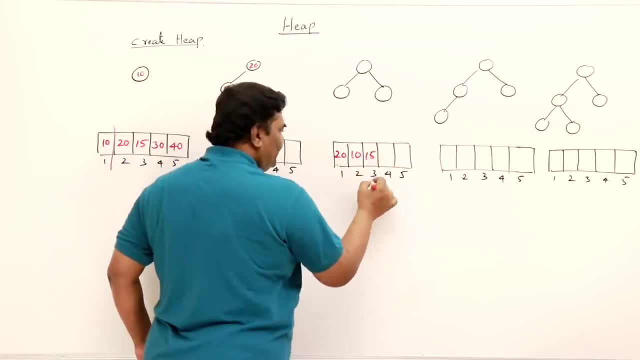 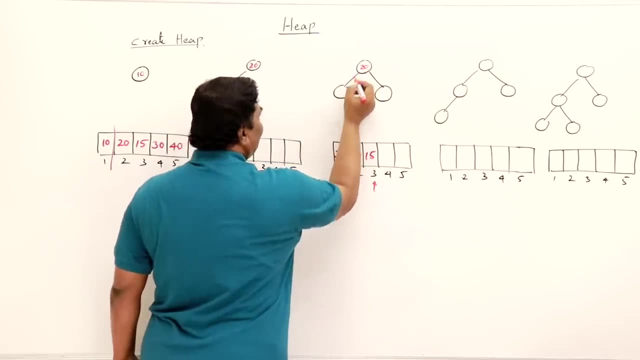 Yes, So the new element is 15.. So we are going to insert 15 now This one Earlier we have inserted the element from here. right Now 15 we are inserting. So right now we have 20 and 10 here. 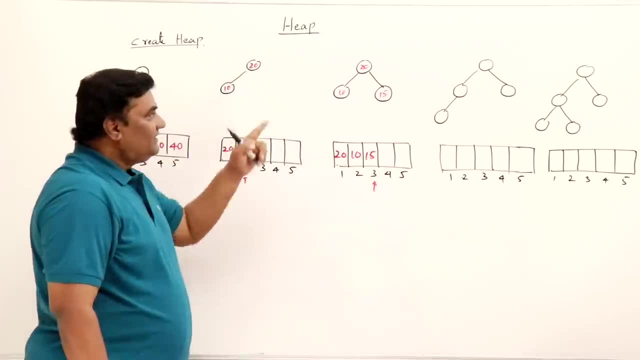 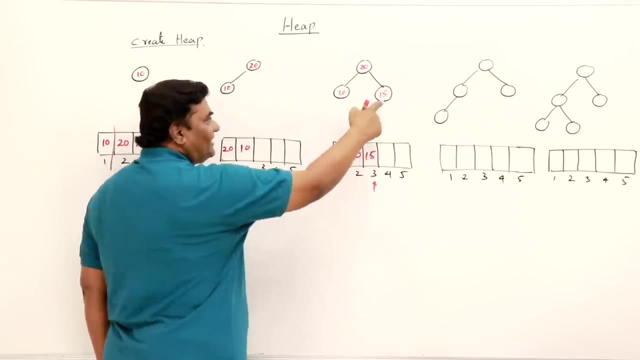 So 15 is inserted here. Now try to adjust it. How Compare with the parent. So who is the parent of 15?? 3 by 2 is 1.. So compared with the parent, 15 is smaller. So already it is in the max heap form. 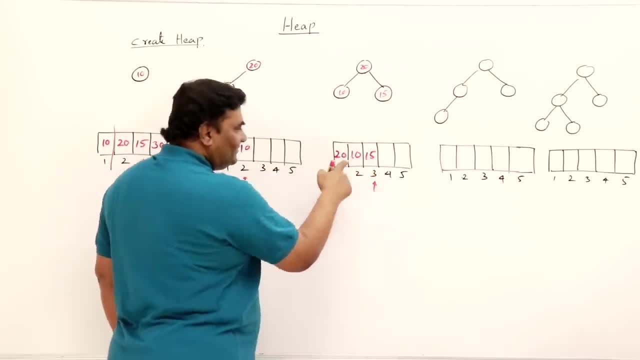 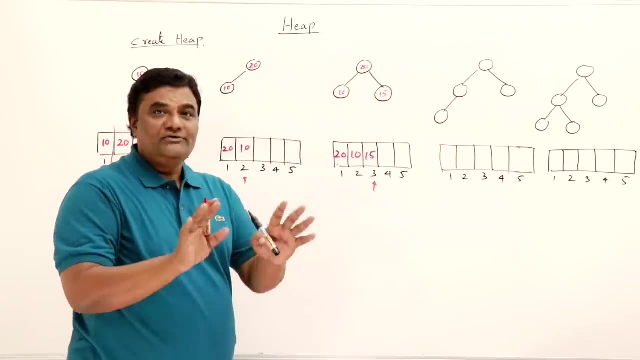 with the parent. so who is the parent of 15? 3 by 2 is 1, so compare with the parent. 15 is smaller. so already it is in the max heap form, we don't have to adjust. so till here we got a heap now. 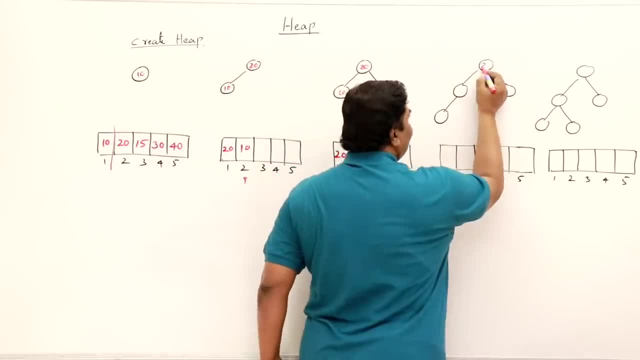 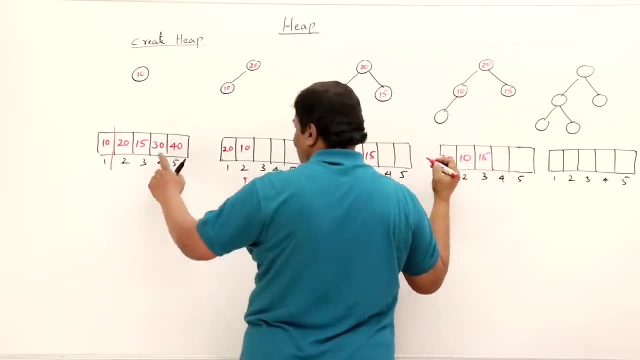 insert the next element 30. so already we have elements 20, 10, 15. now this is the next free space right: 20, 10, 15. next free space: we have 30, so 30. we are going to insert 30. this is complete binary. 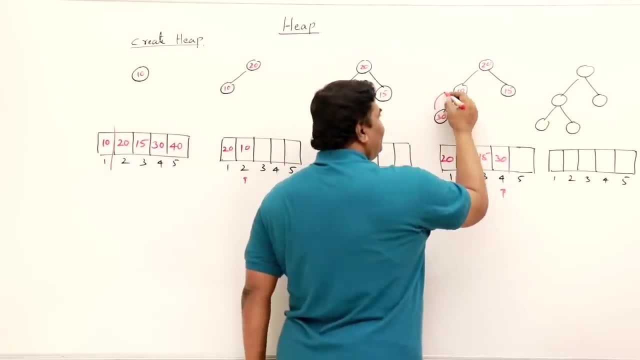 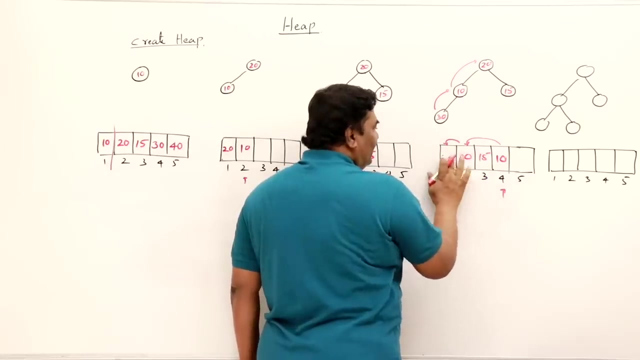 but not some max heap. adjust the element, compare with the parent and its parent. so 30 is greater than 10 and also greater than 20. so 10 will come at the place of 30. yes, here it is compared with this one. then again it is compared with 20. so 20 comes here and at this place, 30 will be inserted. 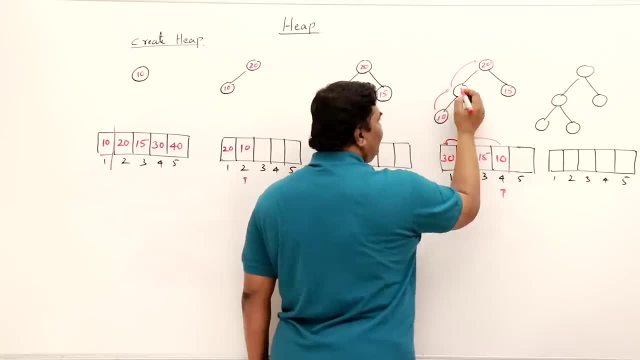 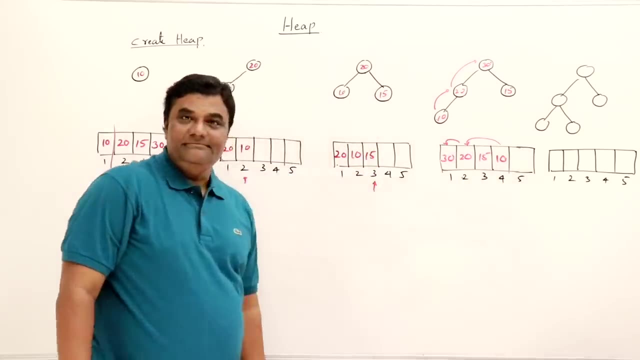 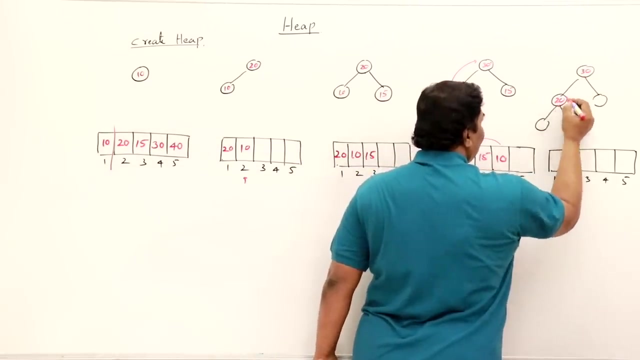 so this will modify: 10 comes here, 20 here and this becomes 30. now this is a heap till here, so we have four elements in the heap. now the last element, 40, i'm going to insert. so right now we have 30, 20, 15 and 10. so 30, 20, 15 and 10. so the new element that we are inserting is 40 here. 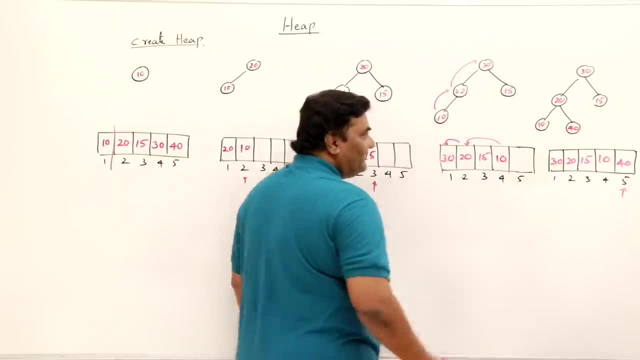 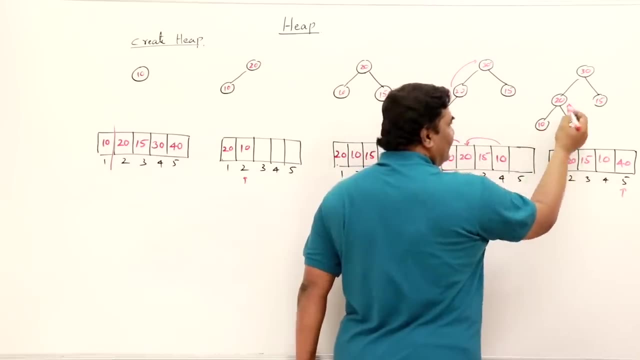 so 40 is inserted at next free space here. so it's a complete binary but not a max heap. compare with the parent: yes, 40 is greater than its parent. 40 is greater than that also, so 40 will move up. so this is the parent. 5 by 2 is 2, then its parent. so yes, 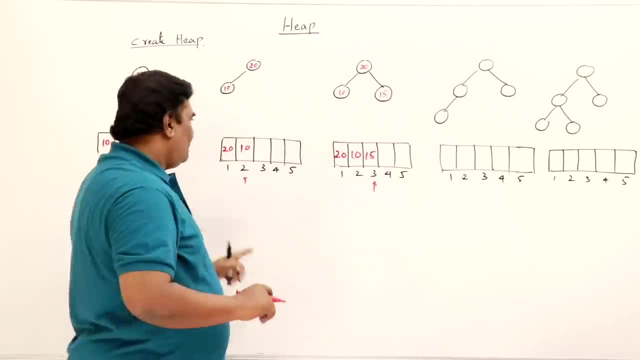 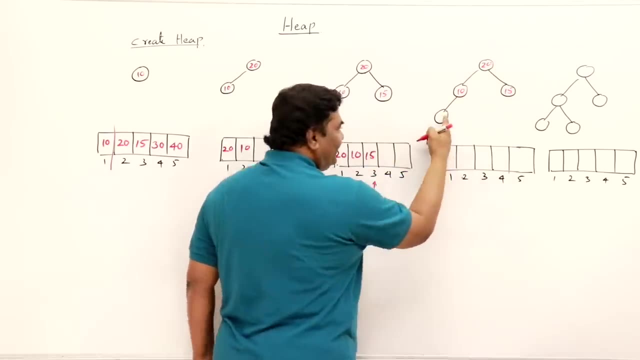 We don't have to adjust. So till here, we got a heap. Now insert the next element, 30. So already we have elements 20, 10, 15.. Now this is the next free space right: 20, 10, 15.. 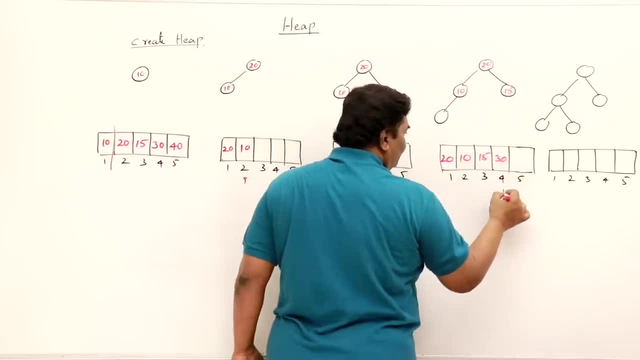 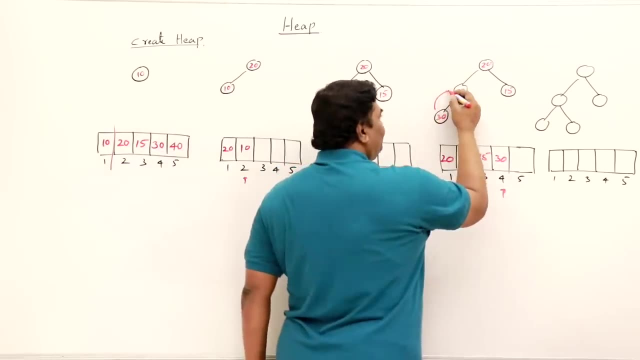 Next free space: we have 30. So 30, we are going to insert 30. This is complete binary but not a max heap. Adjust the element compared with the parent and its parent. So 30 is greater than 10 and also greater than 20.. 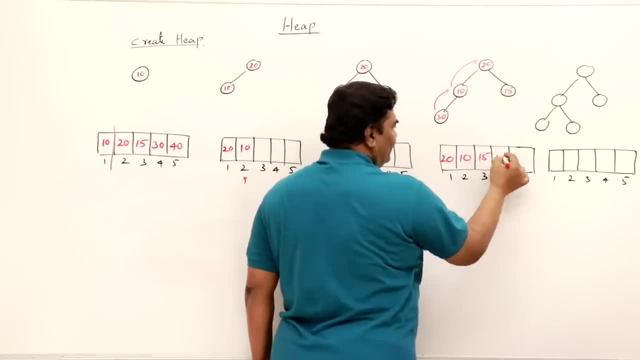 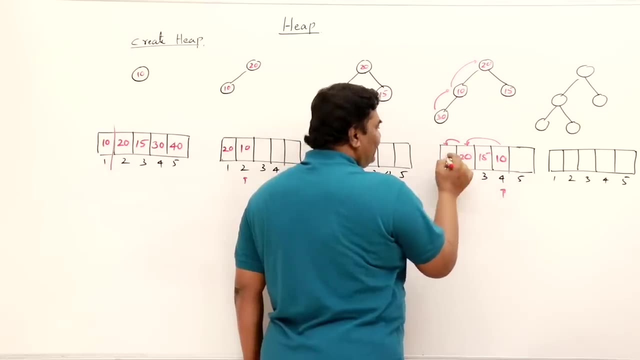 So 10 will come at the place of 30.. Yes, here it is compared with this one, Then again it is compared with 20.. So 20 comes here and at this place 30 will be inserted. So this will modify. 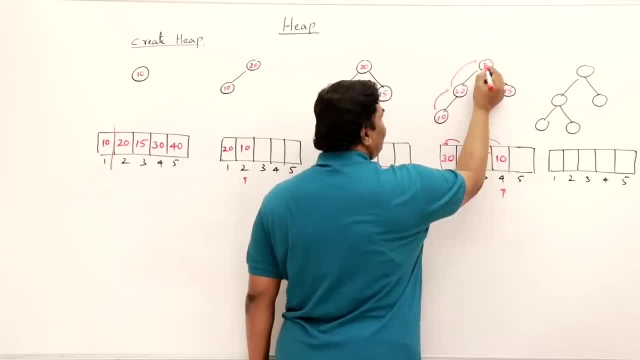 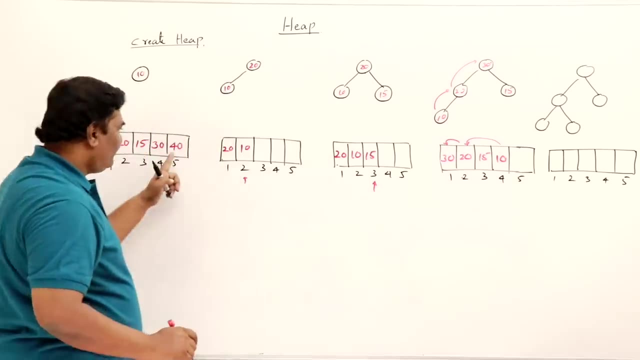 10 comes here, 20 here, and this becomes 30. Now this is a heap till here. So we have four elements in the heap. Now the last element, 40, I'm going to insert. So right now we have 30,, 20,, 15 and 10.. 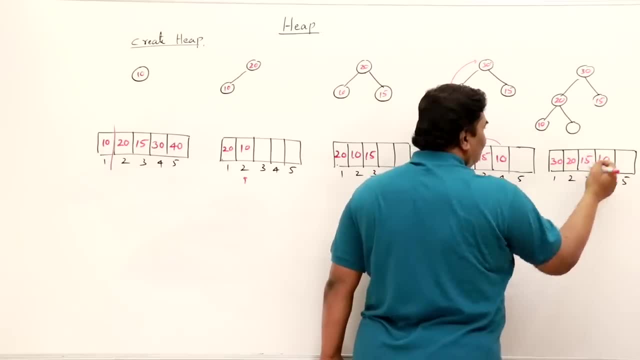 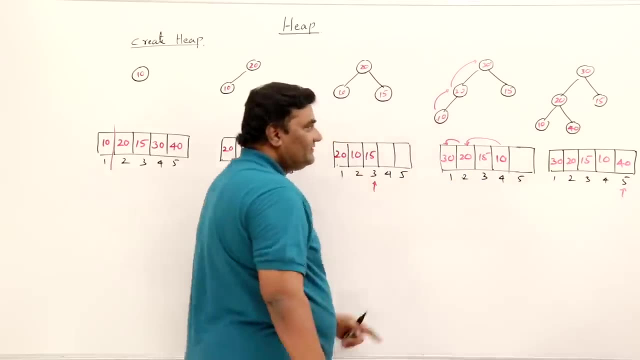 So 30,, 20,, 15, 15 and 10.. So the new element that we are inserting is 40 here, So 40 is inserted at next free space here. So it's a complete binary but not a max heap. 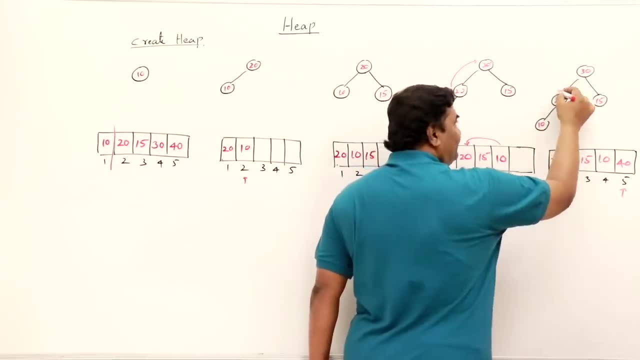 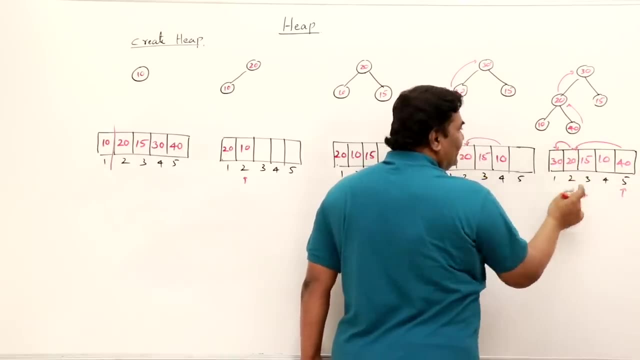 Compare with the parent: Yes, 40 is greater than its parent. 40 is greater than that also, So 40 will move up. So this is the parent: 5 by 2 is 2, then its parent. So, yes, 20 will go at this place and 30 will go at this place and 40 comes here. 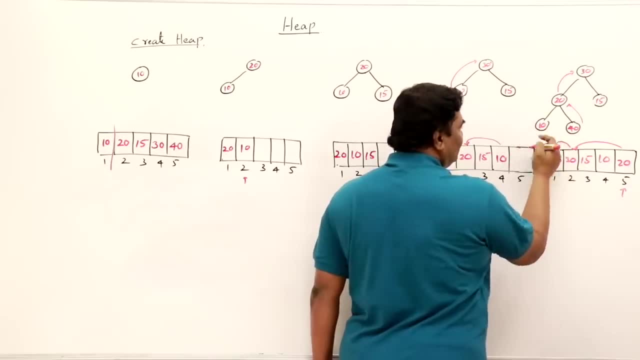 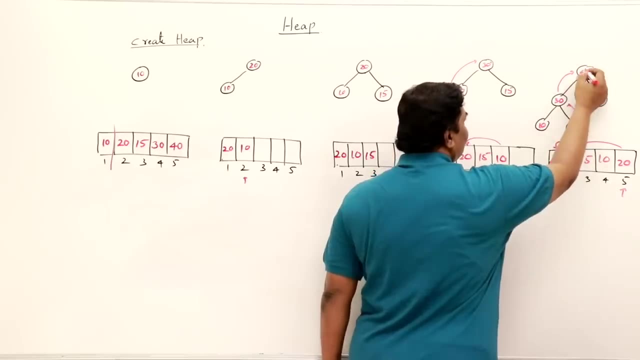 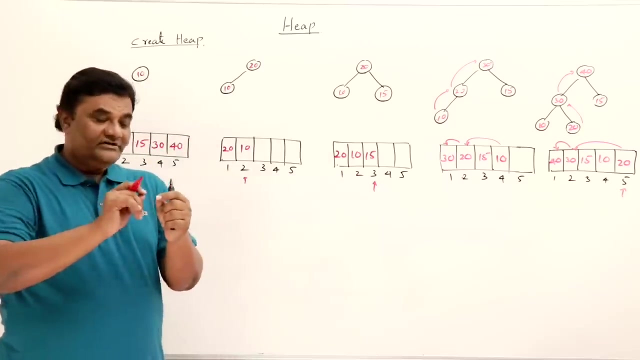 So it means. So it means 20 comes here, 30 comes here and 40 is here. So this is a max heap. So, one by one, we have inserted all the elements, and every element was inserted at a next free space and it was moved upwards and we got a max heap. 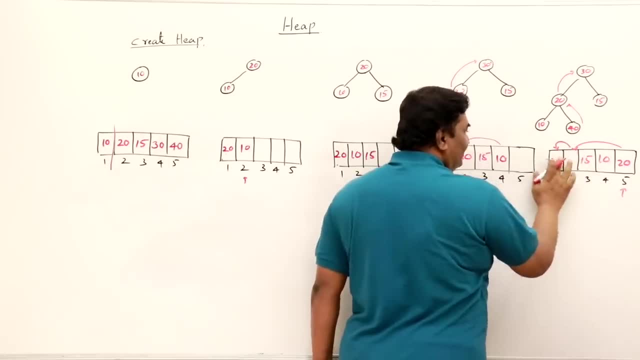 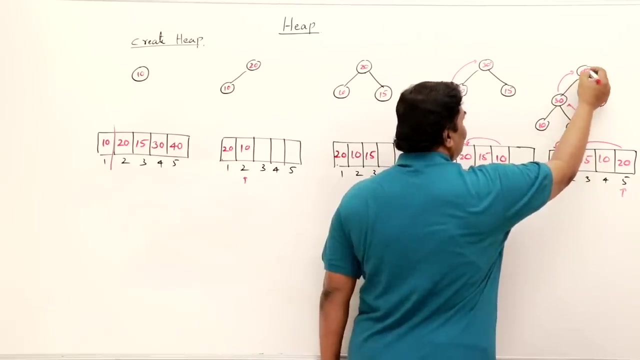 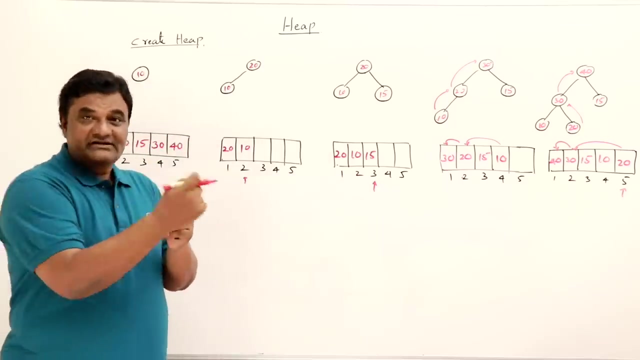 so 20 will go at this place and 30 will go at this place and 40 comes here. So it means 20 comes here, 30 comes here and 40 is here. So this is a max heap. So, one by one, we have inserted all the elements and every element was inserted at a next free space and it was moved upwards and we got a max heap. 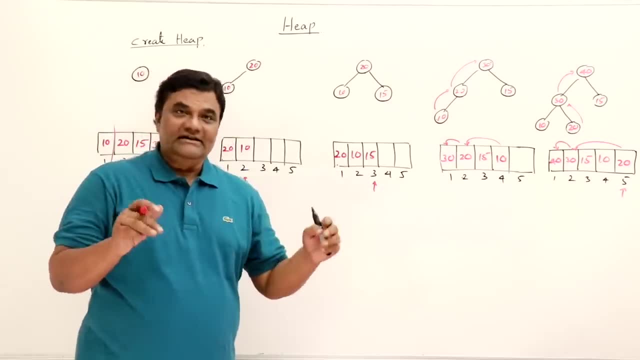 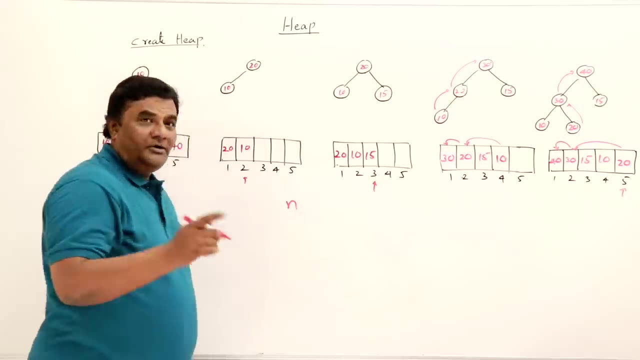 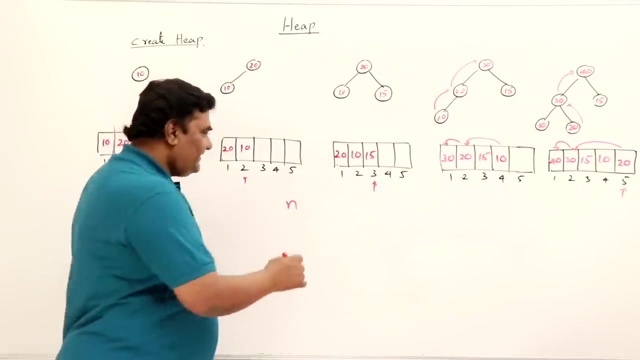 Now, before going to the next step, let us analyze how much time it has taken. We have inserted n elements. total n elements we have inserted. How much time it takes for inserting an element in a heap depends on the height. What is height of a complete binary tree or a heap? 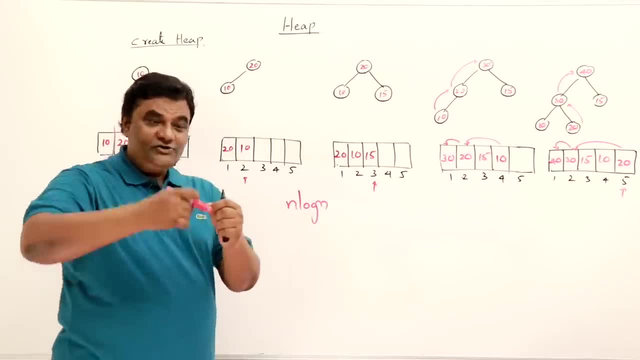 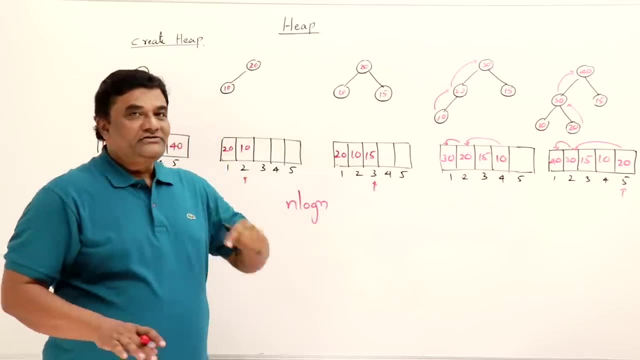 It is log n, So n elements, each element. we assume that it is moved up to the root, So it is log n. So the time taken is n log n. So this was the heap creation first step. Now from that heap I will be going. 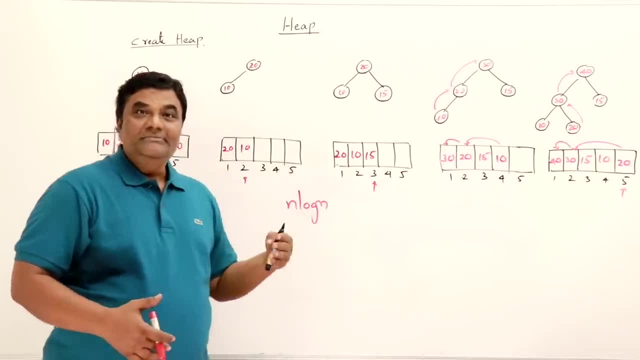 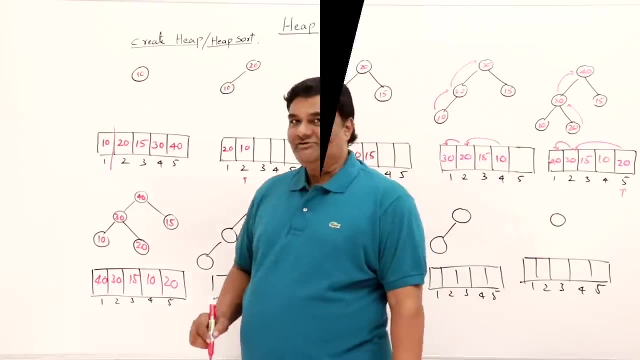 to deleting the elements. So this place I will show you how the elements are deleted and they are also sorted. So let us delete the elements Now. second step, for heap sort. already we have created a heap. Now, the same heap I have taken, this is the heap that we got. 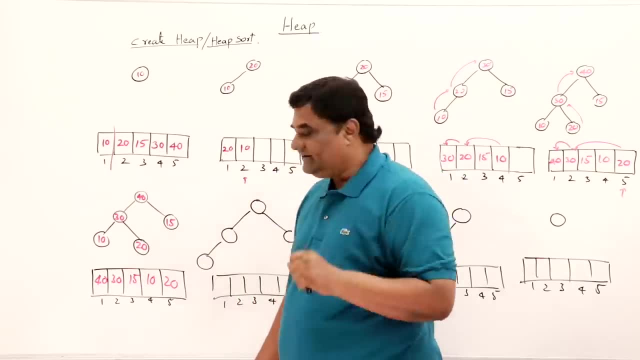 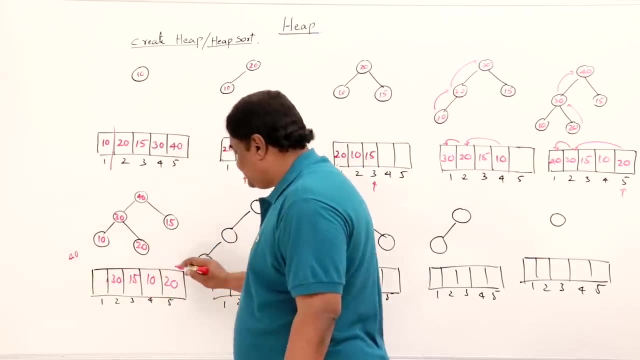 Now let us delete the element. So we know very well how to delete the element. So in this let us delete. So which element gets deleted? 40 gets deleted, 40 is gone out. Then who will take its place? Last 20,, this will take its place. 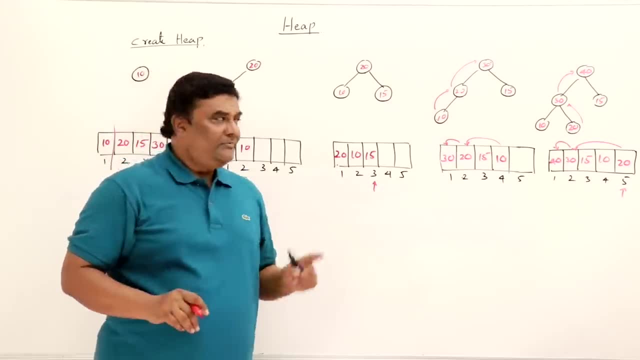 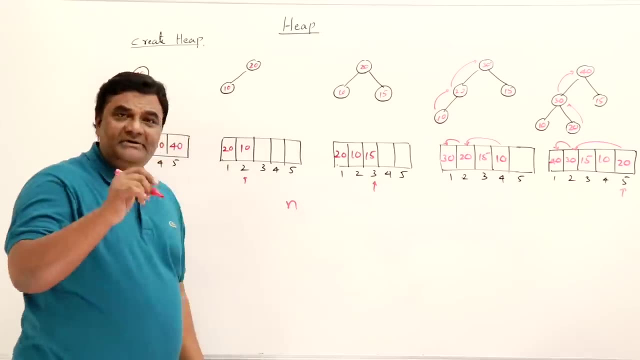 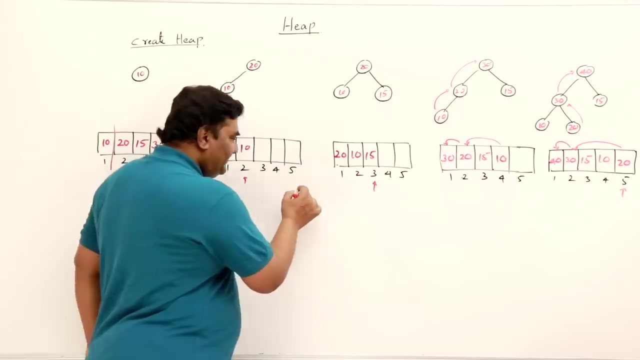 Now, before going to the next step, let us analyze how much time it has taken. We have inserted n elements. total n elements we have inserted. How much time it takes for inserting an element in a heap depends on the height. What is height of a complete binary tree or a heap? 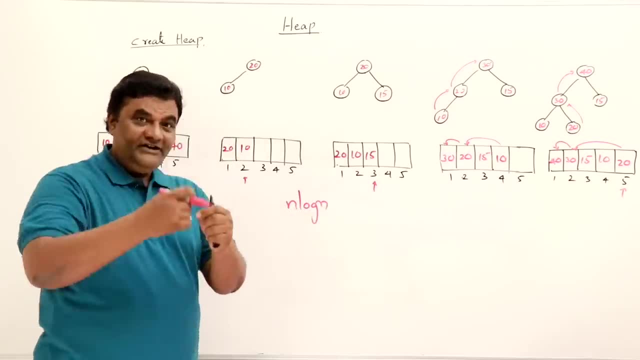 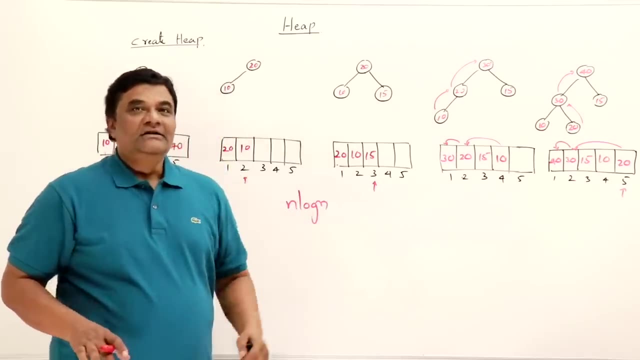 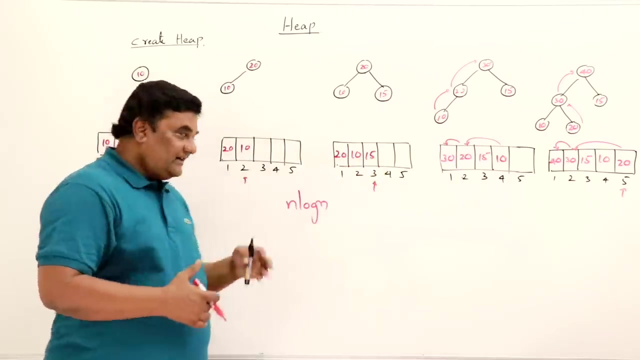 It is log n, So n elements. each element, we assume that it is moved up to the root, so it is log n. So the time taken is n log n. So this was the heap creation for system. Now from that heap I will be going on deleting the elements. So this place I will show you how the elements are deleted and they are also sorted. 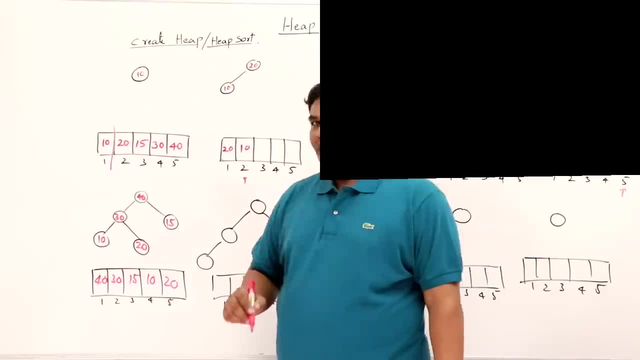 So let us delete the elements Now. second step: for heap sort: Already we have created a heap Now. let us delete the elements Now. second step: for heap sort: Already we have created a heap Now. second step: for heap sort: Already we have created a heap. 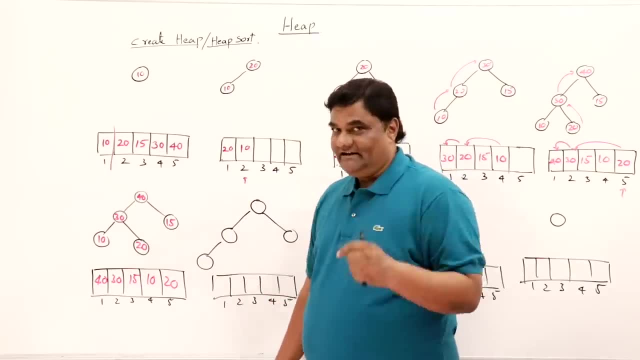 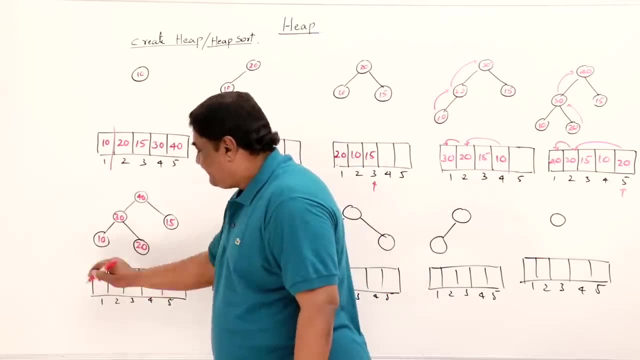 Now the same heap I have taken. This is the heap that we got. Now let us delete the element. So we know very well how to delete the element. So in this, let us delete. So which element gets deleted? Forty gets deleted. Forty is gone out. Then who will take its place? Last twenty? This will take its place. Twenty will take its place. 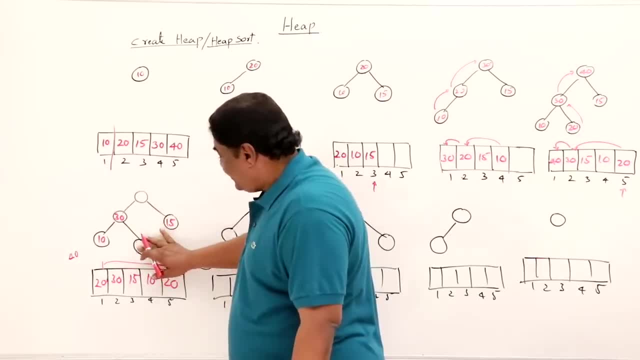 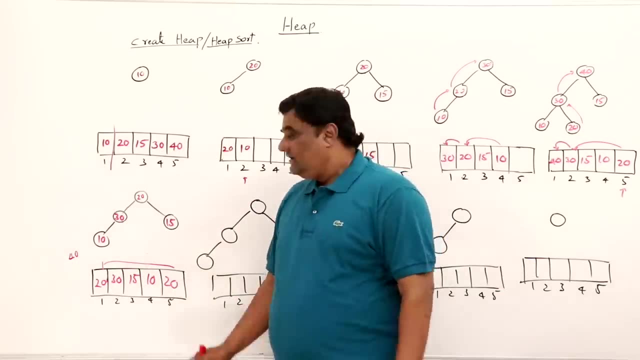 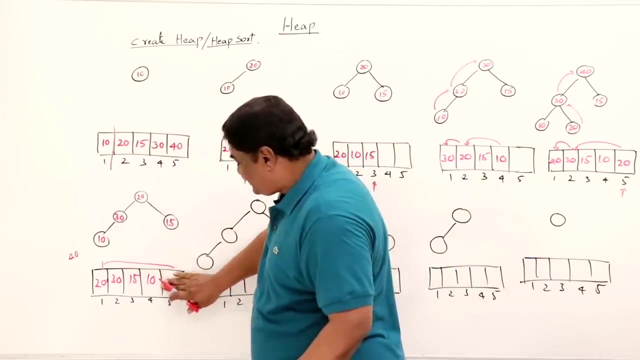 So in the diagram I will show, forty is removed and twenty will go in its place. So it means this element is gone. Now this is complete binary but not a max heap, So we have to adjust. We have to adjust downwards, So this 20 is gone. 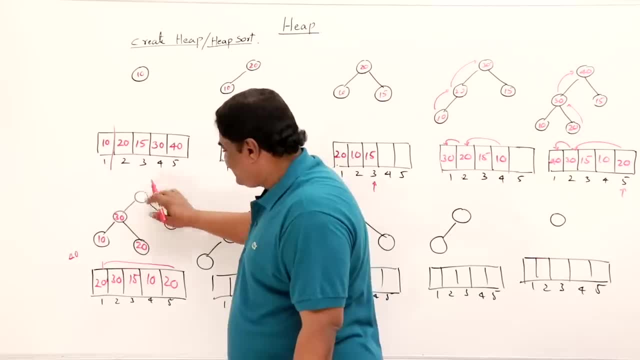 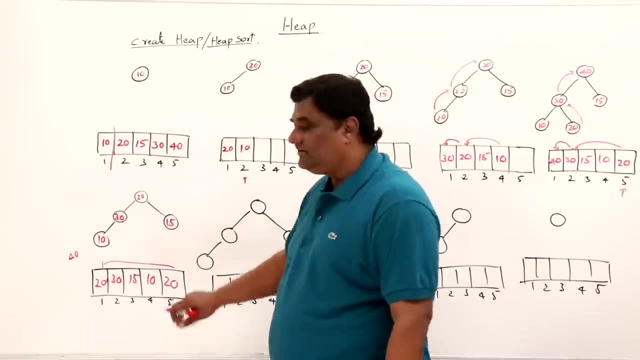 20 will take its place. So in the diagram I will show, 40 is removed and 20 will go in its place. 20 will go in its place. So it means this element is gone. This element is gone. Now, this is complete binary, but not a max heap. 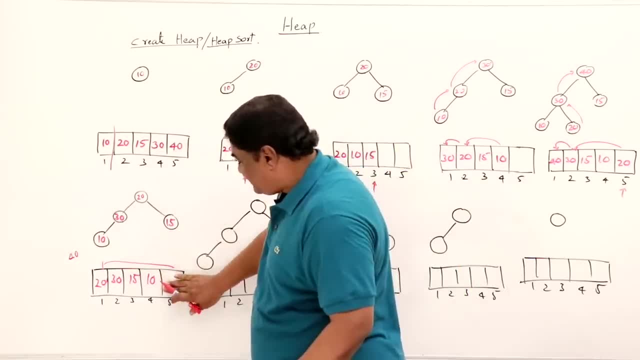 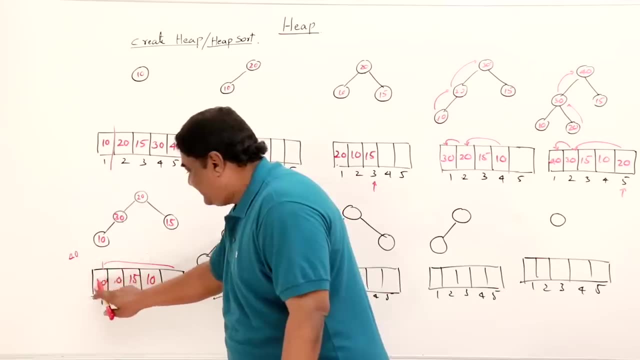 So we have to adjust. We have to adjust downwards. So this 20 is gone, right, 20 is removed. Now 30 and 15, 30 is greater. So 30 will go in the place of 20 and 20 will come here. 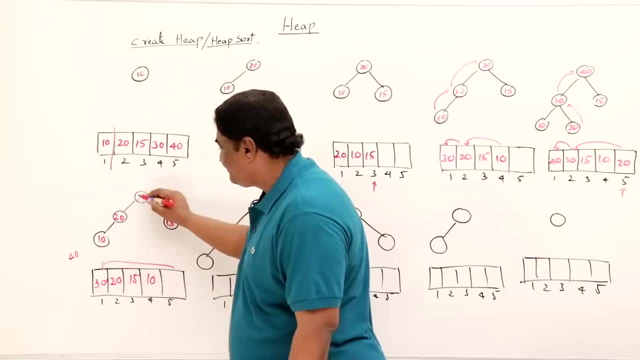 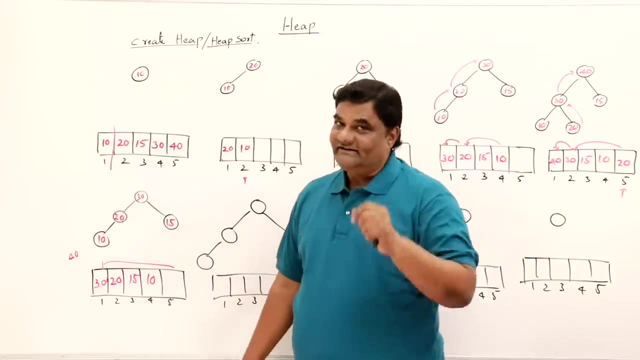 So this becomes 20 and this becomes 30. Then again compare 20 with 10.. So it's perfect. So these are the changes. So now 40 is deleted and we got one free space. Now here I will show. I will add the elements. 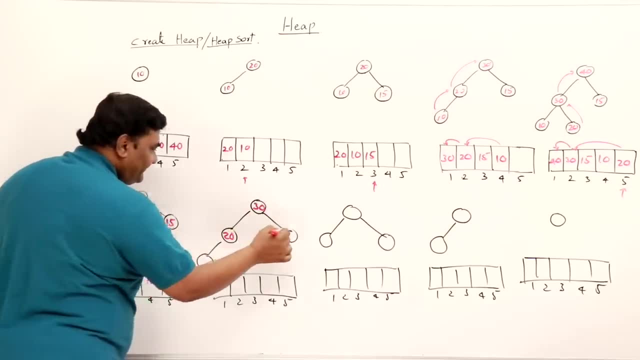 See we have 30 here and 20 here, 15 and 10.. So the elements in the heap are 30,, 20,, 15 and 10.. Heap is till 4 elements, only 40 which was deleted. I will put it here at a free space. 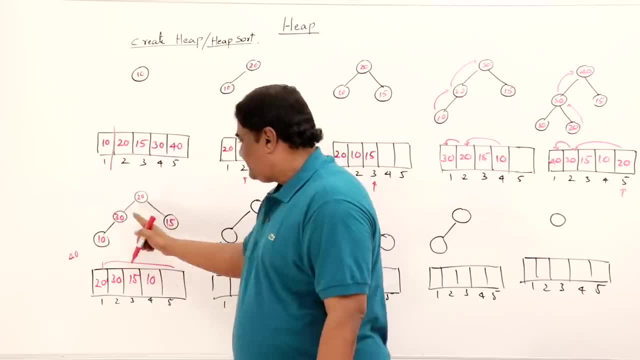 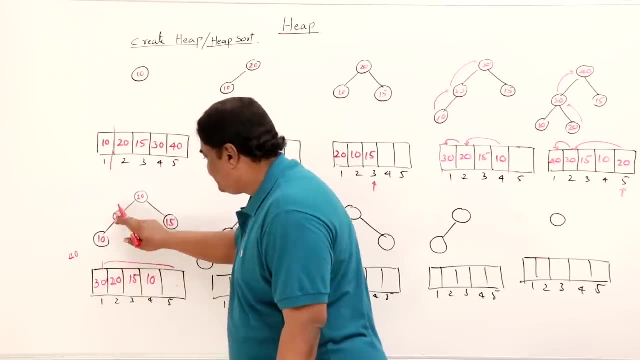 right, 20 is removed, Now 30 and 15,. 30 is greater. So 30 will go in the place of 20 and 20 will come here. So this becomes 20 and this becomes 30. Then again compare 20 with 10.. So 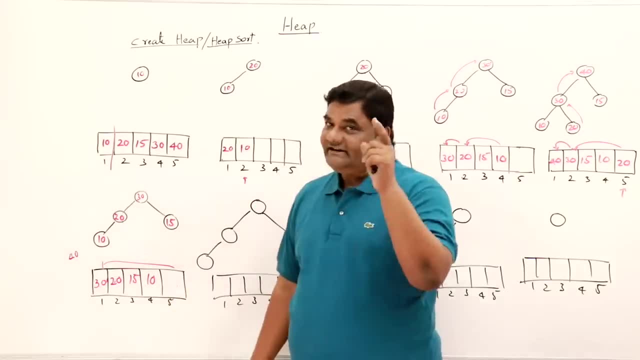 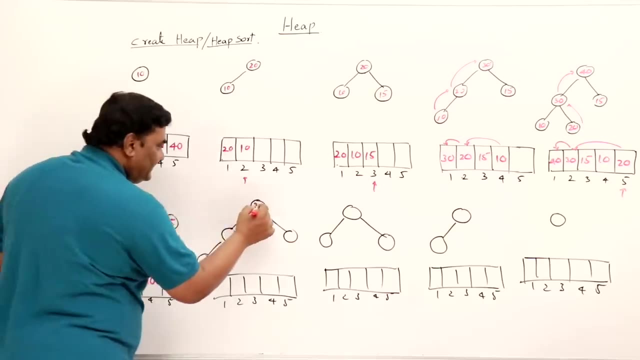 it's perfect. So these are the changes. So now 40 is deleted and we got one free space. Now here I will show, I will add the elements. See, we have 30 here and 20 here, 15 and 10.. So the elements. 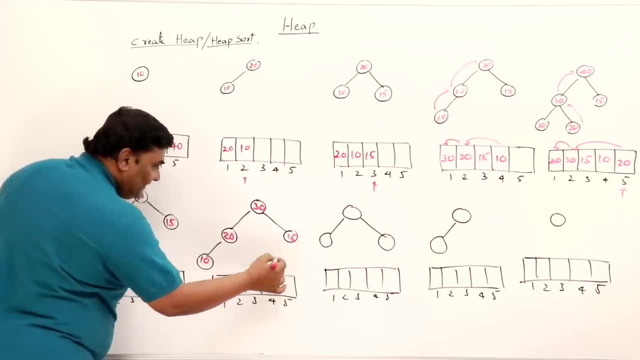 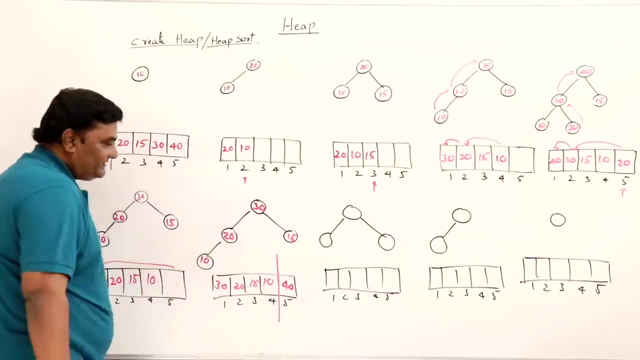 in the heap are 30,, 20,, 15 and 10.. Heap is till 4 elements, only 40 which was deleted. I will put it here at a free space That is not a part of heap. Now delete next element. So next element. 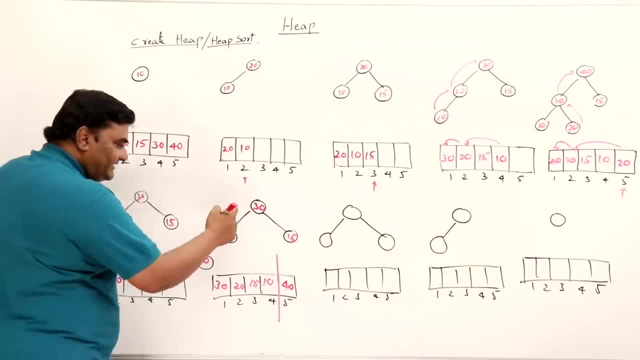 That is not a part of heap. Now delete next element. So next element: which element will be deleted? 30 will be deleted. 30 is gone. Who will take its place? Last element in complete binary: 10.. So in this array, 30 is gone. 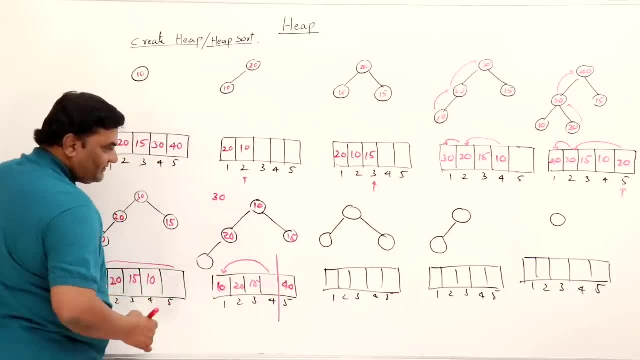 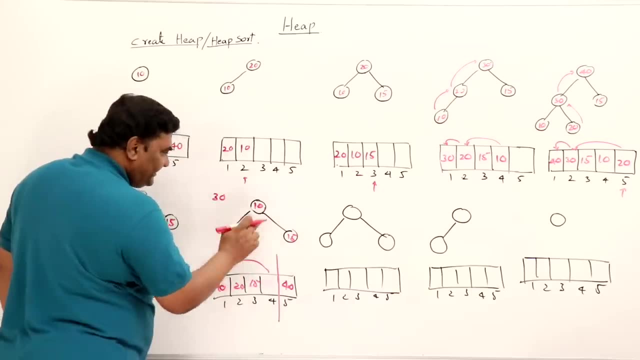 So the 10 last element will come here. This element came here, So this is not there. So one more element reduced. We have to adjust this one. Compare with the children: 20 is greater, So 20 moves up And 10 comes down. right, 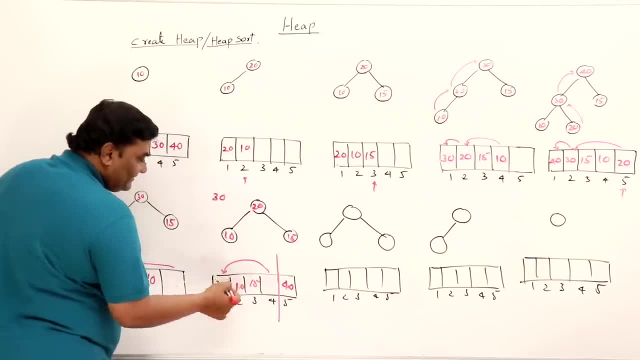 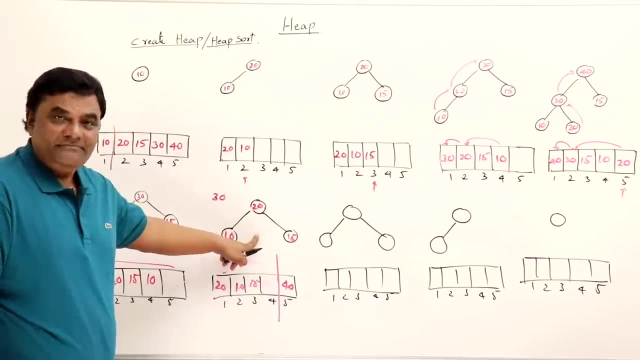 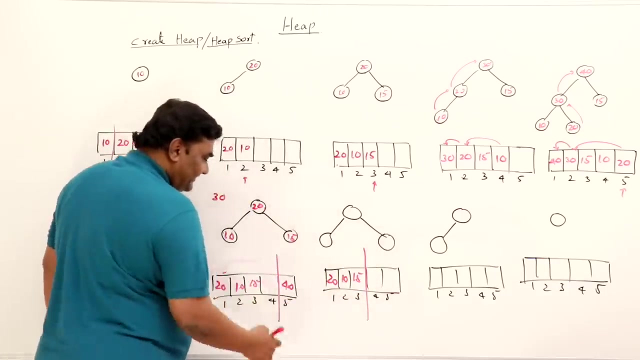 So this becomes 20 and this becomes 10.. So this is deleted. I'll remove this arrow Now. 30 is deleted and this is in a max heap form. Now next step. here I will show: We have the elements 20, 10 and 15, and heap is ending here. 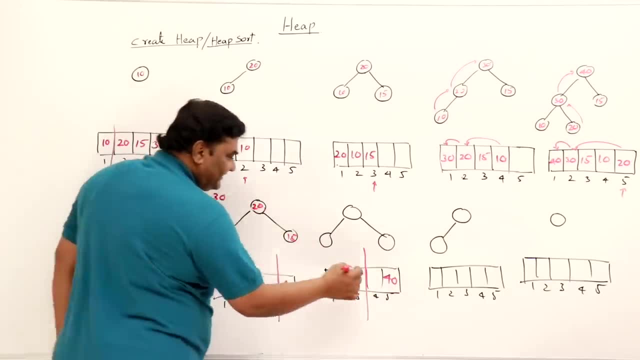 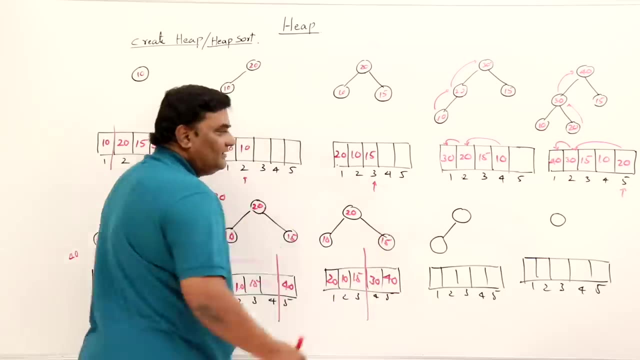 40 was already there. We got one more free space, So keep 30 there. the newly deleted element And in the diagram this is 20, 10 and 50. This is 15.. Still, we have to delete three more elements. 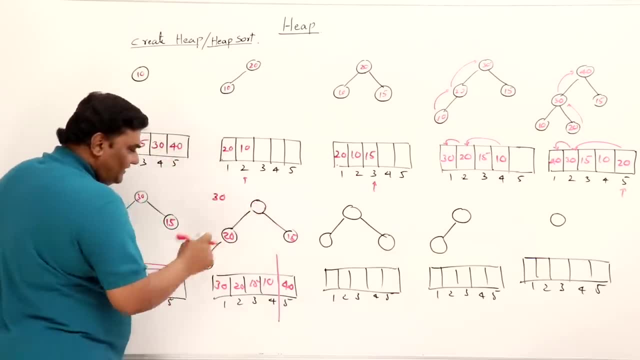 which element will be deleted? 30 will be deleted. 30 is gone. Who will take its place? Last element in complete biotic: 10.. So in this array, 30 is gone. So the 10 last element will come here. This element came here. 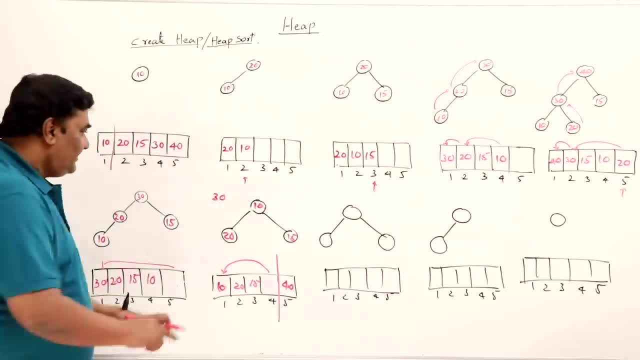 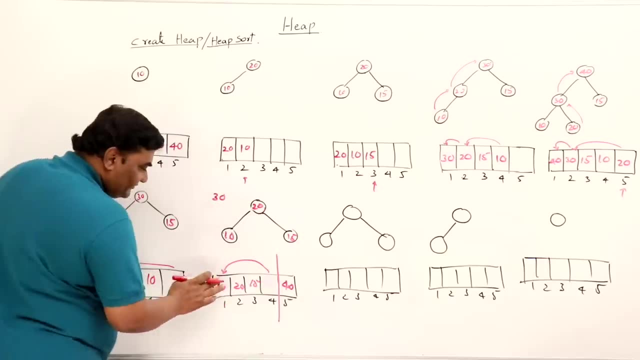 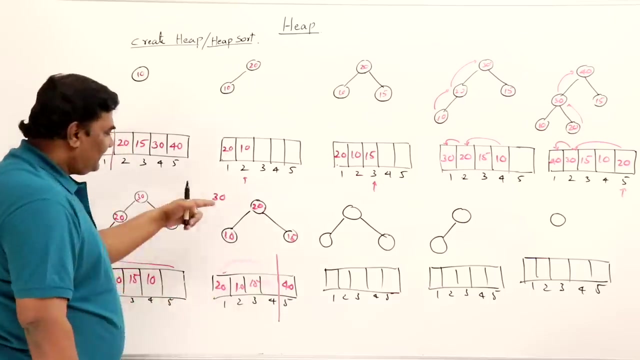 So this is not there. So one more element reduced. We have to adjust this one. Compare with the children: 20 is greater, So 20 moves up and 10 comes down. right, So this becomes 20 and this becomes 10.. So this is deleted. I will remove this arrow Now. 30 is deleted and this is in a max heap. 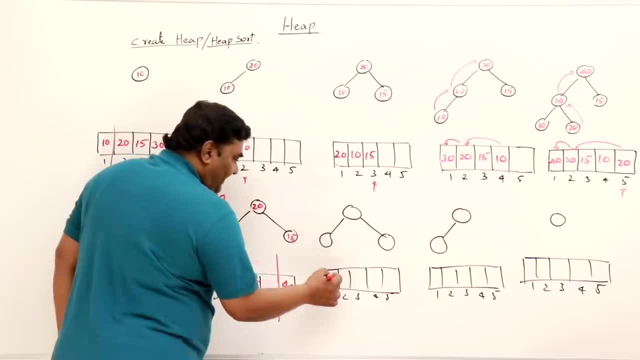 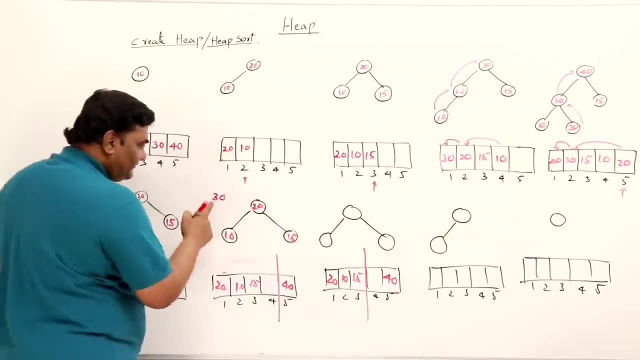 form. Next step: here I will show. We have the elements 20,, 10 and 15, and heap is ending here. 40 was already there. We got one more free space, So keep 30 there, the newly deleted element, And in the diagram. 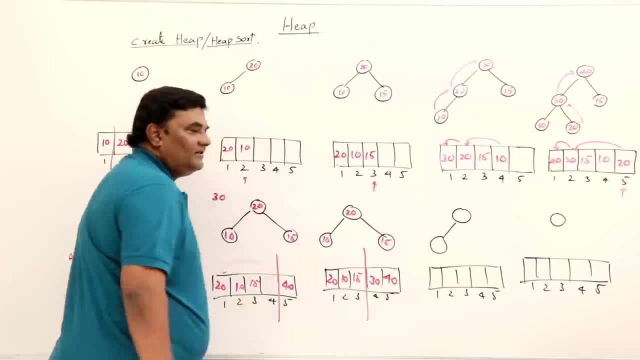 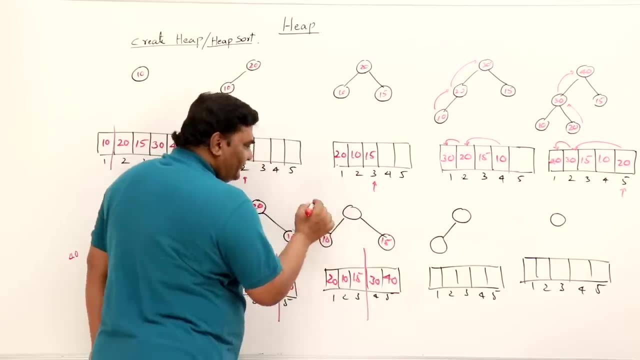 this is 20,, 10 and 15.. Still, we have to delete 3 more elements Now. next delete one more element. Which element get deleted? 20 is deleted From the array. this is gone. Who will take its place Last? 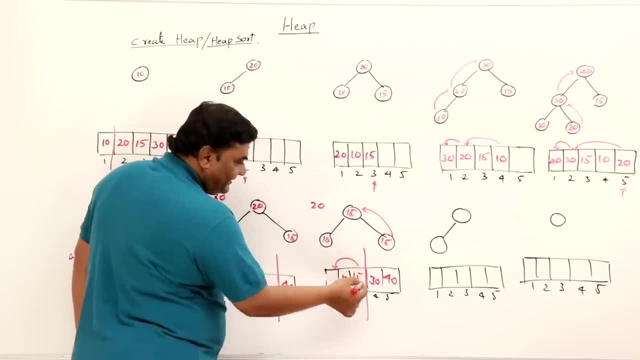 element in complete biotic will take its place. So this is 20, 10 and 15.. So this is 20, 10 and 15.. So 15 will come here. Last element in the array that is in the heap: 15 comes here. So this place is. 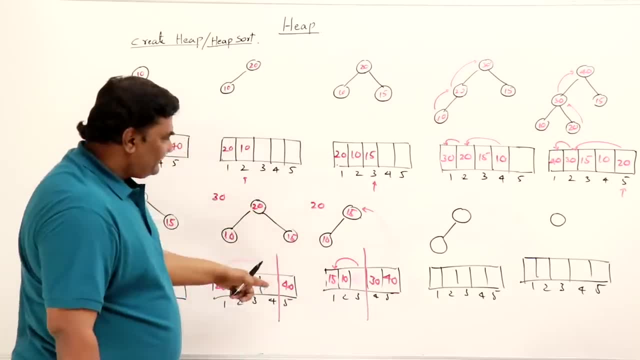 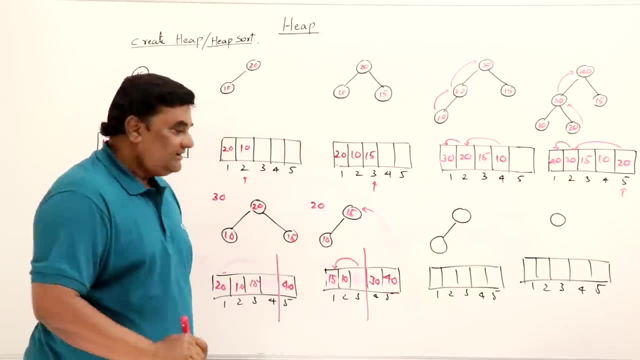 free. So this is gone. Now adjust Already. 15 is greatest, So child is smaller. No need to swap the element, It's already perfect. So this is the result. Then next space I will write down: This is 15. 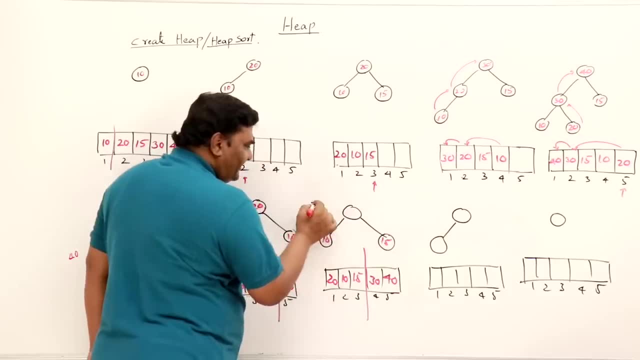 Now next, delete one more element. Which element get deleted? 20 is deleted from the array. This is gone. Who will take its place? Last element in complete binary will take its place 15.. So 15 will come here. 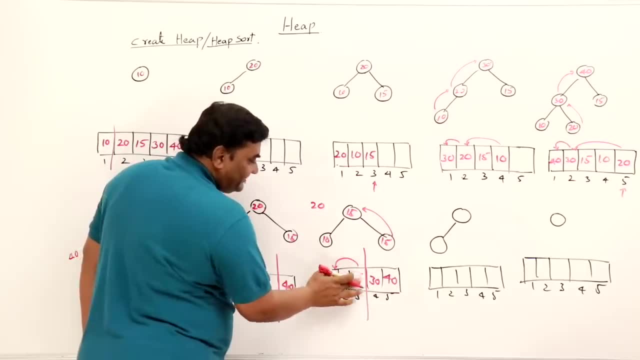 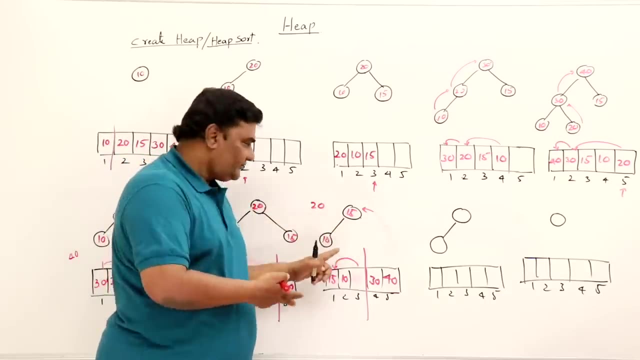 Last element in the array that is in the heap: 15 comes here, So this place is free. So this is gone. Now adjust Already: 15 is greatest, So child is smaller. No need to swap the element, It's already perfect. 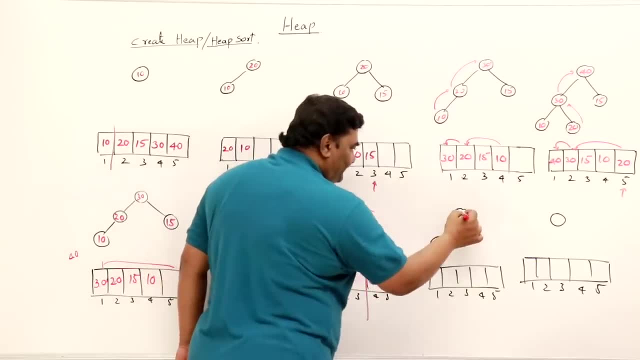 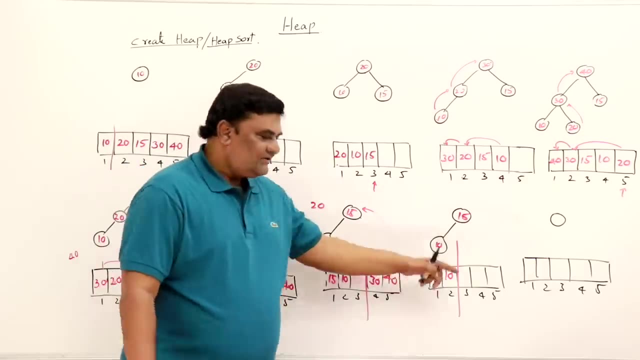 So this is the result. Then next space, I will write down: This is 15 and this is 10.. So this is 15 and 10 and heap is reduced till here. So there were three elements. Now there are only two elements. 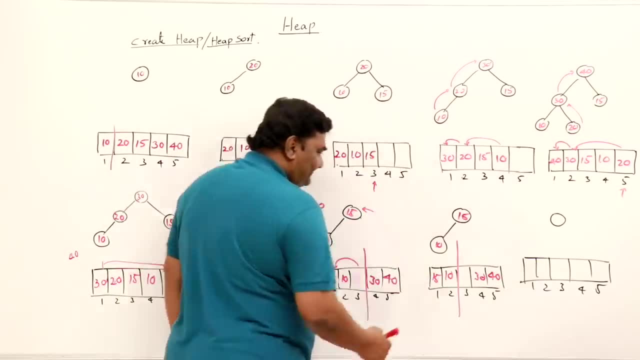 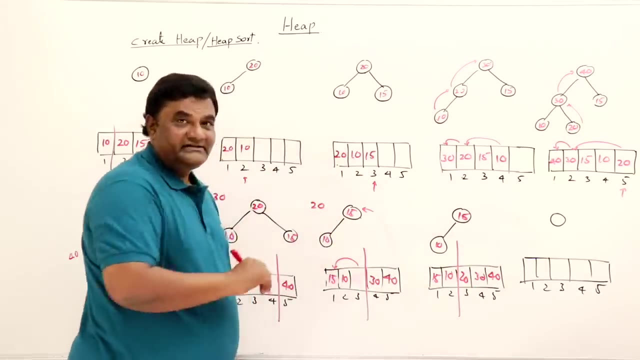 Already I have 40 at the last and 30 at the second last place. One more free space. I got There, I can insert 20.. So just store 20.. I should not say insert, Just I have stored 20 there, kept 20 there. 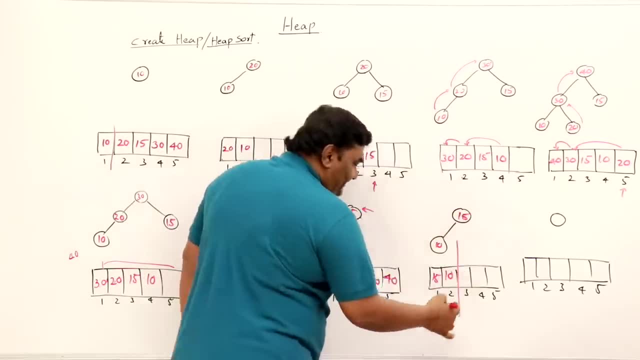 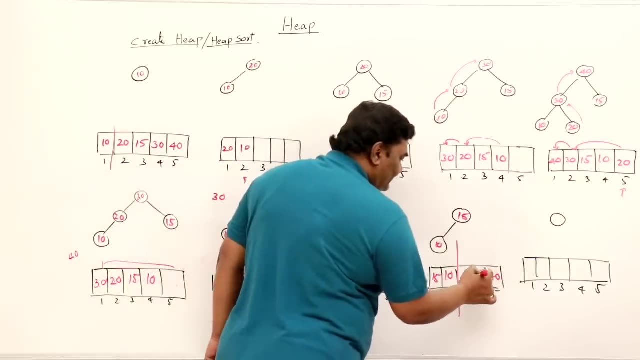 and this is 10.. So this is 15 and 10.. And heap is reduced till here. See, there were 3 elements. Now there are only 2 elements. Already. I have 40 at the last and 30 at the second last place. One more free space. I got There, I can. 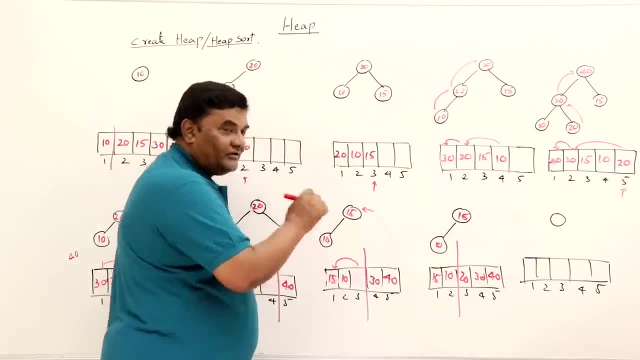 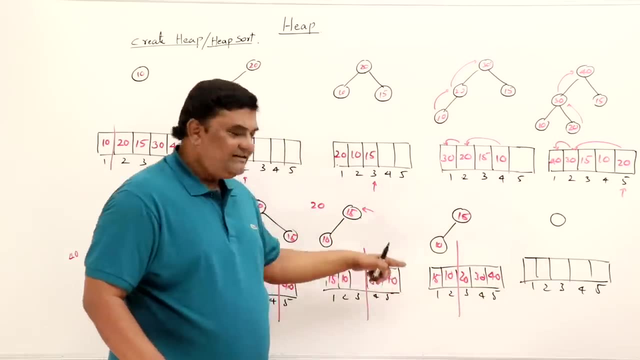 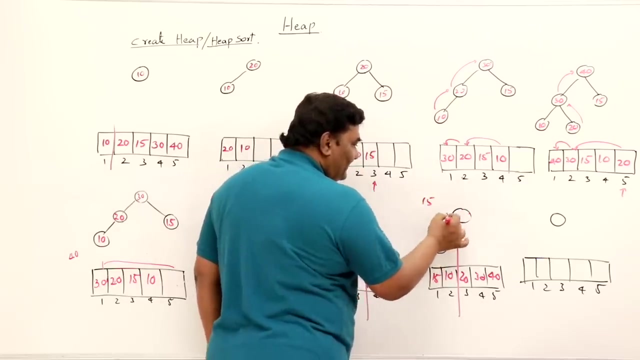 insert 20.. So just store 20.. I should not say insert, Just. I have stored 20 there, Kept 20 there. Now these elements are deleted from the heap. These are remaining still in the heap. Now delete next element. Which element is deleted? 15 is deleted. Who will take its place? Last element? So it means 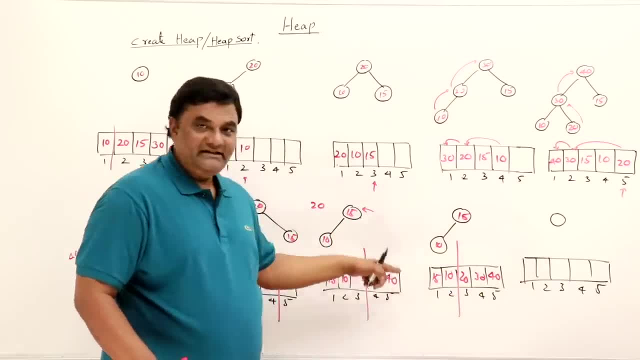 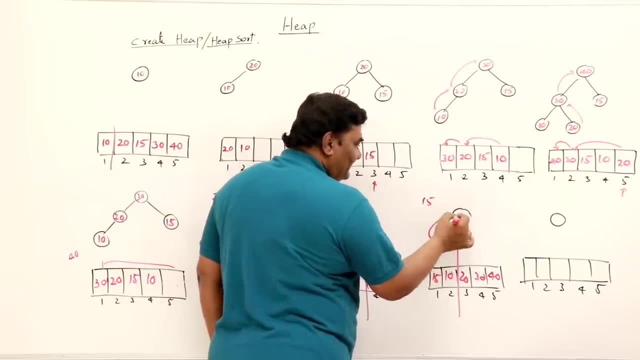 Now these elements are deleted from the heap. These are remaining still in the heap. Now delete next element. Which element is deleted? 15 is deleted. Who will take its place? Last element. So it means this is gone. So here also, 15 is gone. 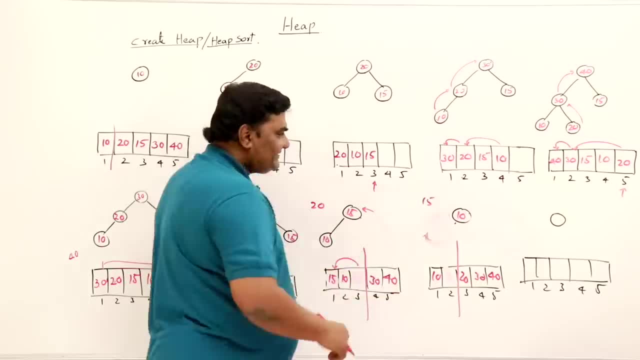 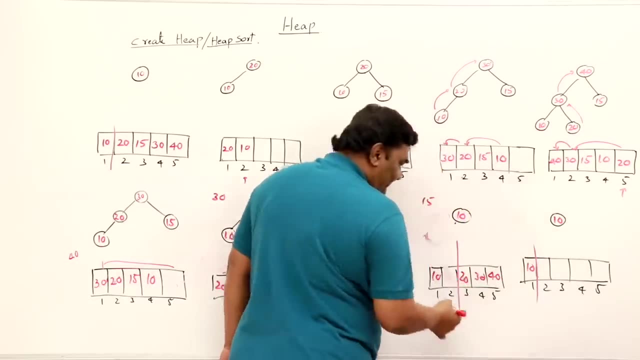 10 will take its place. Now. do you have to adjust? You don't have to adjust anything. Now. what will be the result? This is 10.. So, this is 10.. Now, heap ends here. Now we already have 20,, 30 and 40 here. 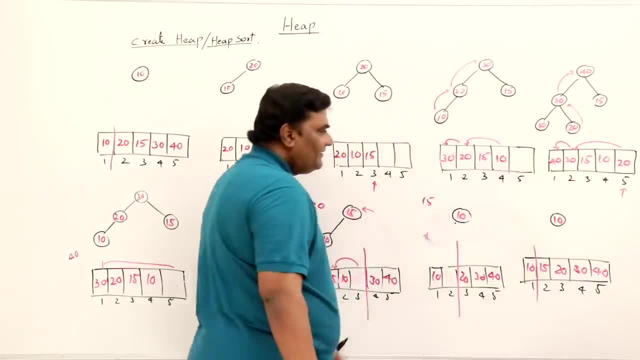 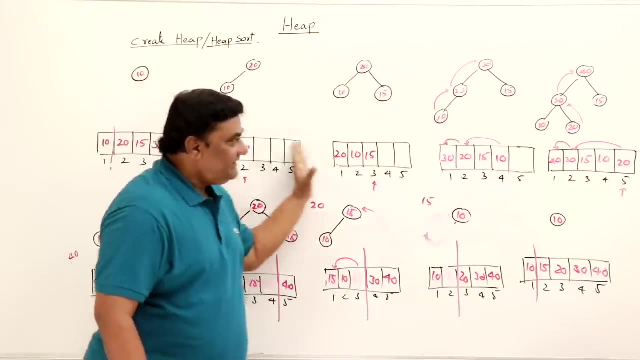 We got one free space, So there you store 15.. So that's how the elements are sorted. So the heap sort. first step. If the elements are given, then create a heap. Then, second step, go on deleting the element and store the element at a free. 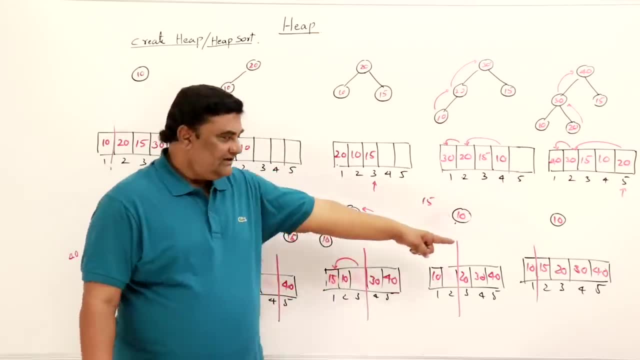 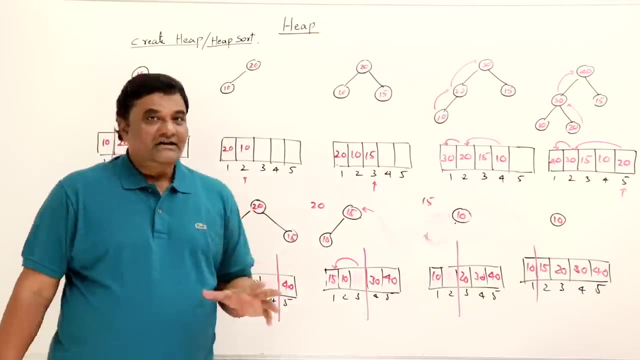 space we are obtaining after deleting the element. So finally, the elements are sorted. So look at this. So you have to observe it, because too much board work is there, A lot of board work is there, So you may miss at some place, or I suggest you just pause the video and 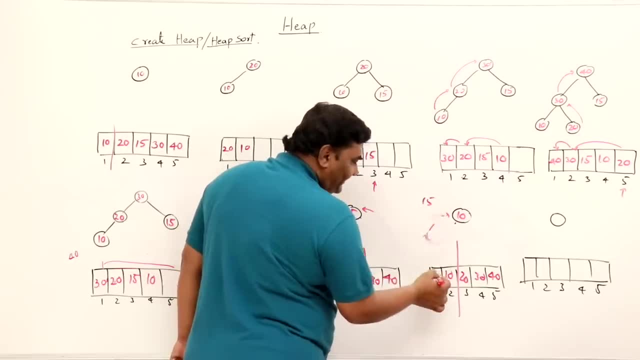 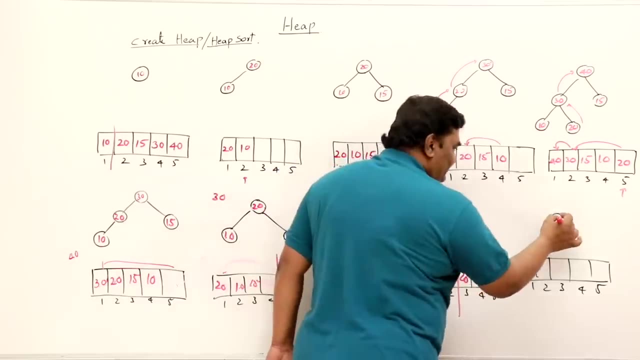 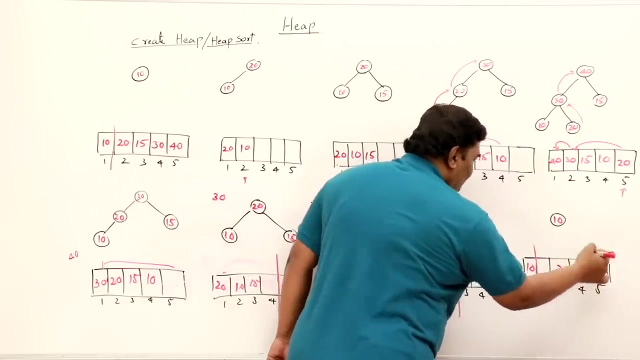 this is gone. So here also, 15 is gone. So when you take this place, Now we have to adjust, You don't have to adjust anything. Now what will be the result? This is 10.. So this is 10.. Now heap ends here. Now we already have 20, 30 and 40 here. 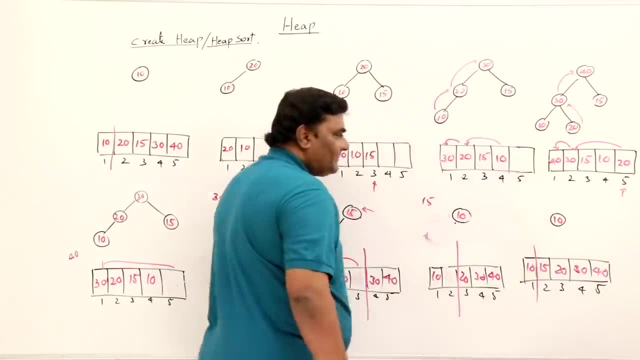 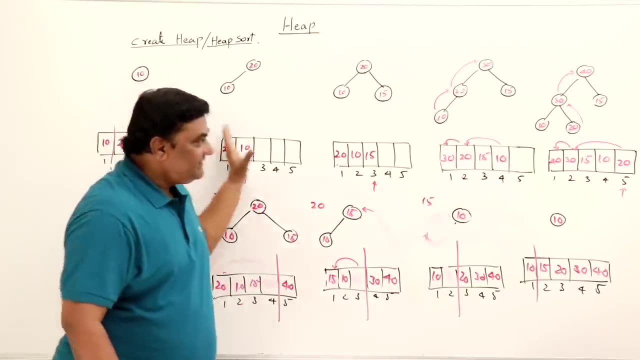 We've got one free space, So there you store 15.. So that's how the elements are sorted. So the heap sort. first step: If the elements are great given, then create a heap. Then, second step, Go on deleting the element and store the. 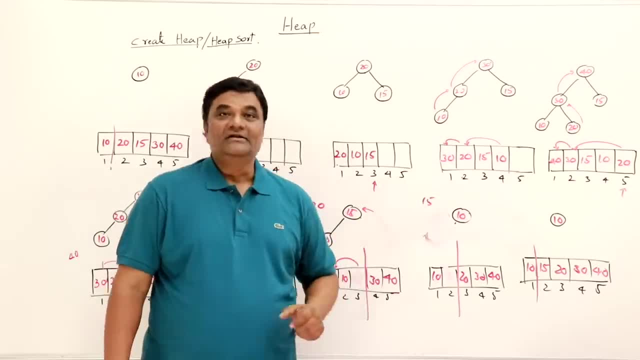 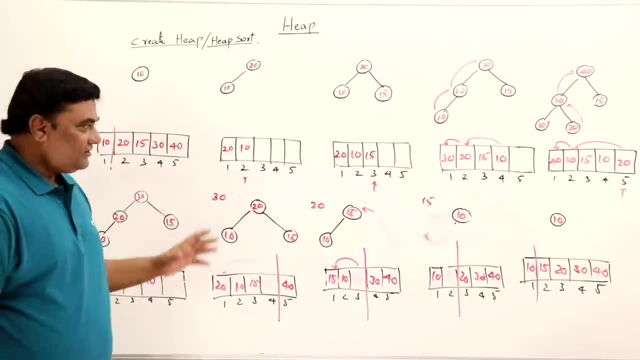 element at a free space we are obtaining after deleting the element. so finally, the elements are sorted. so you look at this, so you have to observe it, because too much board work is there, a lot of board work is there, so you may miss at some place. so i suggest you just pause the video and have a 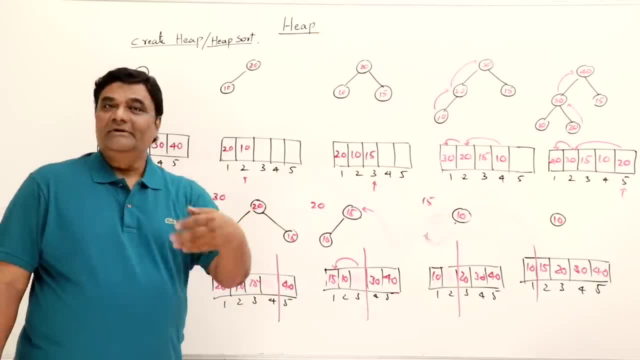 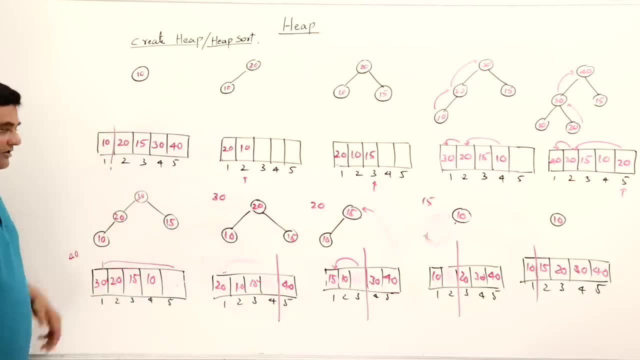 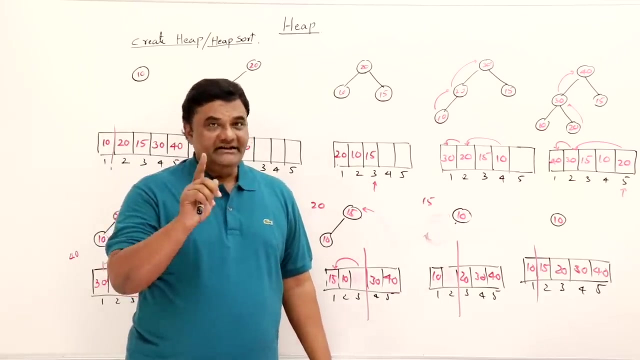 look at it- complete example is there on board right- and do it by yourself. once you do it by yourself then you can remember it always how it is working. just take a snapshot or copy everything from whiteboard. if we do the analysis already- creation process- we have seen n log n creating. 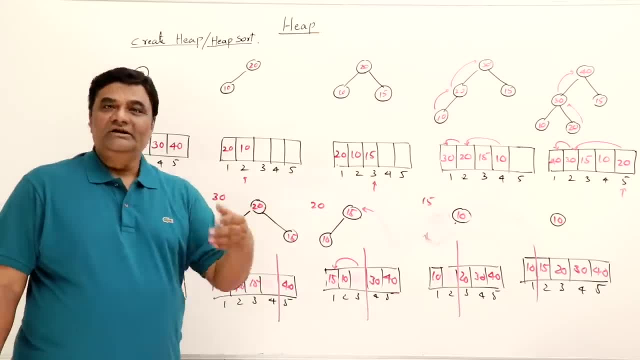 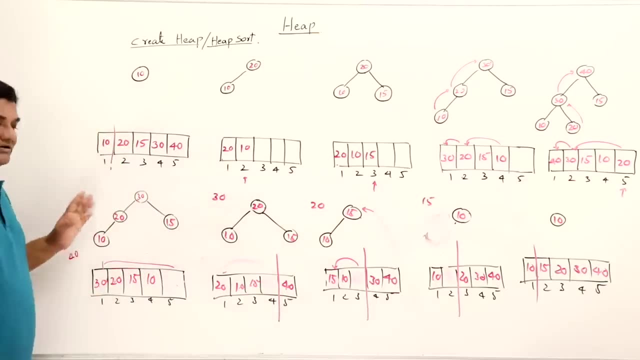 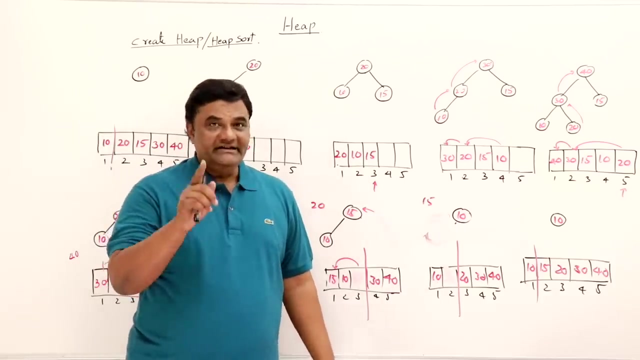 have a look at it- complete example is there on board- and do it by yourself. Once you do it by yourself, then you can remember it always how it is working. Just take a snapshot or copy everything from whiteboard. If we do the analysis already. creation process- we have seen- and login creating. 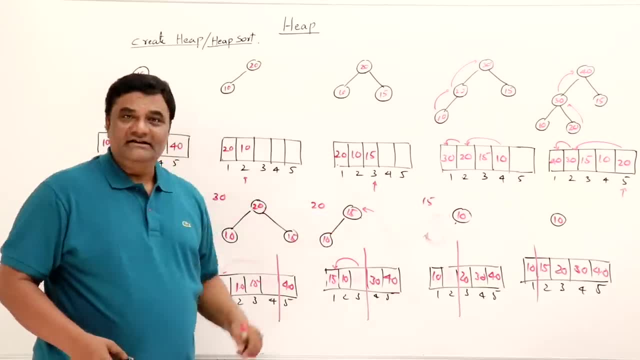 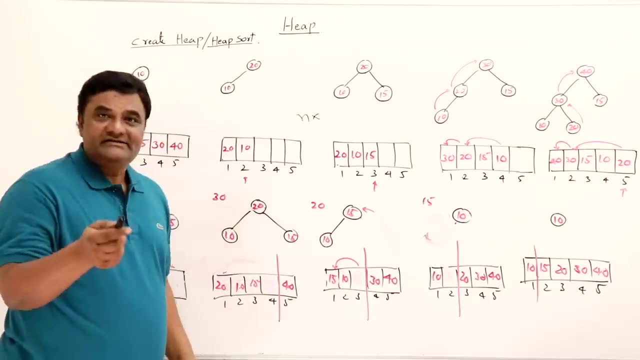 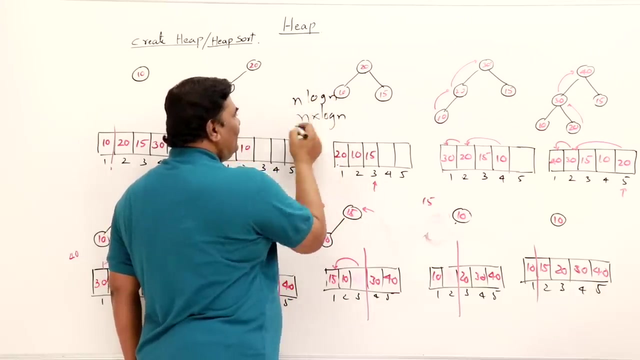 heap and login. now how much time does deleting of all any element is taking and elements we are deleting, and each element takes how much time for deletion? Also, it takes login time. We have already seen it. So that is n log n. So n log n for creation and login for deletion. 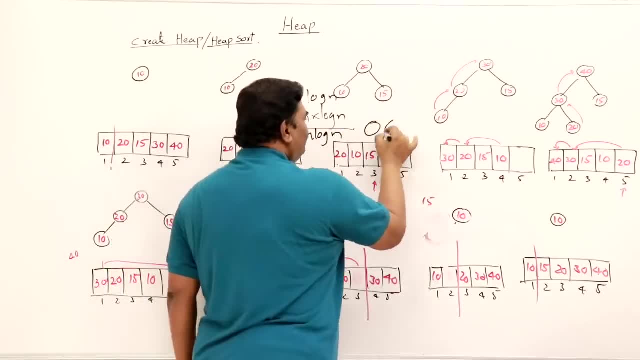 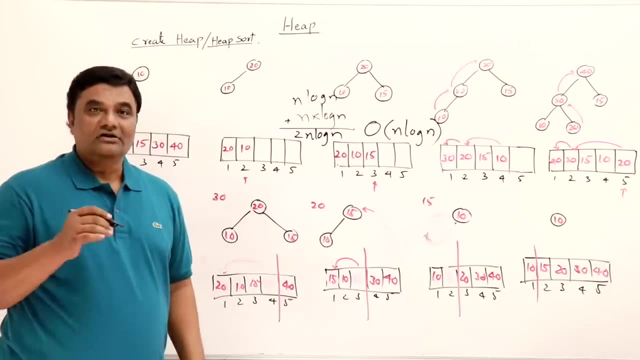 So total, how much to n log n and this is big O of n log n. right, Two times of log n is also dependent on n log n. So the time is order of n log n or big O of n log n. So heap sort takes n log n time. 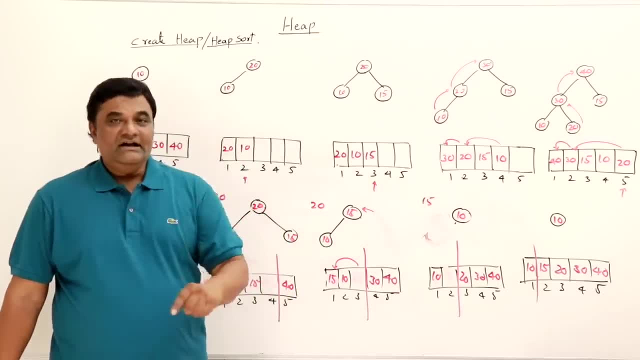 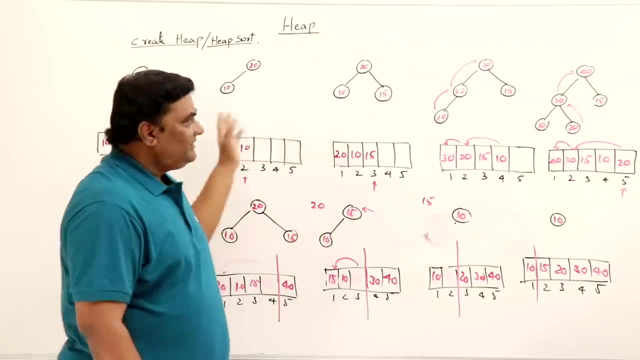 So that's it. This is heap sort. Now I have to explain you What is heapify, and heapify is a process of creating a heap. Already, we have created a heap. How it is different. It's different. How it is different, we will see. 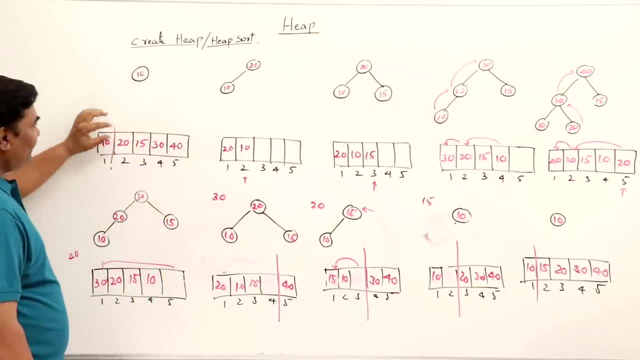 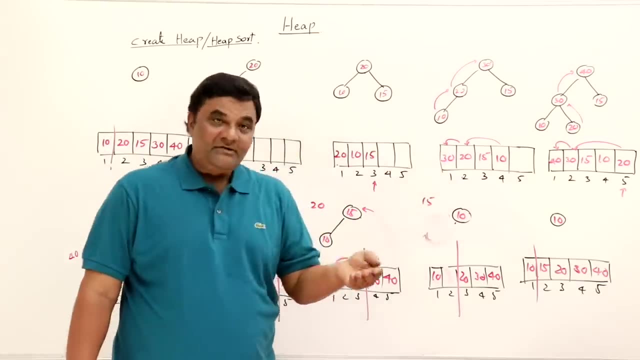 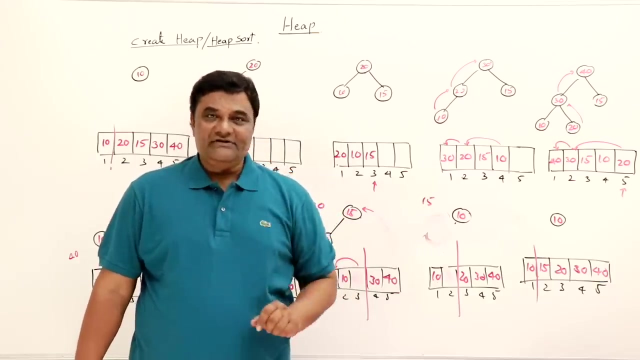 But before that, if you remember, here we were inserting the element always in the leaf and we were adjusting towards root. adjusting towards root, It was sent from leaf towards root. Adjustment was upward. Now in heapify the direction is different How it is done. 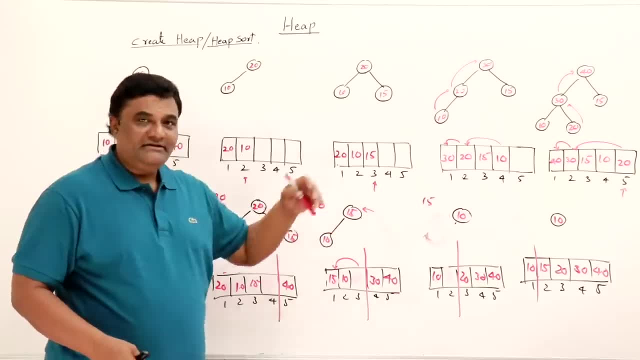 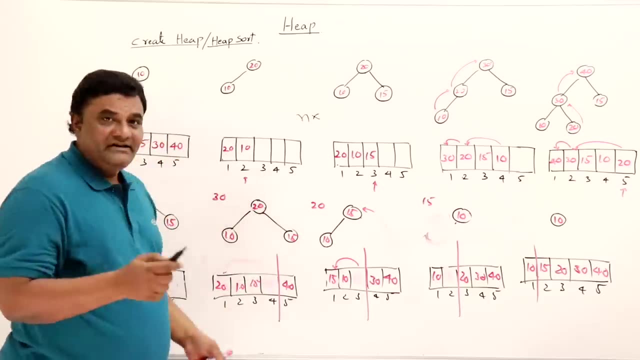 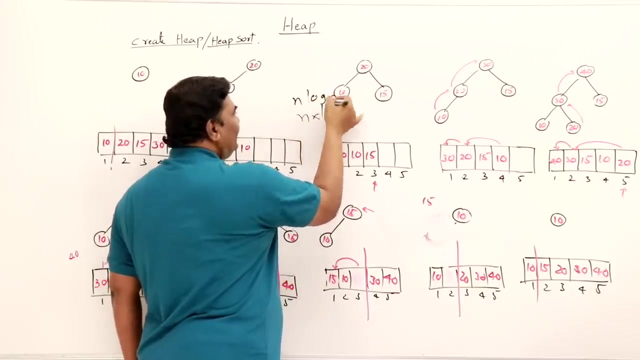 heap n log n now how much time this deleting of all any n element is taking. n elements we are deleting and each element takes how much time for deletion. also, it takes log n time. we have already seen it. so that is n log n. so n log n for creation, n log n for deletion, so total how much to n log n? 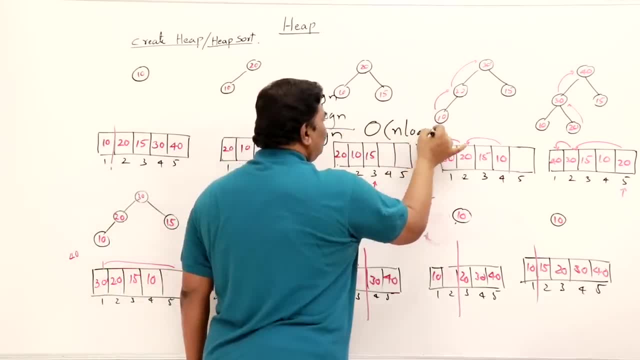 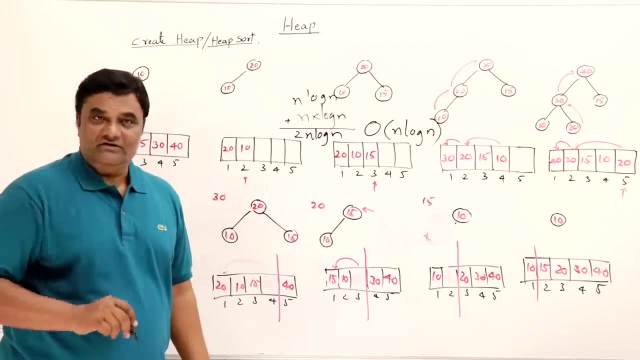 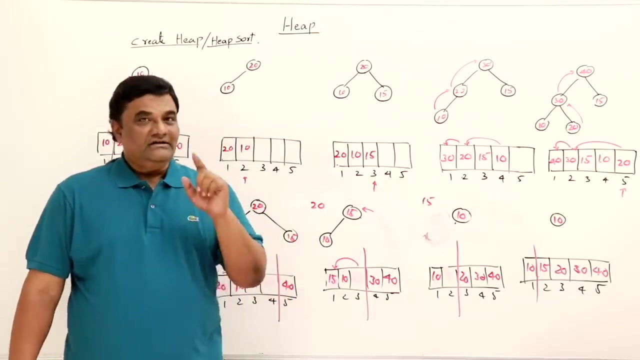 and this is b? o of n log n. right, two times of log n is also dependent on n log n. so the time is order of n log n or bo of n log n. so heap sort takes n log n time. so that is it. this is heap sort. now i have to. 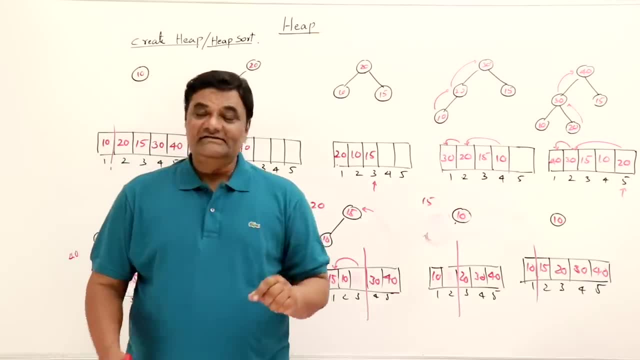 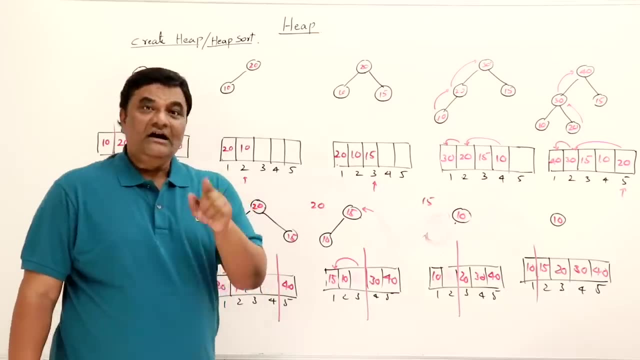 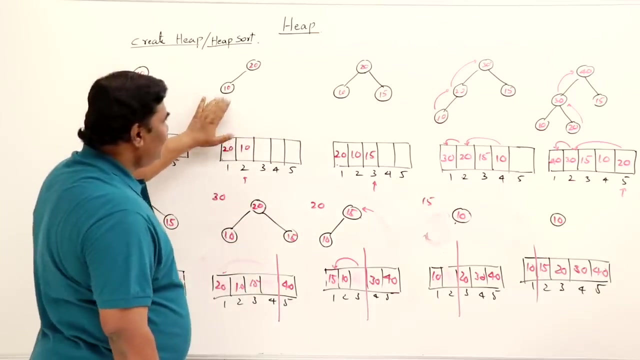 explain you heapify, and heapify is a process of creating a heap. already we have created a heap. how it is different it is different. how it is different we will see. but before that, if you remember, here we were inserting the element always in the leaf and we were adjusting towards root. 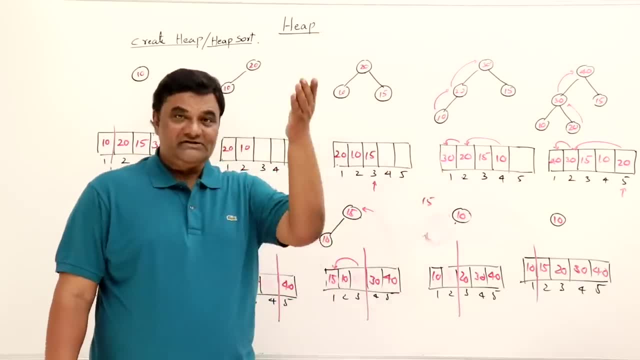 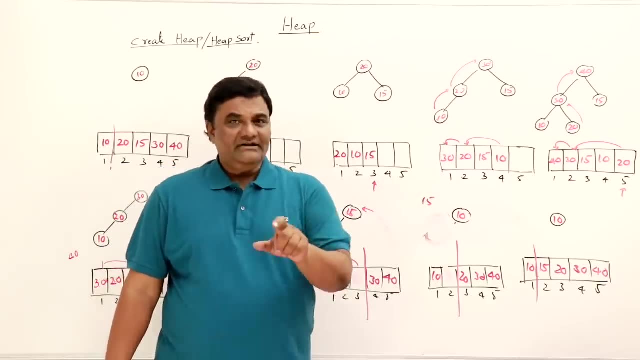 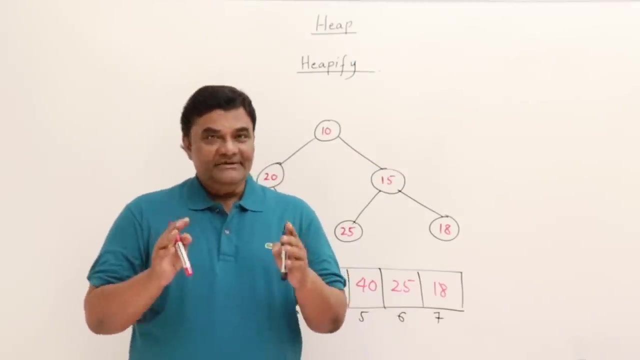 adjusting towards root. it was sent from leaf towards route. adjustment was upward. now in heapify the direction is different. how it is done, i'll show you. i'll remove this and show you now. next topic is heapify. heapify is a procedure for creating a heap. 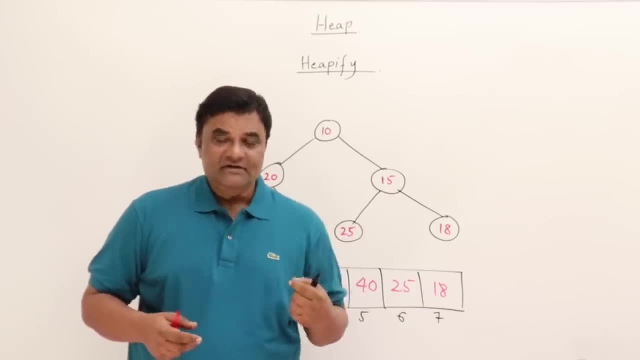 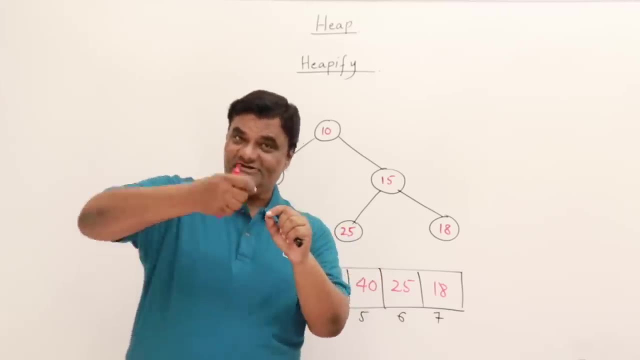 so already we saw how to create a heap by inserting elements one by one. here also we will do the same thing, but the procedure was inserting an element in the leaf and adjusting upwards. now let us see how heapify works. so for explaining heapify- already i have an 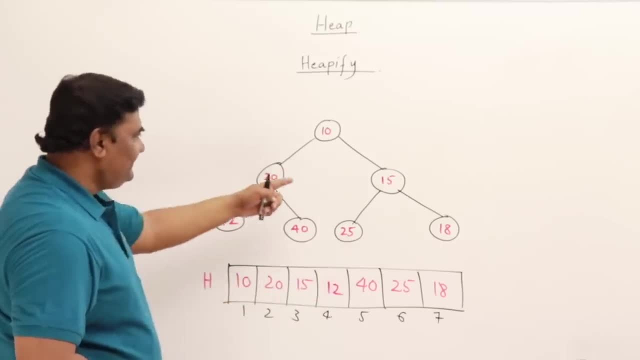 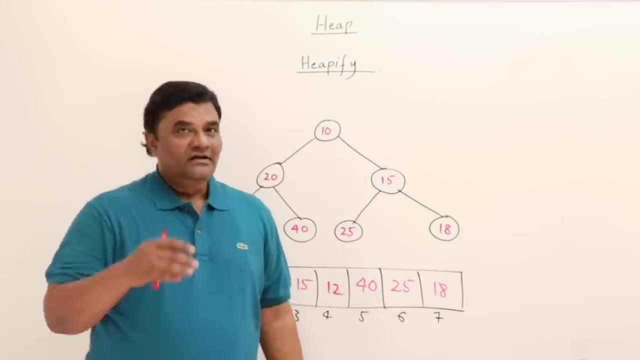 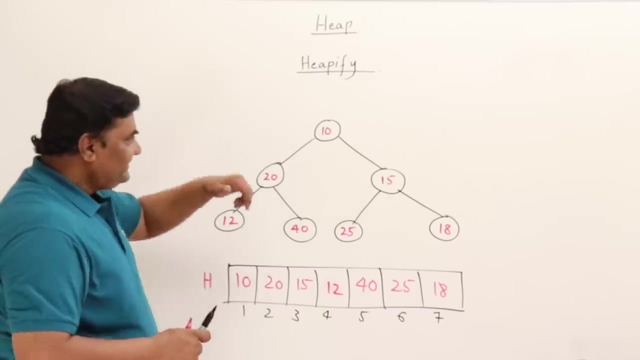 array right and if you see it diagrammatically, it is a binary tree and it's a complete binary, but it's not a max heap. we want max heap. now, if we just repeat the procedure of creation, let us look at it quickly. already we saw in creation process what we did. we kept 10 as it is inserted. 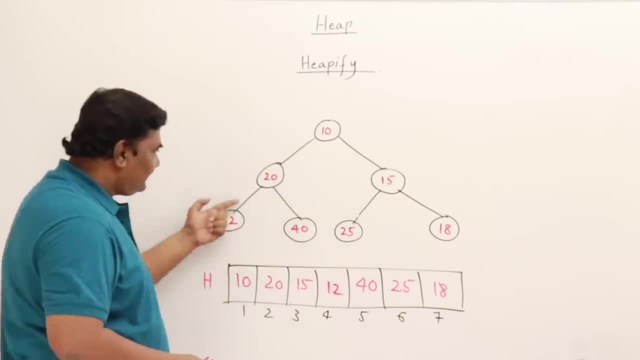 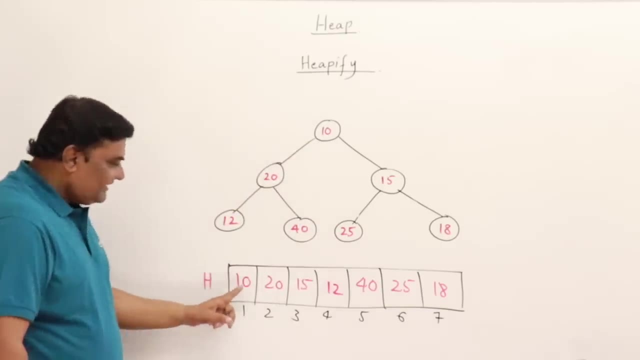 20, 20 went up, then inserted 15, then inserted 12, then 40, then 25, then 18, one by one. we inserted starting from this element. so we inserted except this element. we inserted 20, 15, 12, 40, 25, 18. 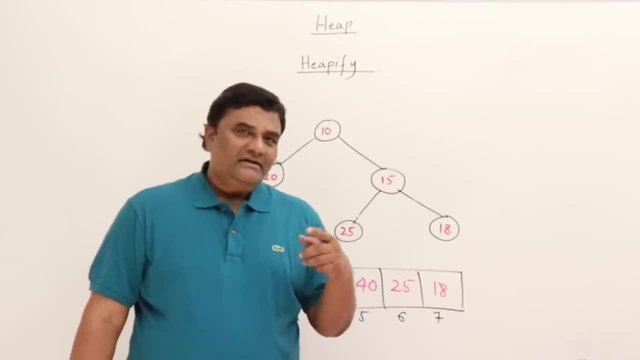 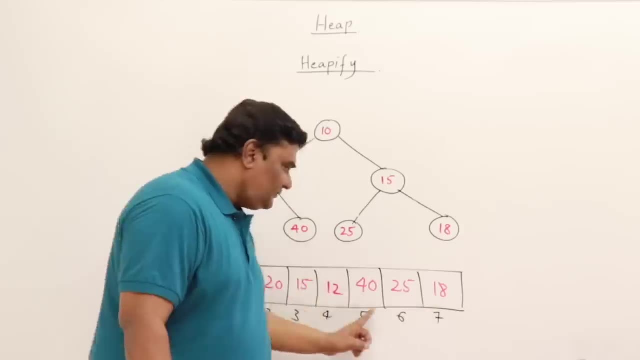 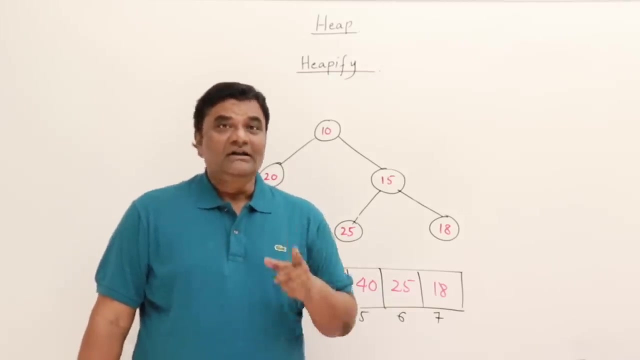 so we started from left to right. is it possible, if we change the direction, can we create a heap? let us start from right to left. so if we start from right to left, then shall we still adjust the element upward. no, let us do it downward, downward. how? in the deletion, if you remember, we were adjusting the element by sending. 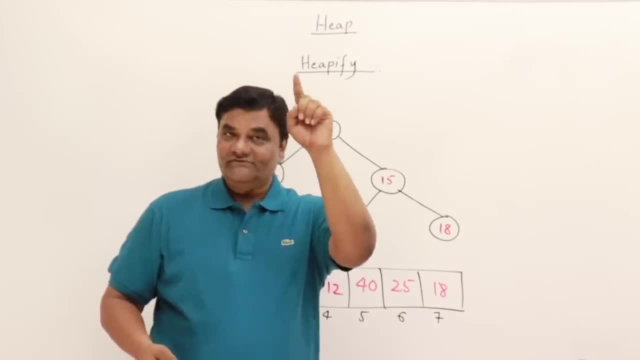 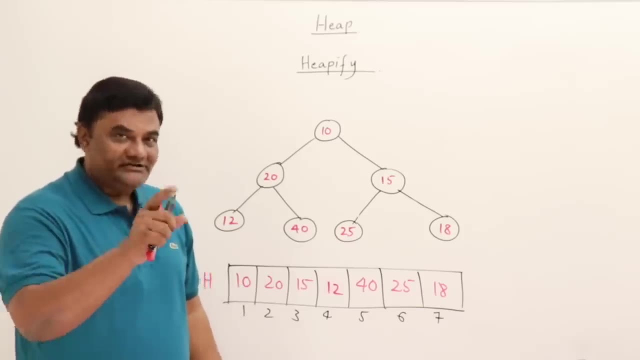 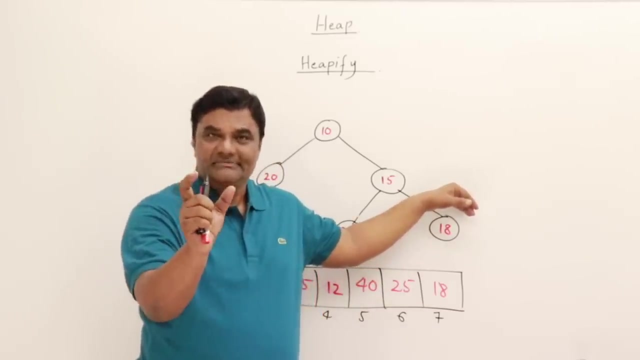 it down towards leaf from root, so the direction was from top towards leaf. that procedure will follow. let us follow the procedure now. i am explaining heapify. watch this first: go to element 18. look down: there are no children, so only a single element. don't look at all other nodes, just 18 and its descendants. there are no. 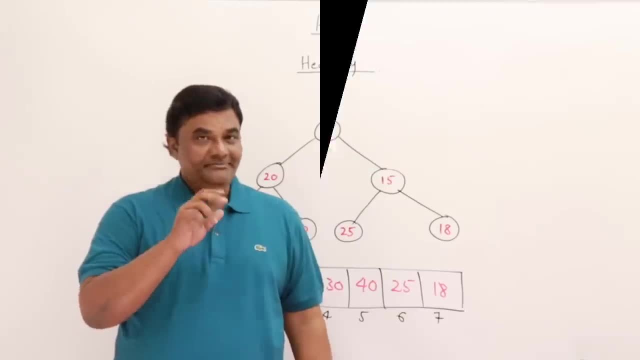 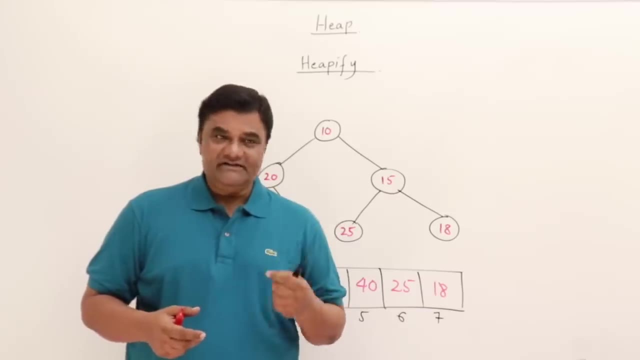 I will show you. I will remove this and show you. Now. heap: next topic is heapify. Heapify is a procedure for creating a heap. So already we saw how to create a heap by inserting elements one by one. Here also, we will do the same thing. 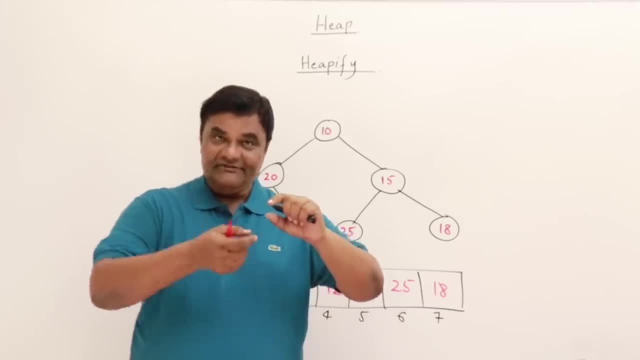 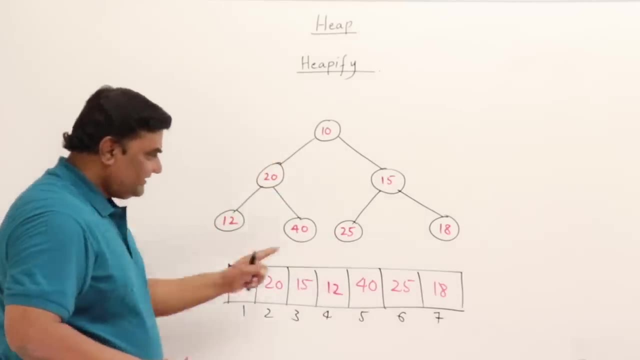 But the procedure was inserting an element in the leaf and adjusting upwards. Now let us see how heapify works. So for explaining heapify, already I have an array Right And if you see it diagrammatically, it is a binary tree and it's a complete binary tree. 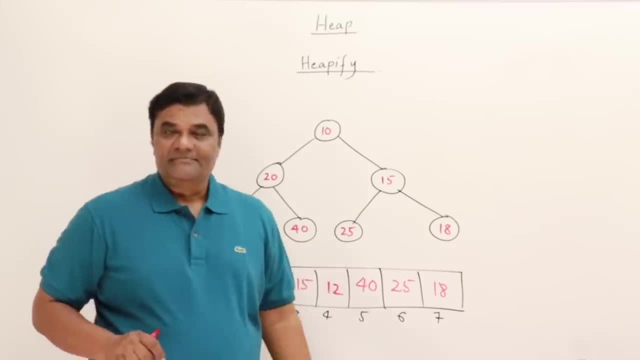 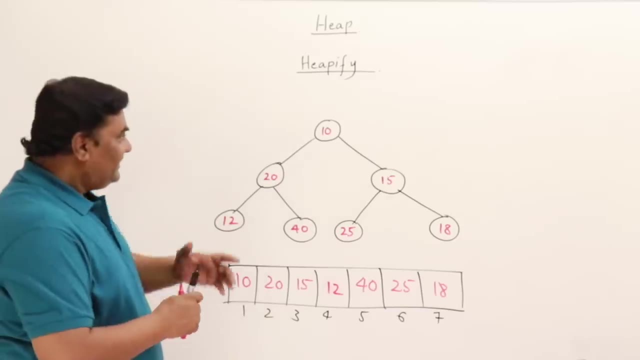 But it's not a max heap. We want max heap. Now, if we just repeat the procedure of creation, Let us look at it quickly. Already we saw in creation process what we did. We kept 10 as it is Inserted, 20. 20 went up. 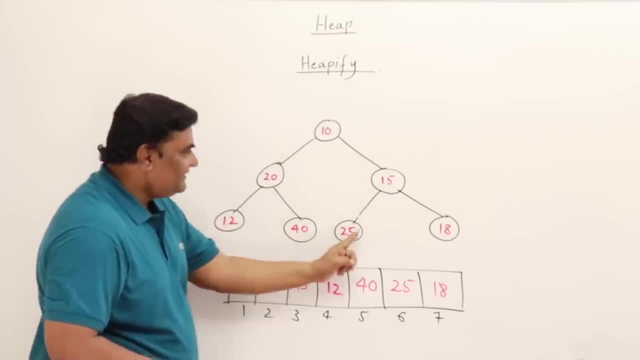 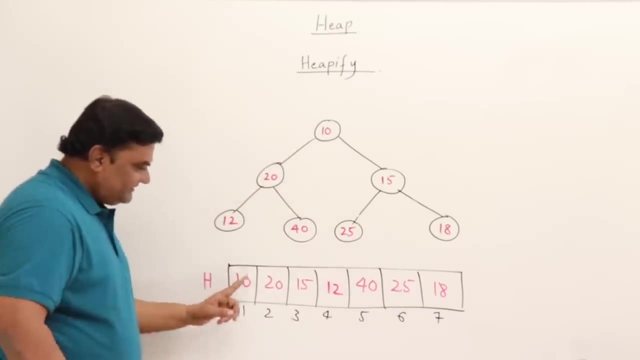 Then inserted 15.. Then inserted 12., Then 40., Then 35., Then 18.. One by one we inserted, starting from this element. So we inserted except this element. we inserted 20,, 15,, 12,, 40,, 25,, 18.. 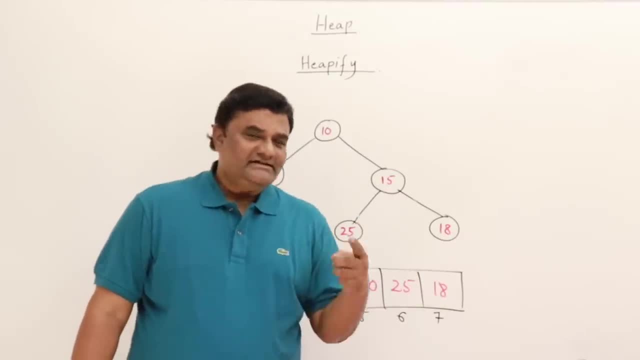 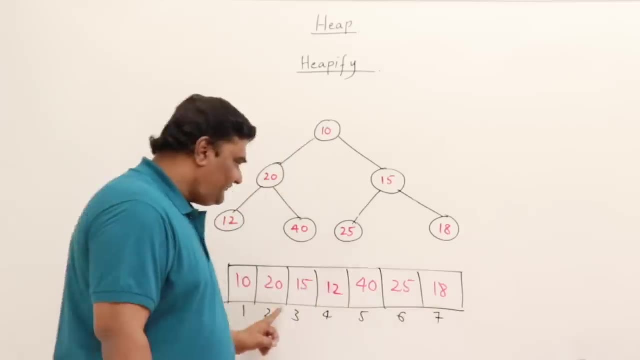 So we started from left to right. Is it possible, if we change the direction, can we create a heap? Let us start from right to left. So if we start from right to left, then shall we still adjust the element upward. No, Let us do it downward. 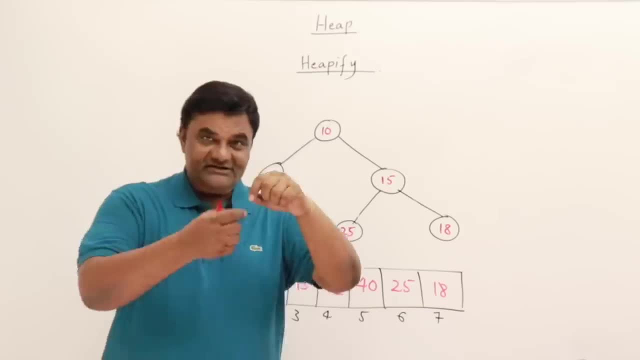 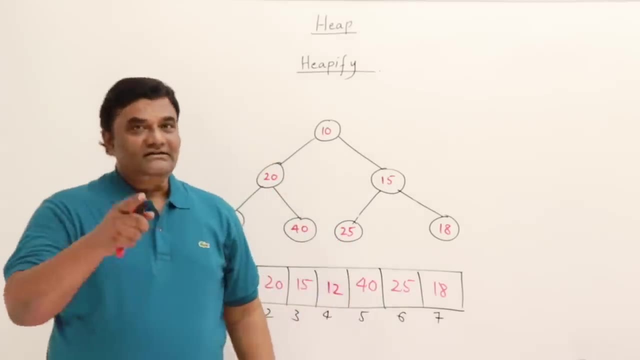 Downward. how? In the deletion, if you remember, we were adjusting the element by sending it down towards leaf, from root, so the direction was from top towards leaf. That procedure will follow. Let us follow the procedure Now. I am explaining heapify, Watch this. 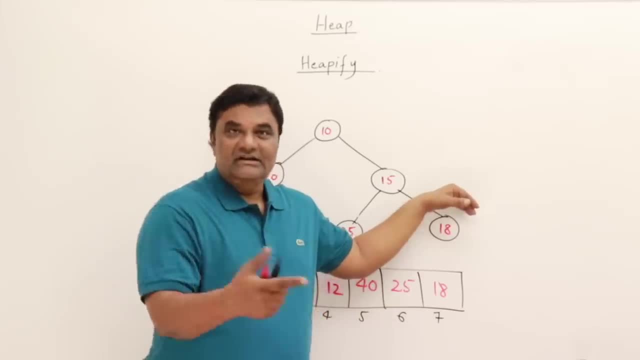 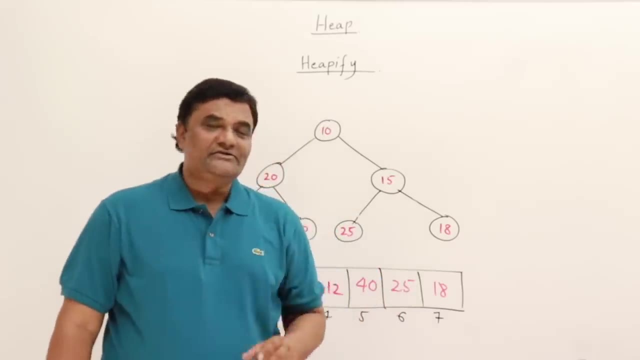 First go to element 18.. Look down: There are no children, So only a single element. Don't look at all other nodes, Just 18 and its descendants. There are no descendants, So 18 is a heap. Yes, Then go to next element 25.. 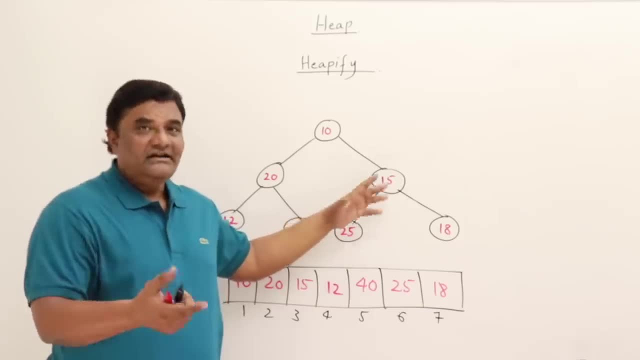 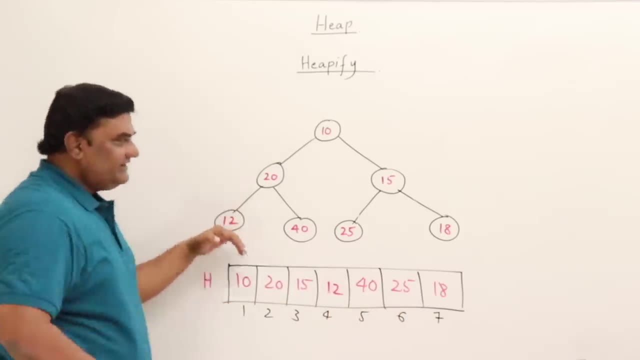 25.. Look downwards: It's a heap. There is nothing. There are no children, It's alone, It's a heap. 40 is a heap. Next element: 40.. Next element: 12.. Downwards, It's a heap. 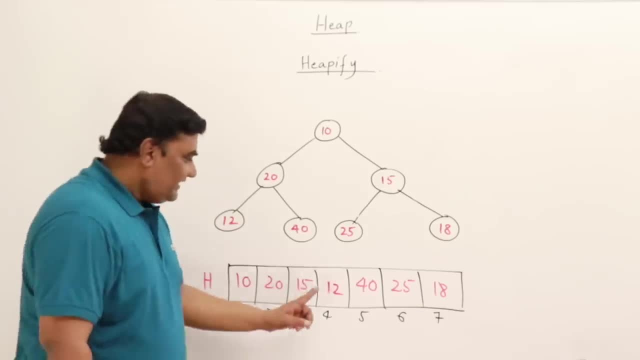 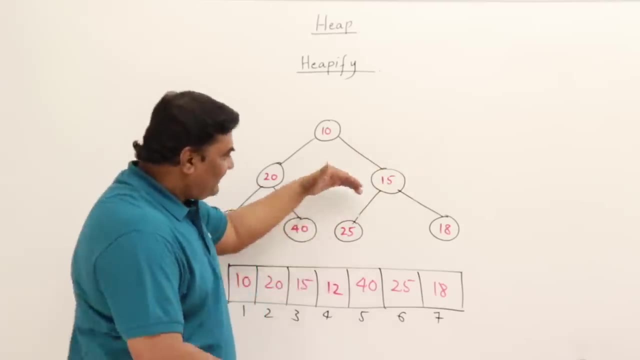 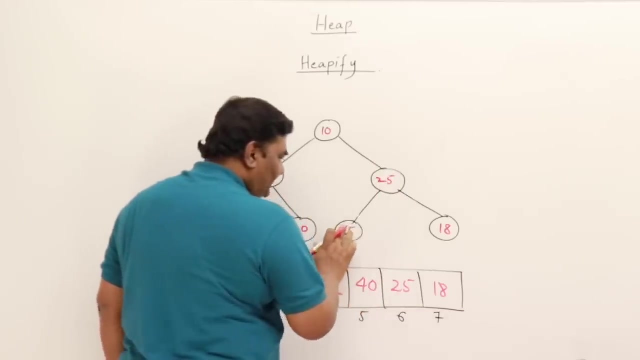 Now you will understand. what does it mean, What I was saying Just next. Next element: 15.. So from here, adjust 15 downwards. Yes, Children are there. Compare Which is greater: 25. So 25 will go up and 15 will come down. 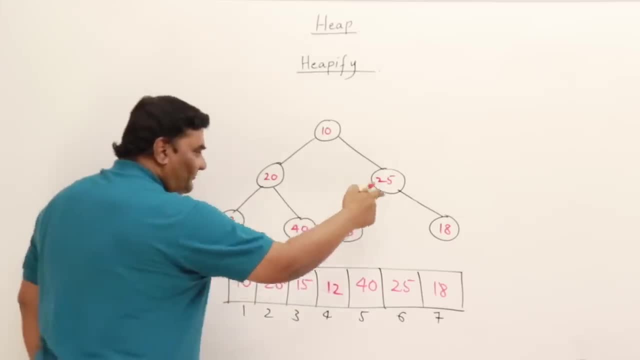 Yes, This is the procedure. 25 will go up and 15 will come down. So 25 will go up and 15 will come in its place. This one Right. So if you look, only these nodes: 25, 15 and 18.. 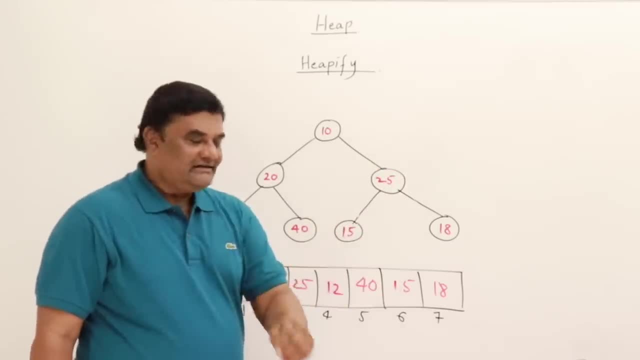 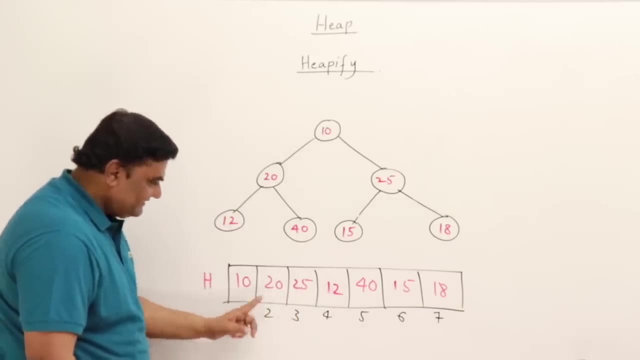 It's a heap. Yes, Only one element I have adjusted Now next, after 25, this one: 20 is there. This is over. Right, 15 was there. This is over. Now we are on second element: Right, This one. Look downwards. 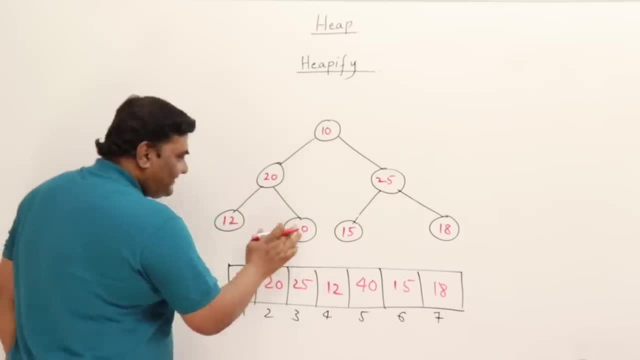 Is it a max heap? No, Adjust this one. So compare with the children. 40 is greater, So 20 will come here. 40 will go up Right, So 40. This will be changed to 20 and this will become 40.. 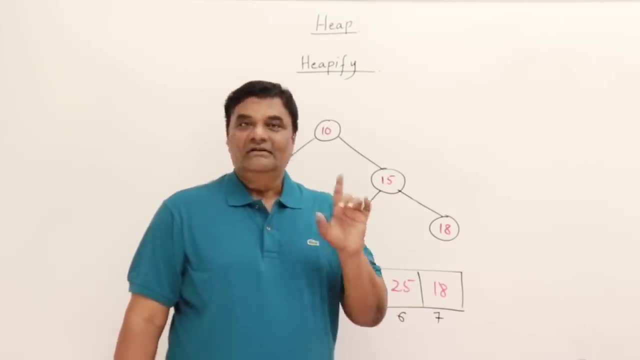 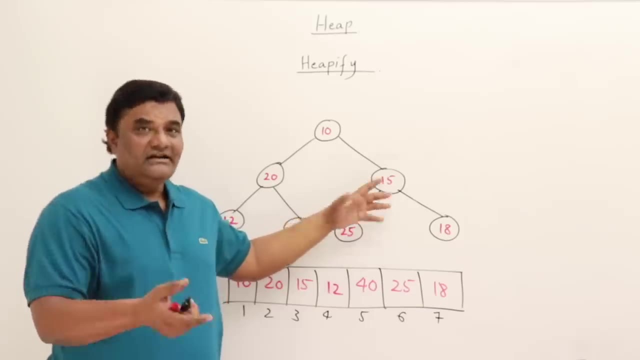 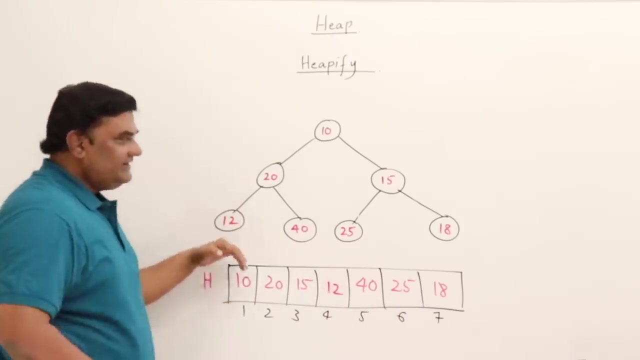 descendants. so 18 is a heap. yes, then go to next element, 25: 25. look downwards. it's a heap. there is nothing, there are no children, it's alone. it's a heap. 40 is a heap. next element: 40. next element: 12 downwards: it's a heap. now you will understand what does it mean what i was saying just next. 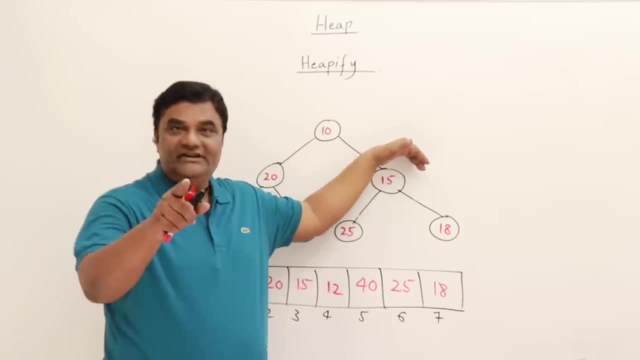 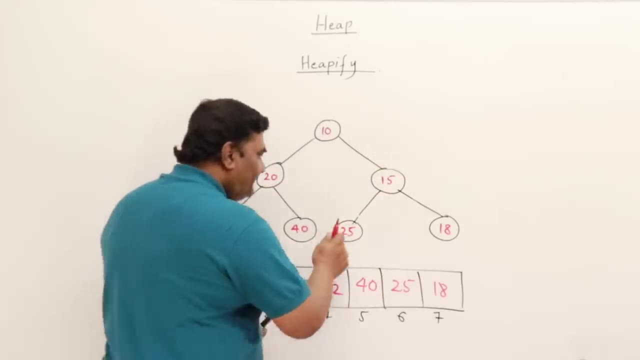 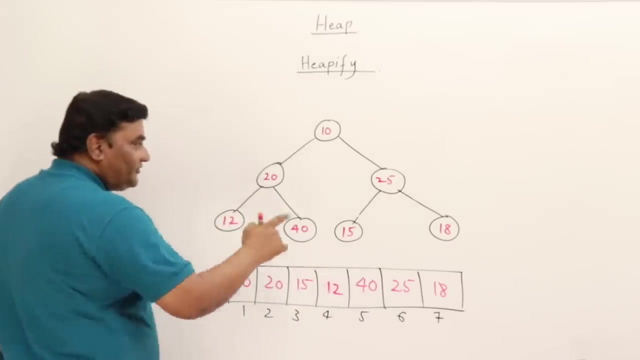 next element: 15. so from here i just 15 downwards. yes, children are there? compare which is greater: 25. so 25 will go up and 15 will come down. yes, this is the procedure: 25 will go up and 15 will come down. so 25 will go up and 15 will. 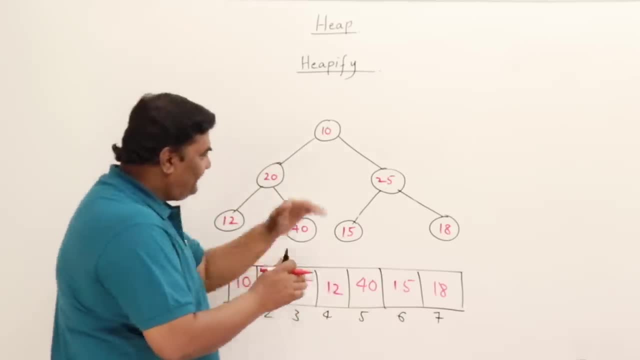 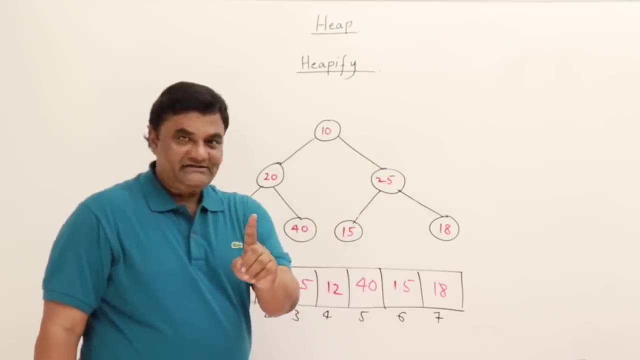 come in its place. this one right. so if you look only these nodes- 25, 15 and 18- it's a heap. yes, only adjusted now. next, after 25: this one: 20 is there. this is over right. 15 was there. this is over now. 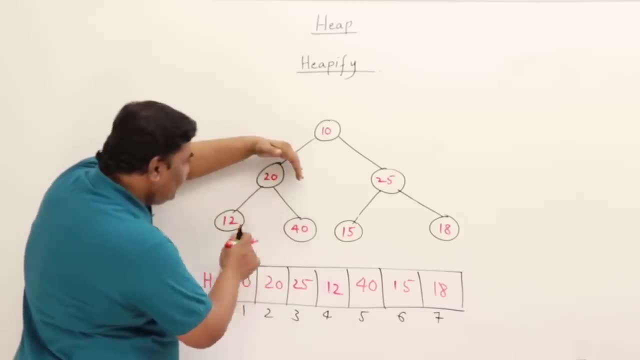 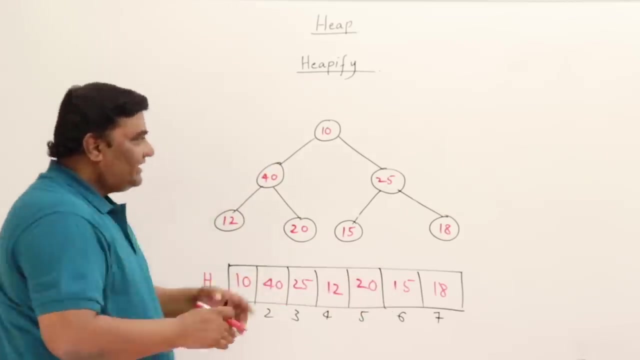 we are on second element. right, this one? look downwards. is it a max heap? no, adjust this one. so compare with the children. 40 is greater, so 20 will come here. 40 will go up, right, so 40. this will be changed to 20 and this will become 40. so i have just adjusted just two elements now, after second. 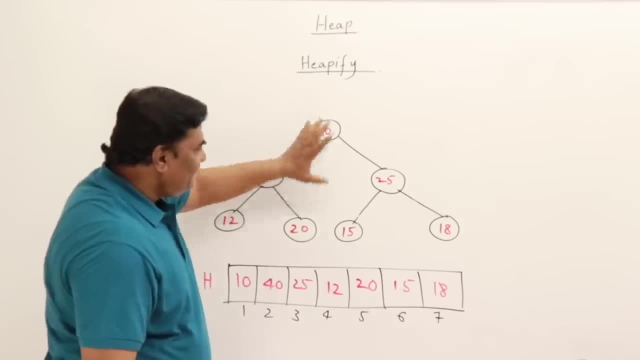 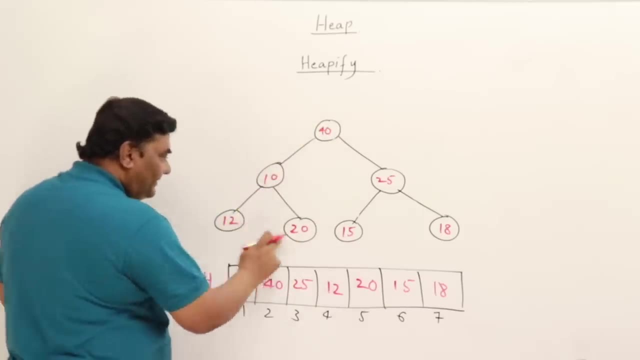 element. first element here. only this element is not in a heap, so adjust it. compare with the children: 40 is greater, so 40 goes up. 10 comes here. compare with the children: 20 is greater, so 20 goes up. 10 comes here. right, so this will be swapped with the child, so this will become 40 and this. 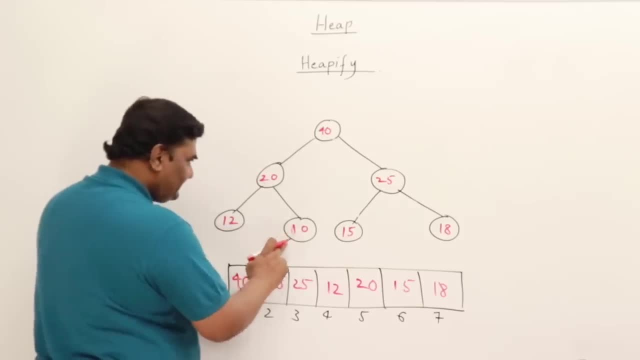 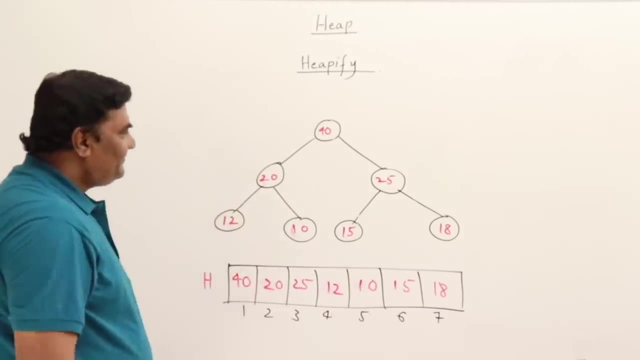 is 10, then again swap with the children. that is 20 and 10, 20. sorry, 12 and 20 was there, so it will be swapped with 20 and this comes here. this is a here heap, so we adjusted the elements downwards and we started from the last element. so we have scanned. 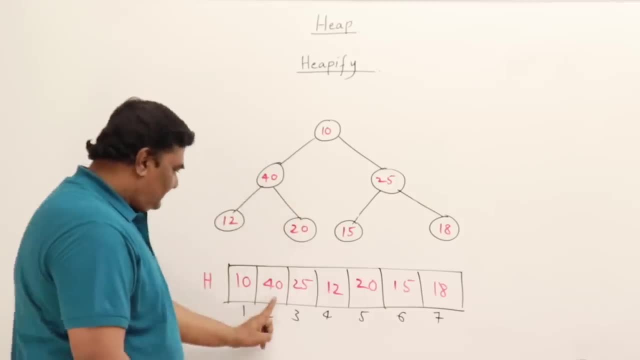 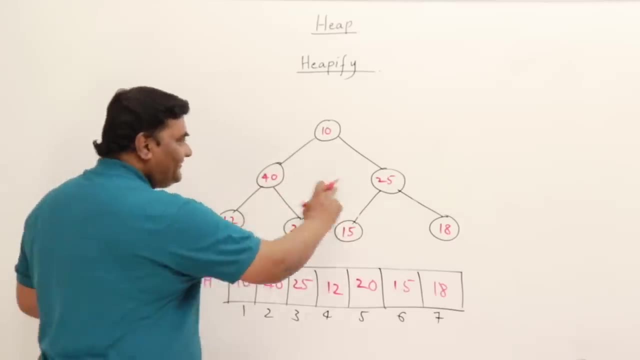 So I have adjusted just two elements Now after second element. first element here Only this element is not in a heap, So adjust it. Compare with the children: 40 is greater, So 40 goes up, 10 comes here. 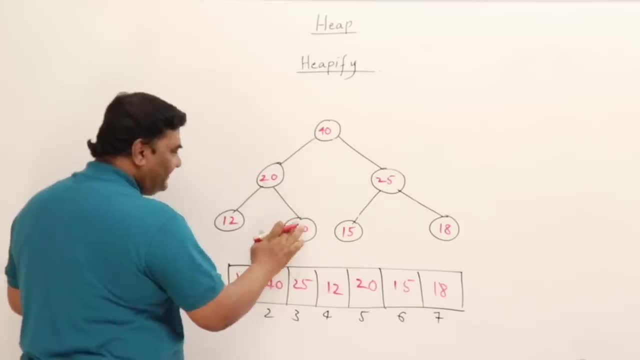 Compare with the children: 20 is greater, So 20 goes up. 10 comes here, Right, So this will be swapped with the child, So this will become 40. 10.. Then again swap with the children. That is 20 and 10, sorry, 12 and 20 was there. 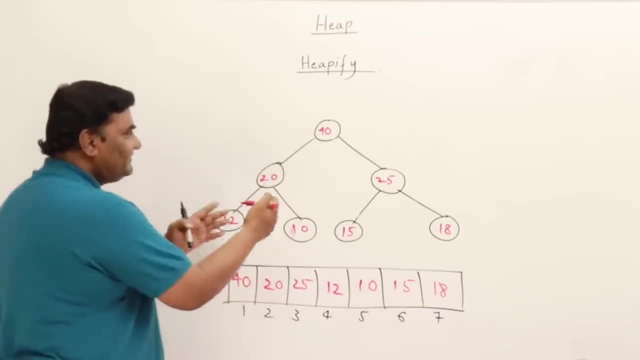 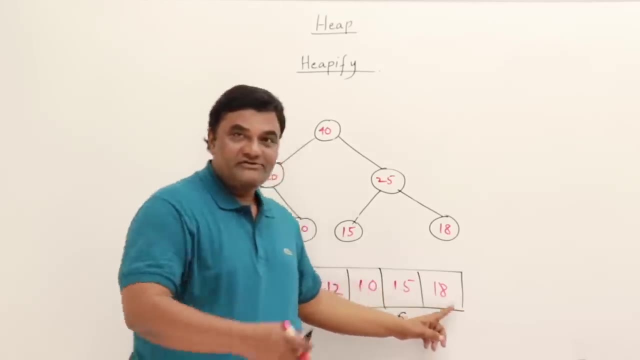 So it will be swapped with 20 and this comes here. This is a heap, So we adjusted the elements downwards and we started from the last element. So we have scanned this array from right to left, The procedure we were using in the deletion. 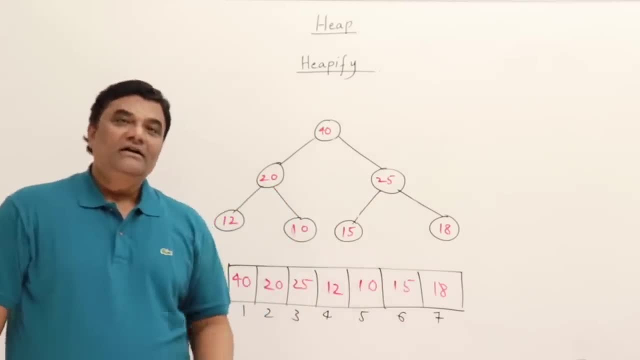 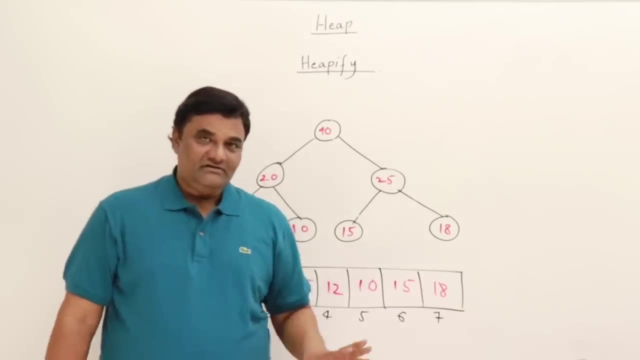 After deletion, we were adjusting the elements. Same procedure we followed and we got the heap created. So this procedure is called as heapify. Right Direction is different, That's all Right. And what's the time taken by this one? 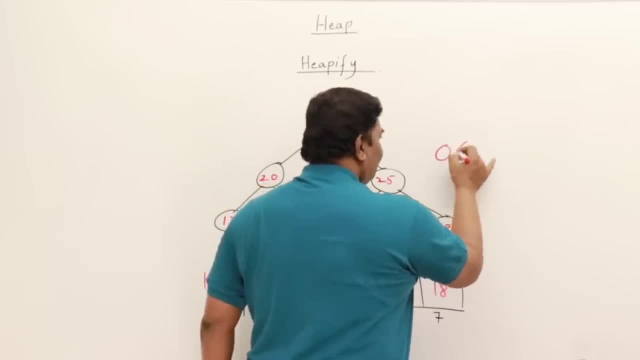 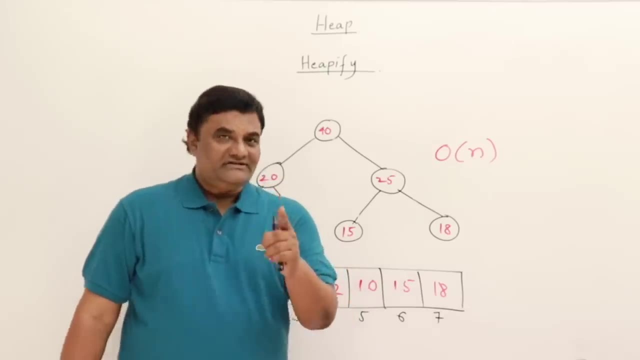 Analytically, the time taken by this heapify procedure is big O of n, Big O theta, omega, whatever you want. Notation, you use anything, commonly we use big O, So this is big O of n. So if you remember the procedure for creating a heap, creating a heap. 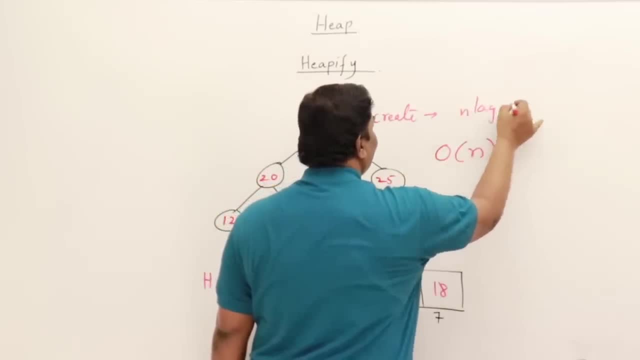 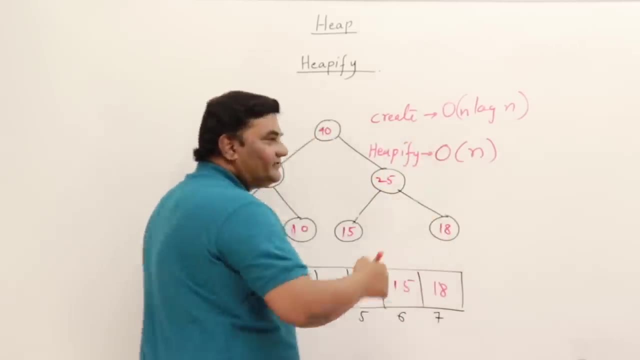 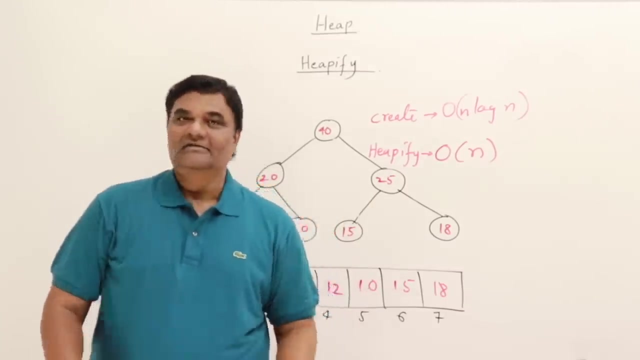 So creating a heap was analog n big O of n log n Right, But this is heapify. Heapify procedure is order of n, So this is faster. Now, what is the minimum time taken for creating a heap- Big O of n using heapify? 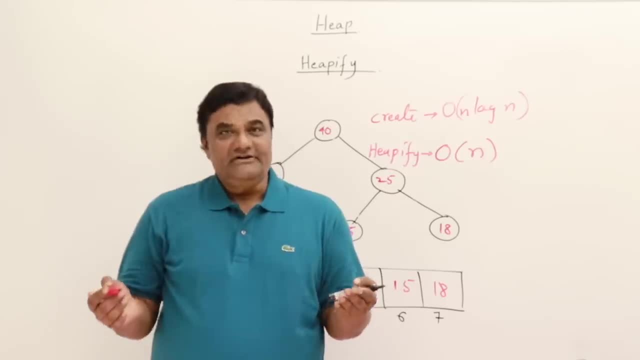 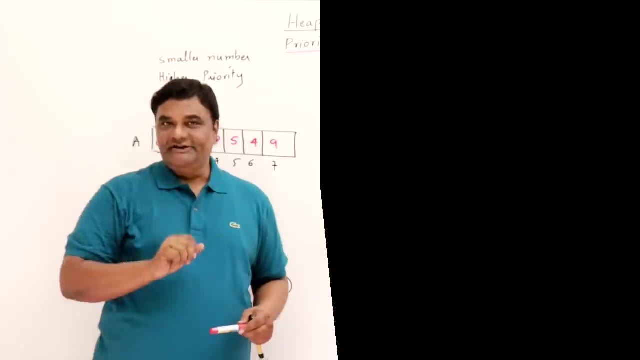 So that's all about heapify. Now, the last thing is: what are priority queues? It's a simple topic, So I will finish with that one. Next we will see priority queues. Now, priority queue, Priority queue. So actually queue means FIFO. 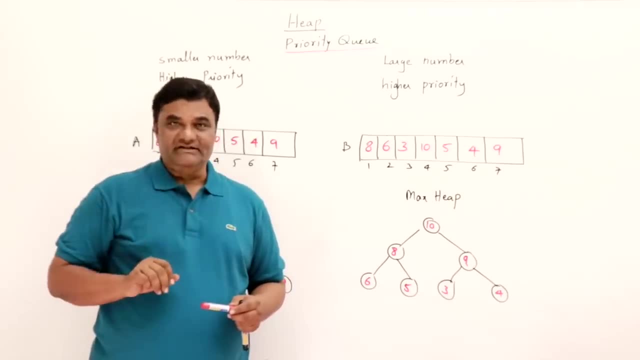 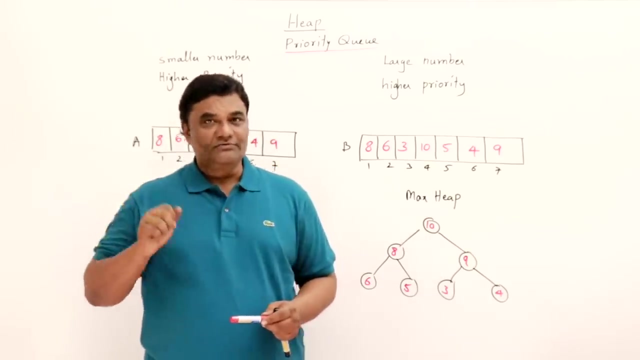 But priority queues For humans. it's not FIFO strictly. The elements will have priority and they are inserted and deleted based on the priority Right. So always if in a queue when you want to delete, always we want highest priority element from the queue. 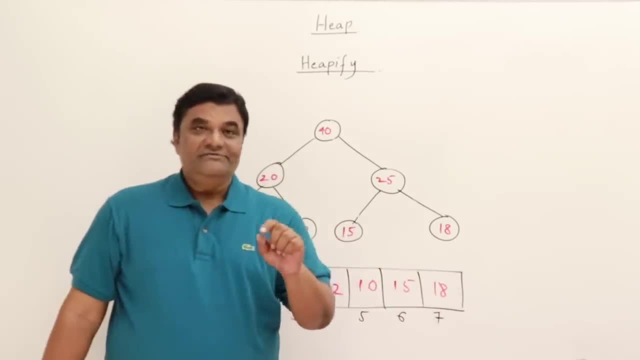 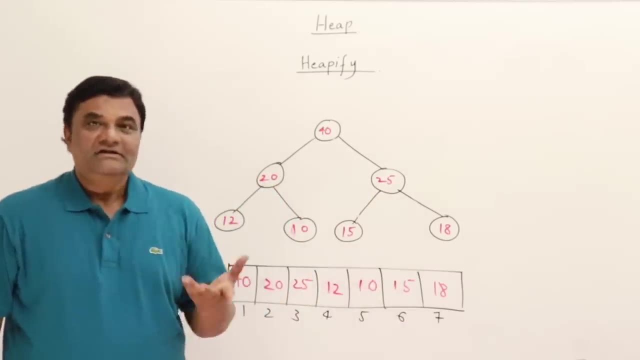 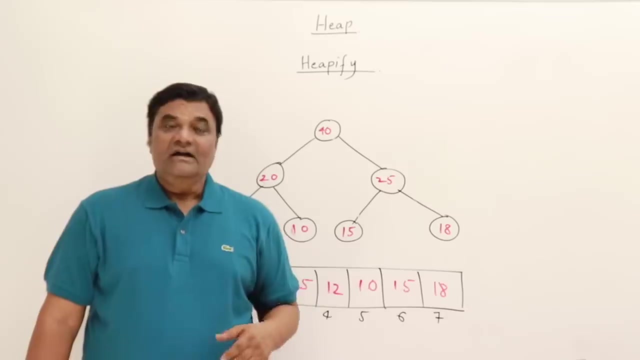 this array from right to left, the procedure we were using in deletion. after deletion we were adjusting the element. same procedure we followed and we got the heap created. so this procedure is called as heapify. right direction is different, that's all right. and what's the time taken by? 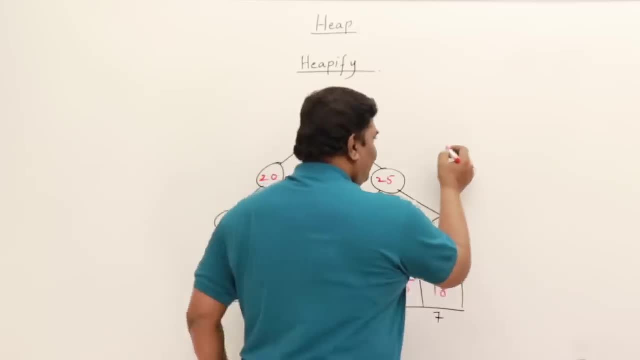 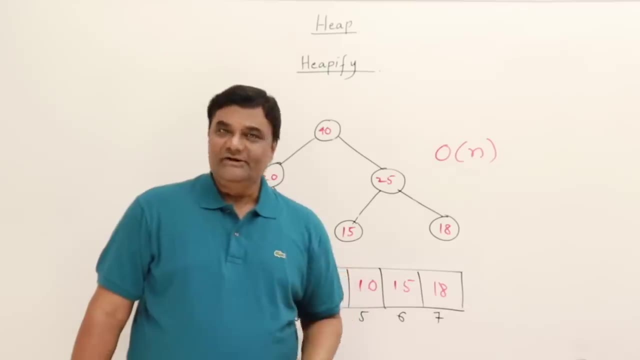 this one. analytically, the time taken by this heapify procedure is bigo of n, bigo theta, omega, whatever you want notation you use anything commonly we use bigo. so this is bigo of n. so if you remember the procedure for creating a heap, 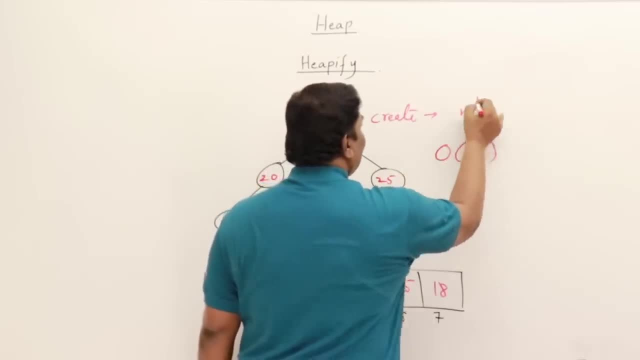 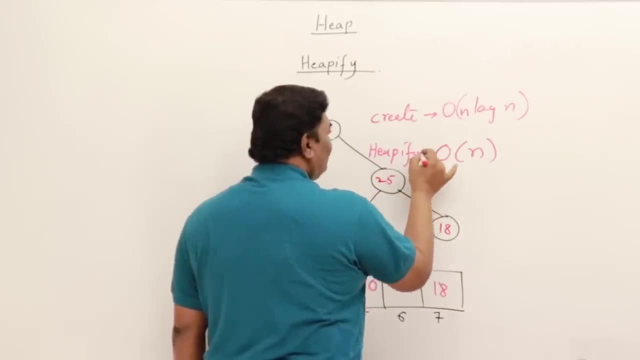 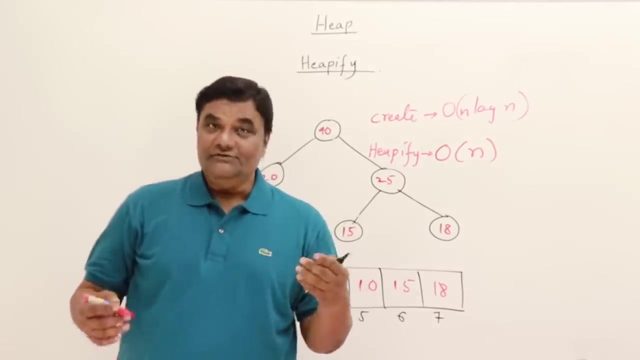 creating a heap. so creating a heap was analog n bigo of n log and right, but this is heapify. heapify procedure is order of n, so this is faster. now, what is the minimum time taken for creating a heap? go of n using heapify. so that's all about heapify. now the last thing is: what are priority queues? 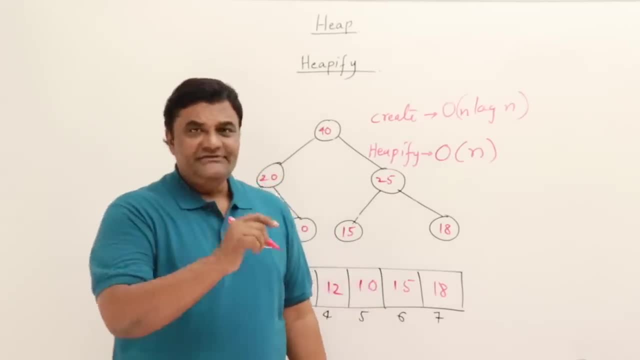 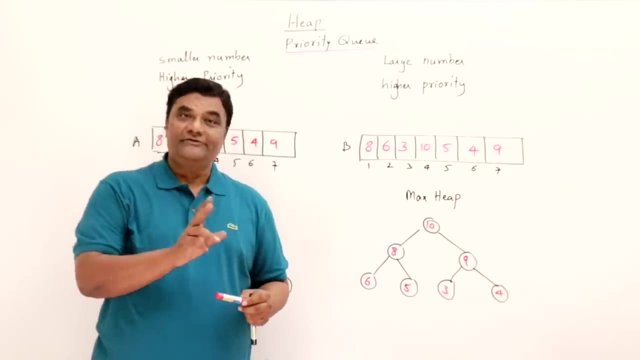 it's a simple topic, so i will finish with that one. next we will see priority queues now, priority queue, priority queue. so actually queue means fifo, but priority queue means it's not fifo strictly. the elements will have priority and they are inserted and deleted based on the priority. 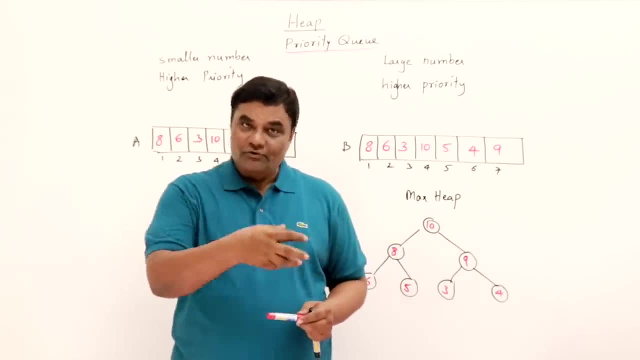 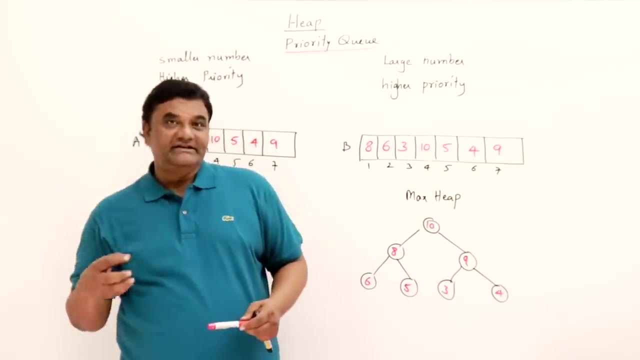 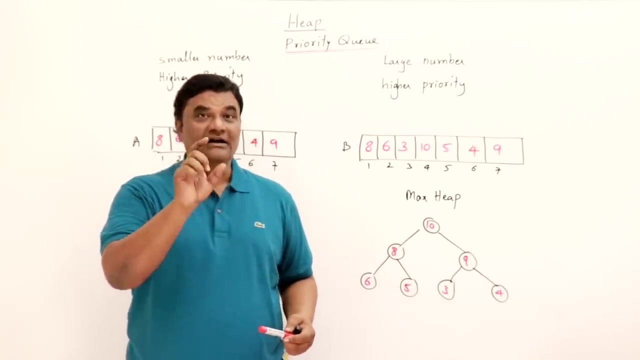 right. so always if in a queue when you want to delete, always we want highest priority element from the queue, the element having the highest priority, that should be deleted first. so this is the discipline of priority: queue elements are inserted with their priority. when you delete, we want higher priority element. so let us see what does it mean by higher priority? 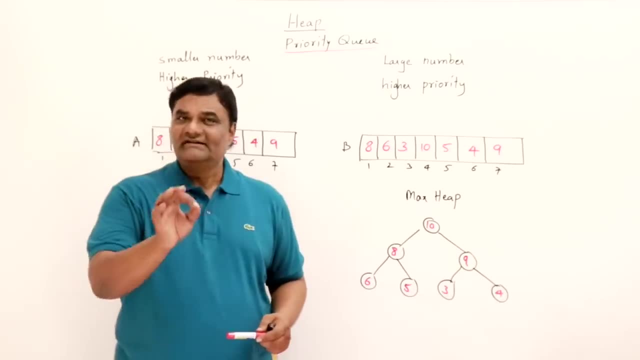 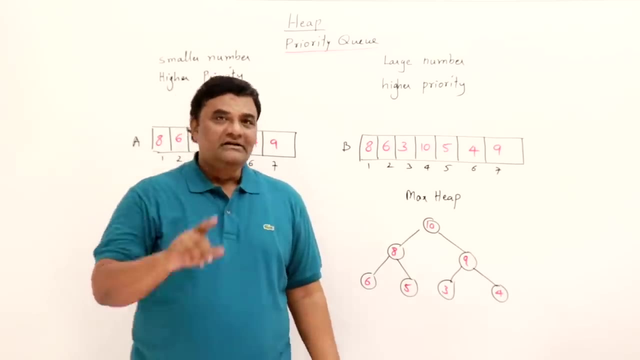 The element having the highest priority that should be deleted first. So this is the discipline of priority queue: Elements are inserted with their priority When you delete. we want higher priority element. So let us see what does it mean by higher priority? See, these are the numbers. 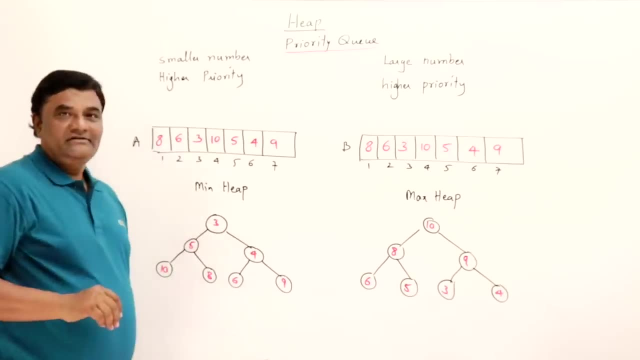 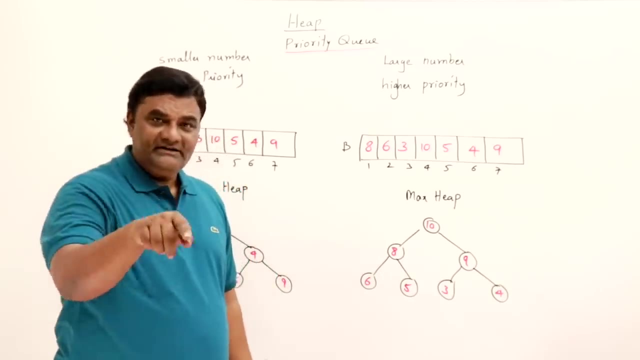 What is the priority of a number? Number itself is the priority. OK, here in our example, number itself is the priority. There are other examples of priority queues, also, like in operating system Also there is a concept of priority queue. 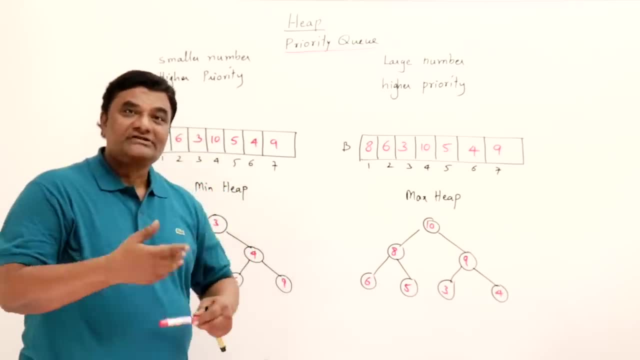 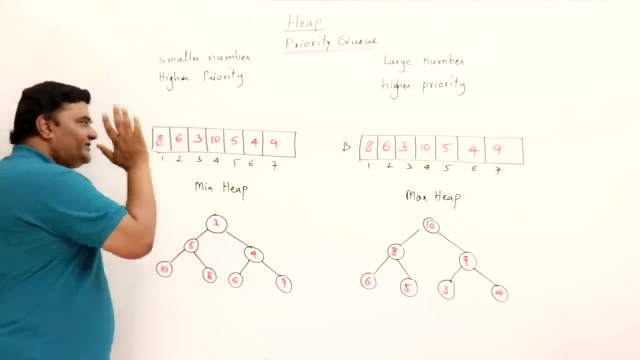 It is not the same as that one. This priority queue is mostly used in algorithms, So let us see what is the priority: Eight is the priority of eight. Six is the priority of six. So ten is the priority of ten, So that number itself is the priority. 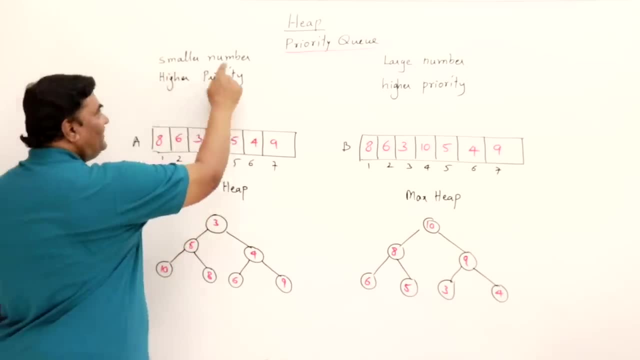 Then who is higher priority? I can say that smaller number, higher priority. So which is highest priority? This one, then this one, then this one. Yes, smaller the number, higher the priority. So three is of highest priority here. 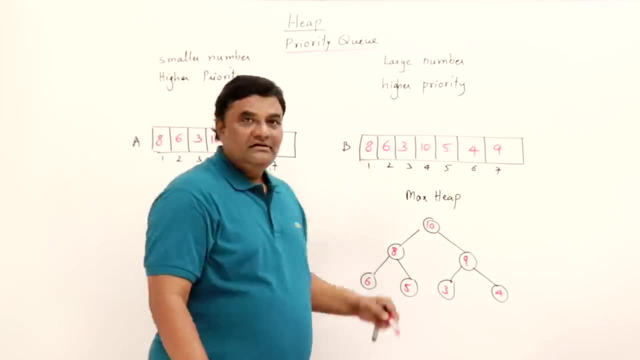 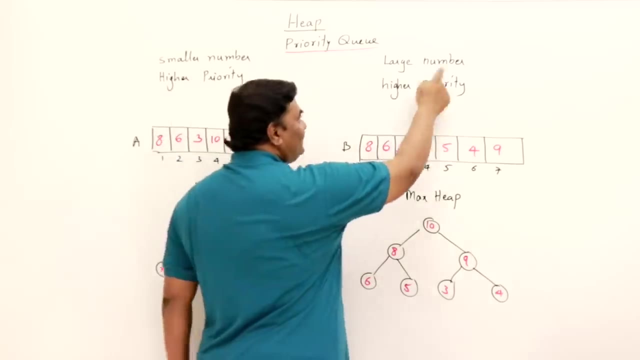 So if I delete, I want three from the array. Then otherwise even I can say that larger the number, higher priority. I can say this also. So larger number, higher priority. So who is having higher priority? Then nine, then eight. 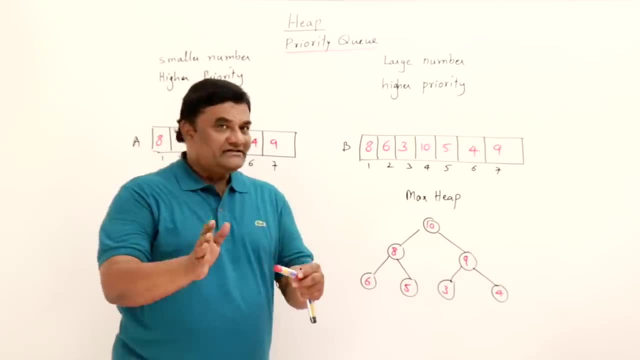 So, yes, when I want delete, I should get ten from that one. So this is about priority queue Elements. they value itself as priority And there are two methods of giving priority: Smaller number- higher priority or larger number- higher priority. 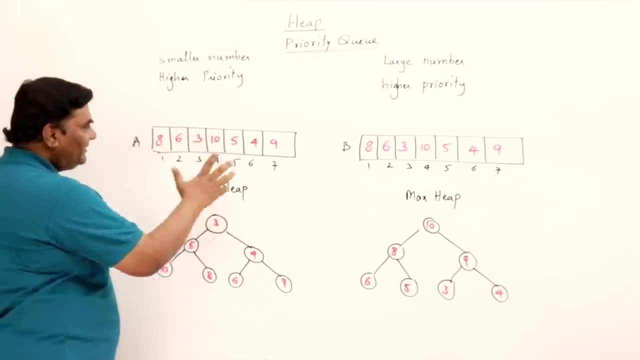 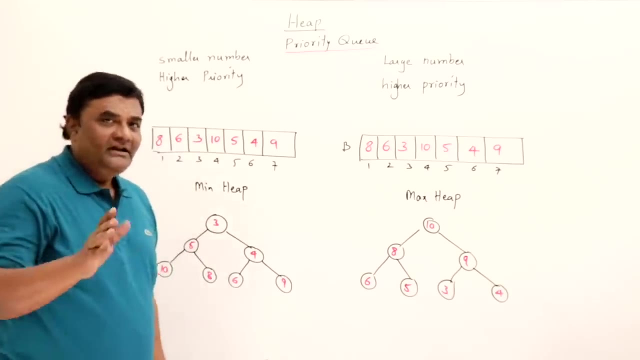 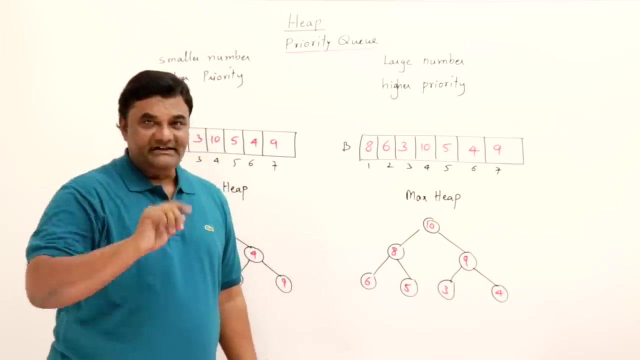 see, these are the numbers. what is the priority of a number? number itself is the priority. okay, here in our example, number itself is the priority. there are other example of priority queues also, like in operating system also, there is a concept of priority queue. it is not same as that one. this: 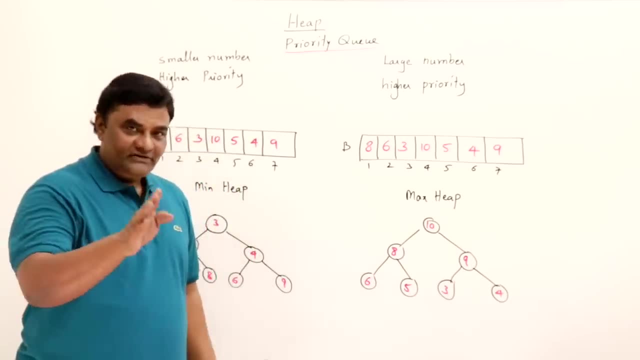 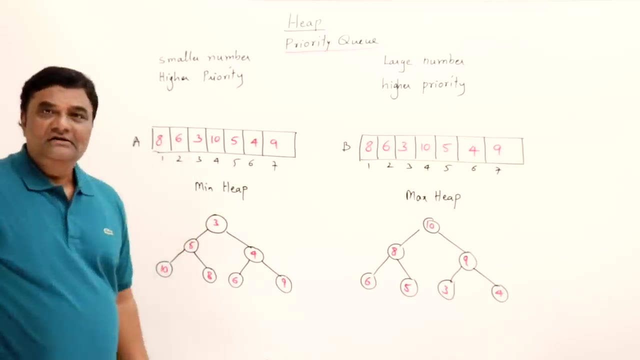 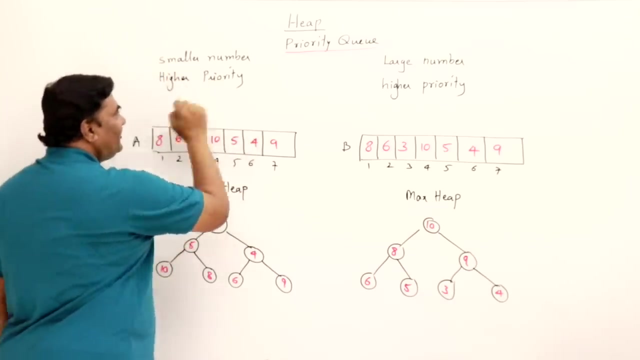 priority queue is mostly used in algorithms, right? so let us see what is the priority: eight is the priority of eight, six is the priority of six. so ten is the priority of ten, so that number itself is the priority. then who is higher priority? i can say that smaller number higher priority. so which? 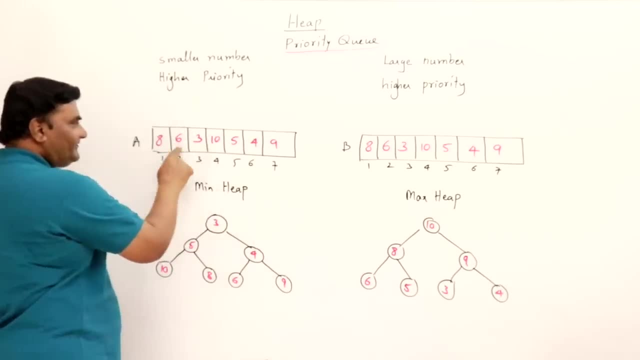 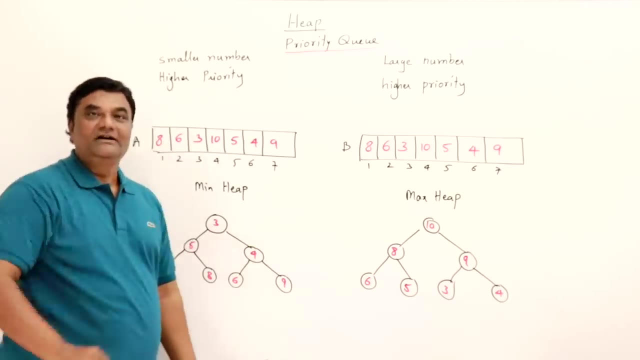 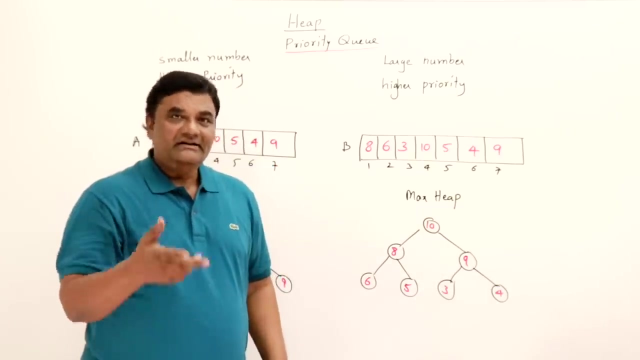 is highest priority: this one, then this one, right, then this one. yes, smaller the number, higher the priority. so three is of highest priority here. so if i delete i want three from the array, then otherwise even i can say that larger the number, higher priority. i can say this also. so larger number, higher priority. so who is having? 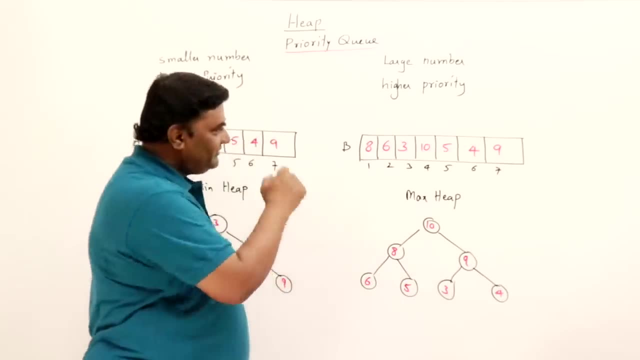 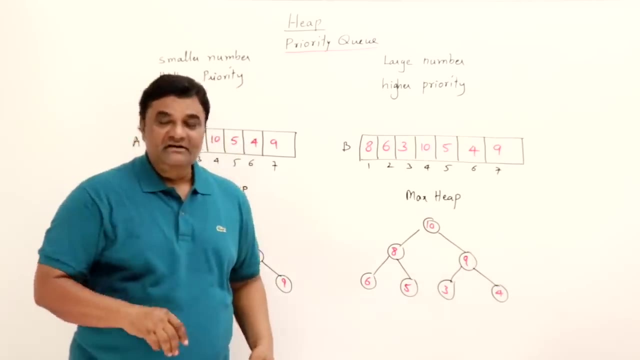 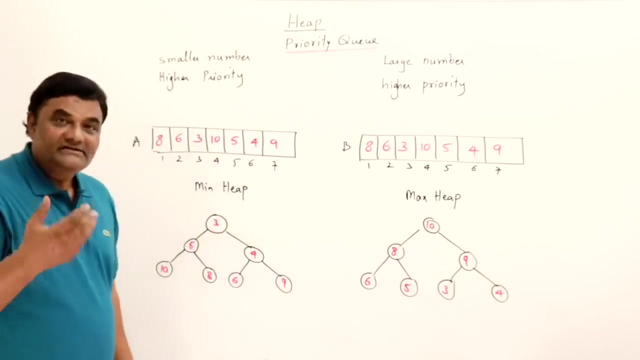 higher priority, ten, then nine, then eight. so yes, when i want delete, i should get ten from that one. so this is about priority queue elements. they value itself priority and there are two methods of giving priority: smaller number, higher priority or larger number- higher priority. okay, now let us see how to insert and delete. see in an array if i want to. 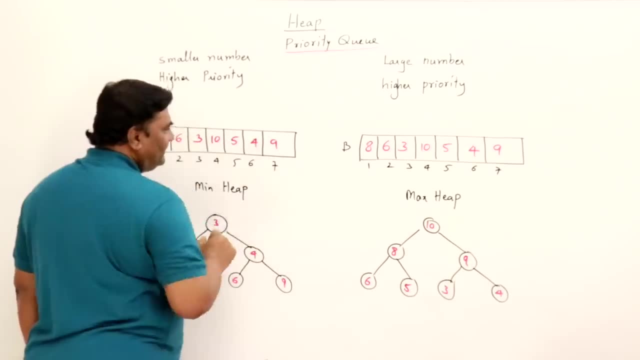 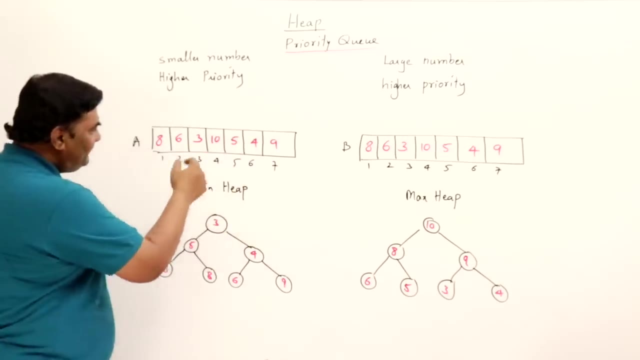 insert. suppose i have one more element, simply i can insert after this one. then when i want to delete from the this type of priority queue, i want three, then four. how much time it takes for deleting an element from an array order of n? because if i am deleting three i should shift. 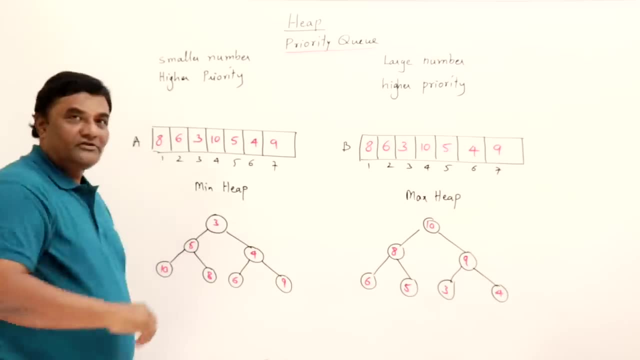 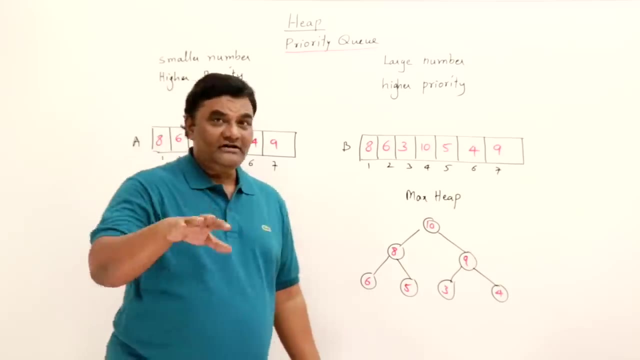 the rest of the elements, rest of the elements, and then i can insert another element and then i can insert another element. i should shift so it takes order of n time. so if you implement priority queue just using normal array, then the time for insert or delete may be order of n. so i don't want to. 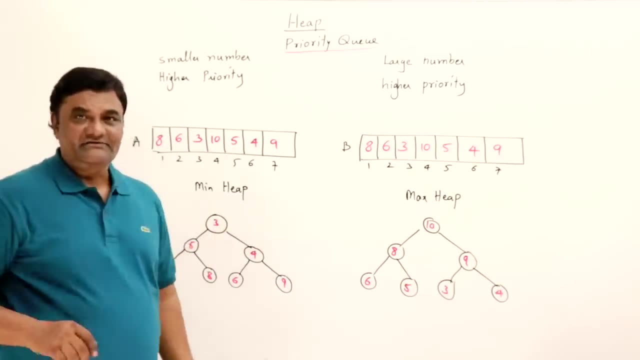 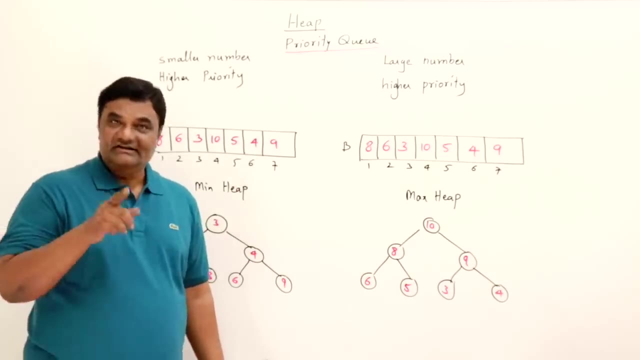 discuss in detail. you can study it by yourself means you can analyze by yourself. if you say no, i want to keep them sorted. order then for sorting. also, it takes time again for deletion or insertion. you have to spend order of n time then what is a better method? heap, which takes how much time. 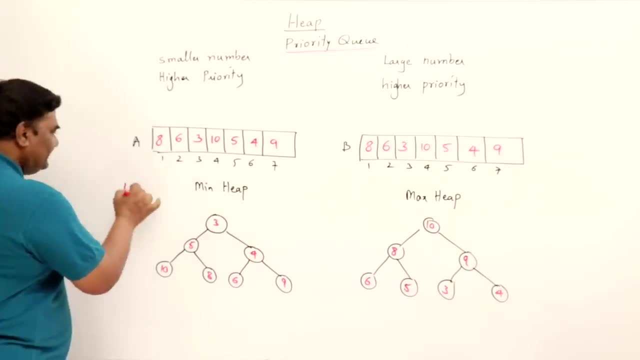 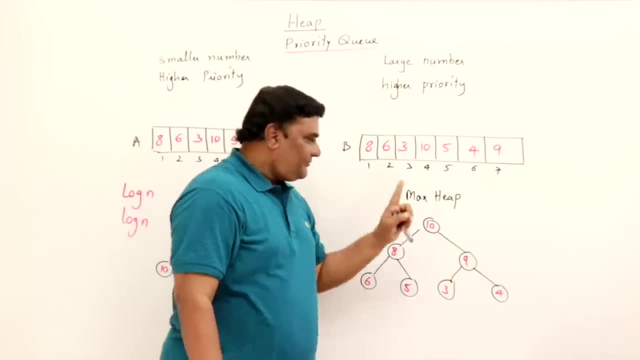 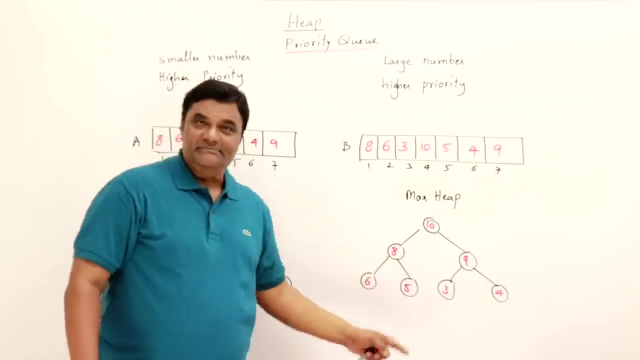 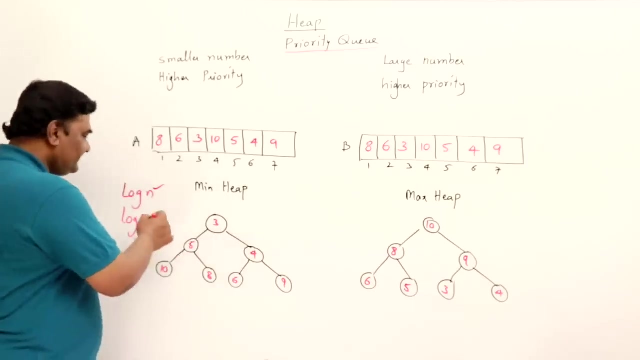 min heap. if you have larger number, higher priority, then use max heap. same set of numbers i have created, already created a min heap, already created max heap. so for one element insertion, how much time it takes log n right. then one element, deletion: how much time it takes log n time for insertion. 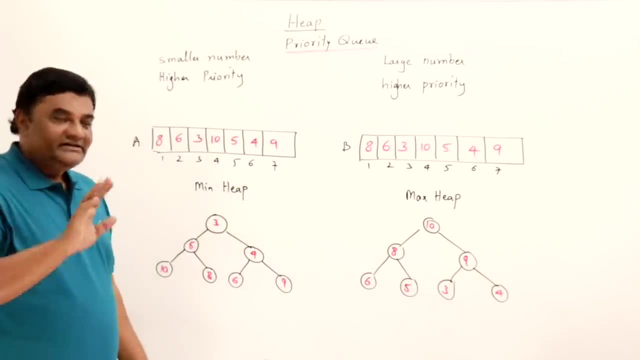 OK, now let us see how to insert and delete. See in an array: if I want to insert- suppose I have one more element- simply I can insert after this one, Then when I want to delete from this type of priority queue, I want three, then four. 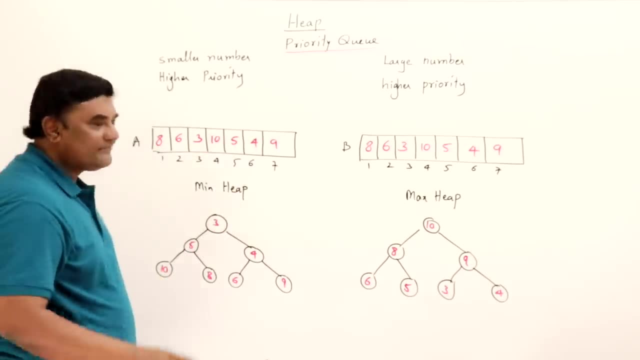 How much time it takes for deleting an element from an array. Order of n, Because if I am deleting three, I should shift the rest of the elements. Rest of the elements I should shift. So it takes order of n time. So if you implement priority queue just using normal array, 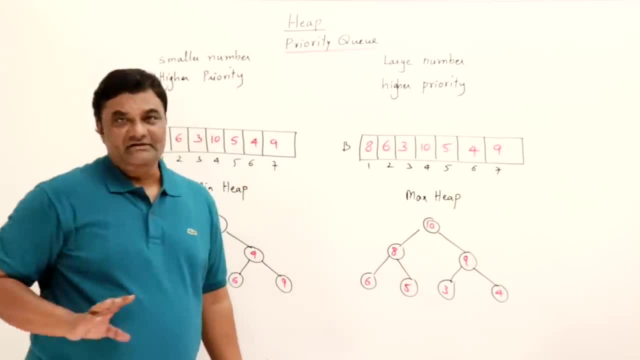 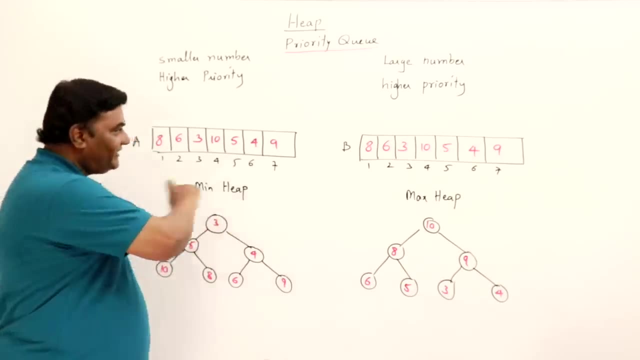 then the time for insert or delete may be. order of n. So I don't want to discuss in detail. You can study it by yourself. Means: you can analyze by yourself. If you say no, I want to keep them sorted. order, then for sorting also it takes.